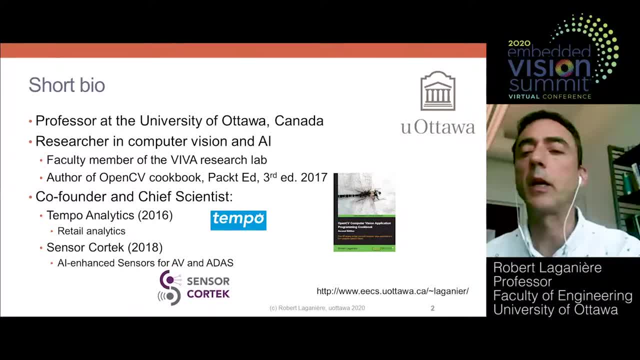 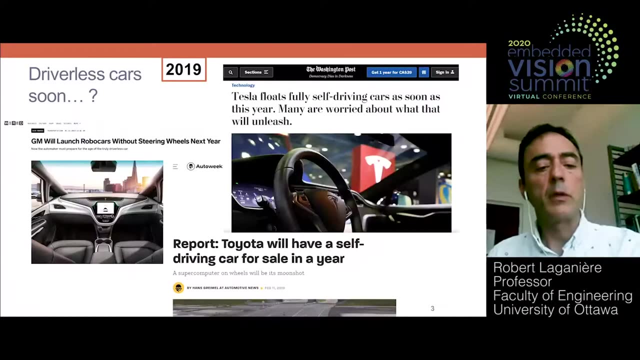 And I'm also involved with a number of startup companies, in particular Tempo Analytics, which is a company that is working on a new technology, which is called Tempo Analytics. The entire automation industry currently stand in as for the development of driverless vehicle. 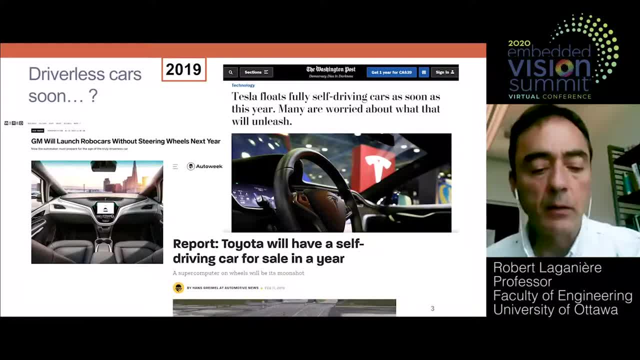 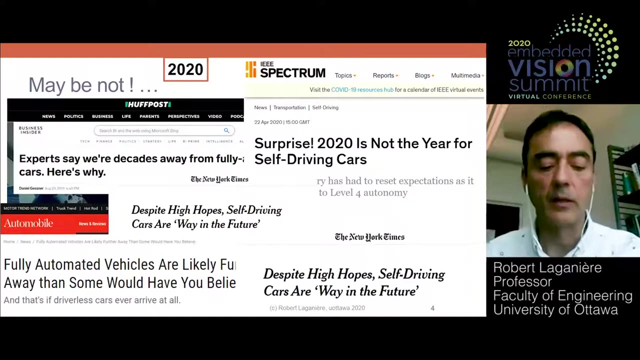 And, as you can see from these headlines, the automaker seems to be very optimistic for a quick development of fully autonomous vehicle. But these articles are from more than a year ago. If we look at the 2020 article, the message is quite different and the industry doesn't seem to be anymore that optimistic. 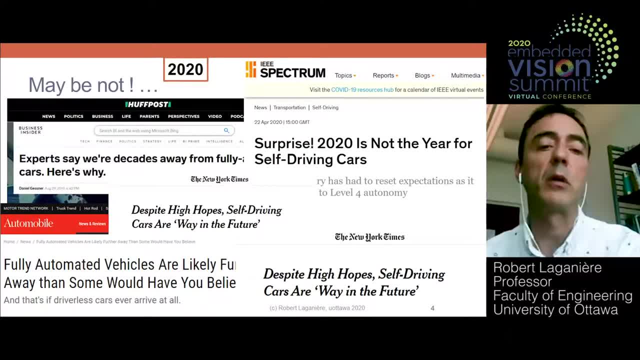 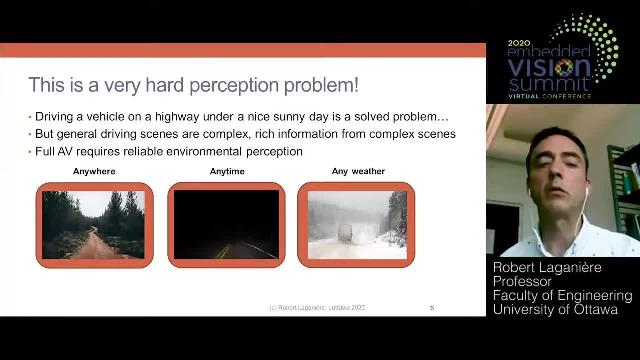 in terms of the development of real autonomous vehicles. Why is that? Well, because even if today, from the recent advance in artificial intelligence, we can say that driving a vehicle on the highway on a sunny day can be considered as a solved problem. 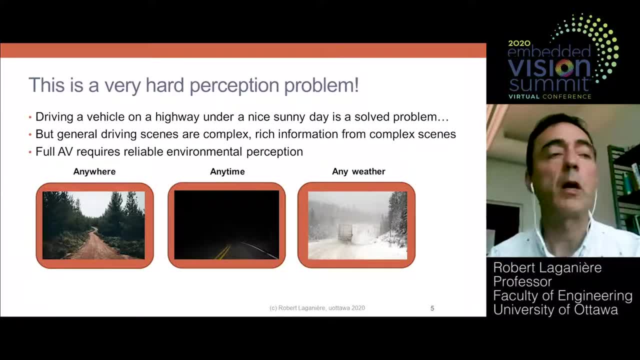 In general, we are far from having a real autonomous vehicle, If you think of a vehicle without steering wheel being able to drive anywhere anytime, under any weather condition. the problem is more, Much more difficult. In fact, this is basically a perception problem, a very, very difficult perception problem. 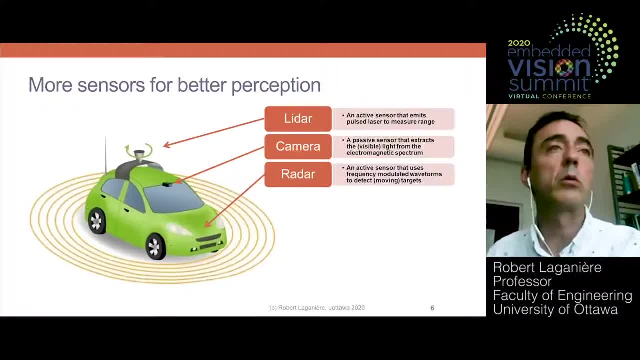 So one of the solutions in order to improve the perception of autonomous vehicles, in order to make them more autonomous well, is to add multiple sensors to these vehicles, So use and to use multiple types. So the main ones that are currently used are the following: 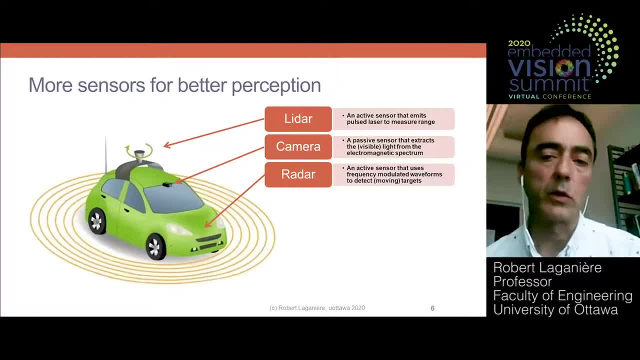 LiDAR or laser scanner. So this is a sensor based on laser that is able to measure distance from the vehicle to the driving, the objects of the driving scene. You have also the camera, which is a well-known sensor that captures the visible light. 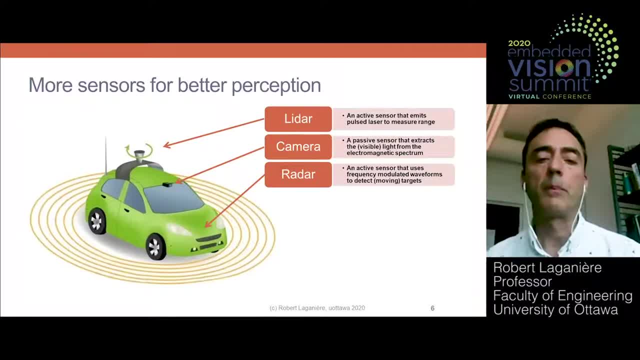 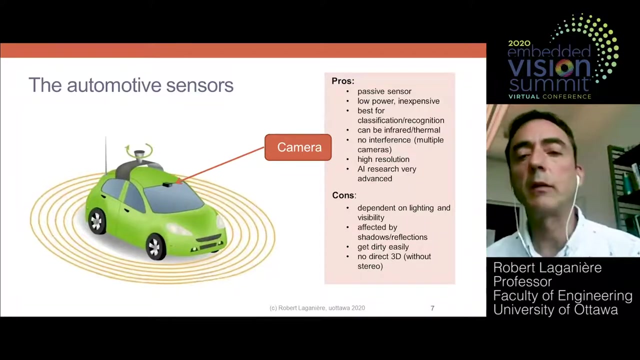 or, in some cases, can be extended to infrared and night vision. And you have the radar, which is also an active sensor and that uses waveform in order to detect moving target around the vehicle. So if we look at, if we look at each of these sensors, we can see that they each have their own advantages and disadvantages. 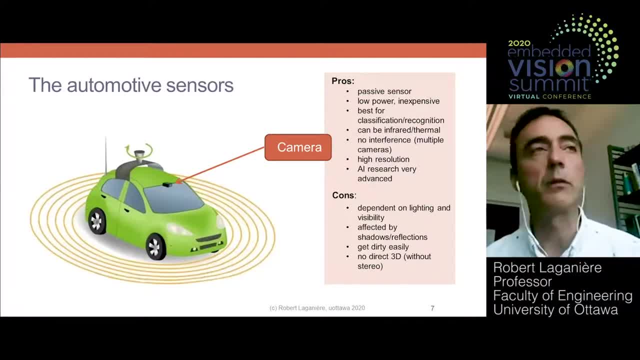 For example, the camera is a passive sensor, so it doesn't have to emit any signal in order to read the environment. It's a relatively low power sensor that is very strong at classifying, recognizing, detecting objects, as long as these ones are visible. 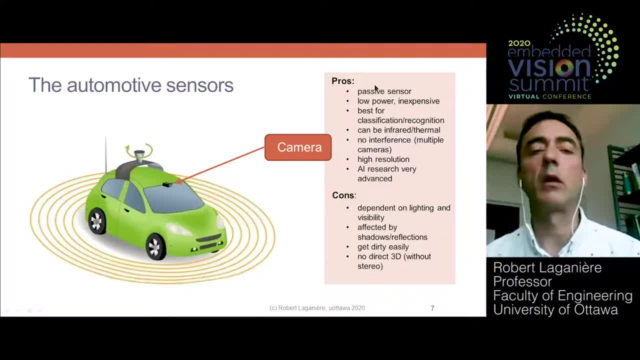 As I mentioned, you can also extend the visibility of objects beyond the visible spectrum, So you can use, for example, thermal cameras, And there's no interference when you use multiple cameras, cameras of relatively high resolution And also the research. 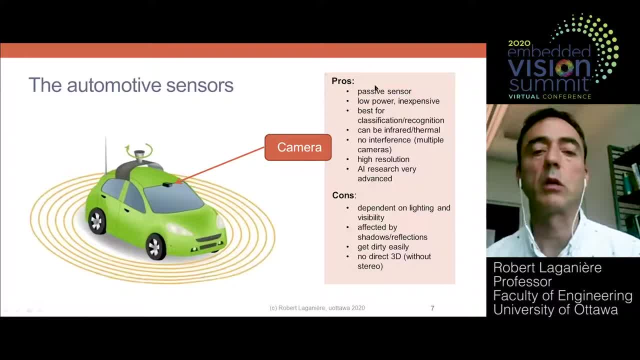 in the artificial intelligence. research with camera and images is very, very advanced. However, camera depends on visibility, so also on good lighting condition. They are very affected by shadows, reflection, heavy sun and also, very important, they get dirty very easily. 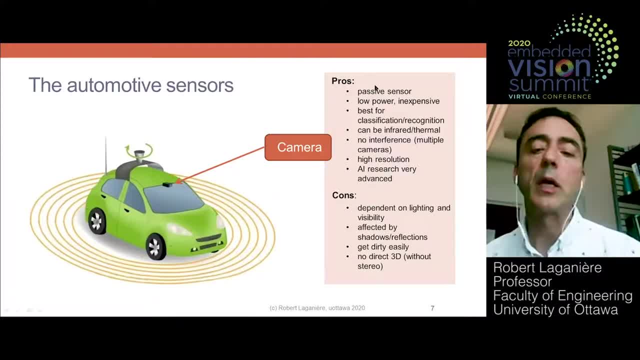 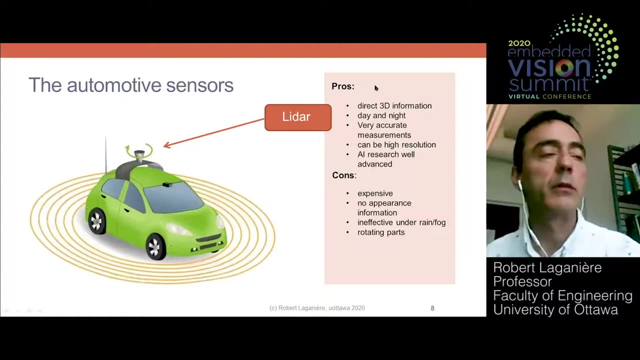 And a camera cannot provide direct 3D information unless you use a stereo system of camera, The LiDAR. the main benefit of these laser scanners is that they provide 3D information. They can work day and night. It's a very accurate sensor. 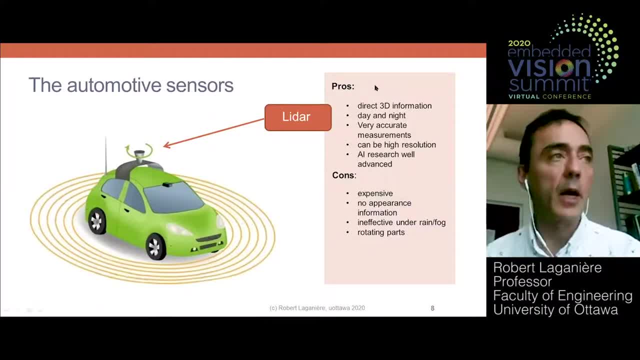 That can be of quite high resolution if you're ready to pay the price. That can be of quite high resolution if you're ready to pay the price. The research in artificial intelligence using LiDAR is also very well advanced. The research in artificial intelligence using LiDAR is also very well advanced. 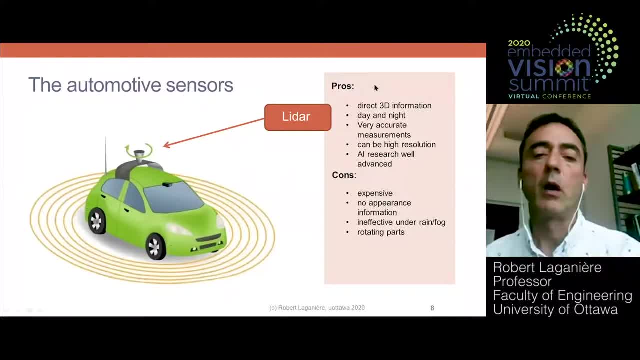 The research in artificial intelligence using LiDAR is also very well advanced. However, this is an expensive sensor and it does not provide any information about the appearance of object, which can make classification and recognition more difficult. However, this is an expensive sensor and it does not provide any information about the appearance of object, which can make classification and recognition more difficult. 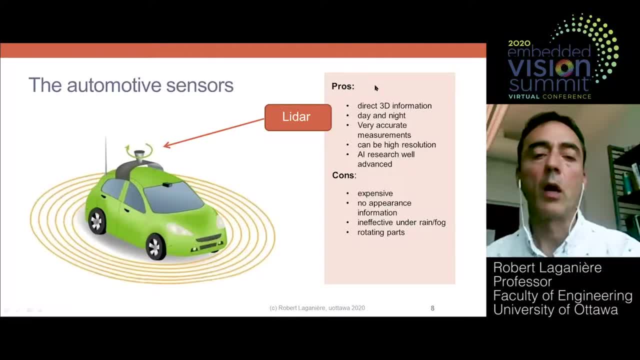 However, this is an expensive sensor and it does not provide any information about the appearance of object, which can make classification and recognition more difficult. However, this is an expensive sensor and it does not provide any information about the appearance of object, which can make classification and recognition more difficult. 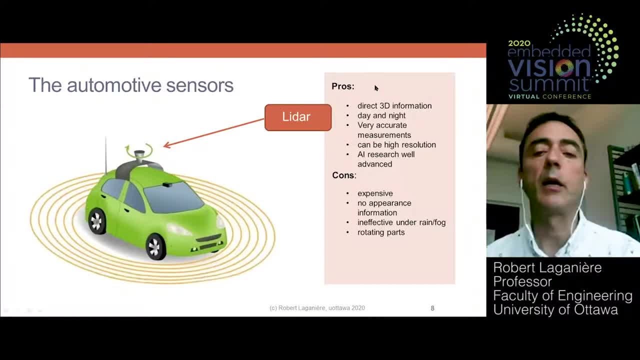 However, this is an expensive sensor and it does not provide any information about the appearance of object, which can make classification and recognition more difficult. However, this is an expensive sensor and it does not provide any information about the appearance of object, which can make classification and recognition more difficult. 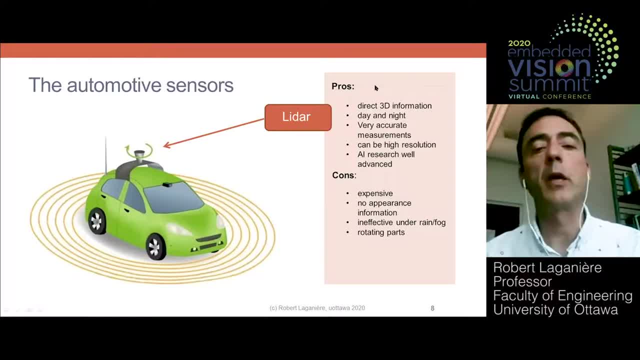 However, this is an expensive sensor and it does not provide any information about the appearance of object, which can make classification and recognition more difficult. However, this is an expensive sensor and it does not provide any information about the appearance of object, which can make classification and recognition more difficult. 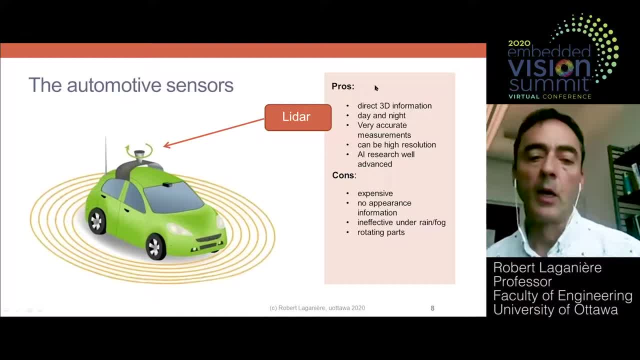 However, this is an expensive sensor and it does not provide any information about the appearance of object, which can make classification and recognition more difficult. However, this is an expensive sensor and it does not provide any information about the appearance of object, which can make classification and recognition more difficult. 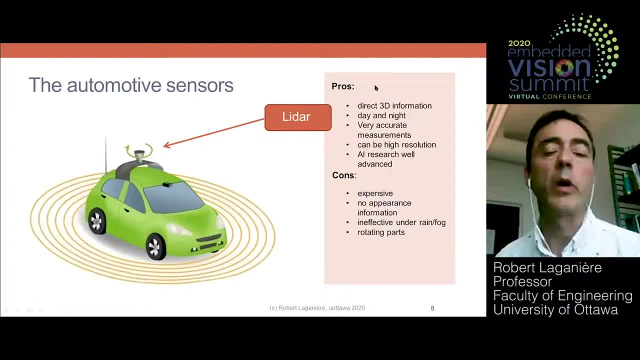 However, this is an expensive sensor and it does not provide any information about the appearance of object, which can make classification and recognition more difficult. However, this is an expensive sensor and it does not provide any information about the appearance of object, which can make classification and recognition more difficult. 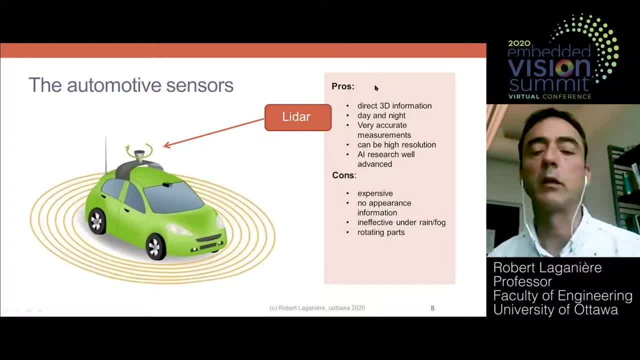 However, this is an expensive sensor and it does not provide any information about the appearance of object, which can make classification and recognition more difficult. However, this is an expensive sensor and it does not provide any information about the appearance of object, which can make classification and recognition more difficult. 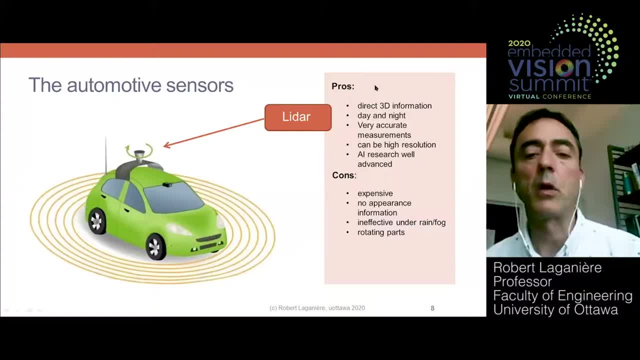 However, this is an expensive sensor and it does not provide any information about the appearance of object, which can make classification and recognition more difficult. However, this is an expensive sensor and it does not provide any information about the appearance of object, which can make classification and recognition more difficult. 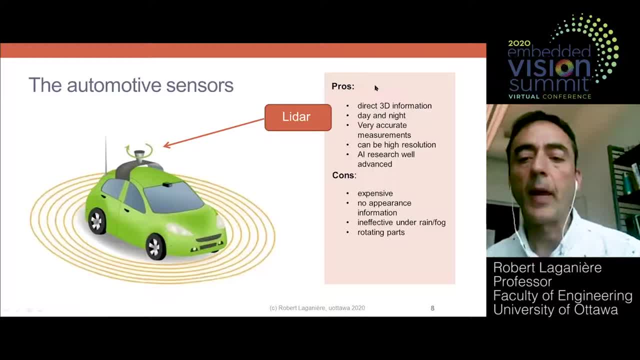 However, this is an expensive sensor and it does not provide any information about the appearance of object, which can make classification and recognition more difficult. However, this is an expensive sensor and it does not provide any information about the appearance of object, which can make classification and recognition more difficult. 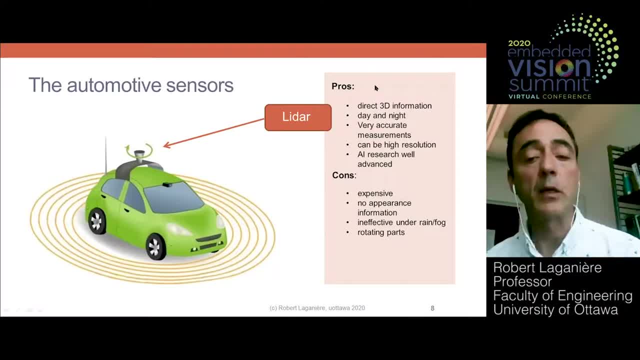 However, this is an expensive sensor and it does not provide any information about the appearance of object, which can make classification and recognition more difficult. However, this is an expensive sensor and it does not provide any information about the appearance of object, which can make classification and recognition more difficult. 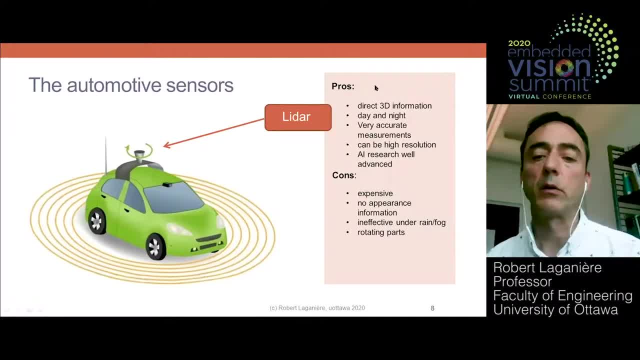 However, this is an expensive sensor and it does not provide any information about the appearance of object, which can make classification and recognition more difficult. However, this is an expensive sensor and it does not provide any information about the appearance of object, which can make classification and recognition more difficult. 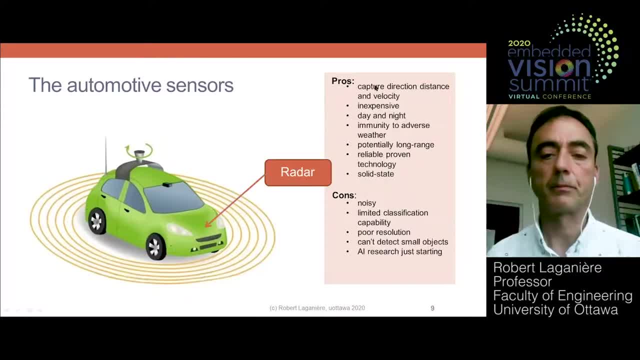 However, this is an expensive sensor and it does not provide any information about the appearance of object, which can make classification and recognition more difficult. However, this is an expensive sensor and it does not provide any information about the appearance of object, which can make classification and recognition more difficult. 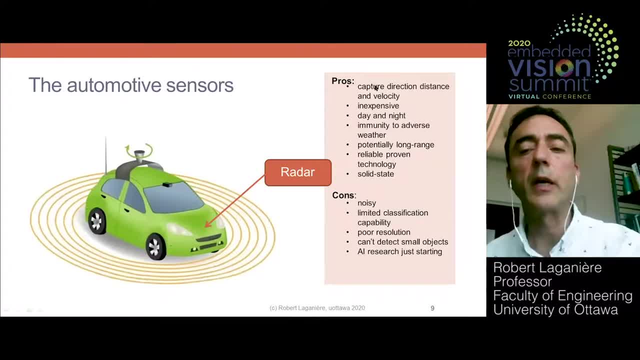 However, this is an expensive sensor and it does not provide any information about the appearance of object, which can make classification and recognition more difficult. However, this is an expensive sensor and it does not provide any information about the appearance of object, which can make classification and recognition more difficult. 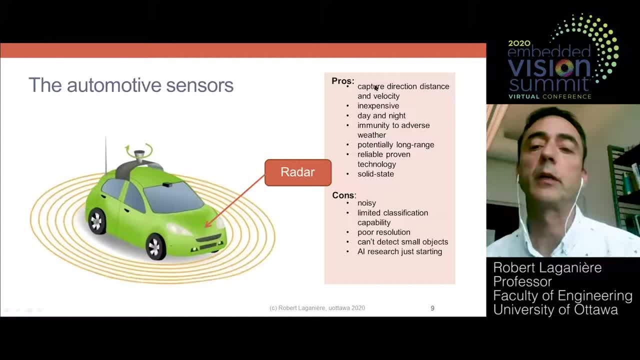 However, this is an expensive sensor and it does not provide any information about the appearance of object, which can make classification and recognition more difficult. However, this is an expensive sensor and it does not provide any information about the appearance of object, which can make classification and recognition more difficult. 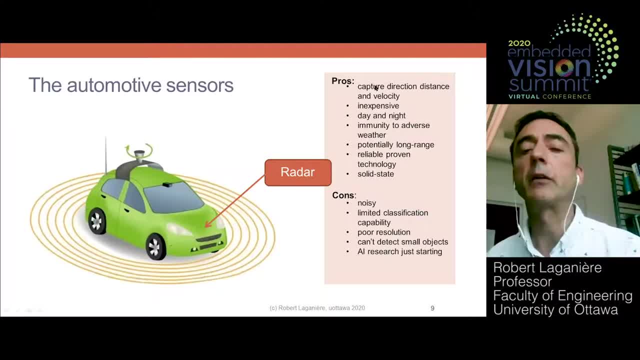 However, this is an expensive sensor and it does not provide any information about the appearance of object, which can make classification and recognition more difficult. However, this is an expensive sensor and it does not provide any information about the appearance of object, which can make classification and recognition more difficult. 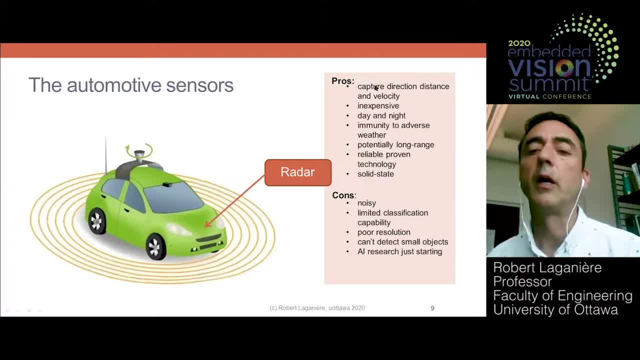 However, this is an expensive sensor and it does not provide any information about the appearance of object, which can make classification and recognition more difficult. However, this is an expensive sensor and it does not provide any information about the appearance of object, which can make classification and recognition more difficult. 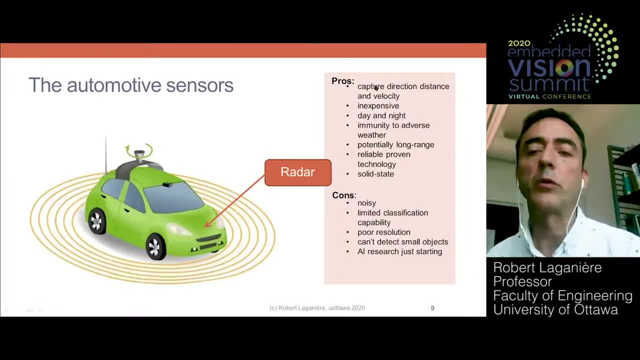 However, this is an expensive sensor and it does not provide any information about the appearance of object, which can make classification and recognition more difficult. However, this is an expensive sensor and it does not provide any information about the appearance of object, which can make classification and recognition more difficult. 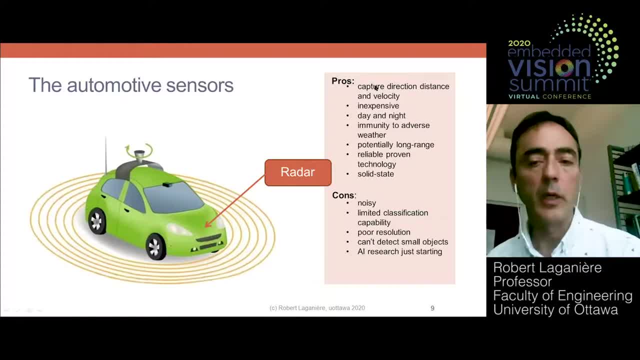 However, this is an expensive sensor and it does not provide any information about the appearance of object, which can make classification and recognition more difficult. However, this is an expensive sensor and it does not provide any information about the appearance of object, which can make classification and recognition more difficult. 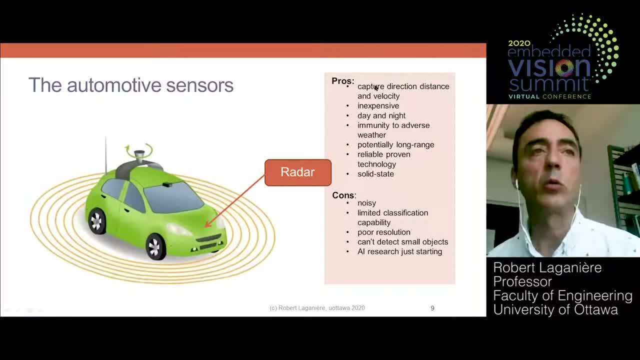 However, this is an expensive sensor and it does not provide any information about the appearance of object, which can make classification and recognition more difficult. However, this is an expensive sensor and it does not provide any information about the appearance of object, which can make classification and recognition more difficult. 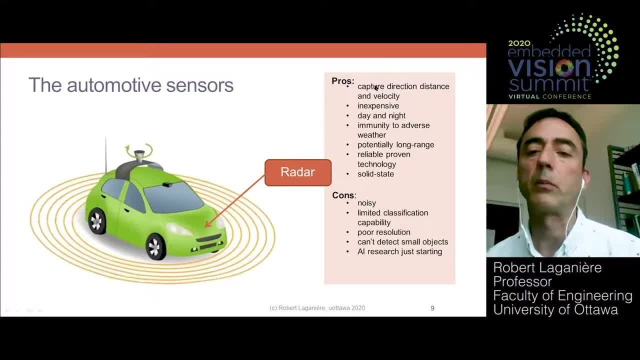 However, this is an expensive sensor and it does not provide any information about the appearance of object, which can make classification and recognition more difficult. However, this is an expensive sensor and it does not provide any information about the appearance of object, which can make classification and recognition more difficult. 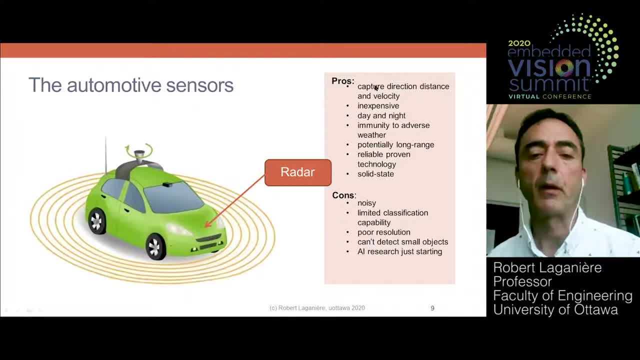 However, this is an expensive sensor and it does not provide any information about the appearance of object, which can make classification and recognition more difficult. However, this is an expensive sensor and it does not provide any information about the appearance of object, which can make classification and recognition more difficult. 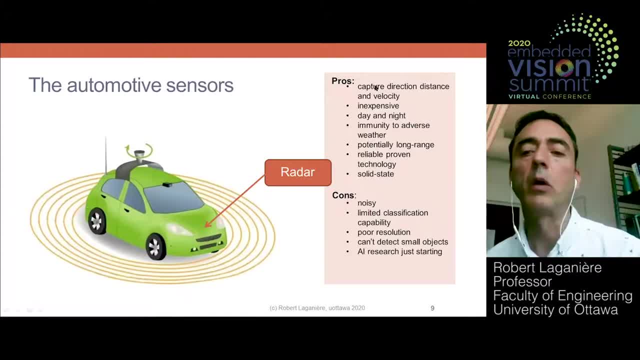 However, this is an expensive sensor and it does not provide any information about the appearance of object, which can make classification and recognition more difficult. However, this is an expensive sensor and it does not provide any information about the appearance of object, which can make classification and recognition more difficult. 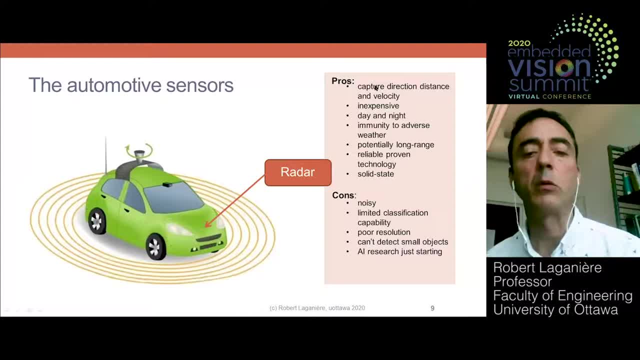 However, this is an expensive sensor and it does not provide any information about the appearance of object, which can make classification and recognition more difficult. However, this is an expensive sensor and it does not provide any information about the appearance of object, which can make classification and recognition more difficult. 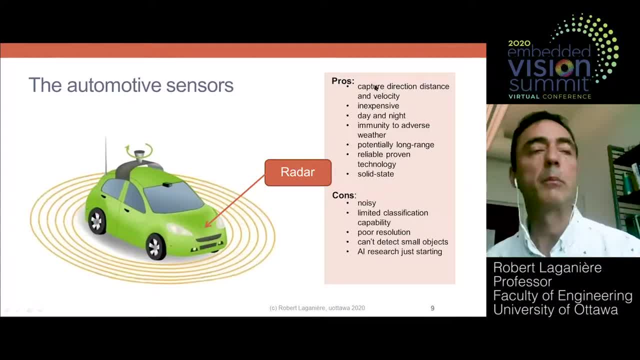 However, this is an expensive sensor and it does not provide any information about the appearance of object, which can make classification and recognition more difficult. However, this is an expensive sensor and it does not provide any information about the appearance of object, which can make classification and recognition more difficult. 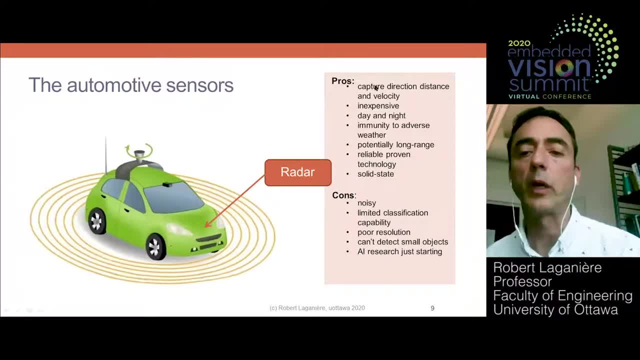 However, this is an expensive sensor and it does not provide any information about the appearance of object, which can make classification and recognition more difficult. However, this is an expensive sensor and it does not provide any information about the appearance of object, which can make classification and recognition more difficult. 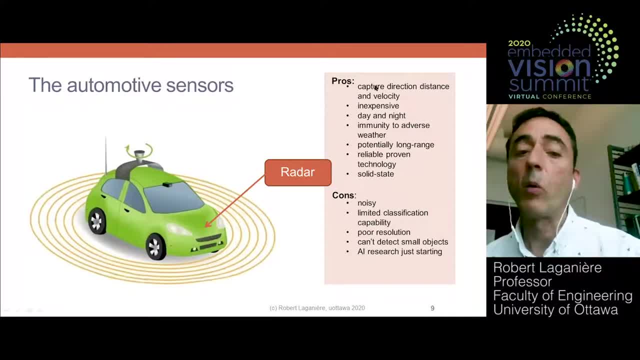 However, this is an expensive sensor and it does not provide any information about the appearance of object, which can make classification and recognition more difficult. However, this is an expensive sensor and it does not provide any information about the appearance of object, which can make classification and recognition more difficult. 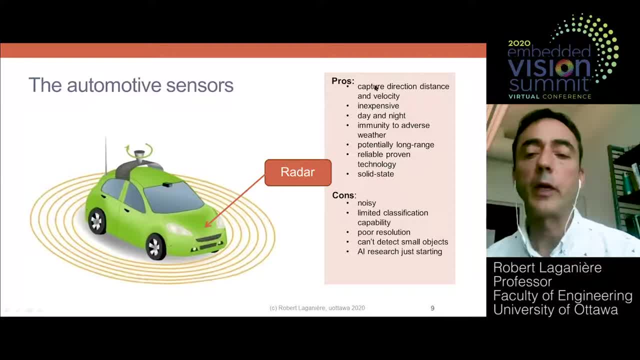 However, this is an expensive sensor and it does not provide any information about the appearance of object, which can make classification and recognition more difficult. However, this is an expensive sensor and it does not provide any information about the appearance of object, which can make classification and recognition more difficult. 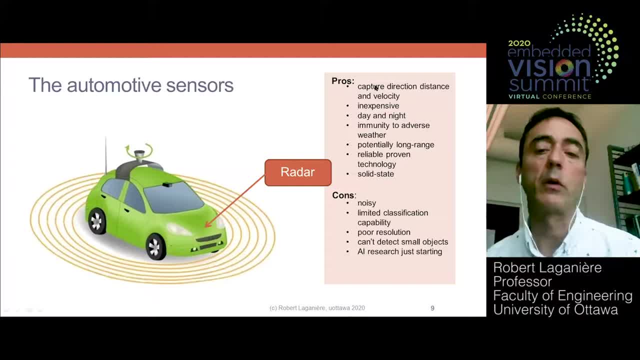 However, this is an expensive sensor and it does not provide any information about the appearance of object, which can make classification and recognition more difficult. However, this is an expensive sensor and it does not provide any information about the appearance of object, which can make classification and recognition more difficult. 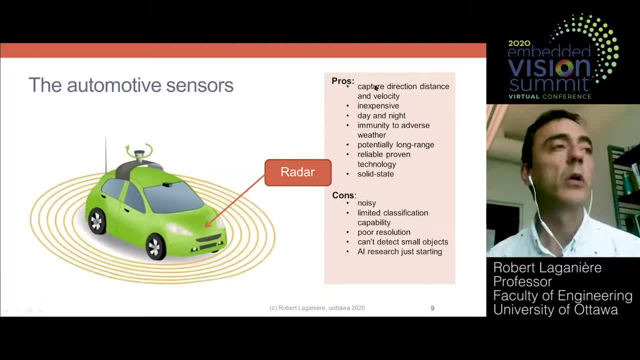 However, this is an expensive sensor and it does not provide any information about the appearance of object, which can make classification and recognition more difficult. However, this is an expensive sensor and it does not provide any information about the appearance of object, which can make classification and recognition more difficult. 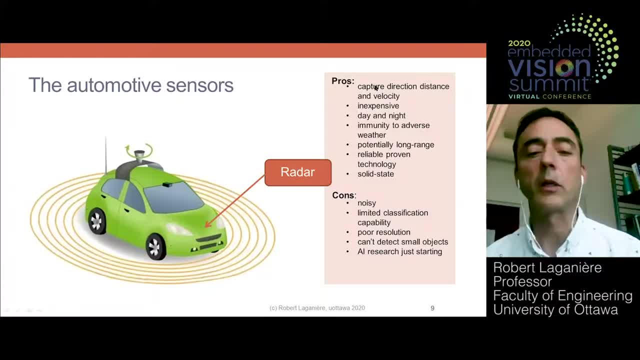 However, this is an expensive sensor and it does not provide any information about the appearance of object, which can make classification and recognition more difficult. However, this is an expensive sensor and it does not provide any information about the appearance of object, which can make classification and recognition more difficult. 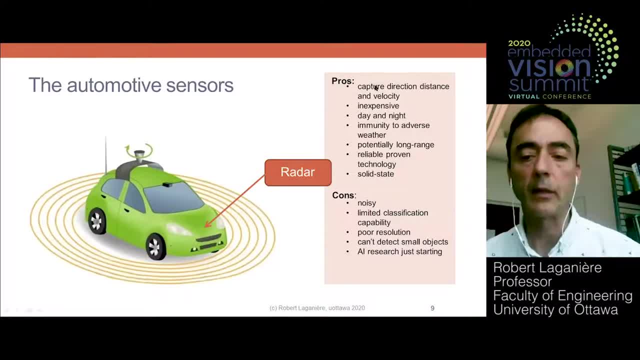 However, this is an expensive sensor and it does not provide any information about the appearance of object, which can make classification and recognition more difficult. However, this is an expensive sensor and it does not provide any information about the appearance of object, which can make classification and recognition more difficult. 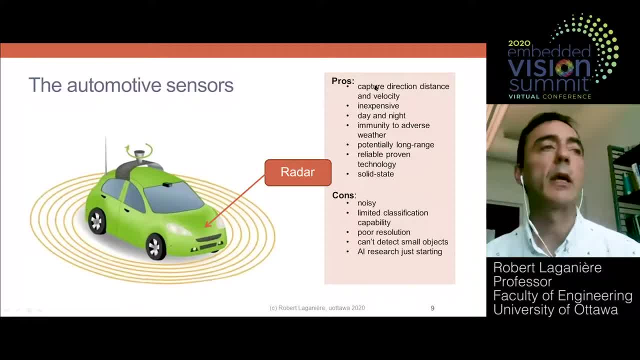 However, this is an expensive sensor and it does not provide any information about the appearance of object, which can make classification and recognition more difficult. However, this is an expensive sensor and it does not provide any information about the appearance of object, which can make classification and recognition more difficult. 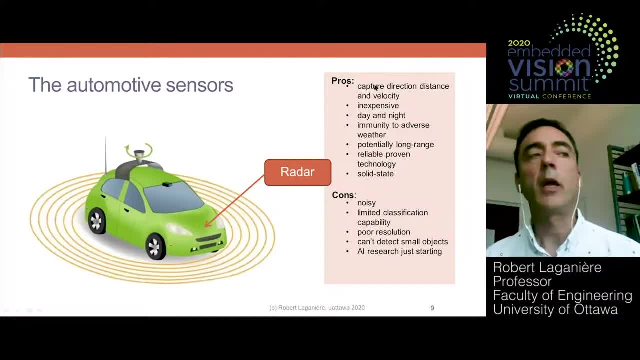 However, this is an expensive sensor and it does not provide any information about the appearance of object, which can make classification and recognition more difficult. However, this is an expensive sensor and it does not provide any information about the appearance of object, which can make classification and recognition more difficult. 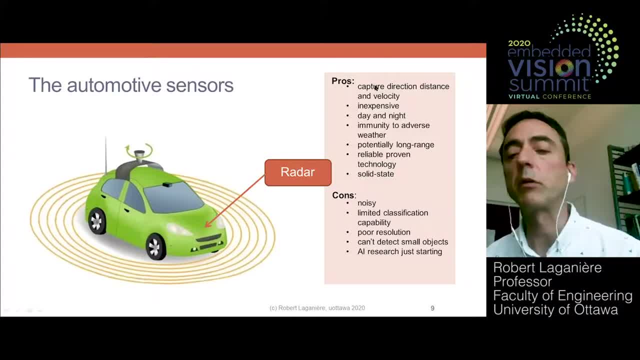 However, this is an expensive sensor and it does not provide any information about the appearance of object, which can make classification and recognition more difficult. However, this is an expensive sensor and it does not provide any information about the appearance of object, which can make classification and recognition more difficult. 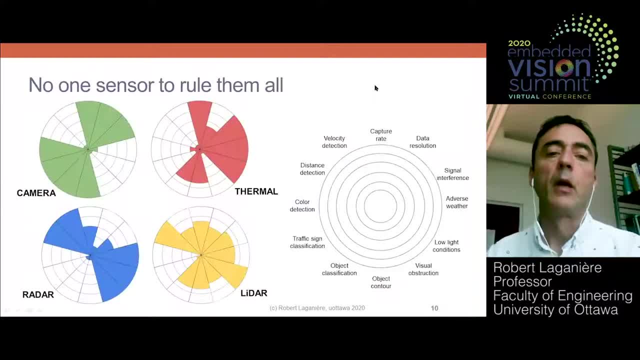 However, this is an expensive sensor and it does not provide any information about the appearance of object, which can make classification and recognition more difficult. However, this is an expensive sensor and it does not provide any information about the appearance of object, which can make classification and recognition more difficult. 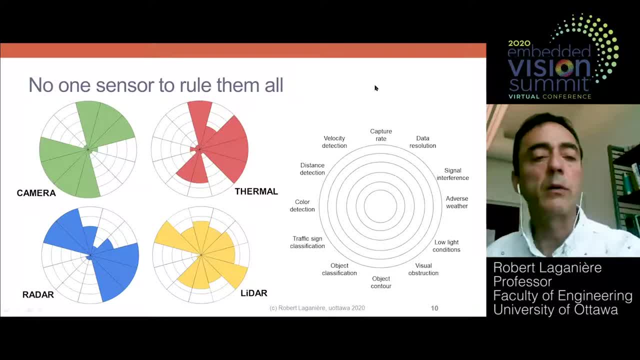 However, this is an expensive sensor and it does not provide any information about the appearance of object, which can make classification and recognition more difficult. However, this is an expensive sensor and it does not provide any information about the appearance of object, which can make classification and recognition more difficult. 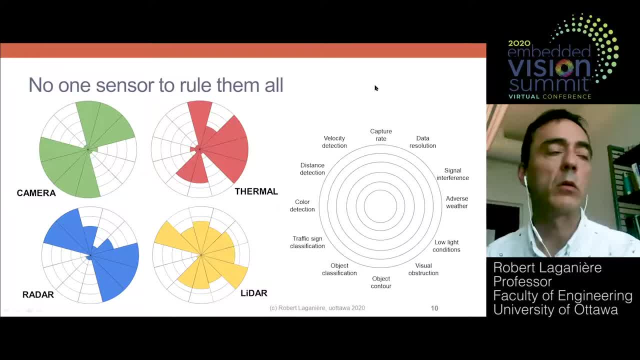 However, this is an expensive sensor and it does not provide any information about the appearance of object, which can make classification and recognition more difficult. However, this is an expensive sensor and it does not provide any information about the appearance of object, which can make classification and recognition more difficult. 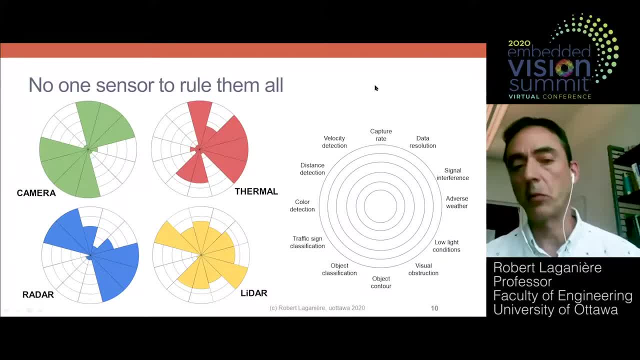 However, this is an expensive sensor and it does not provide any information about the appearance of object, which can make classification and recognition more difficult. However, this is an expensive sensor and it does not provide any information about the appearance of object, which can make classification and recognition more difficult. 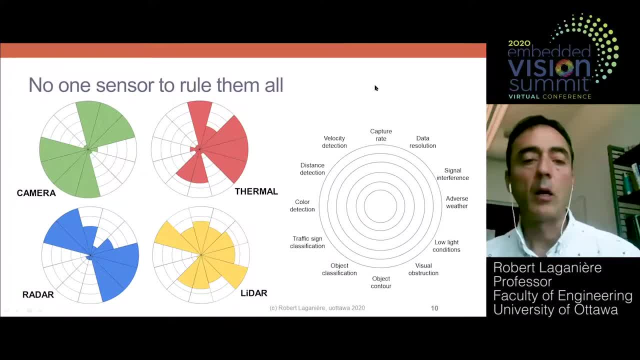 However, this is an expensive sensor and it does not provide any information about the appearance of object, which can make classification and recognition more difficult. However, this is an expensive sensor and it does not provide any information about the appearance of object, which can make classification and recognition more difficult. 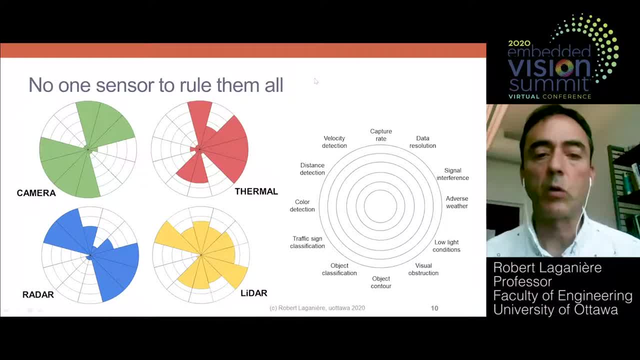 However, this is an expensive sensor and it does not provide any information about the appearance of object, which can make classification and recognition more difficult. However, this is an expensive sensor and it does not provide any information about the appearance of object, which can make classification and recognition more difficult. 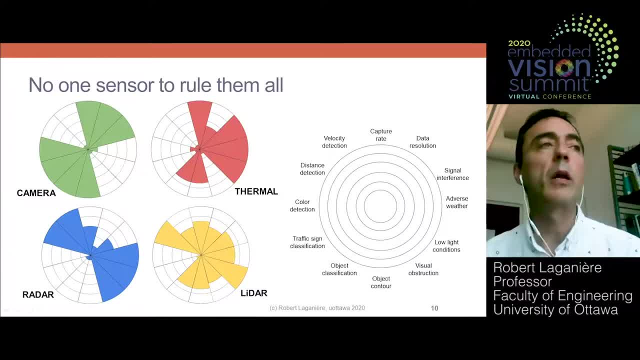 However, this is an expensive sensor and it does not provide any information about the appearance of object, which can make classification and recognition more difficult. However, this is an expensive sensor and it does not provide any information about the appearance of object, which can make classification and recognition more difficult. 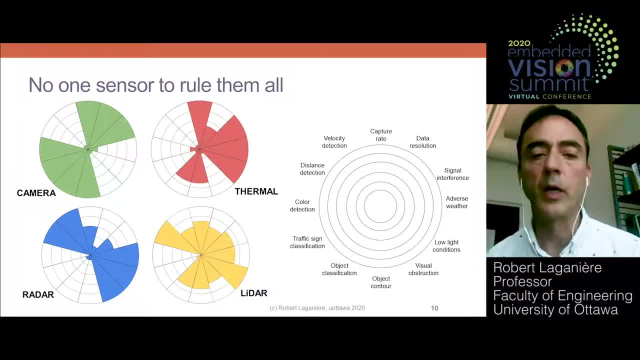 However, this is an expensive sensor and it does not provide any information about the appearance of object, which can make classification and recognition more difficult. However, this is an expensive sensor and it does not provide any information about the appearance of object, which can make classification and recognition more difficult. 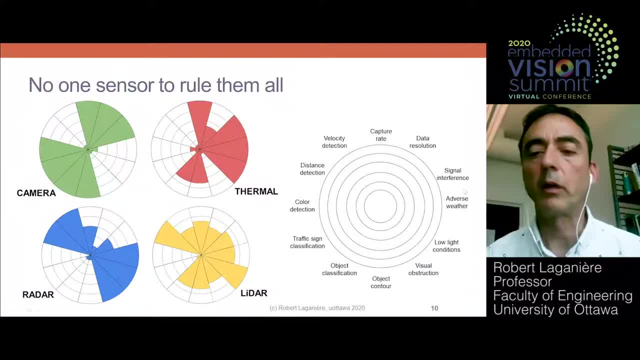 However, this is an expensive sensor and it does not provide any information about the appearance of object, which can make classification and recognition more difficult. However, this is an expensive sensor and it does not provide any information about the appearance of object, which can make classification and recognition more difficult. 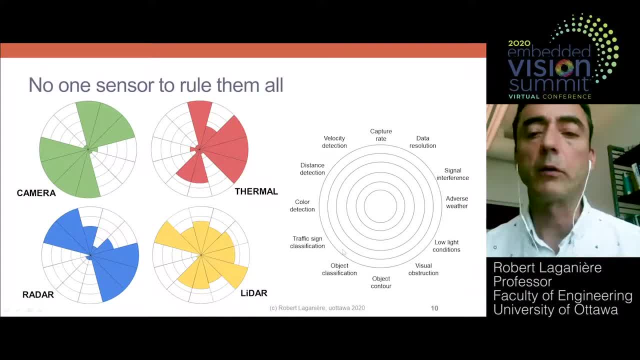 However, this is an expensive sensor and it does not provide any information about the appearance of object, which can make classification and recognition more difficult. However, this is an expensive sensor and it does not provide any information about the appearance of object, which can make classification and recognition more difficult. 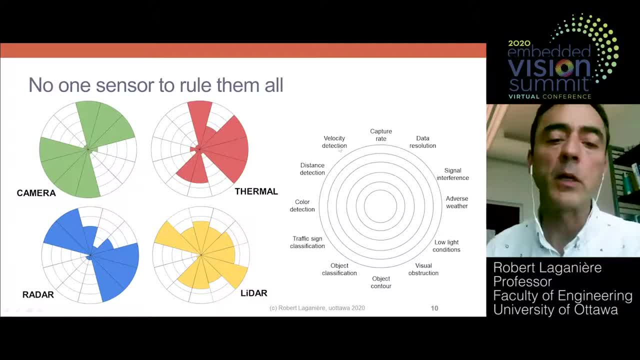 However, this is an expensive sensor and it does not provide any information about the appearance of object, which can make classification and recognition more difficult. However, this is an expensive sensor and it does not provide any information about the appearance of object, which can make classification and recognition more difficult. 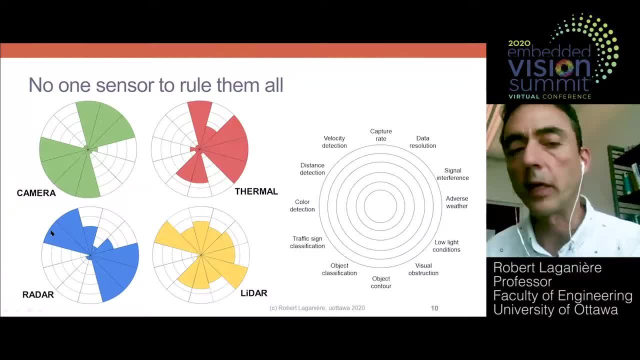 However, this is an expensive sensor and it does not provide any information about the appearance of object, which can make classification and recognition more difficult. However, this is an expensive sensor and it does not provide any information about the appearance of object, which can make classification and recognition more difficult. 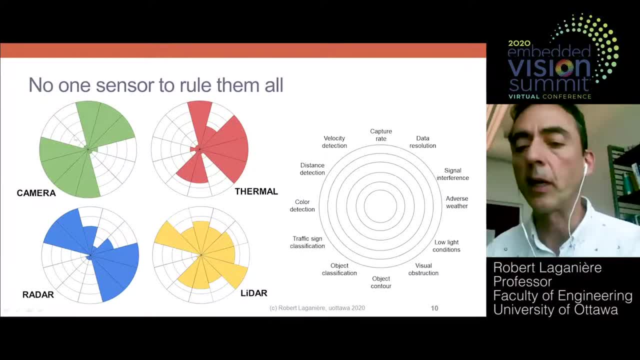 However, this is an expensive sensor and it does not provide any information about the appearance of object, which can make classification and recognition more difficult. However, this is an expensive sensor and it does not provide any information about the appearance of object, which can make classification and recognition more difficult. 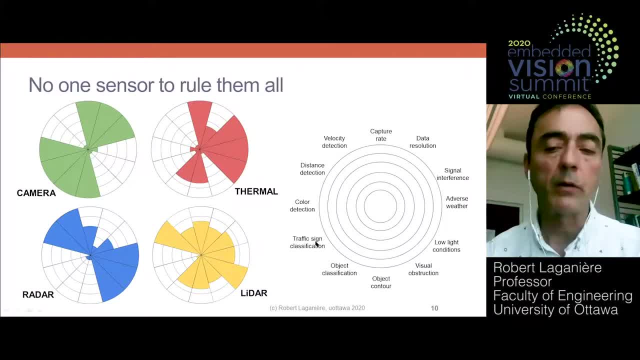 However, this is an expensive sensor and it does not provide any information about the appearance of object, which can make classification and recognition more difficult. However, this is an expensive sensor and it does not provide any information about the appearance of object, which can make classification and recognition more difficult. 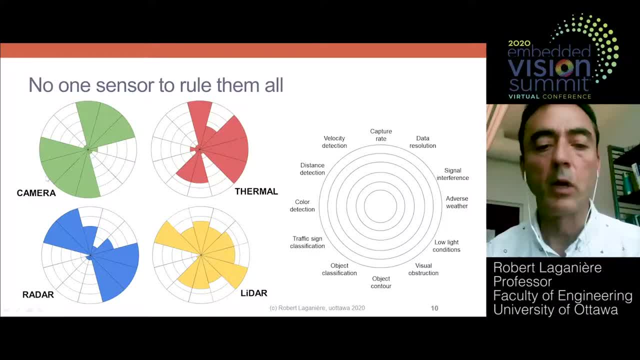 However, this is an expensive sensor and it does not provide any information about the appearance of object, which can make classification and recognition more difficult. However, this is an expensive sensor and it does not provide any information about the appearance of object, which can make classification and recognition more difficult. 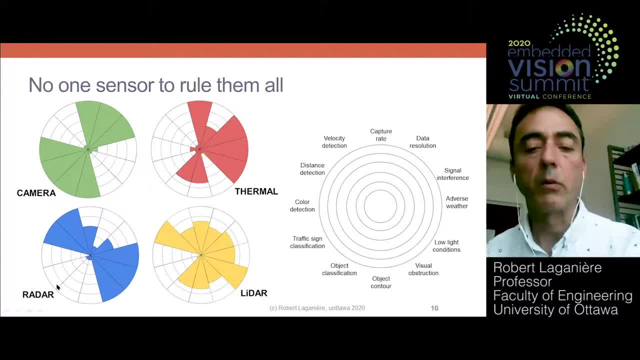 However, this is an expensive sensor and it does not provide any information about the appearance of object, which can make classification and recognition more difficult. However, this is an expensive sensor and it does not provide any information about the appearance of object, which can make classification and recognition more difficult. 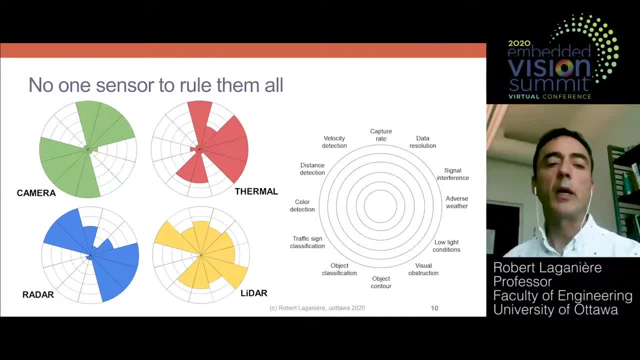 However, this is an expensive sensor and it does not provide any information about the appearance of object, which can make classification and recognition more difficult. However, this is an expensive sensor and it does not provide any information about the appearance of object, which can make classification and recognition more difficult. 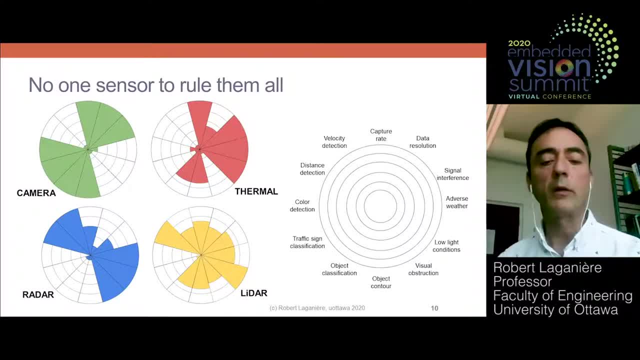 However, this is an expensive sensor and it does not provide any information about the appearance of object, which can make classification and recognition more difficult. However, this is an expensive sensor and it does not provide any information about the appearance of object, which can make classification and recognition more difficult. 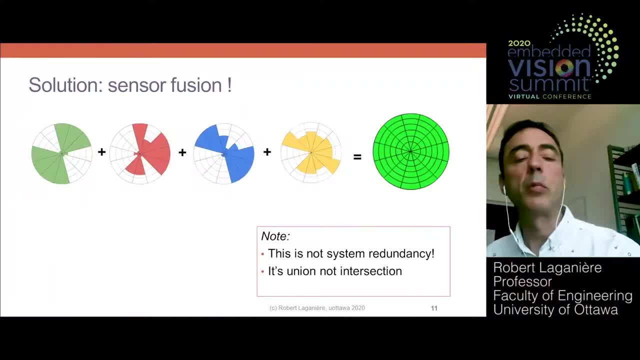 However, this is an expensive sensor and it does not provide any information about the appearance of object, which can make classification and recognition more difficult. However, this is an expensive sensor and it does not provide any information about the appearance of object, which can make classification and recognition more difficult. 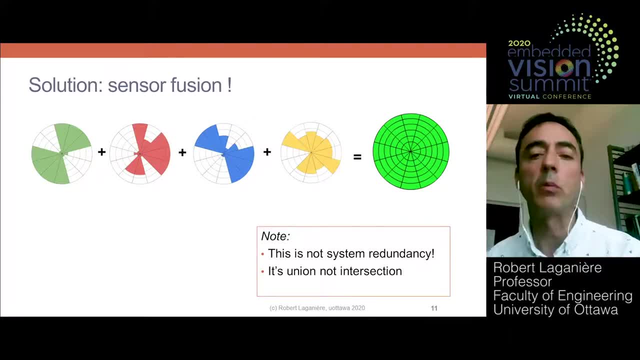 However, this is an expensive sensor and it does not provide any information about the appearance of object, which can make classification and recognition more difficult. However, this is an expensive sensor and it does not provide any information about the appearance of object, which can make classification and recognition more difficult. 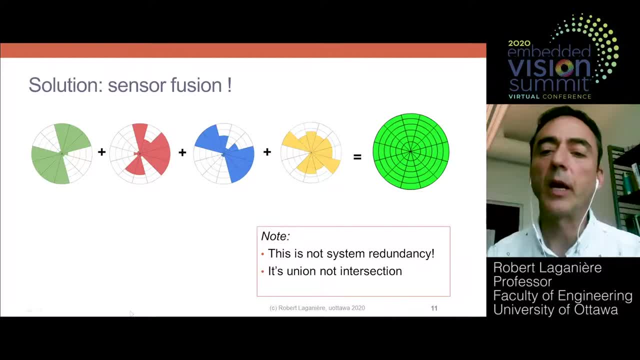 However, this is an expensive sensor and it does not provide any information about the appearance of object, which can make classification and recognition more difficult. However, this is an expensive sensor and it does not provide any information about the appearance of object, which can make classification and recognition more difficult. 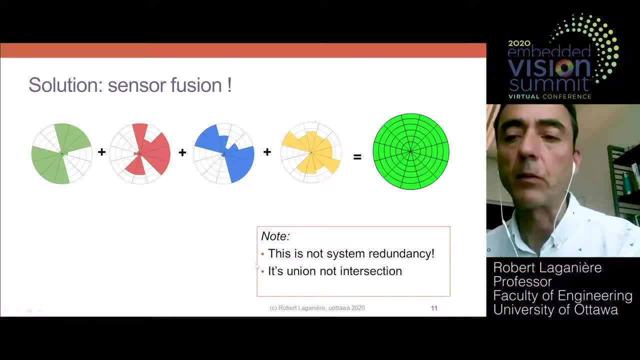 However, this is an expensive sensor and it does not provide any information about the appearance of object, which can make classification and recognition more difficult. However, this is an expensive sensor and it does not provide any information about the appearance of object, which can make classification and recognition more difficult. 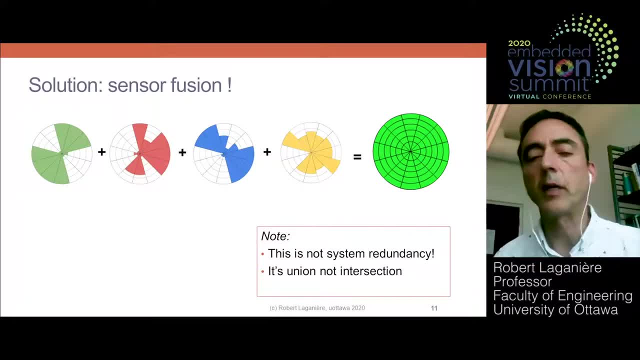 However, this is an expensive sensor and it does not provide any information about the appearance of object, which can make classification and recognition more difficult. However, this is an expensive sensor and it does not provide any information about the appearance of object, which can make classification and recognition more difficult. 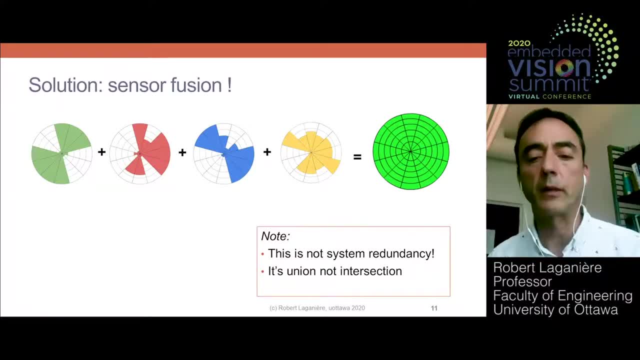 However, this is an expensive sensor and it does not provide any information about the appearance of object, which can make classification and recognition more difficult. However, this is an expensive sensor and it does not provide any information about the appearance of object, which can make classification and recognition more difficult. 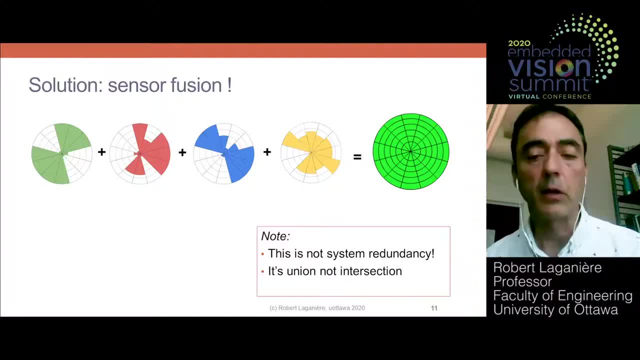 However, this is an expensive sensor and it does not provide any information about the appearance of object, which can make classification and recognition more difficult. However, this is an expensive sensor and it does not provide any information about the appearance of object, which can make classification and recognition more difficult. 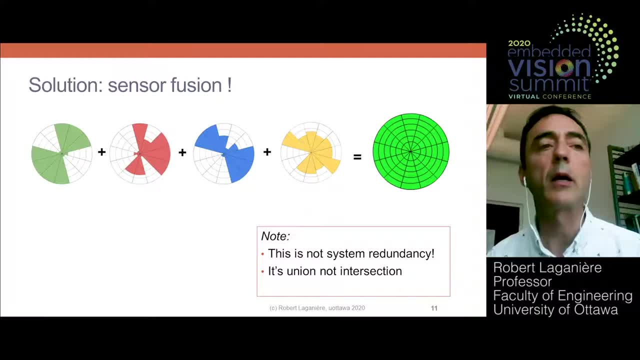 However, this is an expensive sensor and it does not provide any information about the appearance of object, which can make classification and recognition more difficult. However, this is an expensive sensor and it does not provide any information about the appearance of object, which can make classification and recognition more difficult. 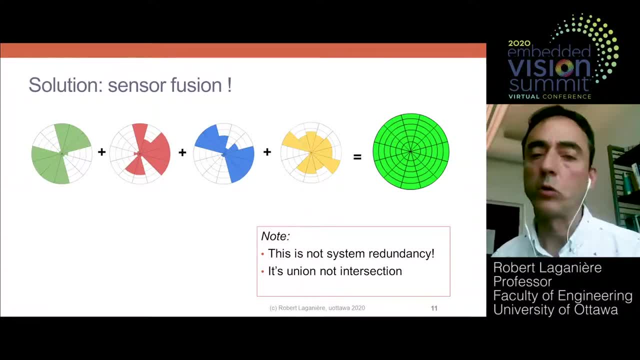 However, this is an expensive sensor and it does not provide any information about the appearance of object, which can make classification and recognition more difficult. However, this is an expensive sensor and it does not provide any information about the appearance of object, which can make classification and recognition more difficult. 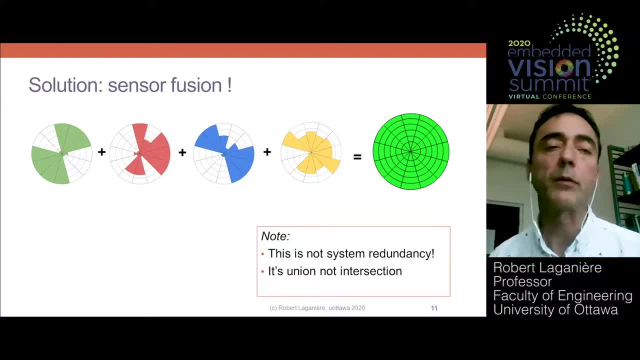 However, this is an expensive sensor and it does not provide any information about the appearance of object, which can make classification and recognition more difficult. However, this is an expensive sensor and it does not provide any information about the appearance of object, which can make classification and recognition more difficult. 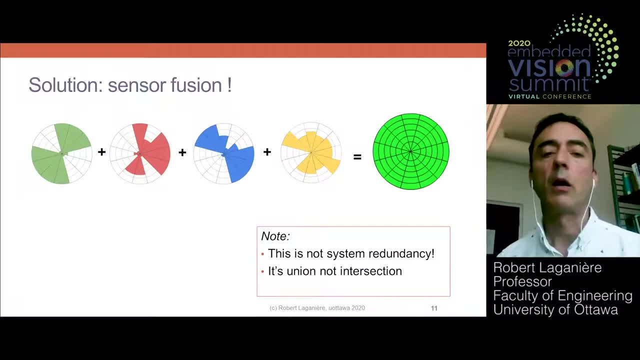 However, this is an expensive sensor and it does not provide any information about the appearance of object, which can make classification and recognition more difficult. However, this is an expensive sensor and it does not provide any information about the appearance of object, which can make classification and recognition more difficult. 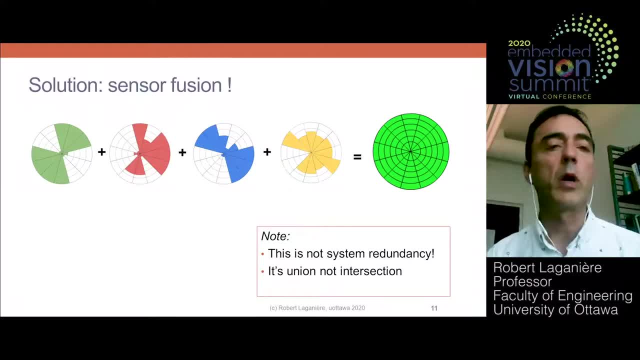 However, this is an expensive sensor and it does not provide any information about the appearance of object, which can make classification and recognition more difficult. However, this is an expensive sensor and it does not provide any information about the appearance of object, which can make classification and recognition more difficult. 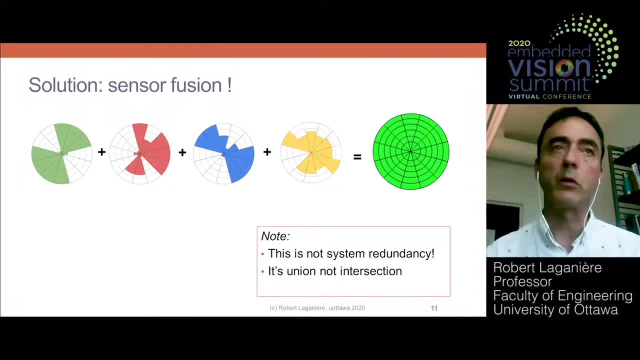 However, this is an expensive sensor and it does not provide any information about the appearance of object, which can make classification and recognition more difficult. However, this is an expensive sensor and it does not provide any information about the appearance of object, which can make classification and recognition more difficult. 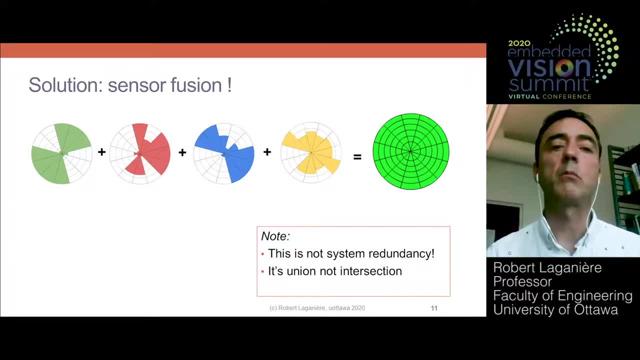 However, this is an expensive sensor and it does not provide any information about the appearance of object, which can make classification and recognition more difficult. However, this is an expensive sensor and it does not provide any information about the appearance of object, which can make classification and recognition more difficult. 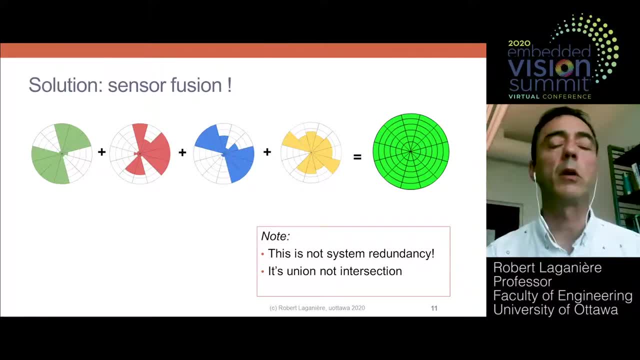 However, this is an expensive sensor and it does not provide any information about the appearance of object, which can make classification and recognition more difficult. However, this is an expensive sensor and it does not provide any information about the appearance of object, which can make classification and recognition more difficult. 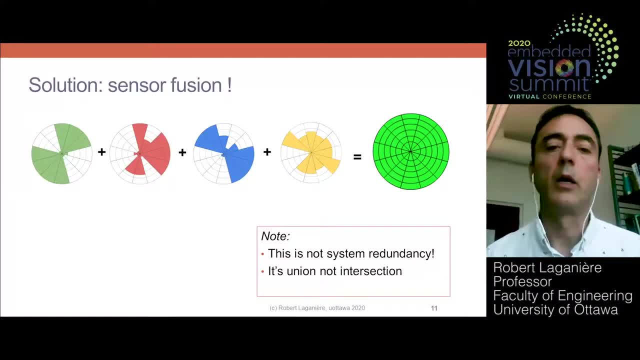 However, this is an expensive sensor and it does not provide any information about the appearance of object, which can make classification and recognition more difficult. However, this is an expensive sensor and it does not provide any information about the appearance of object, which can make classification and recognition more difficult. 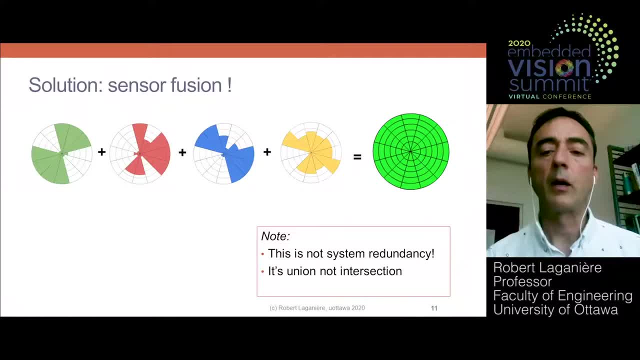 However, this is an expensive sensor and it does not provide any information about the appearance of object, which can make classification and recognition more difficult. However, this is an expensive sensor and it does not provide any information about the appearance of object, which can make classification and recognition more difficult. 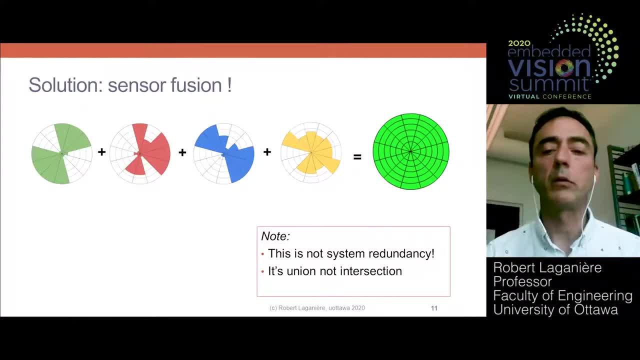 However, this is an expensive sensor and it does not provide any information about the appearance of object, which can make classification and recognition more difficult. However, this is an expensive sensor and it does not provide any information about the appearance of object, which can make classification and recognition more difficult. 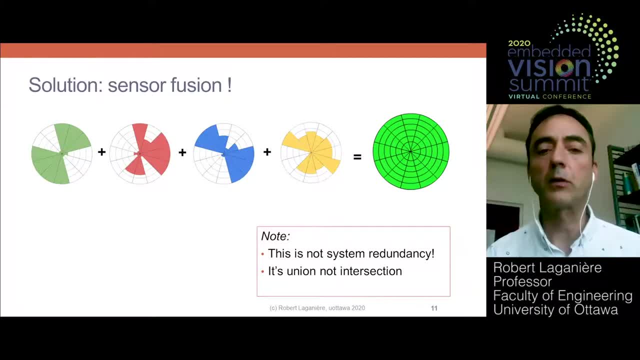 However, this is an expensive sensor and it does not provide any information about the appearance of object, which can make classification and recognition more difficult. However, this is an expensive sensor and it does not provide any information about the appearance of object, which can make classification and recognition more difficult. 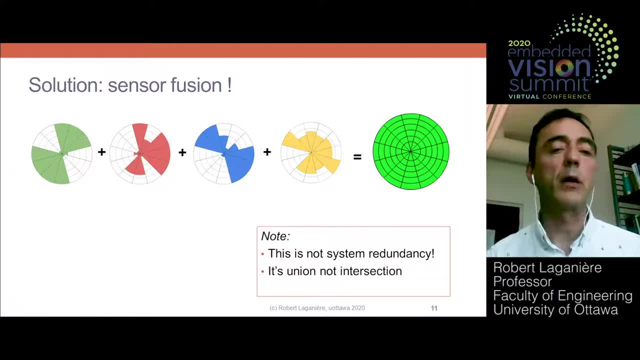 However, this is an expensive sensor and it does not provide any information about the appearance of object, which can make classification and recognition more difficult. However, this is an expensive sensor and it does not provide any information about the appearance of object, which can make classification and recognition more difficult. 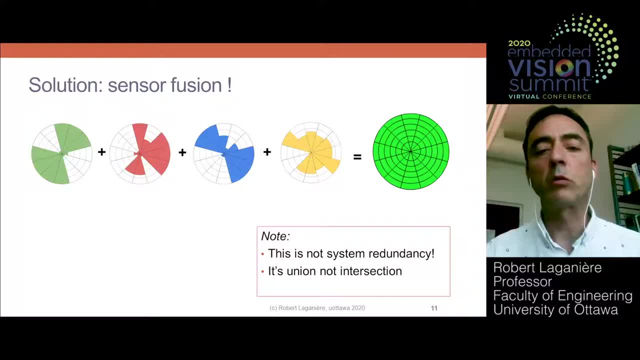 However, this is an expensive sensor and it does not provide any information about the appearance of object, which can make classification and recognition more difficult. However, this is an expensive sensor and it does not provide any information about the appearance of object, which can make classification and recognition more difficult. 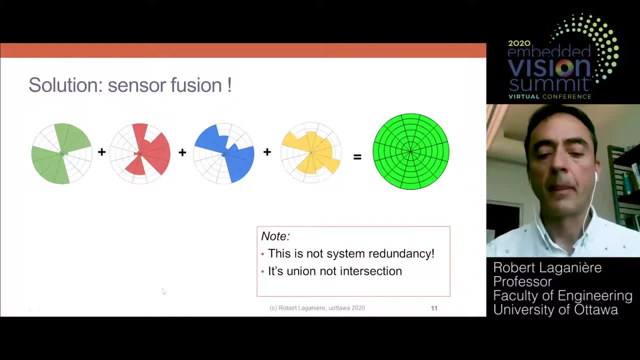 However, this is an expensive sensor and it does not provide any information about the appearance of object, which can make classification and recognition more difficult. However, this is an expensive sensor and it does not provide any information about the appearance of object, which can make classification and recognition more difficult. 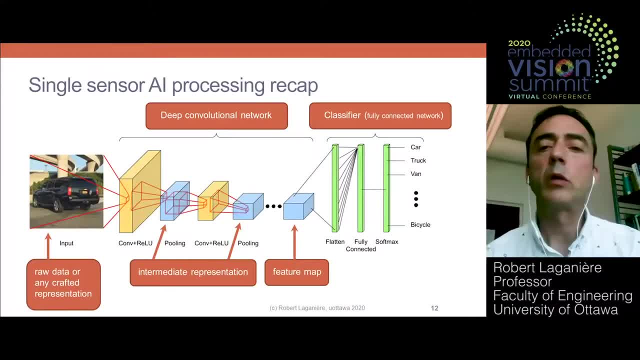 However, this is an expensive sensor and it does not provide any information about the appearance of object, which can make classification and recognition more difficult. However, this is an expensive sensor and it does not provide any information about the appearance of object, which can make classification and recognition more difficult. 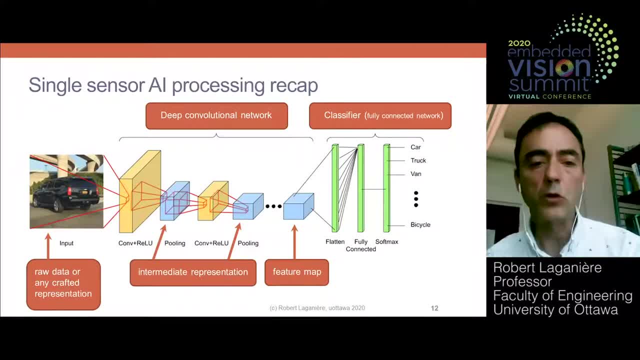 However, this is an expensive sensor and it does not provide any information about the appearance of object, which can make classification and recognition more difficult. However, this is an expensive sensor and it does not provide any information about the appearance of object, which can make classification and recognition more difficult. 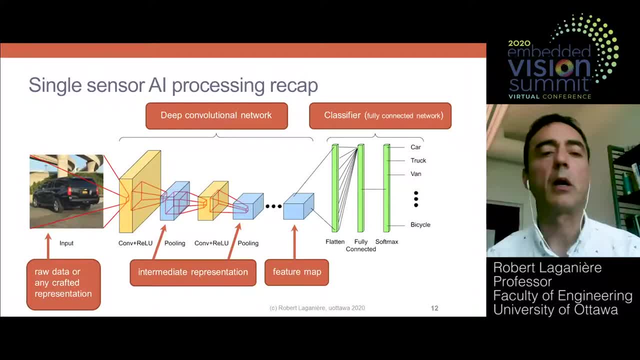 However, this is an expensive sensor and it does not provide any information about the appearance of object, which can make classification and recognition more difficult. However, this is an expensive sensor and it does not provide any information about the appearance of object, which can make classification and recognition more difficult. 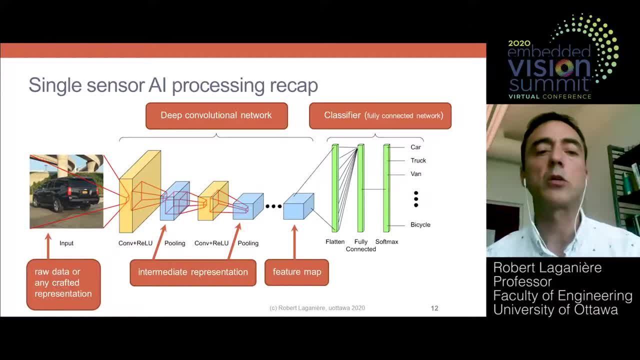 However, this is an expensive sensor and it does not provide any information about the appearance of object, which can make classification and recognition more difficult. However, this is an expensive sensor and it does not provide any information about the appearance of object, which can make classification and recognition more difficult. 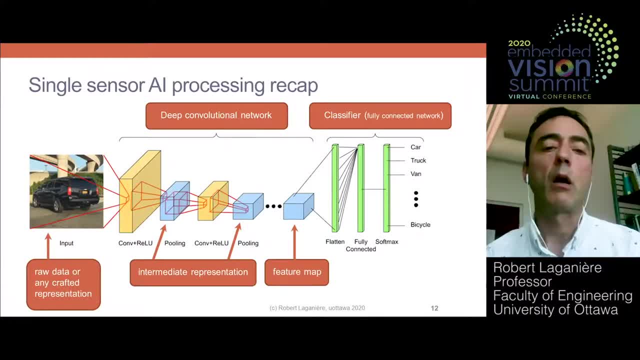 However, this is an expensive sensor and it does not provide any information about the appearance of object, which can make classification and recognition more difficult. However, this is an expensive sensor and it does not provide any information about the appearance of object, which can make classification and recognition more difficult. 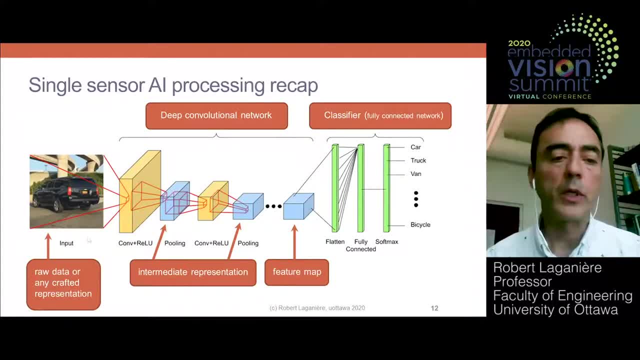 However, this is an expensive sensor and it does not provide any information about the appearance of object, which can make classification and recognition more difficult. However, this is an expensive sensor and it does not provide any information about the appearance of object, which can make classification and recognition more difficult. 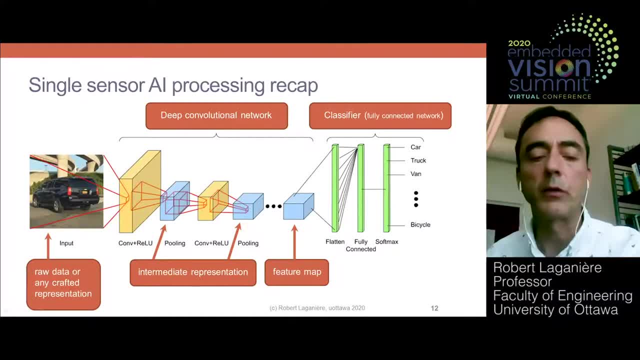 However, this is an expensive sensor and it does not provide any information about the appearance of object, which can make classification and recognition more difficult. However, this is an expensive sensor and it does not provide any information about the appearance of object, which can make classification and recognition more difficult. 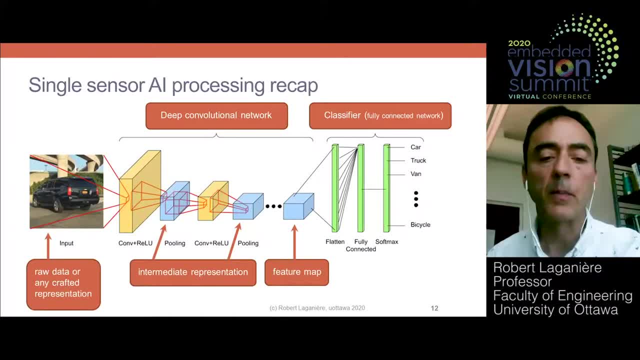 However, this is an expensive sensor and it does not provide any information about the appearance of object, which can make classification and recognition more difficult. However, this is an expensive sensor and it does not provide any information about the appearance of object, which can make classification and recognition more difficult. 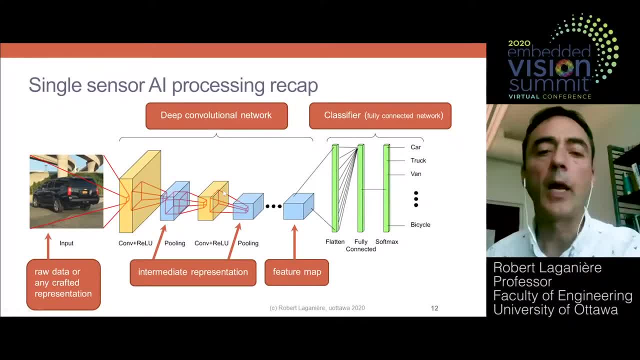 However, this is an expensive sensor and it does not provide any information about the appearance of object, which can make classification and recognition more difficult. However, this is an expensive sensor and it does not provide any information about the appearance of object, which can make classification and recognition more difficult. 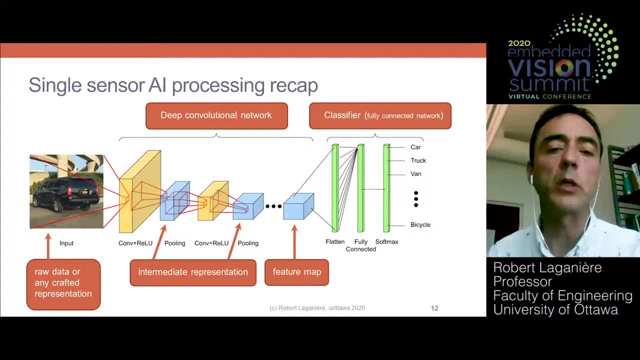 However, this is an expensive sensor and it does not provide any information about the appearance of object, which can make classification and recognition more difficult. However, this is an expensive sensor and it does not provide any information about the appearance of object, which can make classification and recognition more difficult. 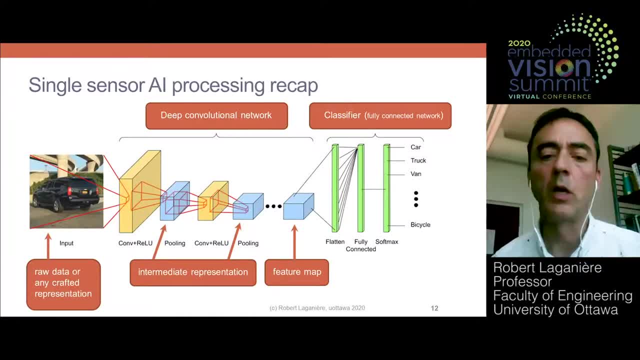 However, this is an expensive sensor and it does not provide any information about the appearance of object, which can make classification and recognition more difficult. However, this is an expensive sensor and it does not provide any information about the appearance of object, which can make classification and recognition more difficult. 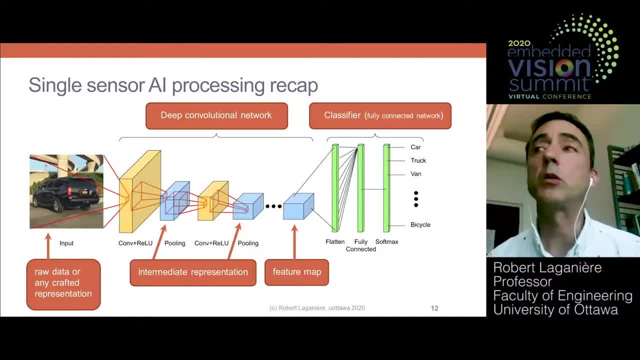 However, this is an expensive sensor and it does not provide any information about the appearance of object, which can make classification and recognition more difficult. However, this is an expensive sensor and it does not provide any information about the appearance of object, which can make classification and recognition more difficult. 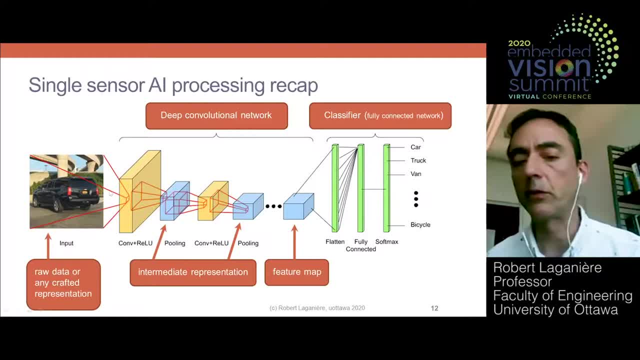 However, this is an expensive sensor and it does not provide any information about the appearance of object, which can make classification and recognition more difficult. However, this is an expensive sensor and it does not provide any information about the appearance of object, which can make classification and recognition more difficult. 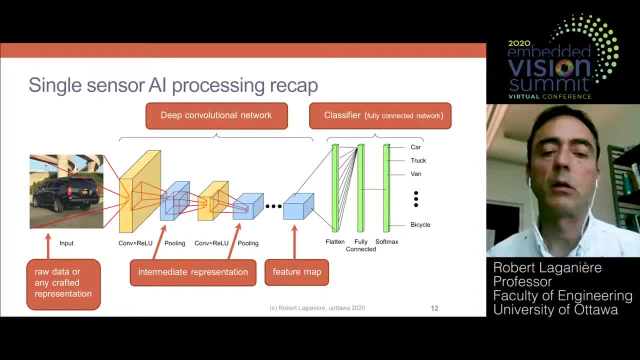 However, this is an expensive sensor and it does not provide any information about the appearance of object, which can make classification and recognition more difficult. However, this is an expensive sensor and it does not provide any information about the appearance of object, which can make classification and recognition more difficult. 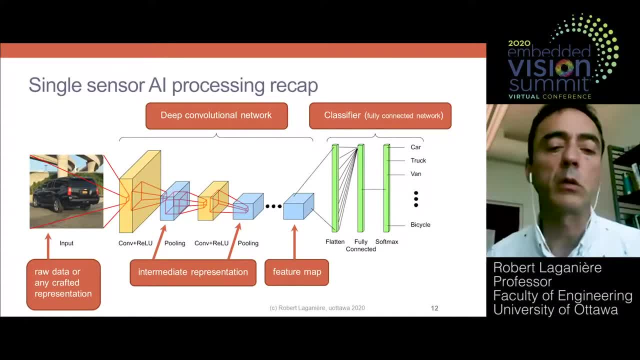 However, this is an expensive sensor and it does not provide any information about the appearance of object, which can make classification and recognition more difficult. However, this is an expensive sensor and it does not provide any information about the appearance of object, which can make classification and recognition more difficult. 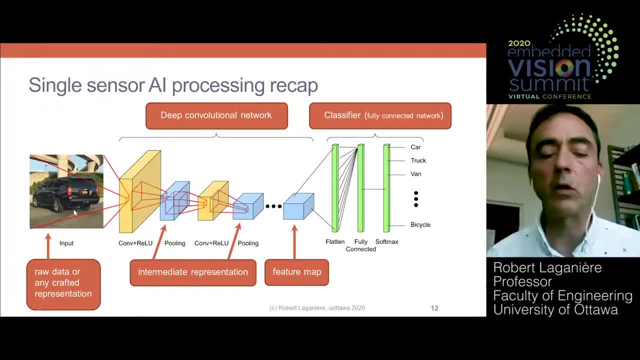 However, this is an expensive sensor and it does not provide any information about the appearance of object, which can make classification and recognition more difficult. However, this is an expensive sensor and it does not provide any information about the appearance of object, which can make classification and recognition more difficult. 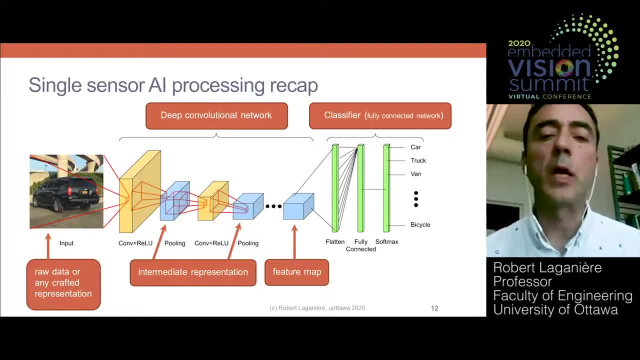 However, this is an expensive sensor and it does not provide any information about the appearance of object, which can make classification and recognition more difficult. However, this is an expensive sensor and it does not provide any information about the appearance of object, which can make classification and recognition more difficult. 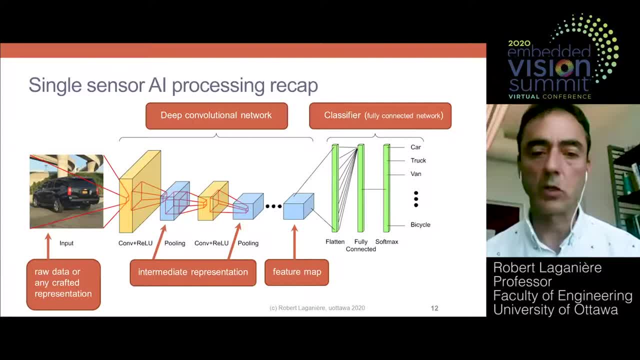 However, this is an expensive sensor and it does not provide any information about the appearance of object, which can make classification and recognition more difficult. However, this is an expensive sensor and it does not provide any information about the appearance of object, which can make classification and recognition more difficult. 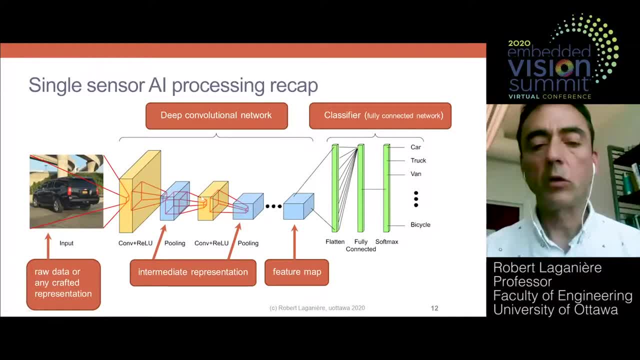 However, this is an expensive sensor and it does not provide any information about the appearance of object, which can make classification and recognition more difficult. However, this is an expensive sensor and it does not provide any information about the appearance of object, which can make classification and recognition more difficult. 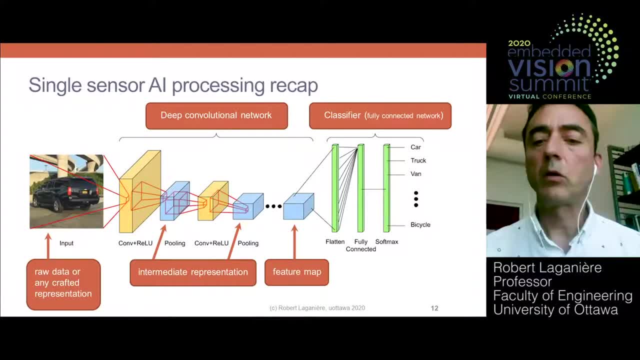 However, this is an expensive sensor and it does not provide any information about the appearance of object, which can make classification and recognition more difficult. However, this is an expensive sensor and it does not provide any information about the appearance of object, which can make classification and recognition more difficult. 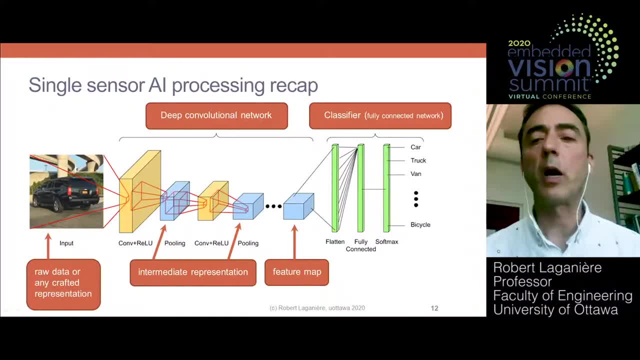 However, this is an expensive sensor and it does not provide any information about the appearance of object, which can make classification and recognition more difficult. However, this is an expensive sensor and it does not provide any information about the appearance of object, which can make classification and recognition more difficult. 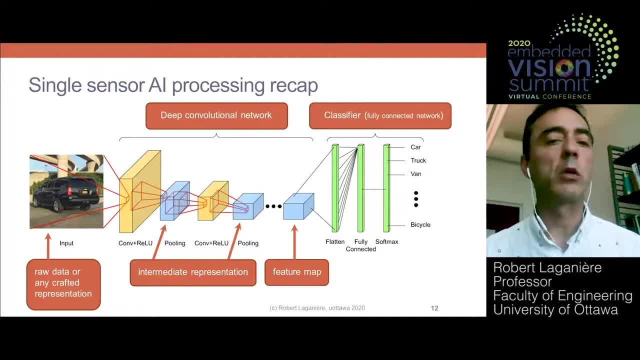 However, this is an expensive sensor and it does not provide any information about the appearance of object, which can make classification and recognition more difficult. However, this is an expensive sensor and it does not provide any information about the appearance of object, which can make classification and recognition more difficult. 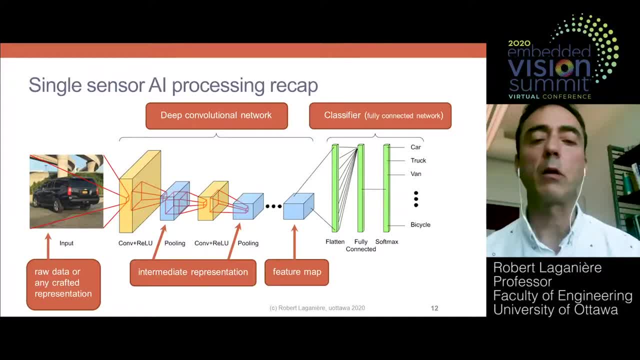 However, this is an expensive sensor and it does not provide any information about the appearance of object, which can make classification and recognition more difficult. However, this is an expensive sensor and it does not provide any information about the appearance of object, which can make classification and recognition more difficult. 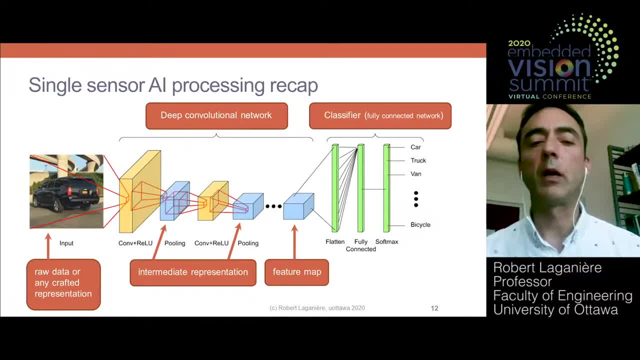 However, this is an expensive sensor and it does not provide any information about the appearance of object, which can make classification and recognition more difficult. However, this is an expensive sensor and it does not provide any information about the appearance of object, which can make classification and recognition more difficult. 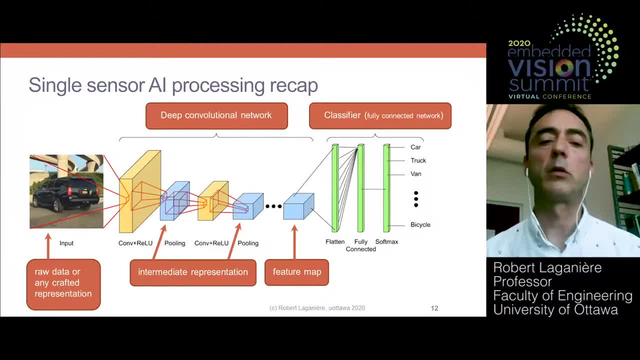 However, this is an expensive sensor and it does not provide any information about the appearance of object, which can make classification and recognition more difficult. However, this is an expensive sensor and it does not provide any information about the appearance of object, which can make classification and recognition more difficult. 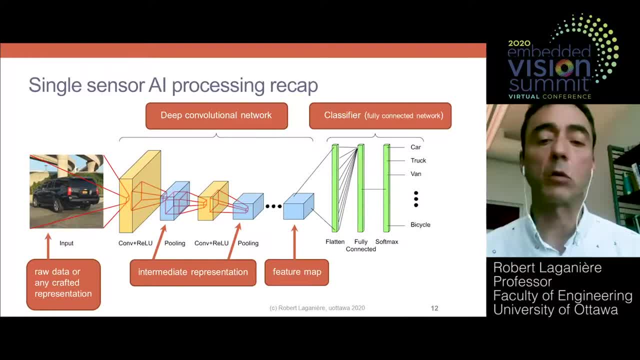 However, this is an expensive sensor and it does not provide any information about the appearance of object, which can make classification and recognition more difficult. However, this is an expensive sensor and it does not provide any information about the appearance of object, which can make classification and recognition more difficult. 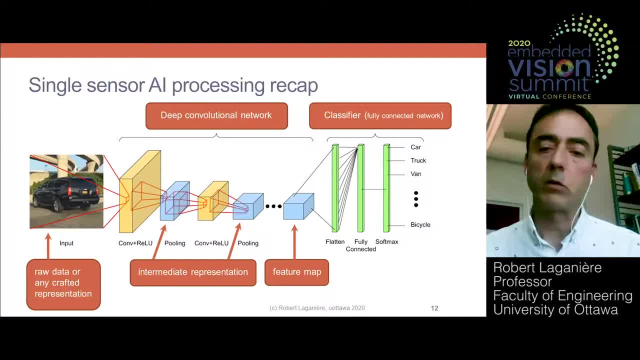 However, this is an expensive sensor and it does not provide any information about the appearance of object, which can make classification and recognition more difficult. However, this is an expensive sensor and it does not provide any information about the appearance of object, which can make classification and recognition more difficult. 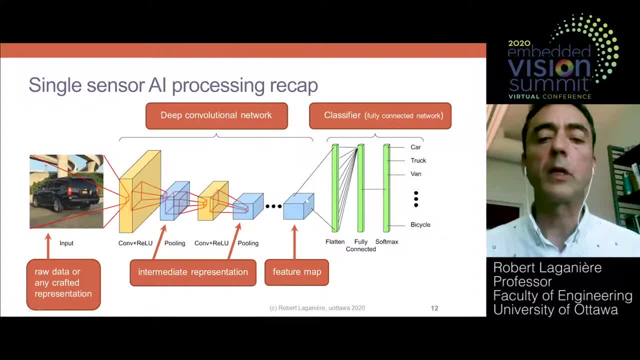 However, this is an expensive sensor and it does not provide any information about the appearance of object, which can make classification and recognition more difficult. However, this is an expensive sensor and it does not provide any information about the appearance of object, which can make classification and recognition more difficult. 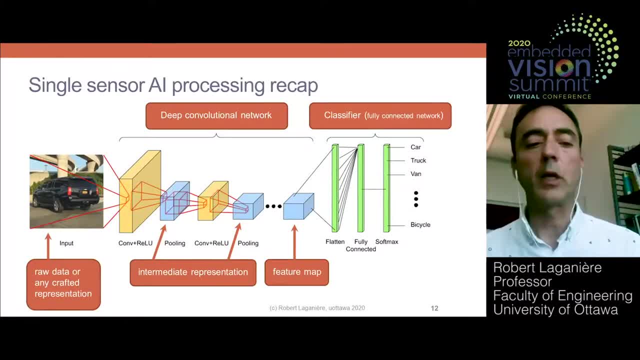 However, this is an expensive sensor and it does not provide any information about the appearance of object, which can make classification and recognition more difficult. However, this is an expensive sensor and it does not provide any information about the appearance of object, which can make classification and recognition more difficult. 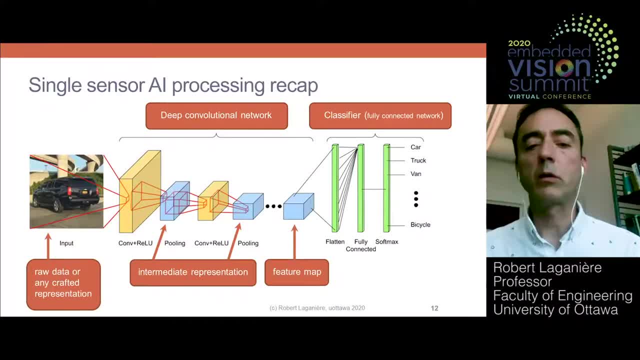 However, this is an expensive sensor and it does not provide any information about the appearance of object, which can make classification and recognition more difficult. However, this is an expensive sensor and it does not provide any information about the appearance of object, which can make classification and recognition more difficult. 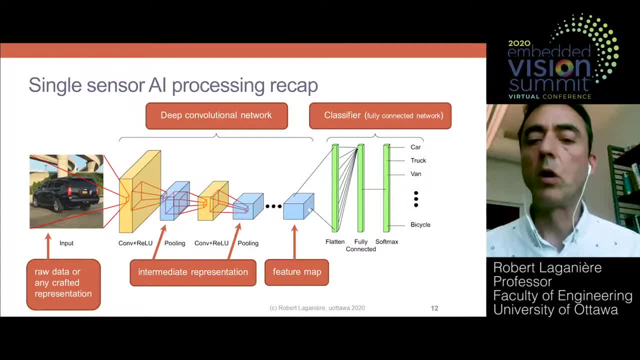 However, this is an expensive sensor and it does not provide any information about the appearance of object, which can make classification and recognition more difficult. However, this is an expensive sensor and it does not provide any information about the appearance of object, which can make classification and recognition more difficult. 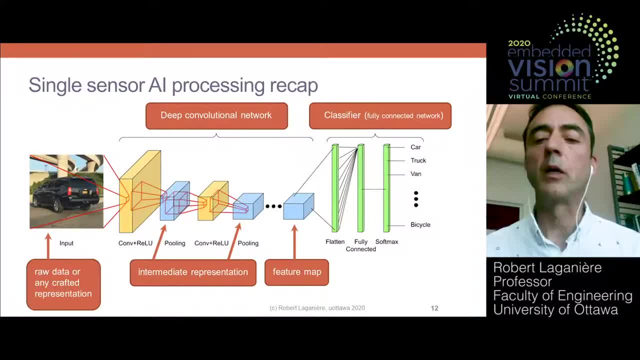 However, this is an expensive sensor and it does not provide any information about the appearance of object, which can make classification and recognition more difficult. However, this is an expensive sensor and it does not provide any information about the appearance of object, which can make classification and recognition more difficult. 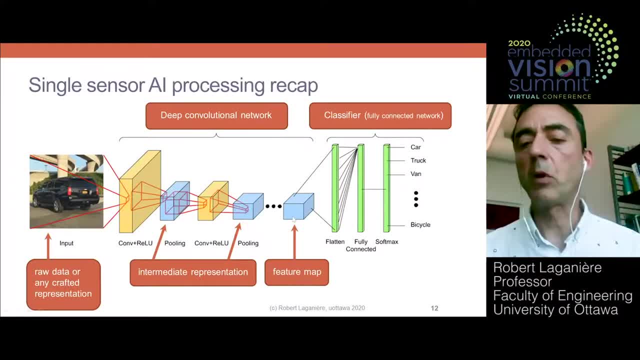 However, this is an expensive sensor and it does not provide any information about the appearance of object, which can make classification and recognition more difficult. However, this is an expensive sensor and it does not provide any information about the appearance of object, which can make classification and recognition more difficult. 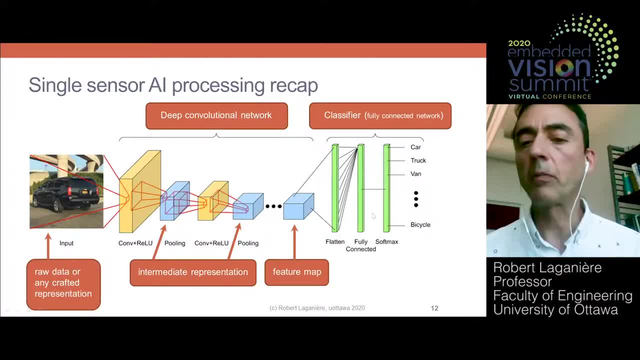 However, this is an expensive sensor and it does not provide any information about the appearance of object, which can make classification and recognition more difficult. However, this is an expensive sensor and it does not provide any information about the appearance of object, which can make classification and recognition more difficult. 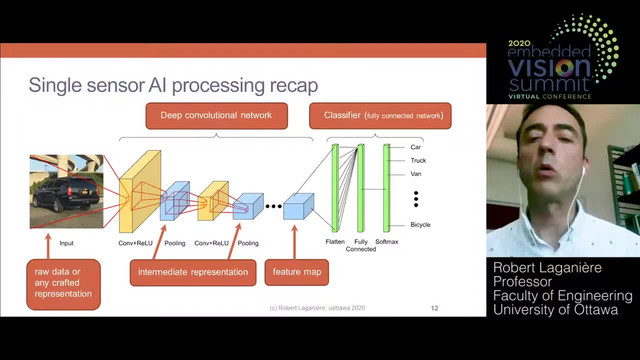 However, this is an expensive sensor and it does not provide any information about the appearance of object, which can make classification and recognition more difficult. However, this is an expensive sensor and it does not provide any information about the appearance of object, which can make classification and recognition more difficult. 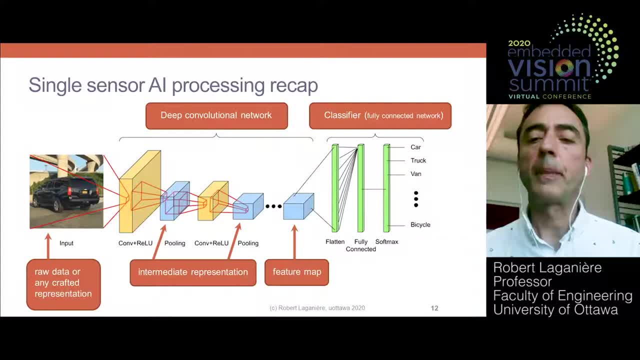 However, this is an expensive sensor and it does not provide any information about the appearance of object, which can make classification and recognition more difficult. However, this is an expensive sensor and it does not provide any information about the appearance of object, which can make classification and recognition more difficult. 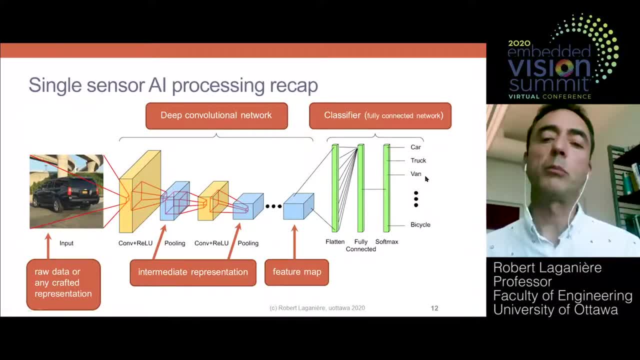 However, this is an expensive sensor and it does not provide any information about the appearance of object, which can make classification and recognition more difficult. However, this is an expensive sensor and it does not provide any information about the appearance of object, which can make classification and recognition more difficult. 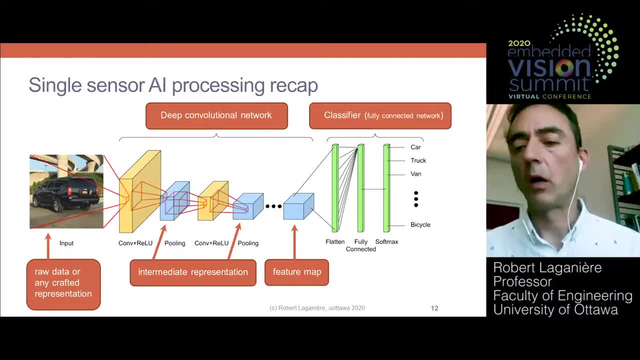 However, this is an expensive sensor and it does not provide any information about the appearance of object, which can make classification and recognition more difficult. However, this is an expensive sensor and it does not provide any information about the appearance of object, which can make classification and recognition more difficult. 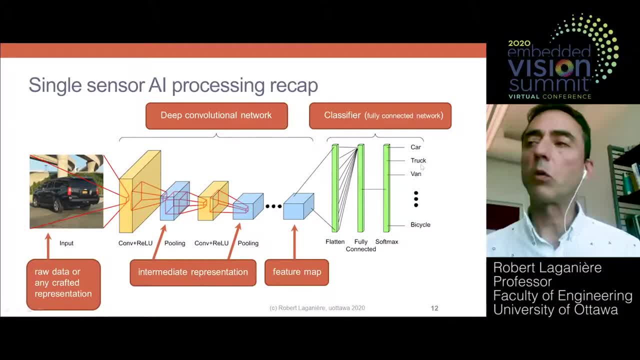 However, this is an expensive sensor and it does not provide any information about the appearance of object, which can make classification and recognition more difficult. However, this is an expensive sensor and it does not provide any information about the appearance of object, which can make classification and recognition more difficult. 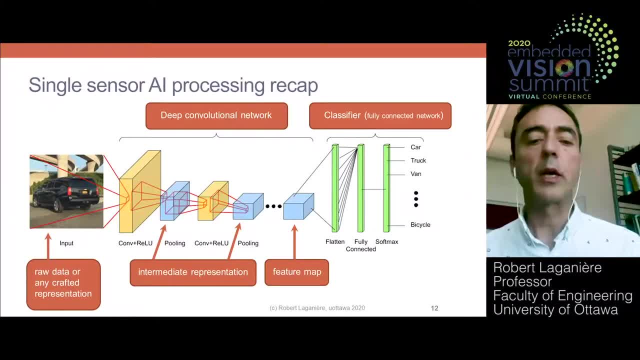 However, this is an expensive sensor and it does not provide any information about the appearance of object, which can make classification and recognition more difficult. However, this is an expensive sensor and it does not provide any information about the appearance of object, which can make classification and recognition more difficult. 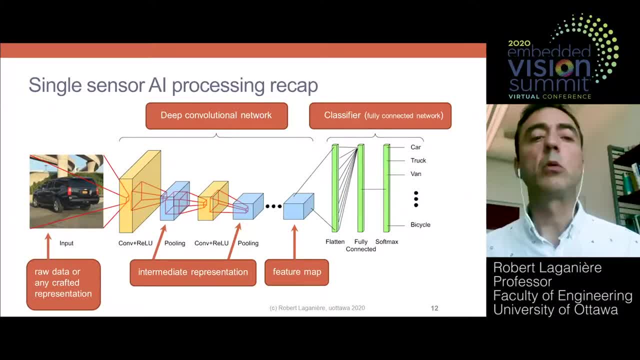 However, this is an expensive sensor and it does not provide any information about the appearance of object, which can make classification and recognition more difficult. However, this is an expensive sensor and it does not provide any information about the appearance of object, which can make classification and recognition more difficult. 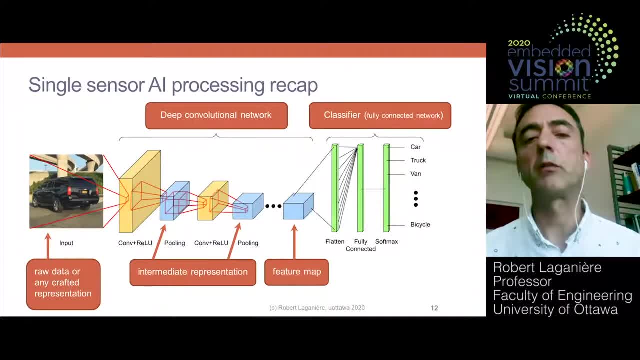 However, this is an expensive sensor and it does not provide any information about the appearance of object, which can make classification and recognition more difficult. However, this is an expensive sensor and it does not provide any information about the appearance of object, which can make classification and recognition more difficult. 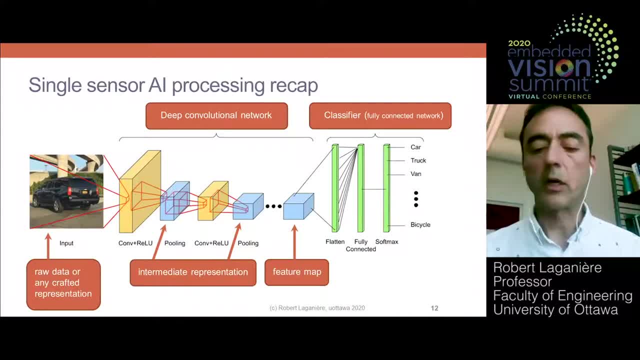 However, this is an expensive sensor and it does not provide any information about the appearance of object, which can make classification and recognition more difficult. However, this is an expensive sensor and it does not provide any information about the appearance of object, which can make classification and recognition more difficult. 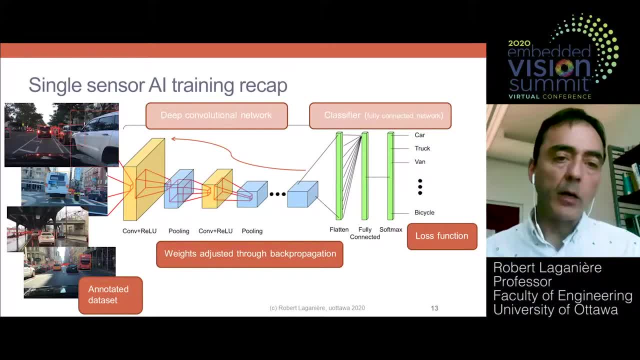 However, this is an expensive sensor and it does not provide any information about the appearance of object, which can make classification and recognition more difficult. However, this is an expensive sensor and it does not provide any information about the appearance of object, which can make classification and recognition more difficult. 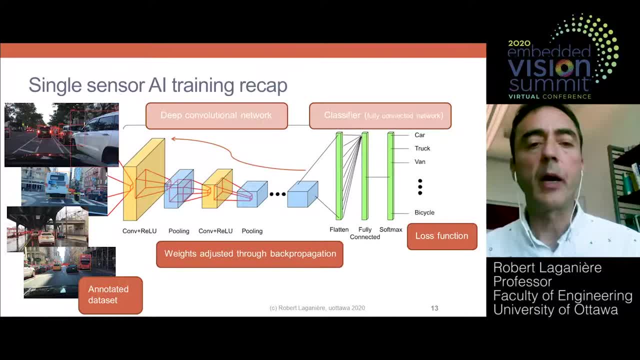 However, this is an expensive sensor and it does not provide any information about the appearance of object, which can make classification and recognition more difficult. However, this is an expensive sensor and it does not provide any information about the appearance of object, which can make classification and recognition more difficult. 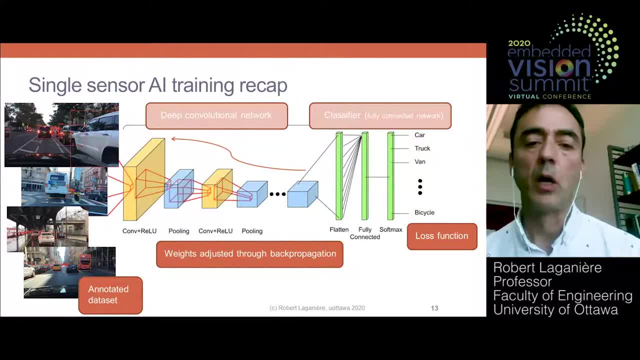 However, this is an expensive sensor and it does not provide any information about the appearance of object, which can make classification and recognition more difficult. However, this is an expensive sensor and it does not provide any information about the appearance of object, which can make classification and recognition more difficult. 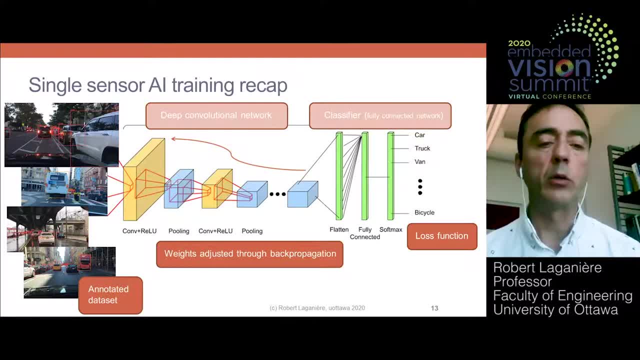 However, this is an expensive sensor and it does not provide any information about the appearance of object, which can make classification and recognition more difficult. However, this is an expensive sensor and it does not provide any information about the appearance of object, which can make classification and recognition more difficult. 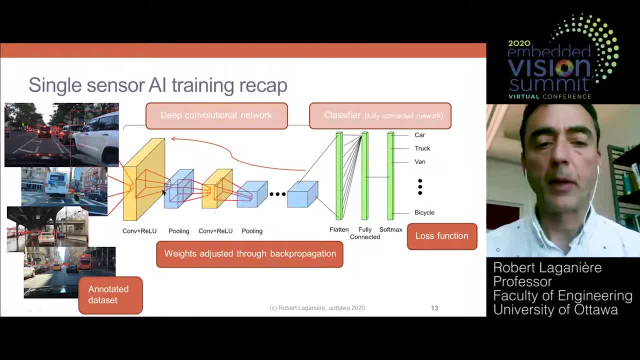 However, this is an expensive sensor and it does not provide any information about the appearance of object, which can make classification and recognition more difficult. However, this is an expensive sensor and it does not provide any information about the appearance of object, which can make classification and recognition more difficult. 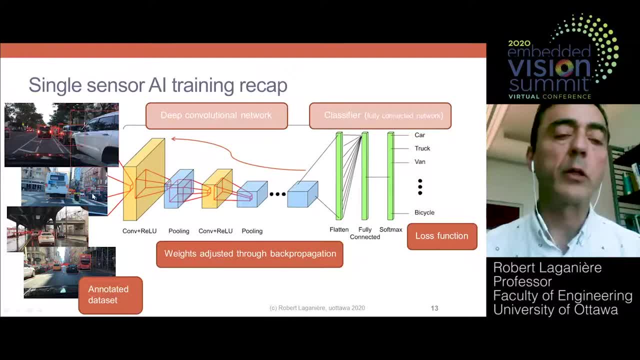 However, this is an expensive sensor and it does not provide any information about the appearance of object, which can make classification and recognition more difficult. However, this is an expensive sensor and it does not provide any information about the appearance of object, which can make classification and recognition more difficult. 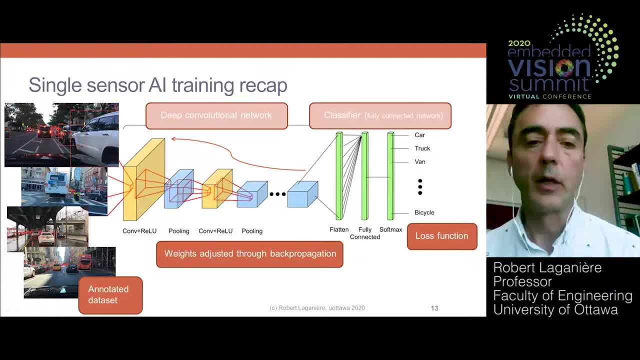 However, this is an expensive sensor and it does not provide any information about the appearance of object, which can make classification and recognition more difficult. However, this is an expensive sensor and it does not provide any information about the appearance of object, which can make classification and recognition more difficult. 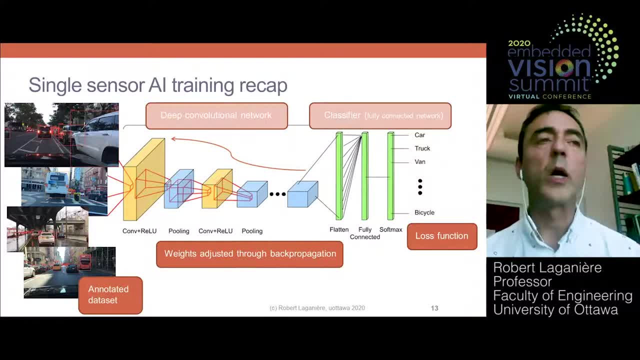 However, this is an expensive sensor and it does not provide any information about the appearance of object, which can make classification and recognition more difficult. However, this is an expensive sensor and it does not provide any information about the appearance of object, which can make classification and recognition more difficult. 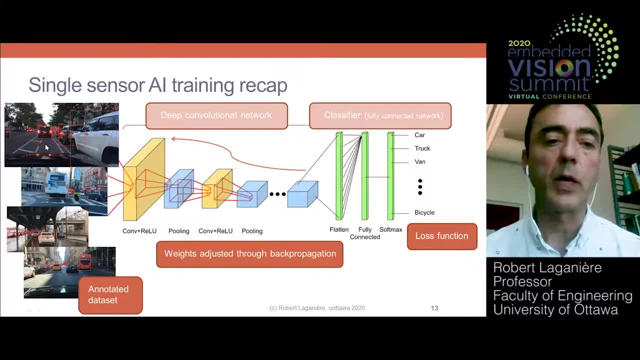 However, this is an expensive sensor and it does not provide any information about the appearance of object, which can make classification and recognition more difficult. However, this is an expensive sensor and it does not provide any information about the appearance of object, which can make classification and recognition more difficult. 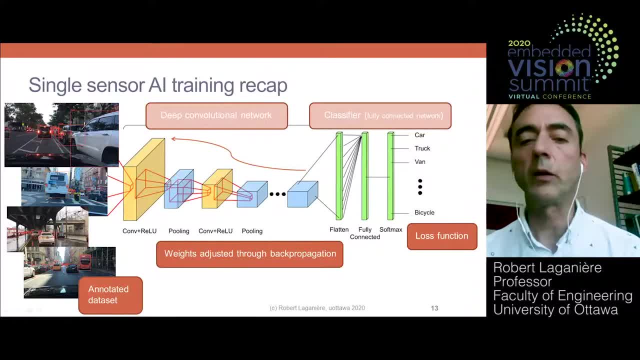 However, this is an expensive sensor and it does not provide any information about the appearance of object, which can make classification and recognition more difficult. However, this is an expensive sensor and it does not provide any information about the appearance of object, which can make classification and recognition more difficult. 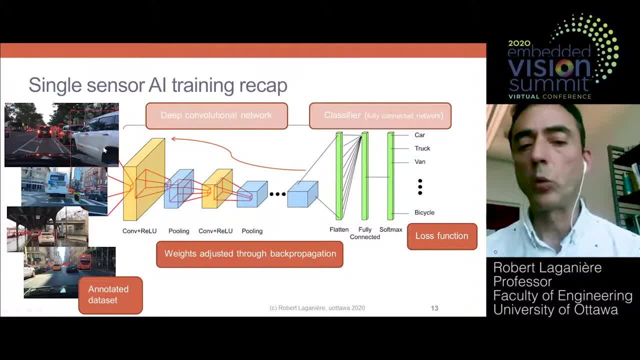 However, this is an expensive sensor and it does not provide any information about the appearance of object, which can make classification and recognition more difficult. However, this is an expensive sensor and it does not provide any information about the appearance of object, which can make classification and recognition more difficult. 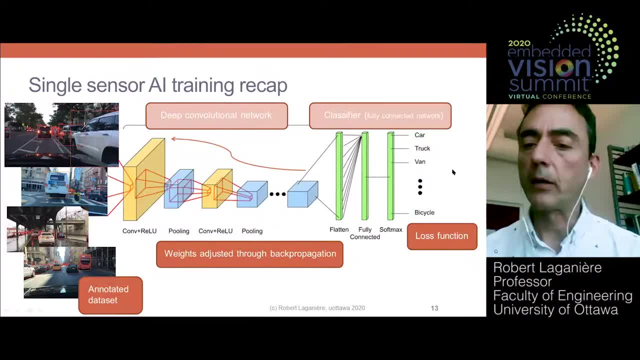 However, this is an expensive sensor and it does not provide any information about the appearance of object, which can make classification and recognition more difficult. However, this is an expensive sensor and it does not provide any information about the appearance of object, which can make classification and recognition more difficult. 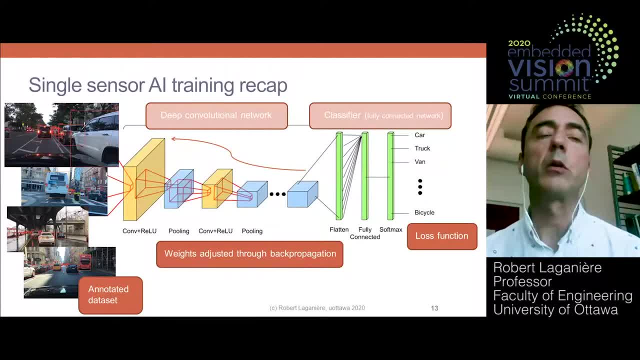 However, this is an expensive sensor and it does not provide any information about the appearance of object, which can make classification and recognition more difficult. However, this is an expensive sensor and it does not provide any information about the appearance of object, which can make classification and recognition more difficult. 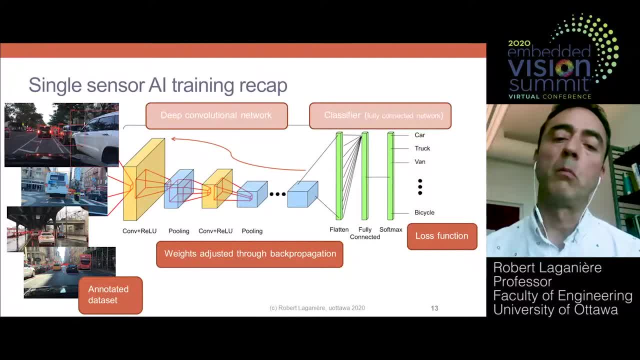 However, this is an expensive sensor and it does not provide any information about the appearance of object, which can make classification and recognition more difficult. However, this is an expensive sensor and it does not provide any information about the appearance of object, which can make classification and recognition more difficult. 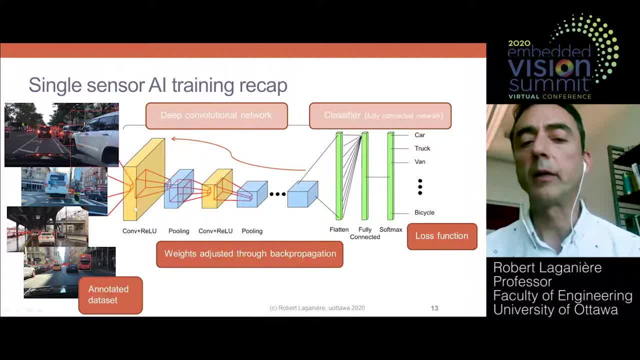 However, this is an expensive sensor and it does not provide any information about the appearance of object, which can make classification and recognition more difficult. However, this is an expensive sensor and it does not provide any information about the appearance of object, which can make classification and recognition more difficult. 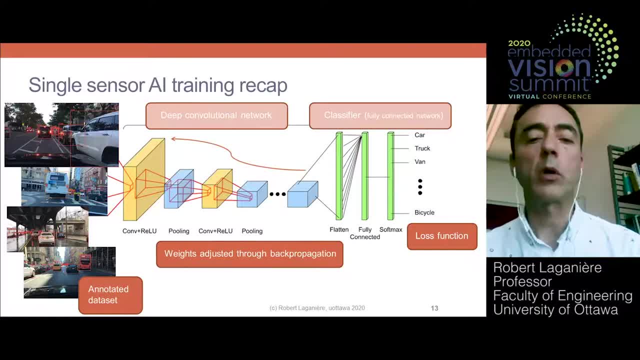 However, this is an expensive sensor and it does not provide any information about the appearance of object, which can make classification and recognition more difficult. However, this is an expensive sensor and it does not provide any information about the appearance of object, which can make classification and recognition more difficult. 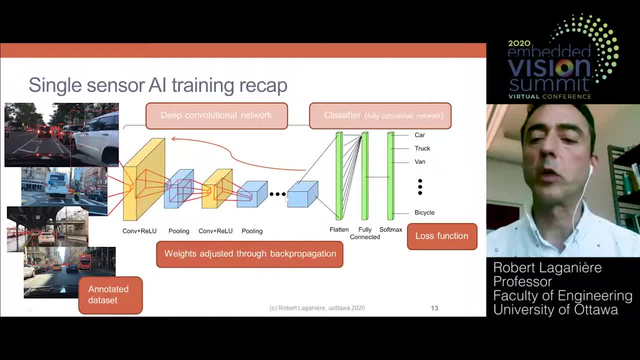 However, this is an expensive sensor and it does not provide any information about the appearance of object, which can make classification and recognition more difficult. However, this is an expensive sensor and it does not provide any information about the appearance of object, which can make classification and recognition more difficult. 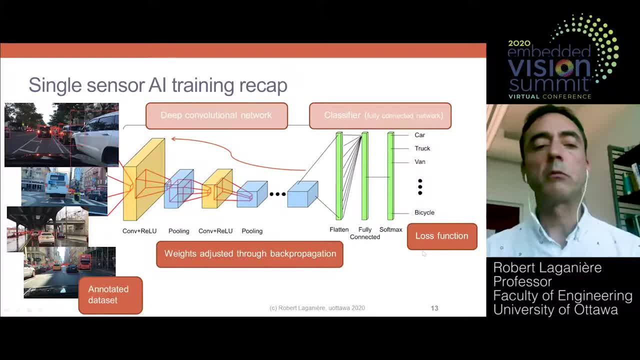 However, this is an expensive sensor and it does not provide any information about the appearance of object, which can make classification and recognition more difficult. However, this is an expensive sensor and it does not provide any information about the appearance of object, which can make classification and recognition more difficult. 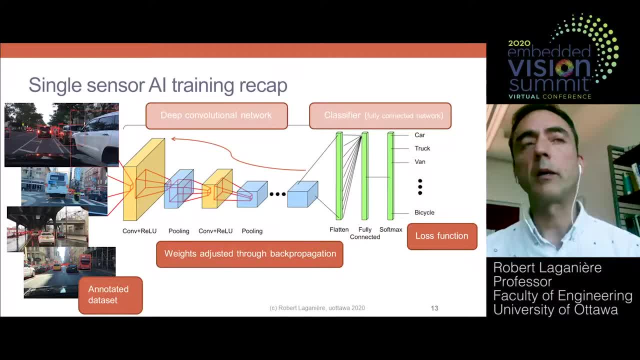 However, this is an expensive sensor and it does not provide any information about the appearance of object, which can make classification and recognition more difficult. However, this is an expensive sensor and it does not provide any information about the appearance of object, which can make classification and recognition more difficult. 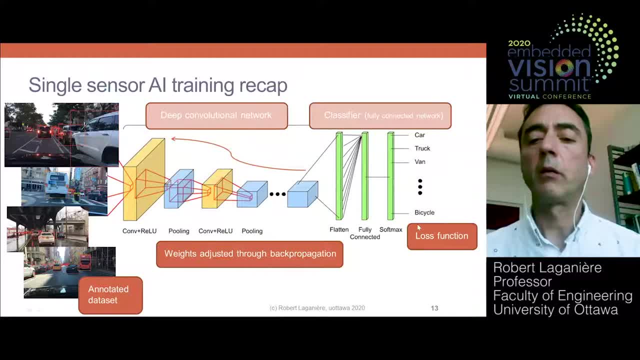 However, this is an expensive sensor and it does not provide any information about the appearance of object, which can make classification and recognition more difficult. However, this is an expensive sensor and it does not provide any information about the appearance of object, which can make classification and recognition more difficult. 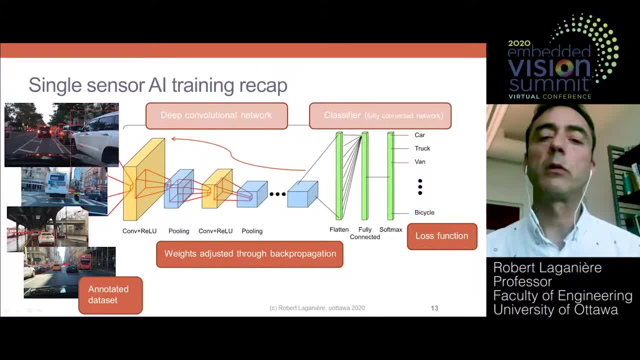 However, this is an expensive sensor and it does not provide any information about the appearance of object, which can make classification and recognition more difficult. However, this is an expensive sensor and it does not provide any information about the appearance of object, which can make classification and recognition more difficult. 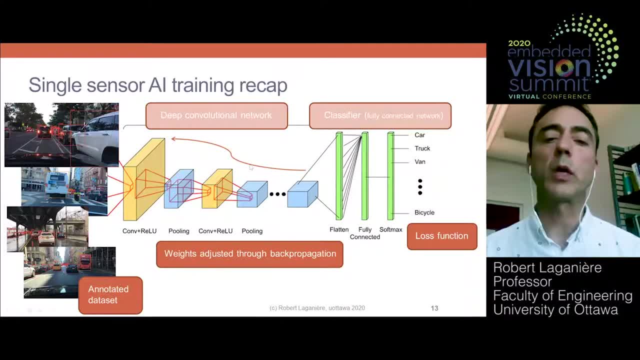 However, this is an expensive sensor and it does not provide any information about the appearance of object, which can make classification and recognition more difficult. However, this is an expensive sensor and it does not provide any information about the appearance of object, which can make classification and recognition more difficult. 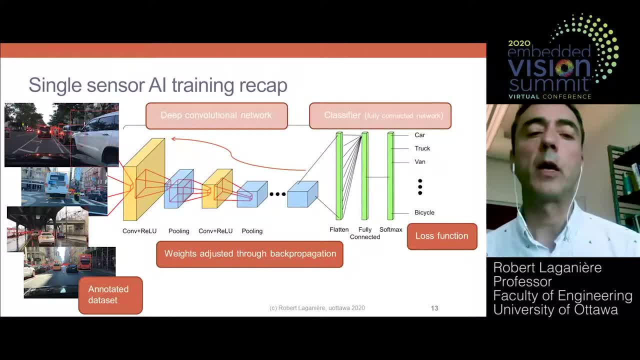 However, this is an expensive sensor and it does not provide any information about the appearance of object, which can make classification and recognition more difficult. However, this is an expensive sensor and it does not provide any information about the appearance of object, which can make classification and recognition more difficult. 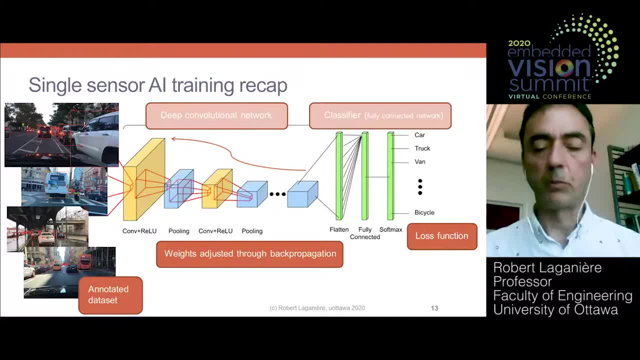 However, this is an expensive sensor and it does not provide any information about the appearance of object, which can make classification and recognition more difficult. However, this is an expensive sensor and it does not provide any information about the appearance of object, which can make classification and recognition more difficult. 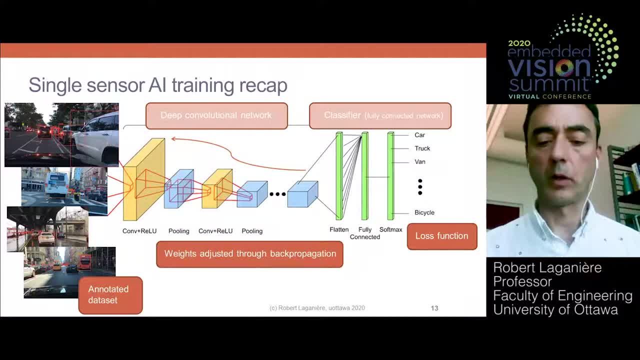 However, this is an expensive sensor and it does not provide any information about the appearance of object, which can make classification and recognition more difficult. However, this is an expensive sensor and it does not provide any information about the appearance of object, which can make classification and recognition more difficult. 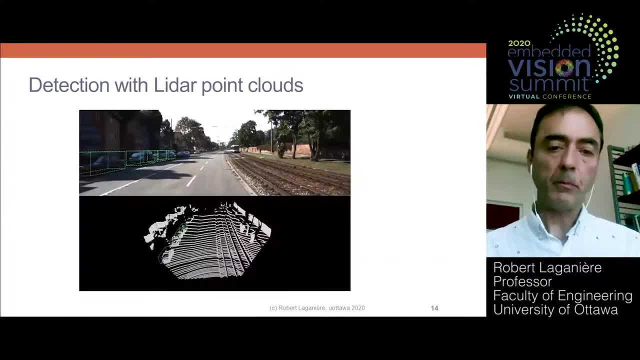 However, this is an expensive sensor and it does not provide any information about the appearance of object, which can make classification and recognition more difficult. However, this is an expensive sensor and it does not provide any information about the appearance of object, which can make classification and recognition more difficult. 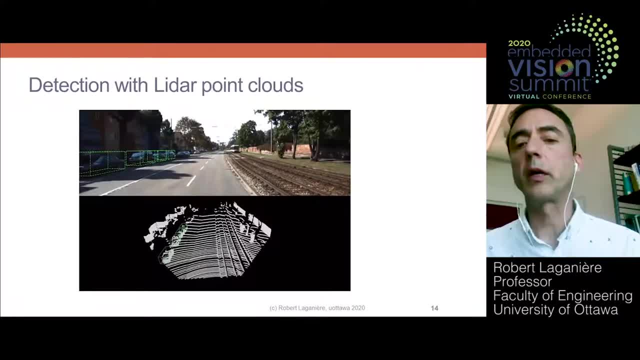 However, this is an expensive sensor and it does not provide any information about the appearance of object, which can make classification and recognition more difficult. However, this is an expensive sensor and it does not provide any information about the appearance of object, which can make classification and recognition more difficult. 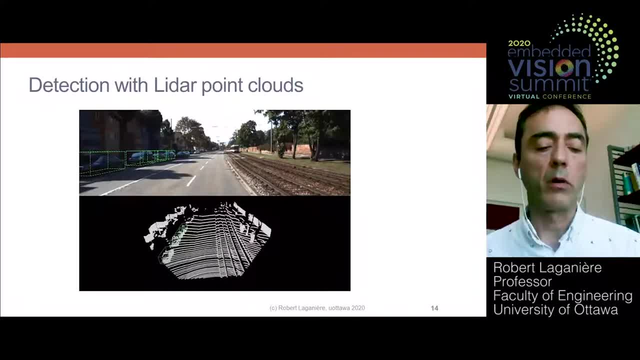 However, this is an expensive sensor and it does not provide any information about the appearance of object, which can make classification and recognition more difficult. However, this is an expensive sensor and it does not provide any information about the appearance of object, which can make classification and recognition more difficult. 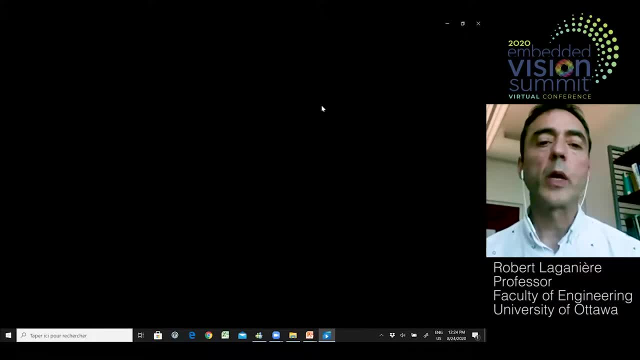 However, this is an expensive sensor and it does not provide any information about the appearance of object, which can make classification and recognition more difficult. However, this is an expensive sensor and it does not provide any information about the appearance of object, which can make classification and recognition more difficult. 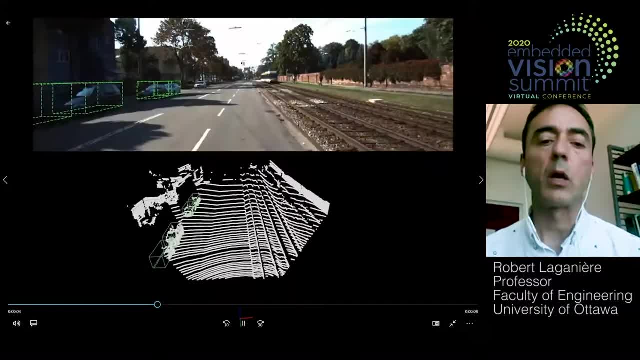 However, this is an expensive sensor and it does not provide any information about the appearance of object, which can make classification and recognition more difficult. However, this is an expensive sensor and it does not provide any information about the appearance of object, which can make classification and recognition more difficult. 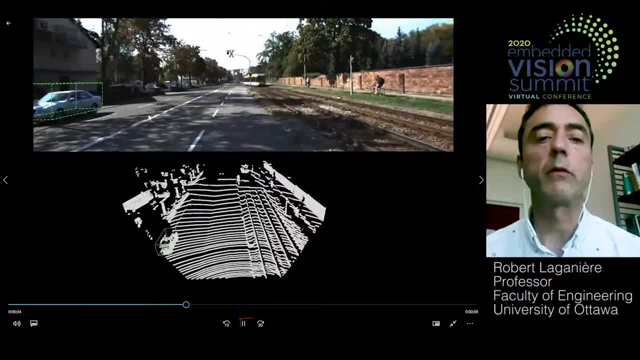 However, this is an expensive sensor and it does not provide any information about the appearance of object, which can make classification and recognition more difficult. However, this is an expensive sensor and it does not provide any information about the appearance of object, which can make classification and recognition more difficult. 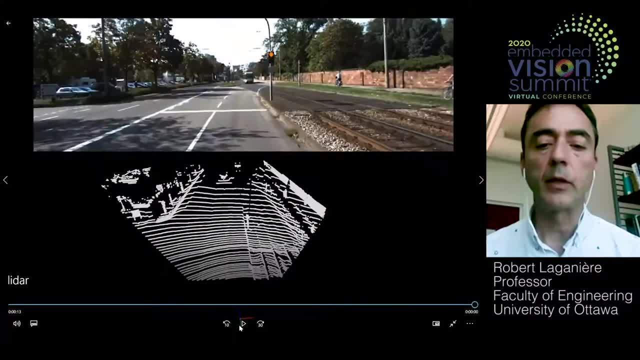 However, this is an expensive sensor and it does not provide any information about the appearance of object, which can make classification and recognition more difficult. However, this is an expensive sensor and it does not provide any information about the appearance of object, which can make classification and recognition more difficult. 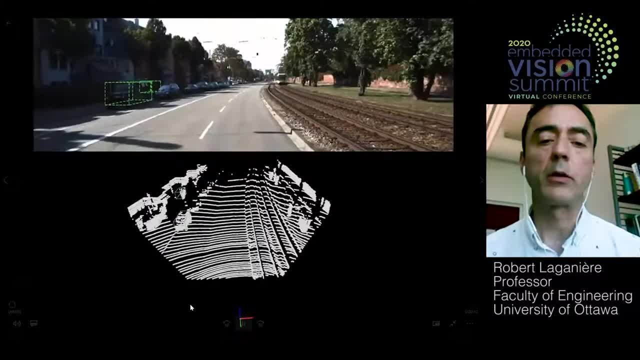 However, this is an expensive sensor and it does not provide any information about the appearance of object, which can make classification and recognition more difficult. However, this is an expensive sensor and it does not provide any information about the appearance of object, which can make classification and recognition more difficult. 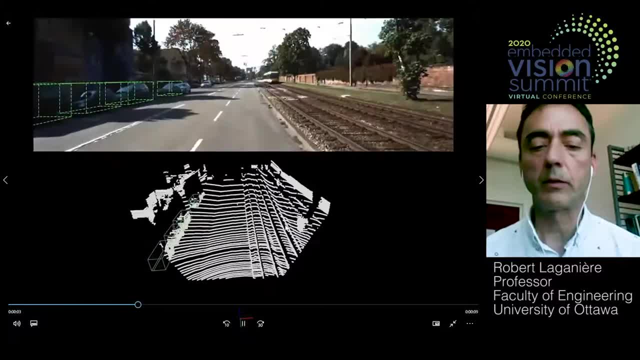 However, this is an expensive sensor and it does not provide any information about the appearance of object, which can make classification and recognition more difficult. However, this is an expensive sensor and it does not provide any information about the appearance of object, which can make classification and recognition more difficult. 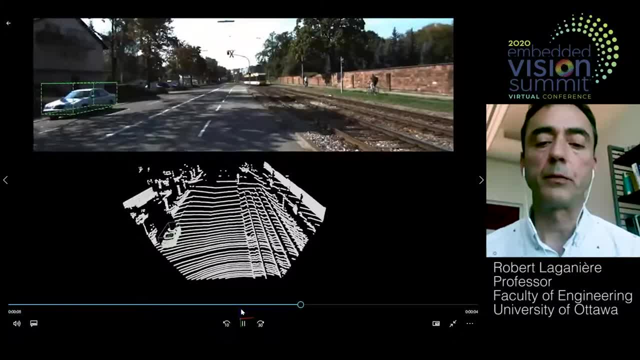 However, this is an expensive sensor and it does not provide any information about the appearance of object, which can make classification and recognition more difficult. However, this is an expensive sensor and it does not provide any information about the appearance of object, which can make classification and recognition more difficult. 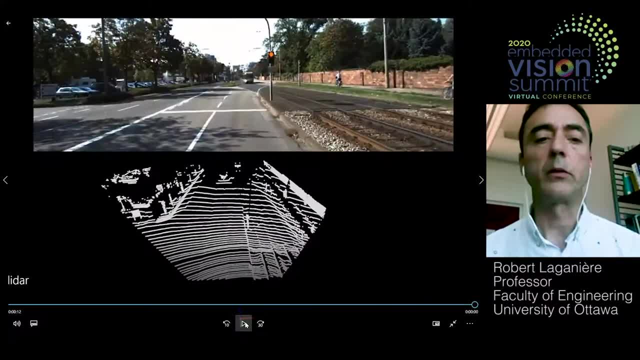 However, this is an expensive sensor and it does not provide any information about the appearance of object, which can make classification and recognition more difficult. However, this is an expensive sensor and it does not provide any information about the appearance of object, which can make classification and recognition more difficult. 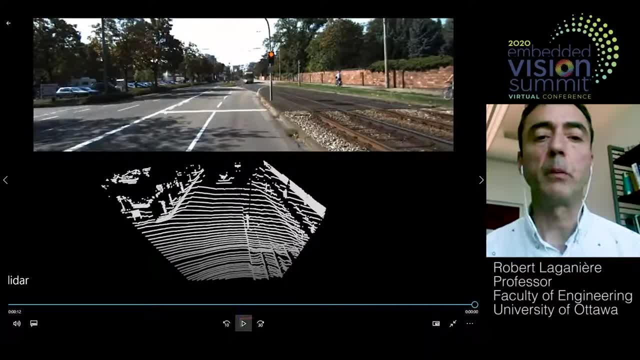 However, this is an expensive sensor and it does not provide any information about the appearance of object, which can make classification and recognition more difficult. However, this is an expensive sensor and it does not provide any information about the appearance of object, which can make classification and recognition more difficult. 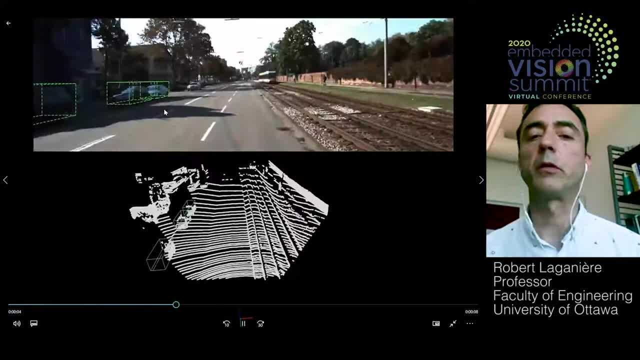 However, this is an expensive sensor and it does not provide any information about the appearance of object, which can make classification and recognition more difficult. However, this is an expensive sensor and it does not provide any information about the appearance of object, which can make classification and recognition more difficult. 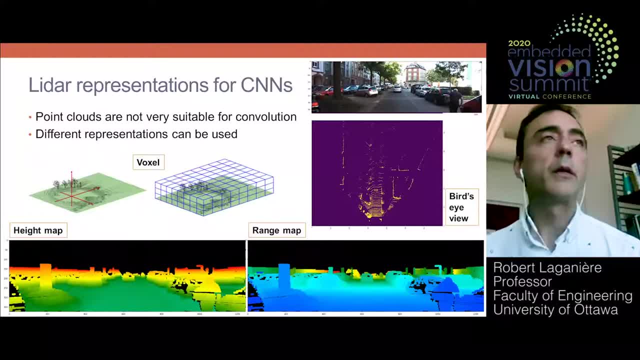 However, this is an expensive sensor and it does not provide any information about the appearance of object, which can make classification and recognition more difficult. However, this is an expensive sensor and it does not provide any information about the appearance of object, which can make classification and recognition more difficult. 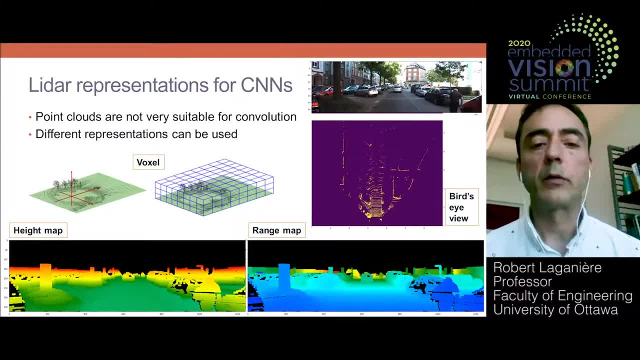 However, this is an expensive sensor and it does not provide any information about the appearance of object, which can make classification and recognition more difficult. However, this is an expensive sensor and it does not provide any information about the appearance of object, which can make classification and recognition more difficult. 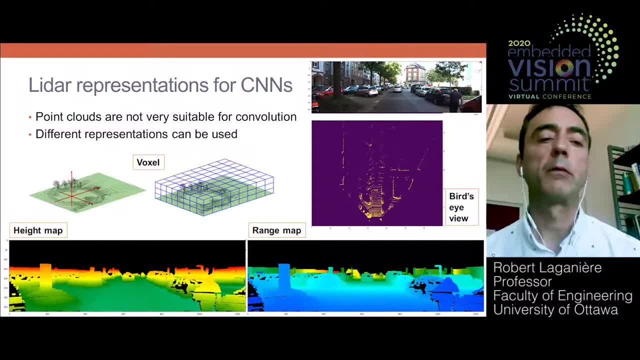 However, this is an expensive sensor and it does not provide any information about the appearance of object, which can make classification and recognition more difficult. However, this is an expensive sensor and it does not provide any information about the appearance of object, which can make classification and recognition more difficult. 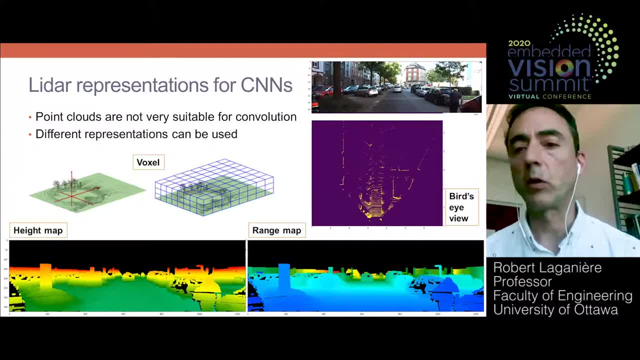 However, this is an expensive sensor and it does not provide any information about the appearance of object, which can make classification and recognition more difficult. However, this is an expensive sensor and it does not provide any information about the appearance of object, which can make classification and recognition more difficult. 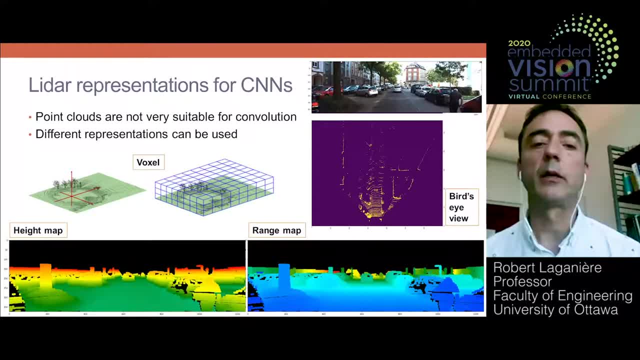 However, this is an expensive sensor and it does not provide any information about the appearance of object, which can make classification and recognition more difficult. However, this is an expensive sensor and it does not provide any information about the appearance of object, which can make classification and recognition more difficult. 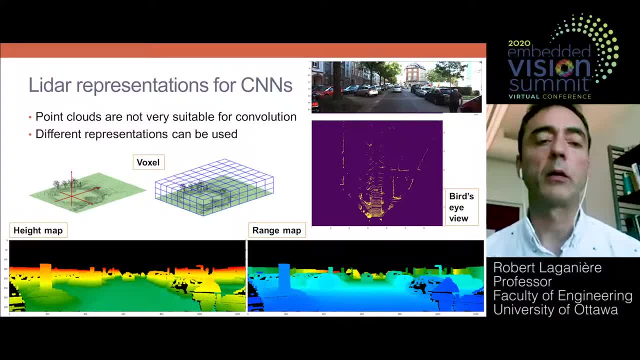 However, this is an expensive sensor and it does not provide any information about the appearance of object, which can make classification and recognition more difficult. However, this is an expensive sensor and it does not provide any information about the appearance of object, which can make classification and recognition more difficult. 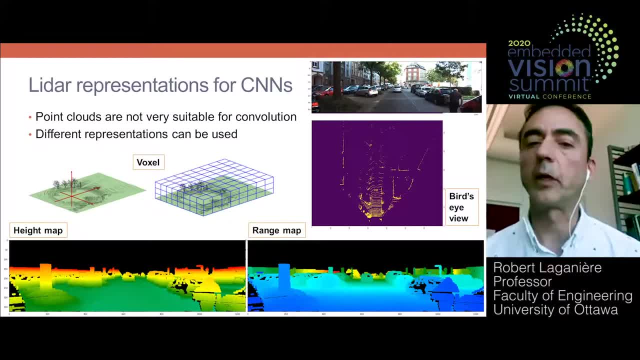 However, this is an expensive sensor and it does not provide any information about the appearance of object, which can make classification and recognition more difficult. However, this is an expensive sensor and it does not provide any information about the appearance of object, which can make classification and recognition more difficult. 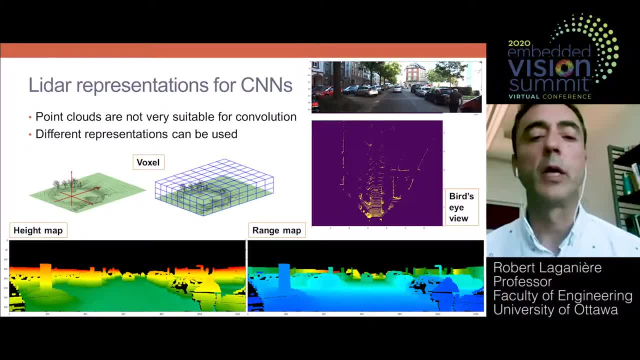 However, this is an expensive sensor and it does not provide any information about the appearance of object, which can make classification and recognition more difficult. However, this is an expensive sensor and it does not provide any information about the appearance of object, which can make classification and recognition more difficult. 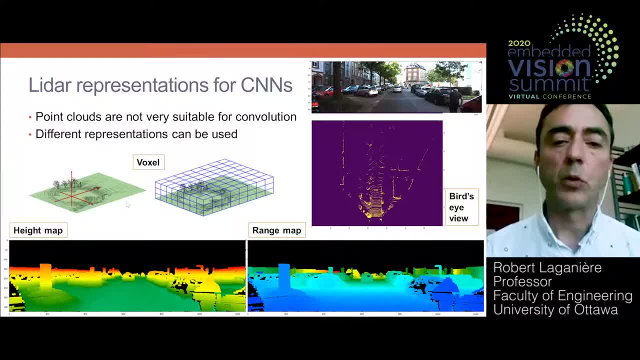 However, this is an expensive sensor and it does not provide any information about the appearance of object, which can make classification and recognition more difficult. However, this is an expensive sensor and it does not provide any information about the appearance of object, which can make classification and recognition more difficult. 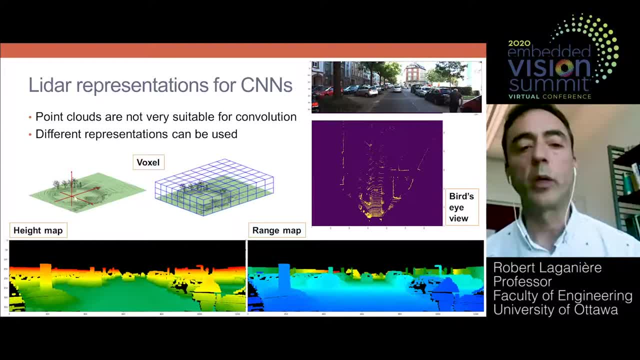 However, this is an expensive sensor and it does not provide any information about the appearance of object, which can make classification and recognition more difficult. However, this is an expensive sensor and it does not provide any information about the appearance of object, which can make classification and recognition more difficult. 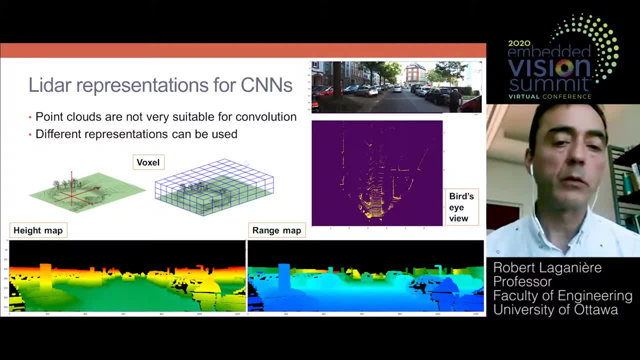 However, this is an expensive sensor and it does not provide any information about the appearance of object, which can make classification and recognition more difficult. However, this is an expensive sensor and it does not provide any information about the appearance of object, which can make classification and recognition more difficult. 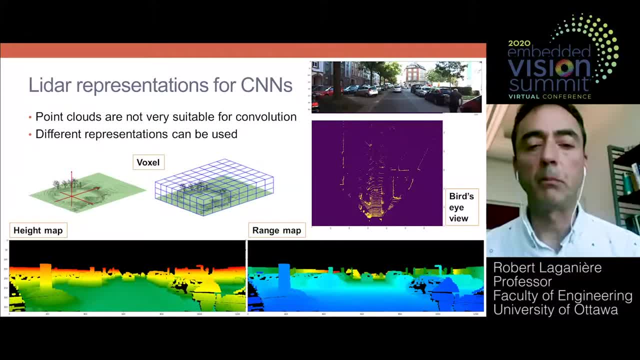 However, this is an expensive sensor and it does not provide any information about the appearance of object, which can make classification and recognition more difficult. However, this is an expensive sensor and it does not provide any information about the appearance of object, which can make classification and recognition more difficult. 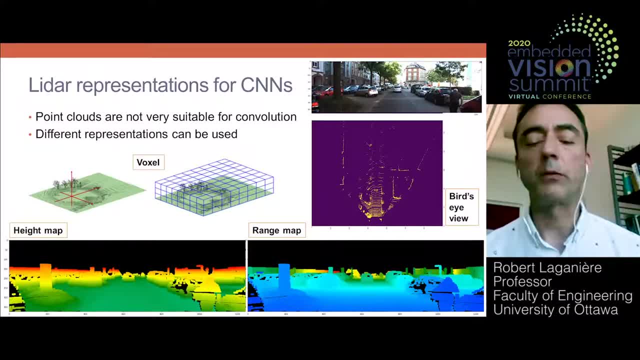 However, this is an expensive sensor and it does not provide any information about the appearance of object, which can make classification and recognition more difficult. However, this is an expensive sensor and it does not provide any information about the appearance of object, which can make classification and recognition more difficult. 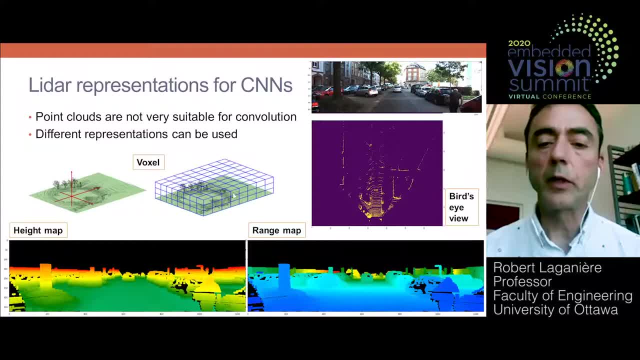 However, this is an expensive sensor and it does not provide any information about the appearance of object, which can make classification and recognition more difficult. However, this is an expensive sensor and it does not provide any information about the appearance of object, which can make classification and recognition more difficult. 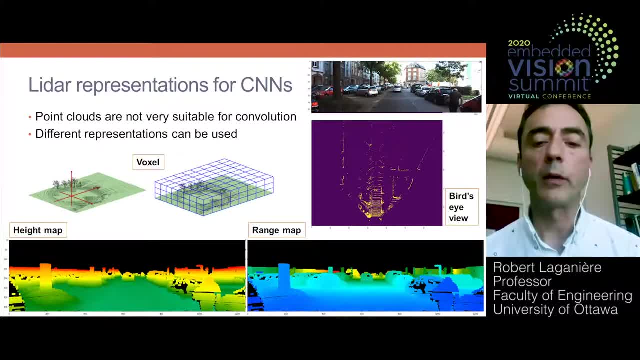 However, this is an expensive sensor and it does not provide any information about the appearance of object, which can make classification and recognition more difficult. However, this is an expensive sensor and it does not provide any information about the appearance of object, which can make classification and recognition more difficult. 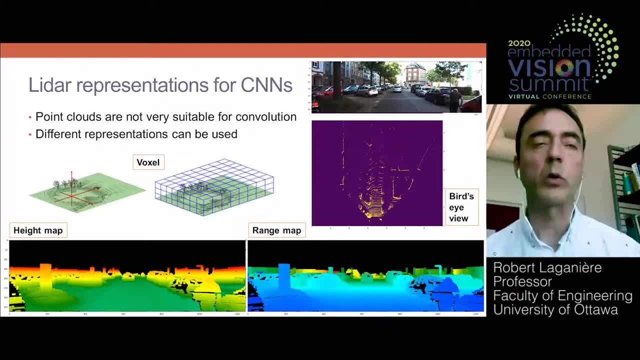 However, this is an expensive sensor and it does not provide any information about the appearance of object, which can make classification and recognition more difficult. However, this is an expensive sensor and it does not provide any information about the appearance of object, which can make classification and recognition more difficult. 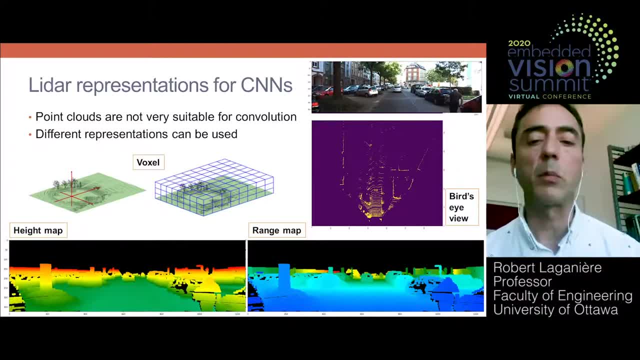 However, this is an expensive sensor and it does not provide any information about the appearance of object, which can make classification and recognition more difficult. However, this is an expensive sensor and it does not provide any information about the appearance of object, which can make classification and recognition more difficult. 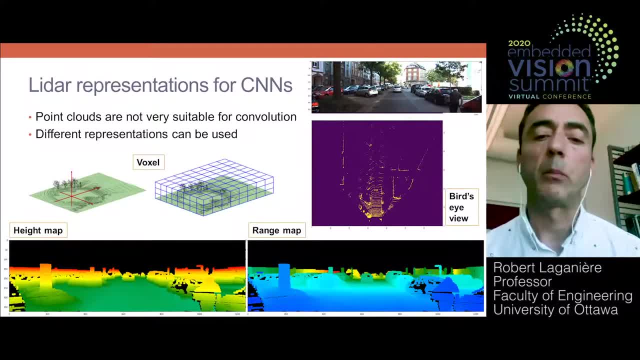 However, this is an expensive sensor and it does not provide any information about the appearance of object, which can make classification and recognition more difficult. However, this is an expensive sensor and it does not provide any information about the appearance of object, which can make classification and recognition more difficult. 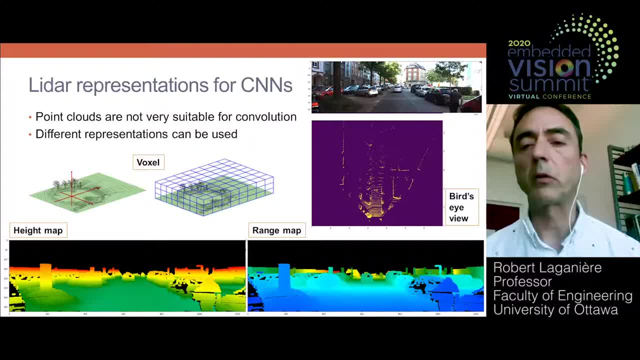 However, this is an expensive sensor and it does not provide any information about the appearance of object, which can make classification and recognition more difficult. However, this is an expensive sensor and it does not provide any information about the appearance of object, which can make classification and recognition more difficult. 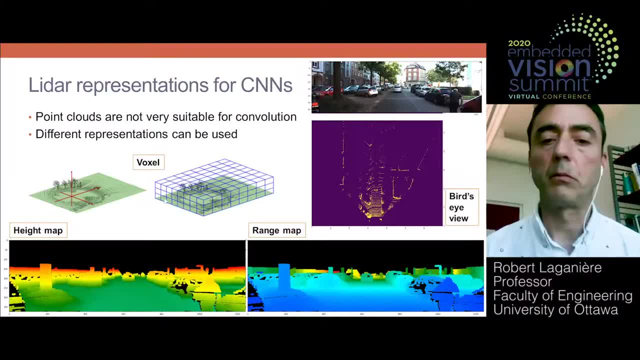 However, this is an expensive sensor and it does not provide any information about the appearance of object, which can make classification and recognition more difficult. However, this is an expensive sensor and it does not provide any information about the appearance of object, which can make classification and recognition more difficult. 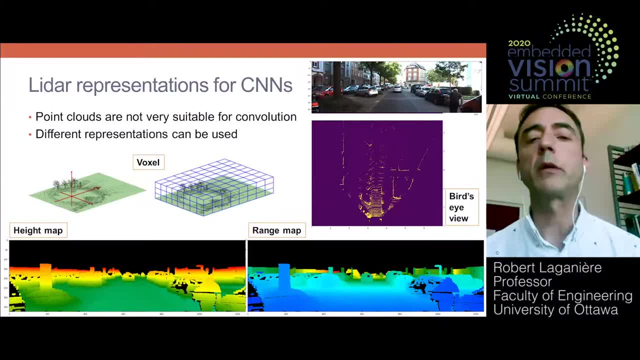 However, this is an expensive sensor and it does not provide any information about the appearance of object, which can make classification and recognition more difficult. However, this is an expensive sensor and it does not provide any information about the appearance of object, which can make classification and recognition more difficult. 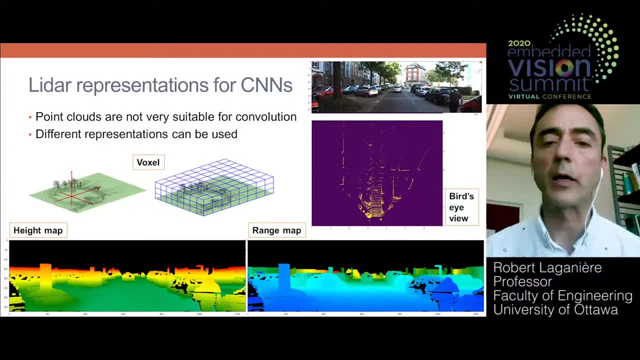 However, this is an expensive sensor and it does not provide any information about the appearance of object, which can make classification and recognition more difficult. However, this is an expensive sensor and it does not provide any information about the appearance of object, which can make classification and recognition more difficult. 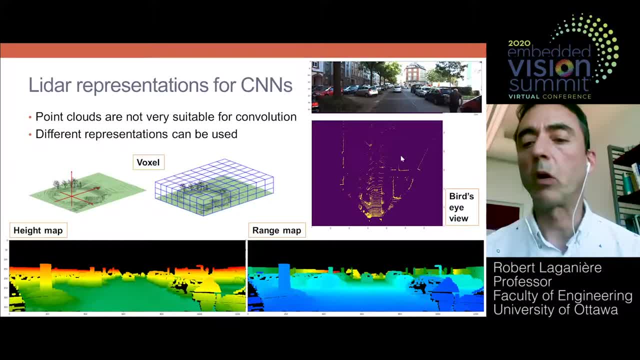 However, this is an expensive sensor and it does not provide any information about the appearance of object, which can make classification and recognition more difficult. However, this is an expensive sensor and it does not provide any information about the appearance of object, which can make classification and recognition more difficult. 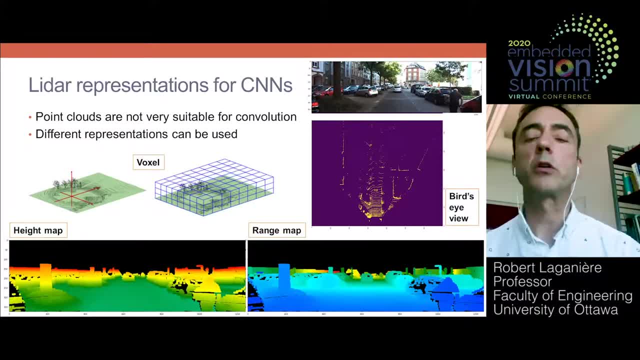 However, this is an expensive sensor and it does not provide any information about the appearance of object, which can make classification and recognition more difficult. However, this is an expensive sensor and it does not provide any information about the appearance of object, which can make classification and recognition more difficult. 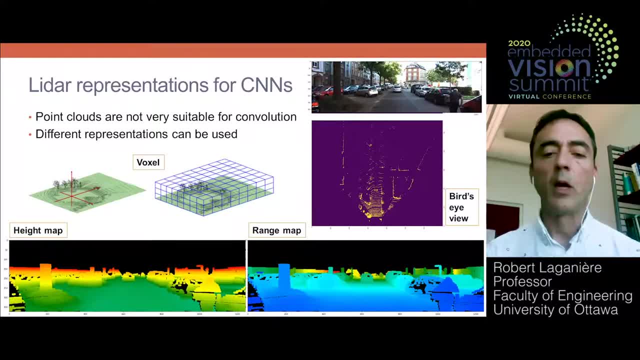 However, this is an expensive sensor and it does not provide any information about the appearance of object, which can make classification and recognition more difficult. However, this is an expensive sensor and it does not provide any information about the appearance of object, which can make classification and recognition more difficult. 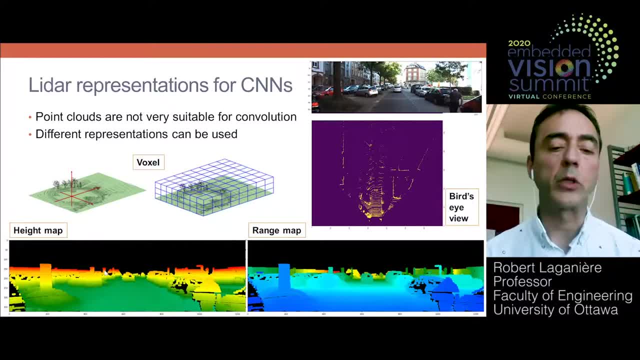 However, this is an expensive sensor and it does not provide any information about the appearance of object, which can make classification and recognition more difficult. However, this is an expensive sensor and it does not provide any information about the appearance of object, which can make classification and recognition more difficult. 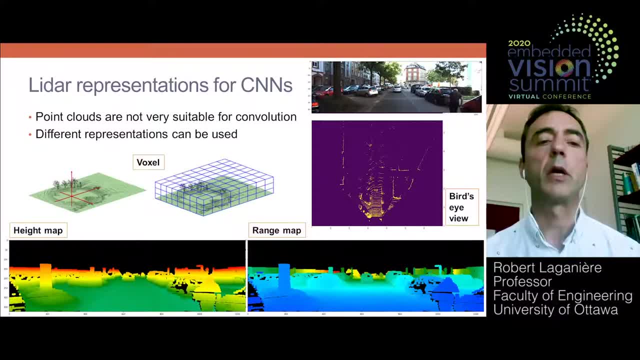 However, this is an expensive sensor and it does not provide any information about the appearance of object, which can make classification and recognition more difficult. However, this is an expensive sensor and it does not provide any information about the appearance of object, which can make classification and recognition more difficult. 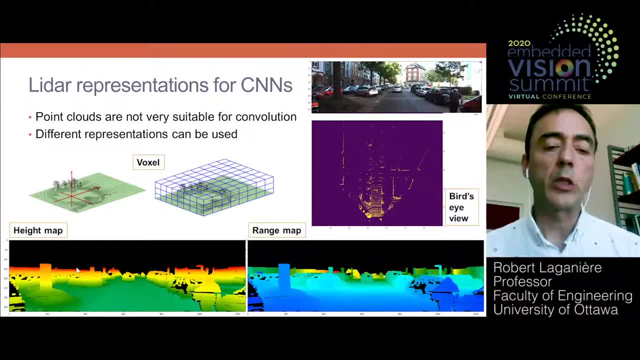 However, this is an expensive sensor and it does not provide any information about the appearance of object, which can make classification and recognition more difficult. However, this is an expensive sensor and it does not provide any information about the appearance of object, which can make classification and recognition more difficult. 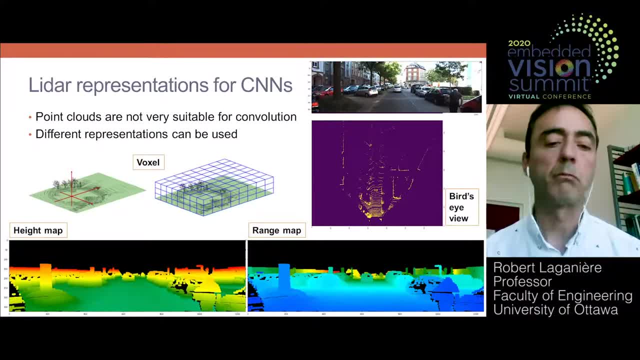 However, this is an expensive sensor and it does not provide any information about the appearance of object, which can make classification and recognition more difficult. However, this is an expensive sensor and it does not provide any information about the appearance of object, which can make classification and recognition more difficult. 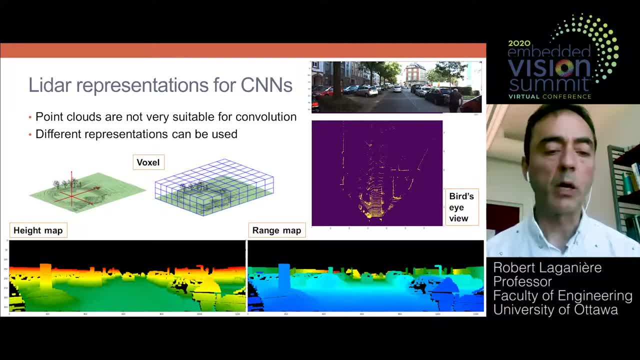 However, this is an expensive sensor and it does not provide any information about the appearance of object, which can make classification and recognition more difficult. However, this is an expensive sensor and it does not provide any information about the appearance of object, which can make classification and recognition more difficult. 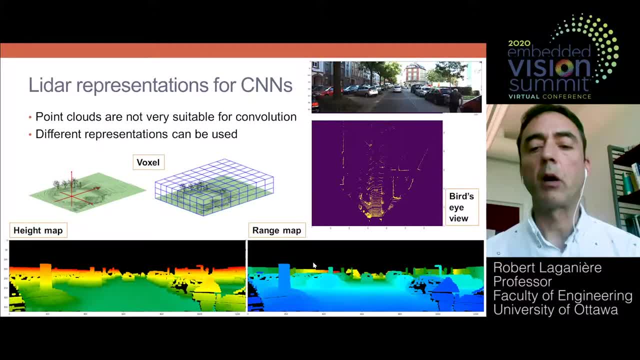 However, this is an expensive sensor and it does not provide any information about the appearance of object, which can make classification and recognition more difficult. However, this is an expensive sensor and it does not provide any information about the appearance of object, which can make classification and recognition more difficult. 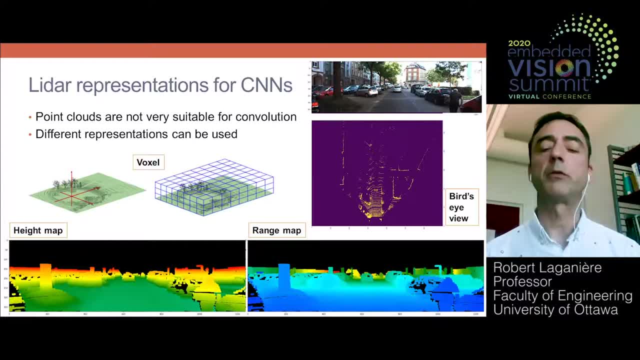 However, this is an expensive sensor and it does not provide any information about the appearance of object, which can make classification and recognition more difficult. However, this is an expensive sensor and it does not provide any information about the appearance of object, which can make classification and recognition more difficult. 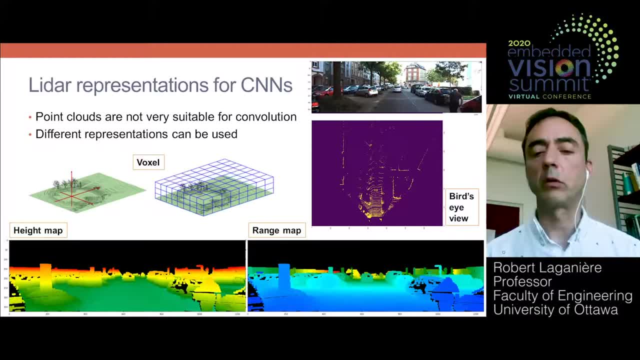 However, this is an expensive sensor and it does not provide any information about the appearance of object, which can make classification and recognition more difficult. However, this is an expensive sensor and it does not provide any information about the appearance of object, which can make classification and recognition more difficult. 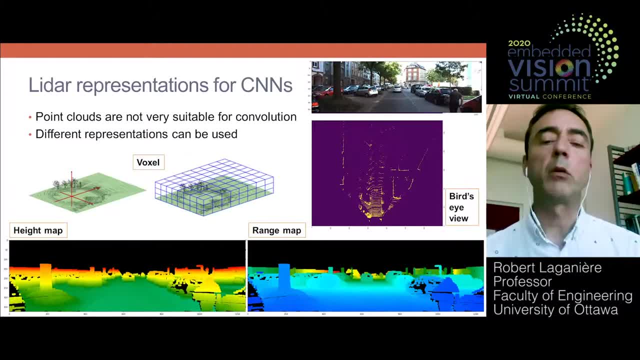 However, this is an expensive sensor and it does not provide any information about the appearance of object, which can make classification and recognition more difficult. However, this is an expensive sensor and it does not provide any information about the appearance of object, which can make classification and recognition more difficult. 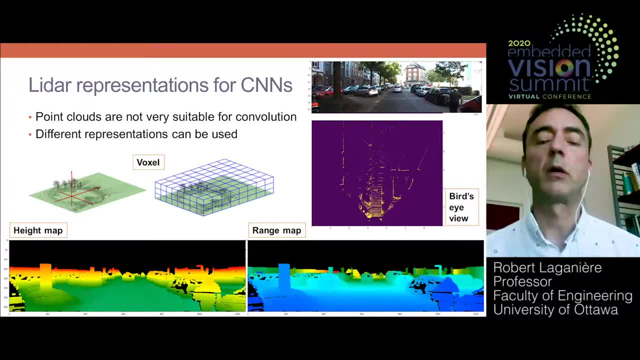 However, this is an expensive sensor and it does not provide any information about the appearance of object, which can make classification and recognition more difficult. However, this is an expensive sensor and it does not provide any information about the appearance of object, which can make classification and recognition more difficult. 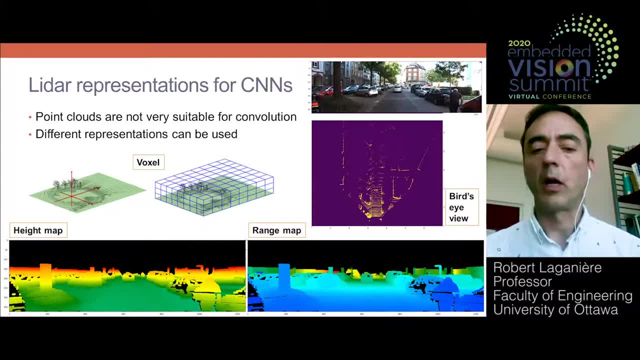 However, this is an expensive sensor and it does not provide any information about the appearance of object, which can make classification and recognition more difficult. However, this is an expensive sensor and it does not provide any information about the appearance of object, which can make classification and recognition more difficult. 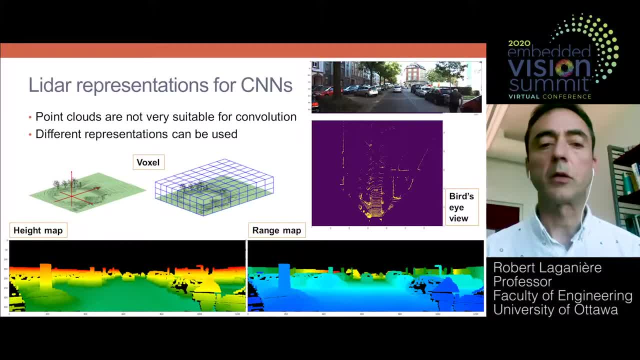 However, this is an expensive sensor and it does not provide any information about the appearance of object, which can make classification and recognition more difficult. However, this is an expensive sensor and it does not provide any information about the appearance of object, which can make classification and recognition more difficult. 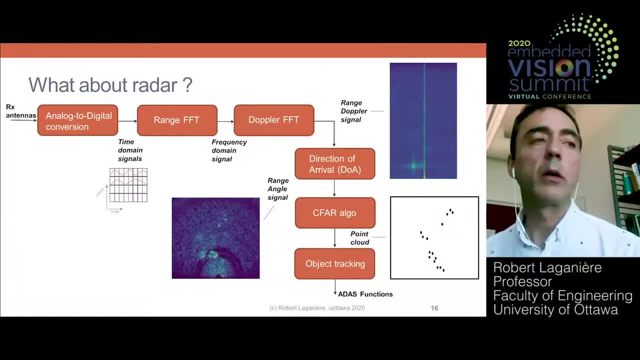 However, this is an expensive sensor and it does not provide any information about the appearance of object, which can make classification and recognition more difficult. However, this is an expensive sensor and it does not provide any information about the appearance of object, which can make classification and recognition more difficult. 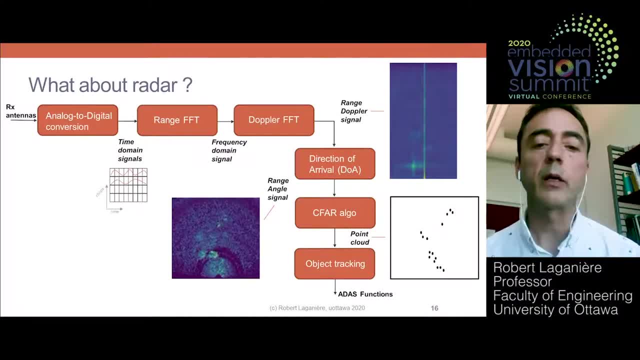 However, this is an expensive sensor and it does not provide any information about the appearance of object, which can make classification and recognition more difficult. However, this is an expensive sensor and it does not provide any information about the appearance of object, which can make classification and recognition more difficult. 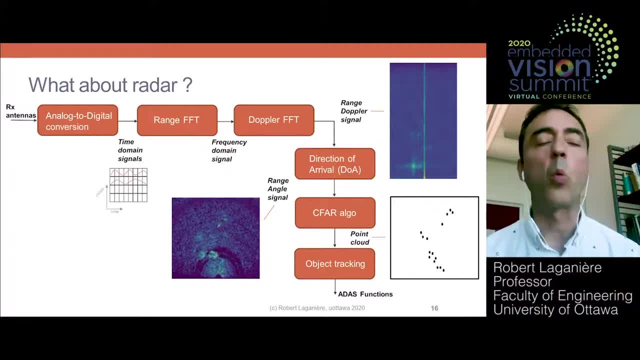 However, this is an expensive sensor and it does not provide any information about the appearance of object, which can make classification and recognition more difficult. However, this is an expensive sensor and it does not provide any information about the appearance of object, which can make classification and recognition more difficult. 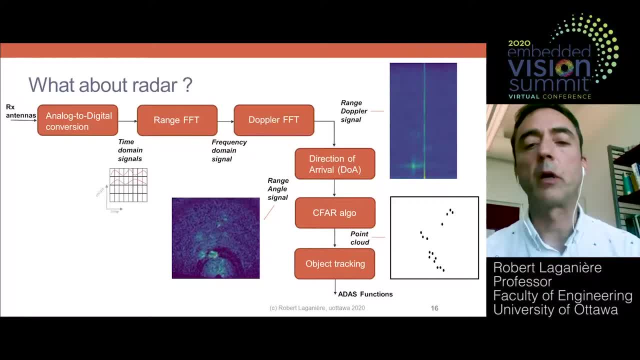 However, this is an expensive sensor and it does not provide any information about the appearance of object, which can make classification and recognition more difficult. However, this is an expensive sensor and it does not provide any information about the appearance of object, which can make classification and recognition more difficult. 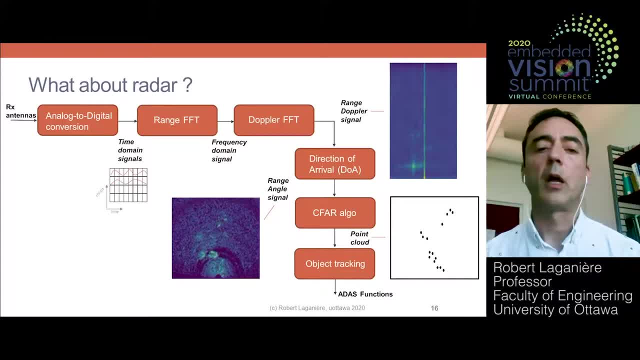 However, this is an expensive sensor and it does not provide any information about the appearance of object, which can make classification and recognition more difficult. However, this is an expensive sensor and it does not provide any information about the appearance of object, which can make classification and recognition more difficult. 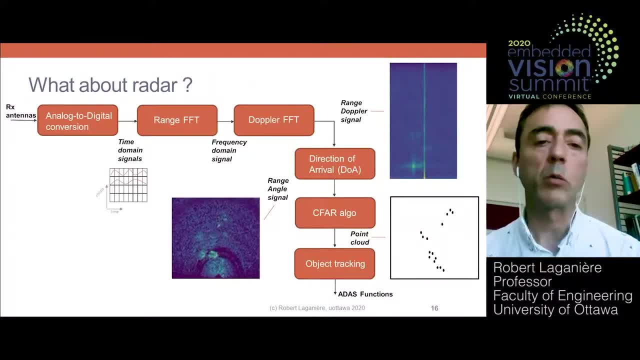 However, this is an expensive sensor and it does not provide any information about the appearance of object, which can make classification and recognition more difficult. However, this is an expensive sensor and it does not provide any information about the appearance of object, which can make classification and recognition more difficult. 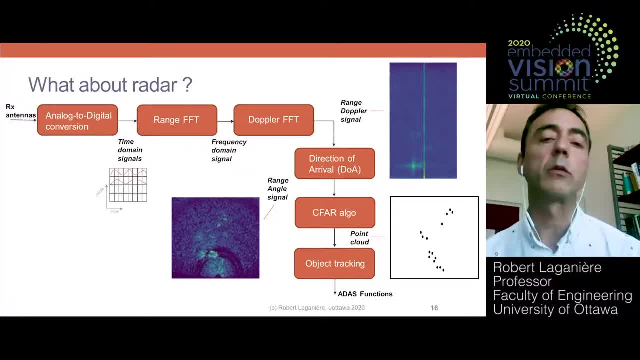 However, this is an expensive sensor and it does not provide any information about the appearance of object, which can make classification and recognition more difficult. However, this is an expensive sensor and it does not provide any information about the appearance of object, which can make classification and recognition more difficult. 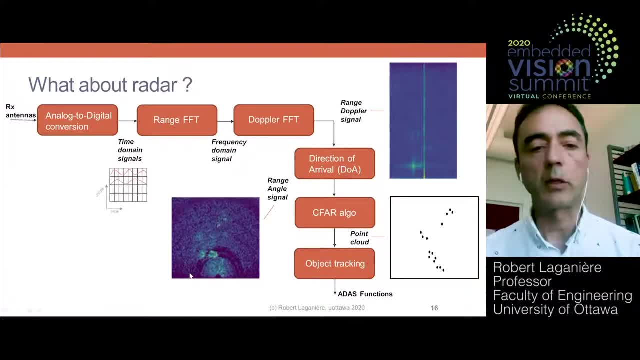 However, this is an expensive sensor and it does not provide any information about the appearance of object, which can make classification and recognition more difficult. However, this is an expensive sensor and it does not provide any information about the appearance of object, which can make classification and recognition more difficult. 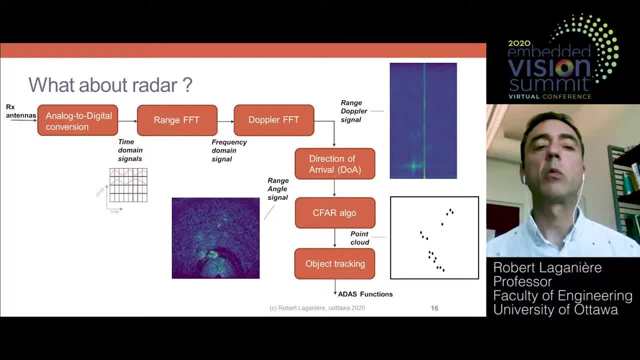 However, this is an expensive sensor and it does not provide any information about the appearance of object, which can make classification and recognition more difficult. However, this is an expensive sensor and it does not provide any information about the appearance of object, which can make classification and recognition more difficult. 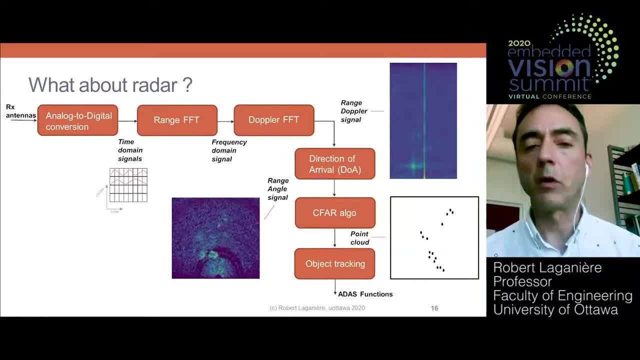 However, this is an expensive sensor and it does not provide any information about the appearance of object, which can make classification and recognition more difficult. However, this is an expensive sensor and it does not provide any information about the appearance of object, which can make classification and recognition more difficult. 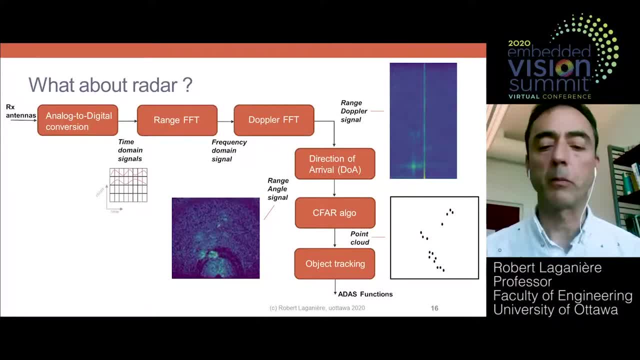 However, this is an expensive sensor and it does not provide any information about the appearance of object, which can make classification and recognition more difficult. However, this is an expensive sensor and it does not provide any information about the appearance of object, which can make classification and recognition more difficult. 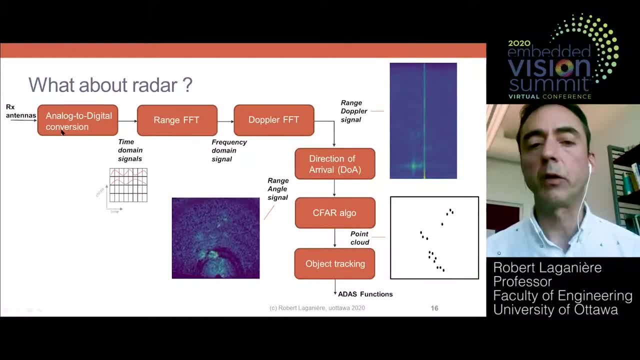 However, this is an expensive sensor and it does not provide any information about the appearance of object, which can make classification and recognition more difficult. However, this is an expensive sensor and it does not provide any information about the appearance of object, which can make classification and recognition more difficult. 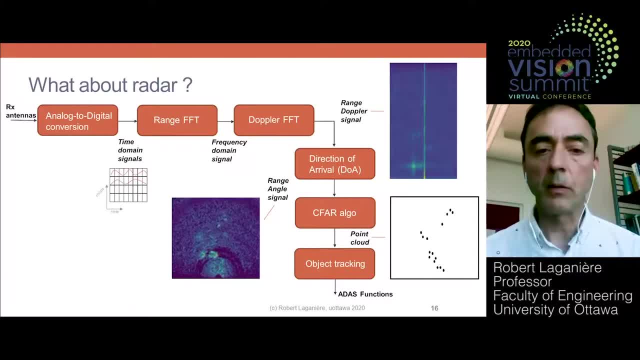 However, this is an expensive sensor and it does not provide any information about the appearance of object, which can make classification and recognition more difficult. However, this is an expensive sensor and it does not provide any information about the appearance of object, which can make classification and recognition more difficult. 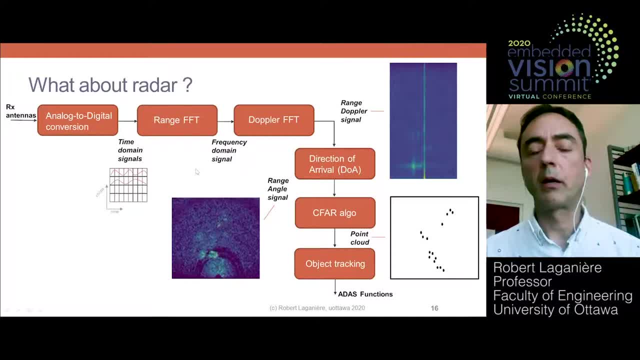 However, this is an expensive sensor and it does not provide any information about the appearance of object, which can make classification and recognition more difficult. However, this is an expensive sensor and it does not provide any information about the appearance of object, which can make classification and recognition more difficult. 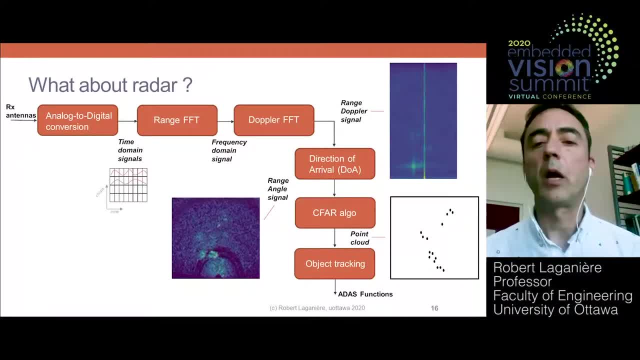 However, this is an expensive sensor and it does not provide any information about the appearance of object, which can make classification and recognition more difficult. However, this is an expensive sensor and it does not provide any information about the appearance of object, which can make classification and recognition more difficult. 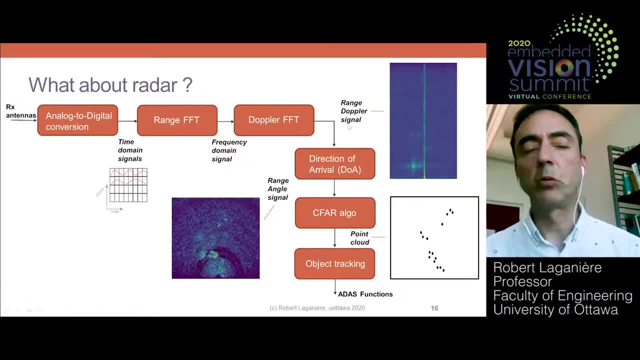 However, this is an expensive sensor and it does not provide any information about the appearance of object, which can make classification and recognition more difficult. However, this is an expensive sensor and it does not provide any information about the appearance of object, which can make classification and recognition more difficult. 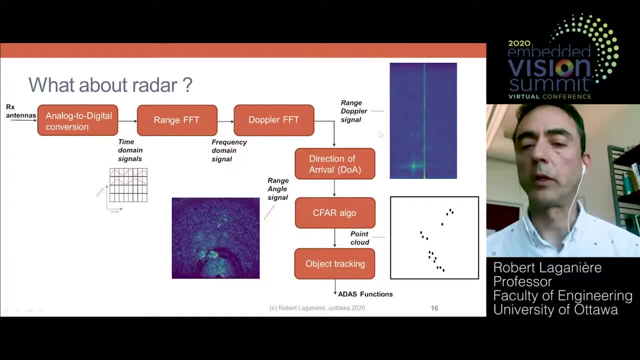 However, this is an expensive sensor and it does not provide any information about the appearance of object, which can make classification and recognition more difficult. However, this is an expensive sensor and it does not provide any information about the appearance of object, which can make classification and recognition more difficult. 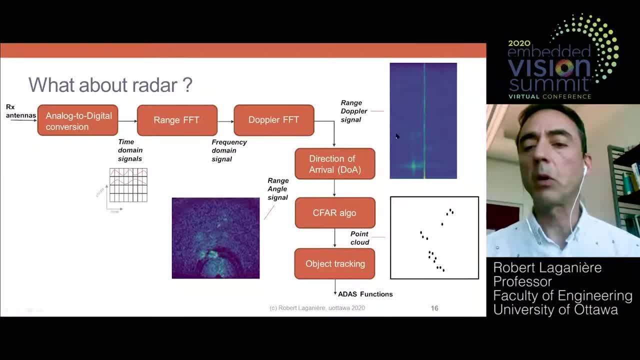 However, this is an expensive sensor and it does not provide any information about the appearance of object, which can make classification and recognition more difficult. However, this is an expensive sensor and it does not provide any information about the appearance of object, which can make classification and recognition more difficult. 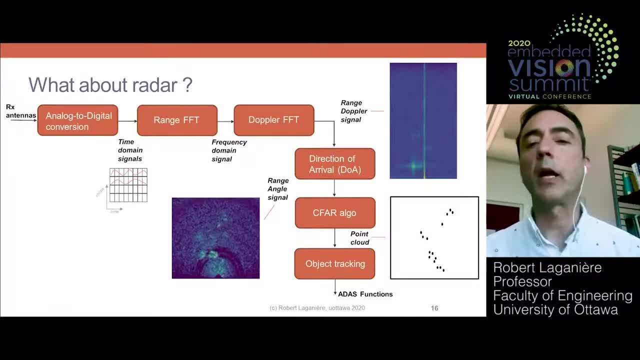 However, this is an expensive sensor and it does not provide any information about the appearance of object, which can make classification and recognition more difficult. However, this is an expensive sensor and it does not provide any information about the appearance of object, which can make classification and recognition more difficult. 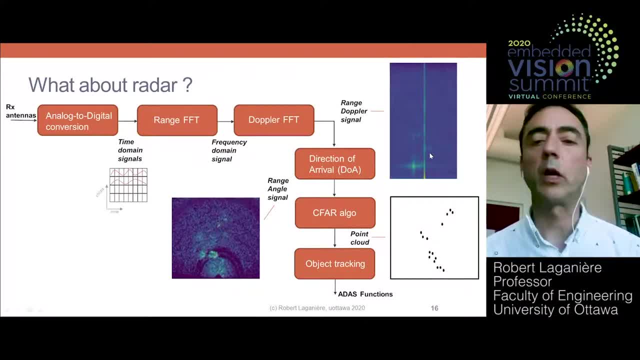 However, this is an expensive sensor and it does not provide any information about the appearance of object, which can make classification and recognition more difficult. However, this is an expensive sensor and it does not provide any information about the appearance of object, which can make classification and recognition more difficult. 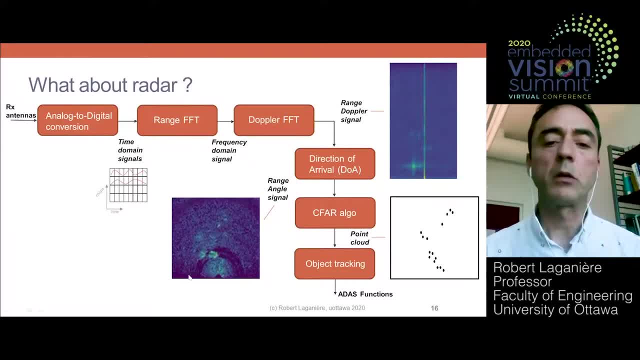 However, this is an expensive sensor and it does not provide any information about the appearance of object, which can make classification and recognition more difficult. However, this is an expensive sensor and it does not provide any information about the appearance of object, which can make classification and recognition more difficult. 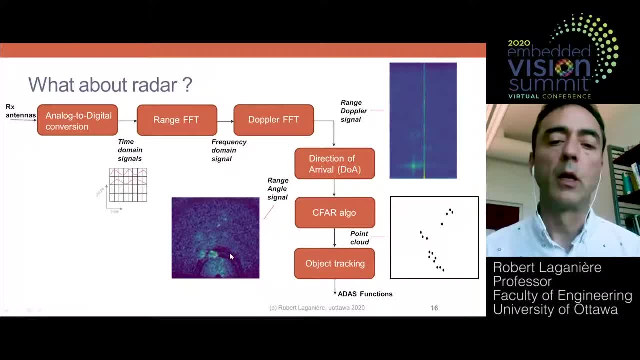 However, this is an expensive sensor and it does not provide any information about the appearance of object, which can make classification and recognition more difficult. However, this is an expensive sensor and it does not provide any information about the appearance of object, which can make classification and recognition more difficult. 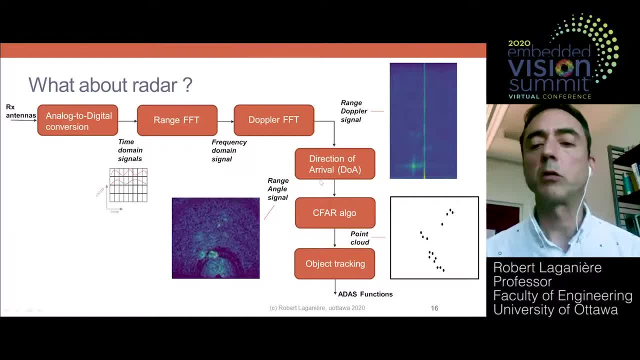 However, this is an expensive sensor and it does not provide any information about the appearance of object, which can make classification and recognition more difficult. However, this is an expensive sensor and it does not provide any information about the appearance of object, which can make classification and recognition more difficult. 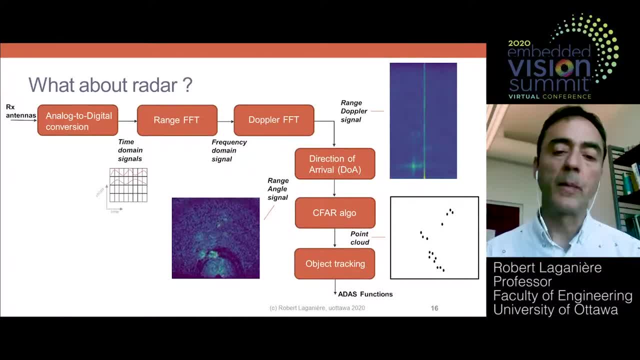 However, this is an expensive sensor and it does not provide any information about the appearance of object, which can make classification and recognition more difficult. However, this is an expensive sensor and it does not provide any information about the appearance of object, which can make classification and recognition more difficult. 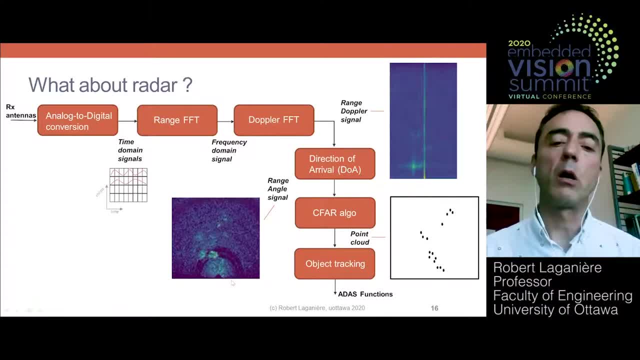 However, this is an expensive sensor and it does not provide any information about the appearance of object, which can make classification and recognition more difficult. However, this is an expensive sensor and it does not provide any information about the appearance of object, which can make classification and recognition more difficult. 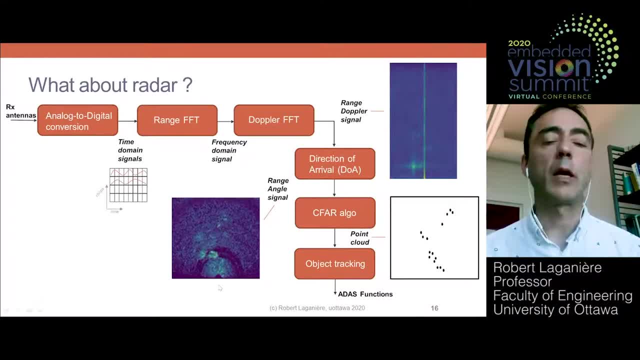 However, this is an expensive sensor and it does not provide any information about the appearance of object, which can make classification and recognition more difficult. However, this is an expensive sensor and it does not provide any information about the appearance of object, which can make classification and recognition more difficult. 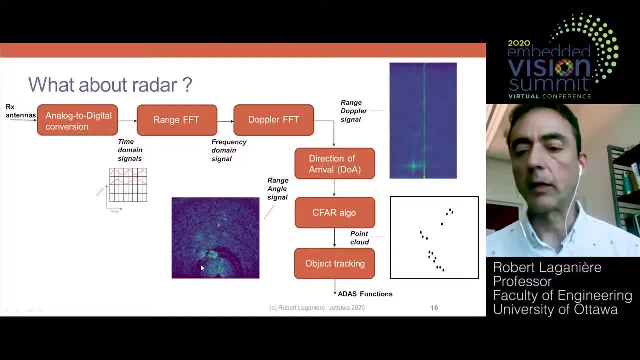 However, this is an expensive sensor and it does not provide any information about the appearance of object, which can make classification and recognition more difficult. However, this is an expensive sensor and it does not provide any information about the appearance of object, which can make classification and recognition more difficult. 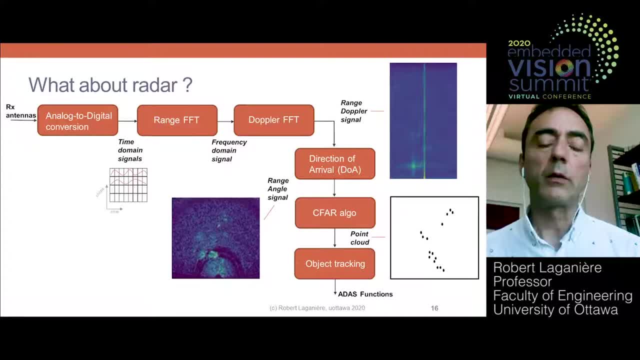 However, this is an expensive sensor and it does not provide any information about the appearance of object, which can make classification and recognition more difficult. However, this is an expensive sensor and it does not provide any information about the appearance of object, which can make classification and recognition more difficult. 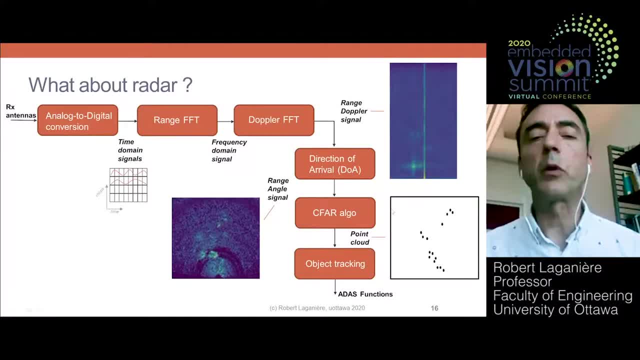 However, this is an expensive sensor and it does not provide any information about the appearance of object, which can make classification and recognition more difficult. However, this is an expensive sensor and it does not provide any information about the appearance of object, which can make classification and recognition more difficult. 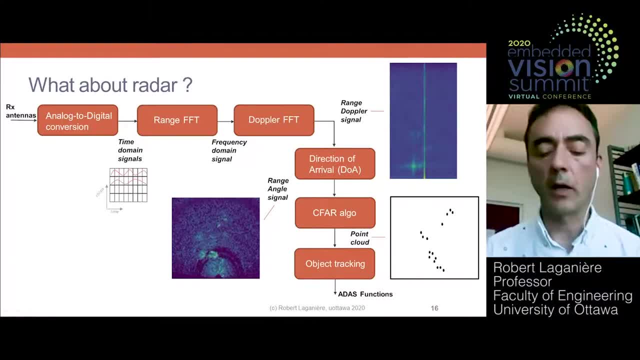 However, this is an expensive sensor and it does not provide any information about the appearance of object, which can make classification and recognition more difficult. However, this is an expensive sensor and it does not provide any information about the appearance of object, which can make classification and recognition more difficult. 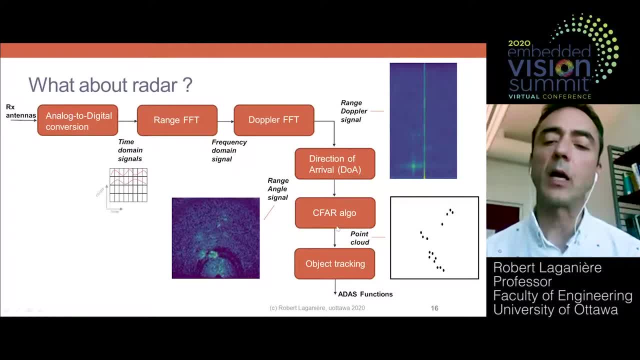 However, this is an expensive sensor and it does not provide any information about the appearance of object, which can make classification and recognition more difficult. However, this is an expensive sensor and it does not provide any information about the appearance of object, which can make classification and recognition more difficult. 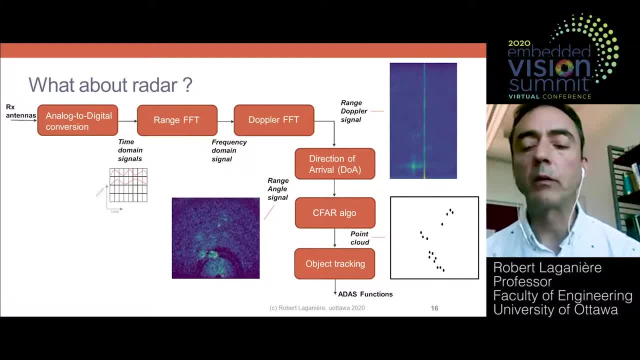 However, this is an expensive sensor and it does not provide any information about the appearance of object, which can make classification and recognition more difficult. However, this is an expensive sensor and it does not provide any information about the appearance of object, which can make classification and recognition more difficult. 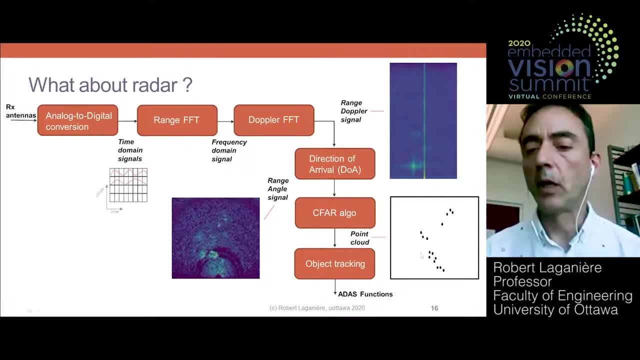 However, this is an expensive sensor and it does not provide any information about the appearance of object, which can make classification and recognition more difficult. However, this is an expensive sensor and it does not provide any information about the appearance of object, which can make classification and recognition more difficult. 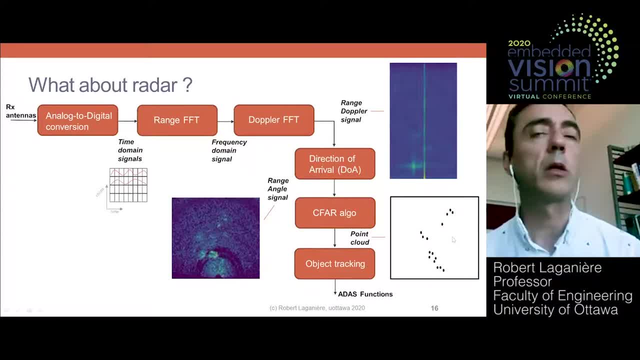 However, this is an expensive sensor and it does not provide any information about the appearance of object, which can make classification and recognition more difficult. However, this is an expensive sensor and it does not provide any information about the appearance of object, which can make classification and recognition more difficult. 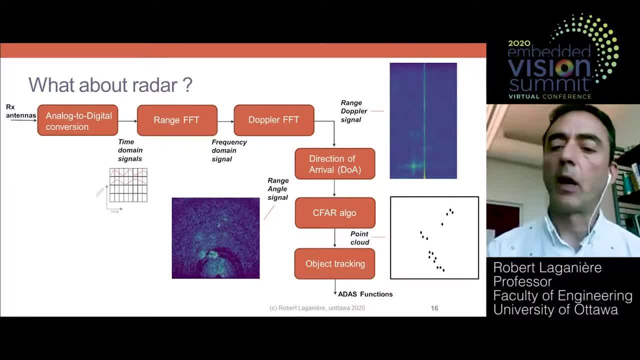 However, this is an expensive sensor and it does not provide any information about the appearance of object, which can make classification and recognition more difficult. However, this is an expensive sensor and it does not provide any information about the appearance of object, which can make classification and recognition more difficult. 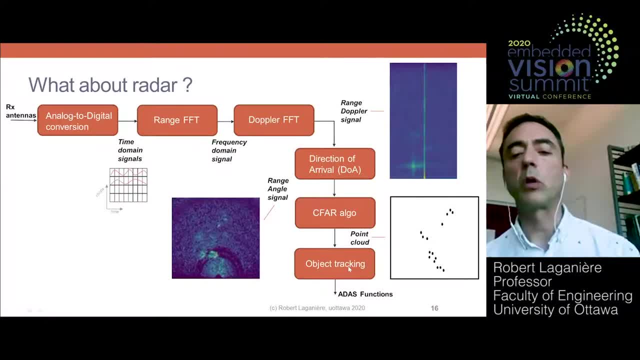 However, this is an expensive sensor and it does not provide any information about the appearance of object, which can make classification and recognition more difficult. However, this is an expensive sensor and it does not provide any information about the appearance of object, which can make classification and recognition more difficult. 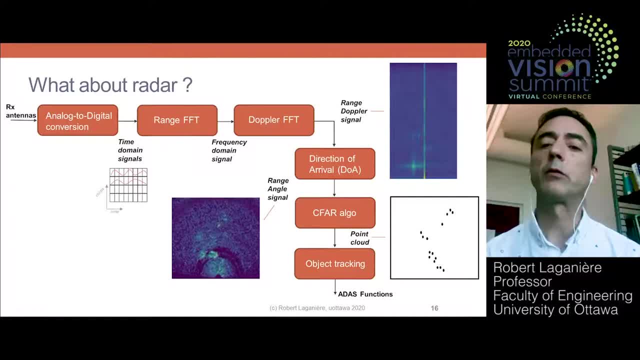 However, this is an expensive sensor and it does not provide any information about the appearance of object, which can make classification and recognition more difficult. However, this is an expensive sensor and it does not provide any information about the appearance of object, which can make classification and recognition more difficult. 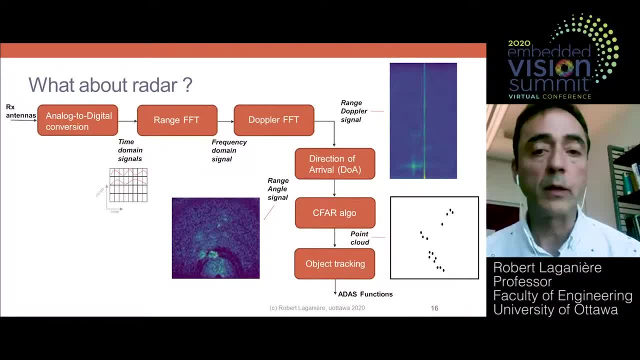 However, this is an expensive sensor and it does not provide any information about the appearance of object, which can make classification and recognition more difficult. However, this is an expensive sensor and it does not provide any information about the appearance of object, which can make classification and recognition more difficult. 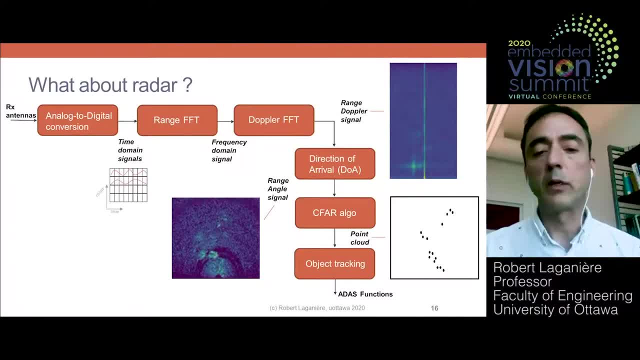 However, this is an expensive sensor and it does not provide any information about the appearance of object, which can make classification and recognition more difficult. However, this is an expensive sensor and it does not provide any information about the appearance of object, which can make classification and recognition more difficult. 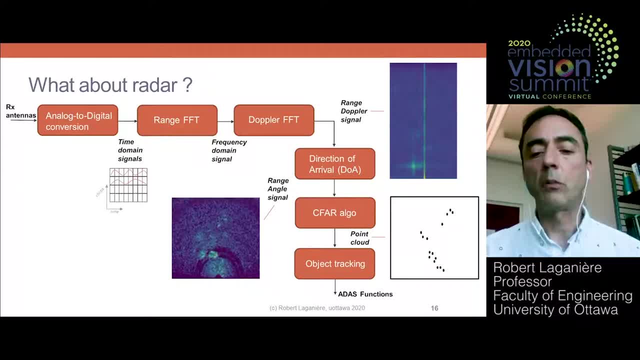 However, this is an expensive sensor and it does not provide any information about the appearance of object, which can make classification and recognition more difficult. However, this is an expensive sensor and it does not provide any information about the appearance of object, which can make classification and recognition more difficult. 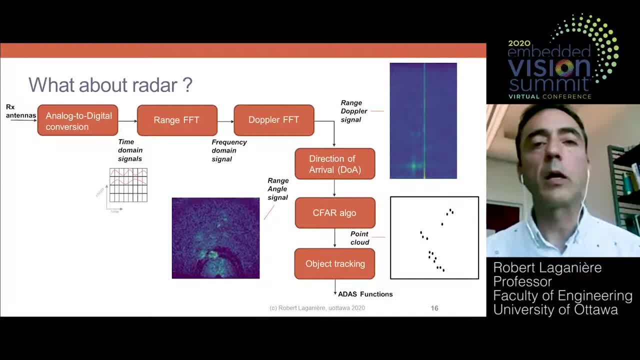 However, this is an expensive sensor and it does not provide any information about the appearance of object, which can make classification and recognition more difficult. However, this is an expensive sensor and it does not provide any information about the appearance of object, which can make classification and recognition more difficult. 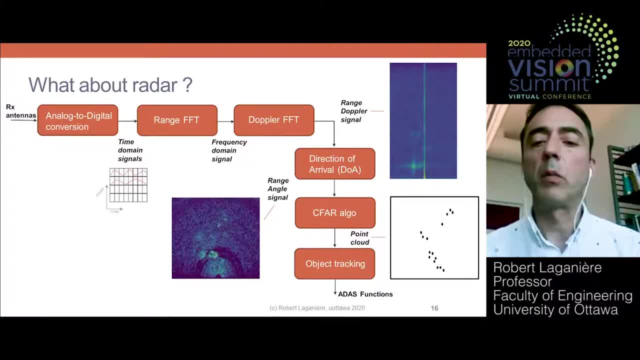 However, this is an expensive sensor and it does not provide any information about the appearance of object, which can make classification and recognition more difficult. However, this is an expensive sensor and it does not provide any information about the appearance of object, which can make classification and recognition more difficult. 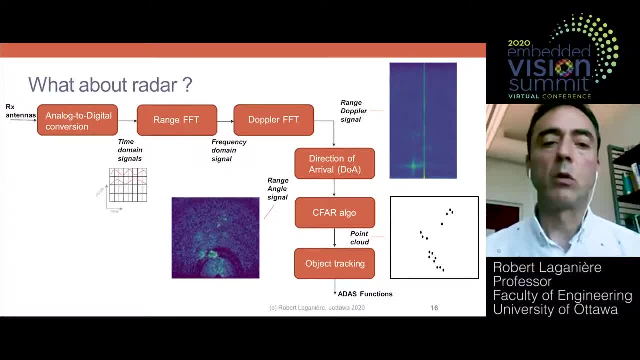 However, this is an expensive sensor and it does not provide any information about the appearance of object, which can make classification and recognition more difficult. However, this is an expensive sensor and it does not provide any information about the appearance of object, which can make classification and recognition more difficult. 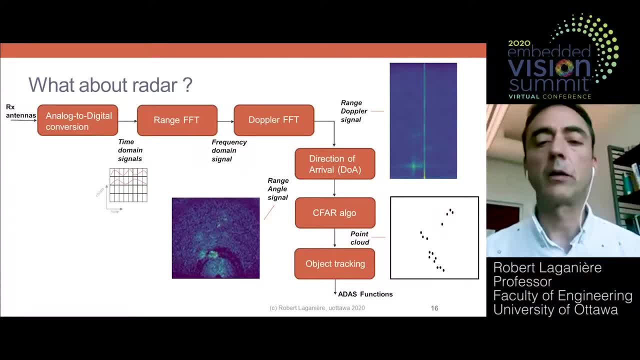 However, this is an expensive sensor and it does not provide any information about the appearance of object, which can make classification and recognition more difficult. However, this is an expensive sensor and it does not provide any information about the appearance of object, which can make classification and recognition more difficult. 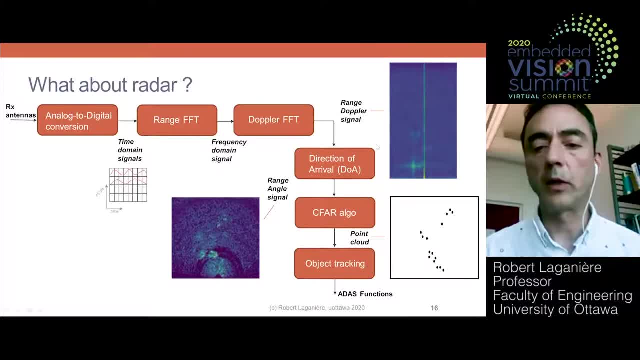 However, this is an expensive sensor and it does not provide any information about the appearance of object, which can make classification and recognition more difficult. However, this is an expensive sensor and it does not provide any information about the appearance of object, which can make classification and recognition more difficult. 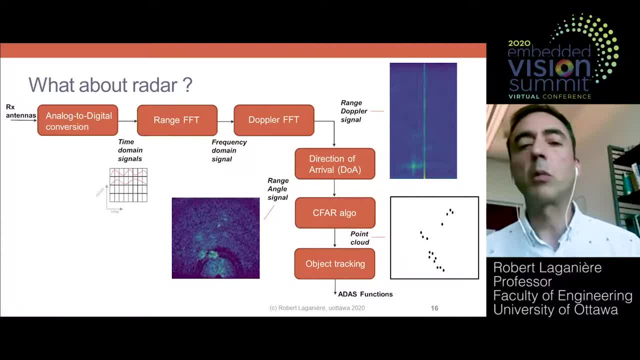 However, this is an expensive sensor and it does not provide any information about the appearance of object, which can make classification and recognition more difficult. However, this is an expensive sensor and it does not provide any information about the appearance of object, which can make classification and recognition more difficult. 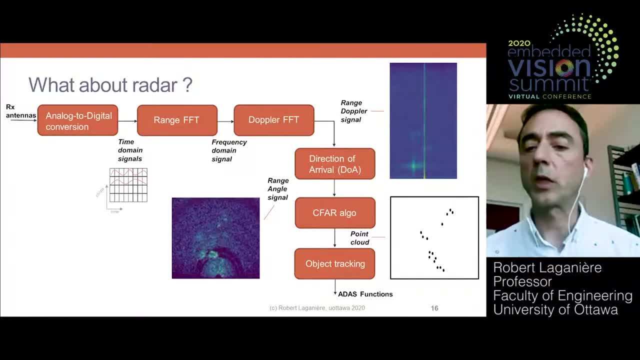 However, this is an expensive sensor and it does not provide any information about the appearance of object, which can make classification and recognition more difficult. However, this is an expensive sensor and it does not provide any information about the appearance of object, which can make classification and recognition more difficult. 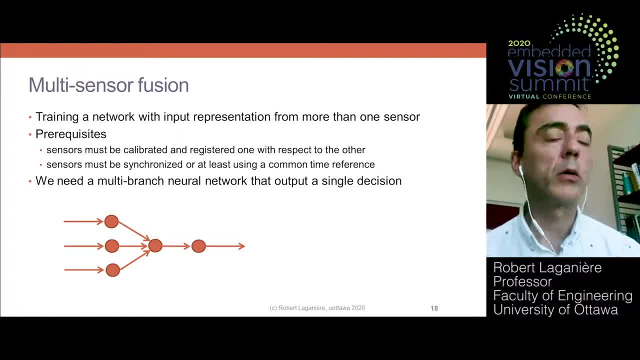 However, this is an expensive sensor and it does not provide any information about the appearance of object, which can make classification and recognition more difficult. However, this is an expensive sensor and it does not provide any information about the appearance of object, which can make classification and recognition more difficult. 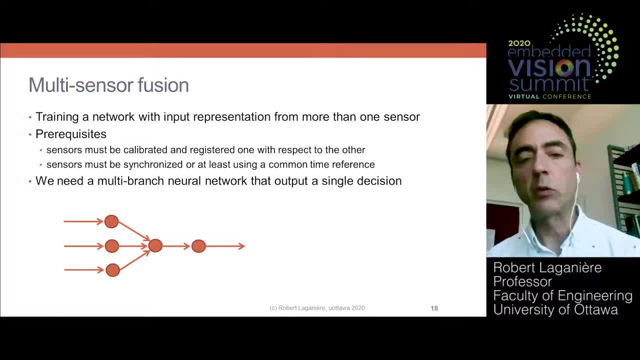 However, this is an expensive sensor and it does not provide any information about the appearance of object, which can make classification and recognition more difficult. However, this is an expensive sensor and it does not provide any information about the appearance of object, which can make classification and recognition more difficult. 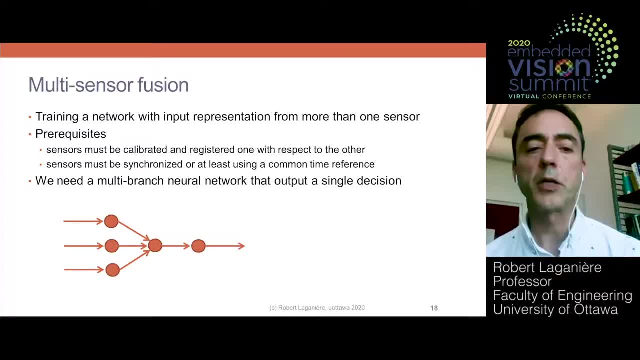 However, this is an expensive sensor and it does not provide any information about the appearance of object, which can make classification and recognition more difficult. However, this is an expensive sensor and it does not provide any information about the appearance of object, which can make classification and recognition more difficult. 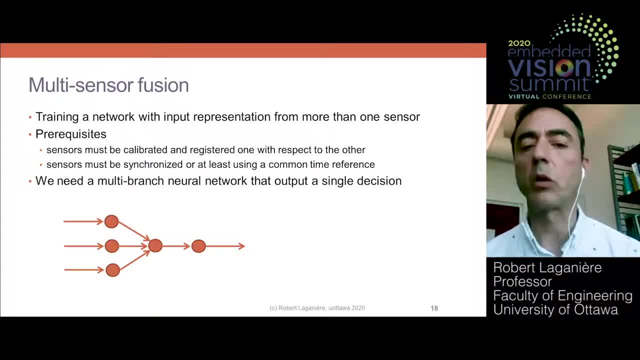 However, this is an expensive sensor and it does not provide any information about the appearance of object, which can make classification and recognition more difficult. However, this is an expensive sensor and it does not provide any information about the appearance of object, which can make classification and recognition more difficult. 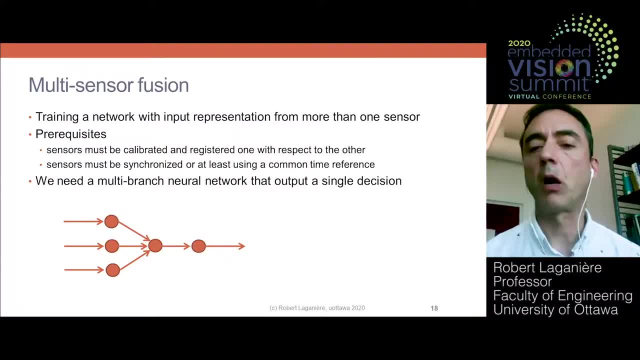 However, this is an expensive sensor and it does not provide any information about the appearance of object, which can make classification and recognition more difficult. However, this is an expensive sensor and it does not provide any information about the appearance of object, which can make classification and recognition more difficult. 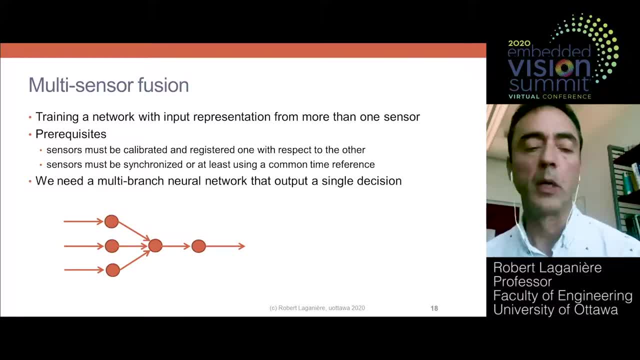 However, this is an expensive sensor and it does not provide any information about the appearance of object, which can make classification and recognition more difficult. However, this is an expensive sensor and it does not provide any information about the appearance of object, which can make classification and recognition more difficult. 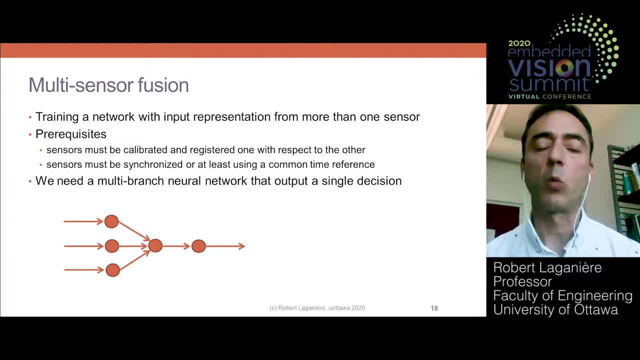 However, this is an expensive sensor and it does not provide any information about the appearance of object, which can make classification and recognition more difficult. However, this is an expensive sensor and it does not provide any information about the appearance of object, which can make classification and recognition more difficult. 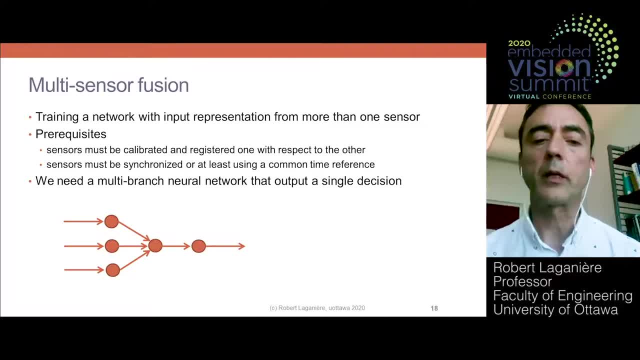 However, this is an expensive sensor and it does not provide any information about the appearance of object, which can make classification and recognition more difficult. However, this is an expensive sensor and it does not provide any information about the appearance of object, which can make classification and recognition more difficult. 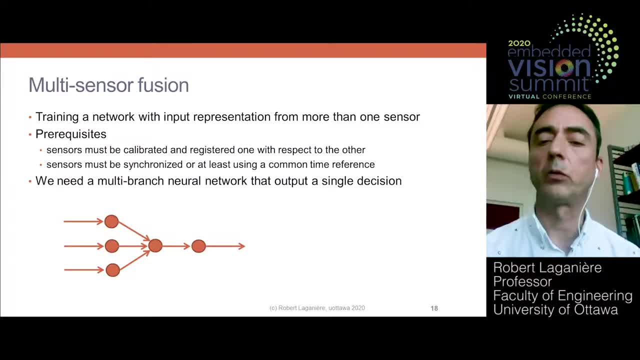 However, this is an expensive sensor and it does not provide any information about the appearance of object, which can make classification and recognition more difficult. However, this is an expensive sensor and it does not provide any information about the appearance of object, which can make classification and recognition more difficult. 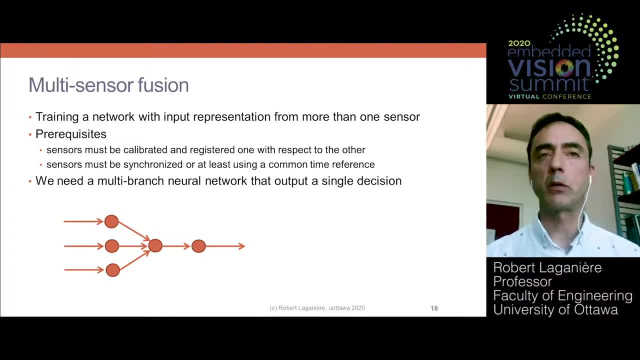 However, this is an expensive sensor and it does not provide any information about the appearance of object, which can make classification and recognition more difficult. However, this is an expensive sensor and it does not provide any information about the appearance of object, which can make classification and recognition more difficult. 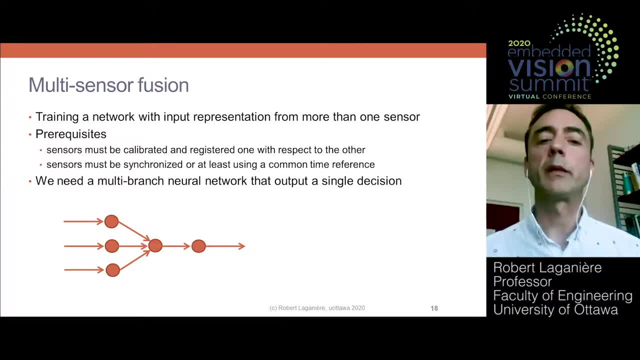 However, this is an expensive sensor and it does not provide any information about the appearance of object, which can make classification and recognition more difficult. However, this is an expensive sensor and it does not provide any information about the appearance of object, which can make classification and recognition more difficult. 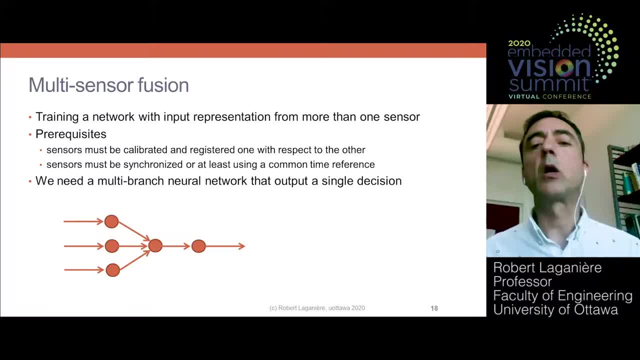 However, this is an expensive sensor and it does not provide any information about the appearance of object, which can make classification and recognition more difficult. However, this is an expensive sensor and it does not provide any information about the appearance of object, which can make classification and recognition more difficult. 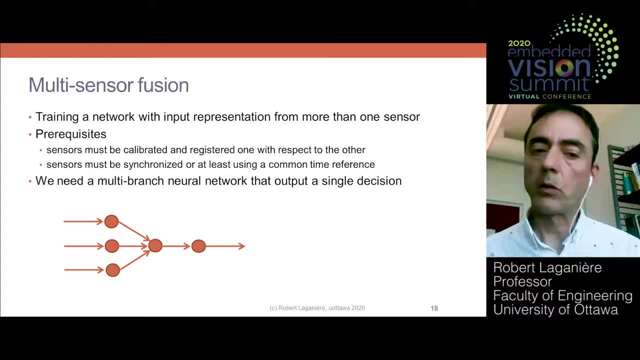 However, this is an expensive sensor and it does not provide any information about the appearance of object, which can make classification and recognition more difficult. However, this is an expensive sensor and it does not provide any information about the appearance of object, which can make classification and recognition more difficult. 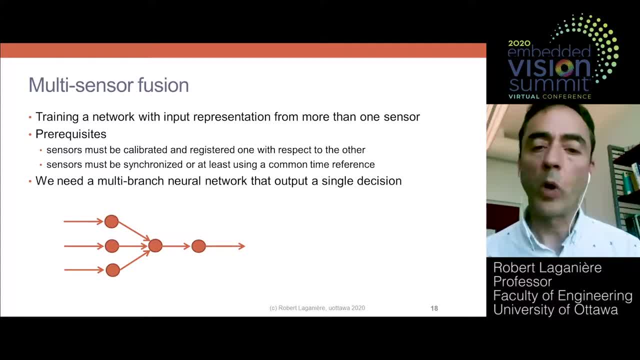 However, this is an expensive sensor and it does not provide any information about the appearance of object, which can make classification and recognition more difficult. However, this is an expensive sensor and it does not provide any information about the appearance of object, which can make classification and recognition more difficult. 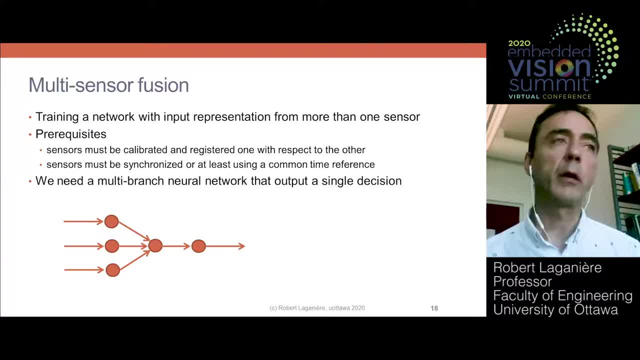 However, this is an expensive sensor and it does not provide any information about the appearance of object, which can make classification and recognition more difficult. However, this is an expensive sensor and it does not provide any information about the appearance of object, which can make classification and recognition more difficult. 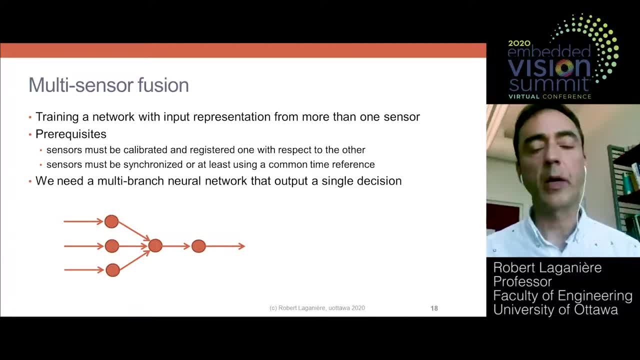 However, this is an expensive sensor and it does not provide any information about the appearance of object, which can make classification and recognition more difficult. However, this is an expensive sensor and it does not provide any information about the appearance of object, which can make classification and recognition more difficult. 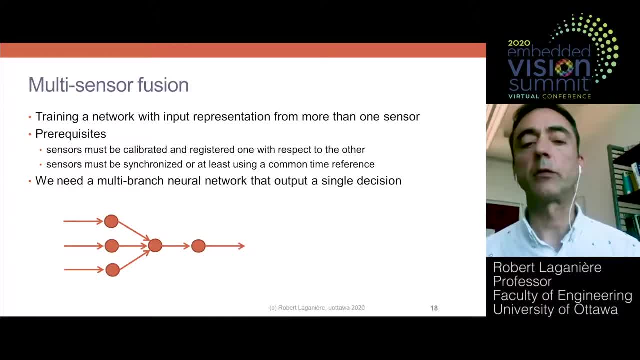 However, this is an expensive sensor and it does not provide any information about the appearance of object, which can make classification and recognition more difficult. However, this is an expensive sensor and it does not provide any information about the appearance of object, which can make classification and recognition more difficult. 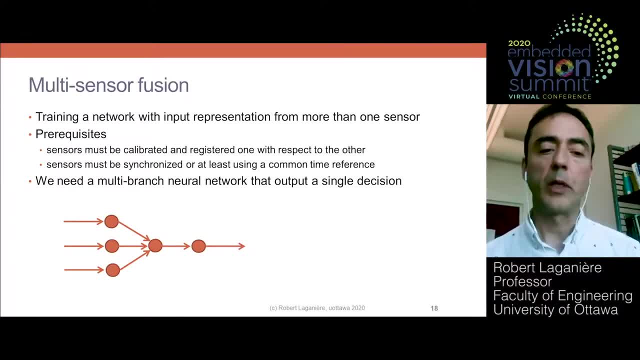 However, this is an expensive sensor and it does not provide any information about the appearance of object, which can make classification and recognition more difficult. However, this is an expensive sensor and it does not provide any information about the appearance of object, which can make classification and recognition more difficult. 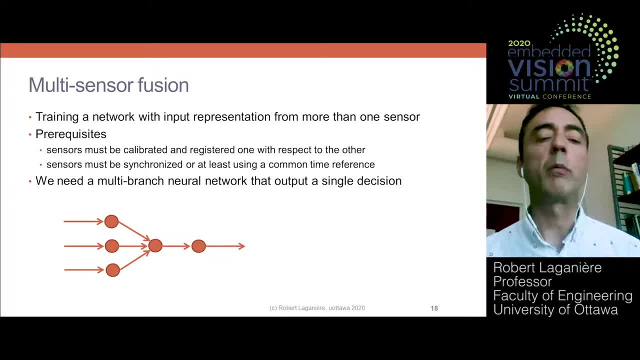 However, this is an expensive sensor and it does not provide any information about the appearance of object, which can make classification and recognition more difficult. However, this is an expensive sensor and it does not provide any information about the appearance of object, which can make classification and recognition more difficult. 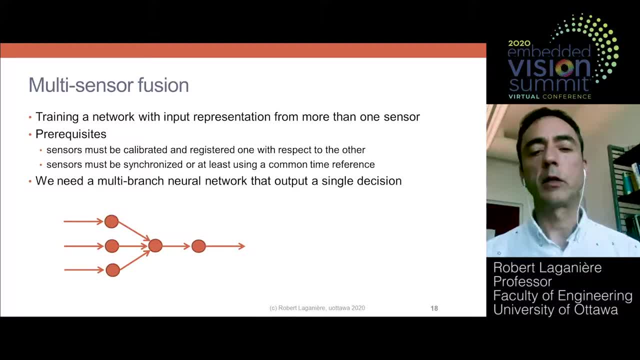 However, this is an expensive sensor and it does not provide any information about the appearance of object, which can make classification and recognition more difficult. However, this is an expensive sensor and it does not provide any information about the appearance of object, which can make classification and recognition more difficult. 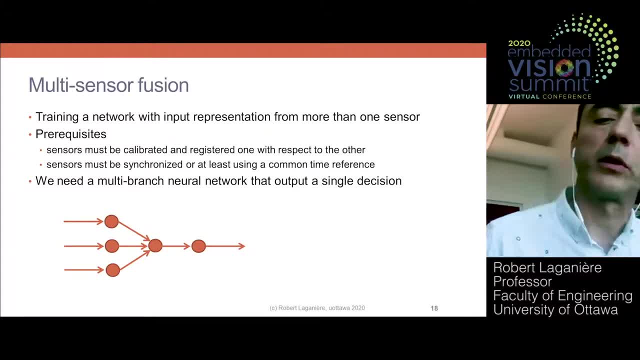 However, this is an expensive sensor and it does not provide any information about the appearance of object, which can make classification and recognition more difficult. However, this is an expensive sensor and it does not provide any information about the appearance of object, which can make classification and recognition more difficult. 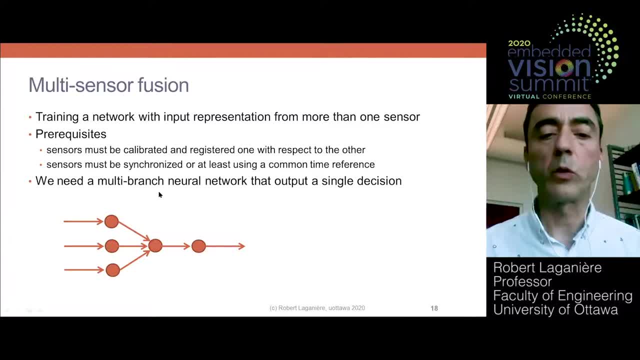 However, this is an expensive sensor and it does not provide any information about the appearance of object, which can make classification and recognition more difficult. However, this is an expensive sensor and it does not provide any information about the appearance of object, which can make classification and recognition more difficult. 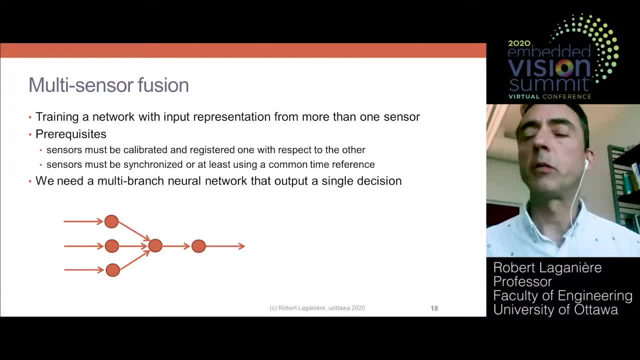 However, this is an expensive sensor and it does not provide any information about the appearance of object, which can make classification and recognition more difficult. However, this is an expensive sensor and it does not provide any information about the appearance of object, which can make classification and recognition more difficult. 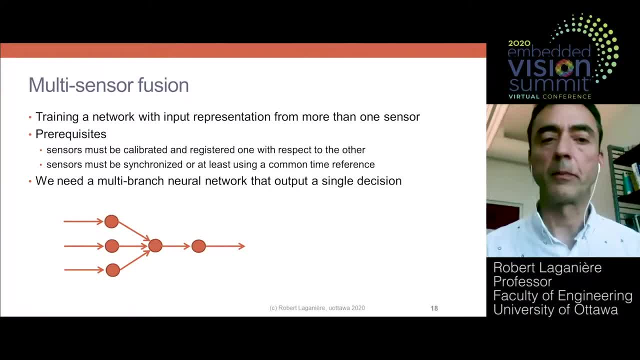 However, this is an expensive sensor and it does not provide any information about the appearance of object, which can make classification and recognition more difficult. However, this is an expensive sensor and it does not provide any information about the appearance of object, which can make classification and recognition more difficult. 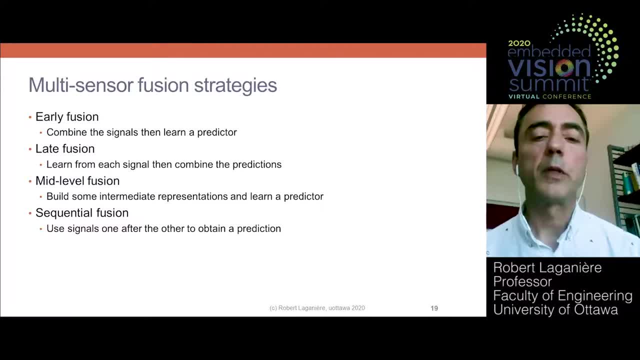 However, this is an expensive sensor and it does not provide any information about the appearance of object, which can make classification and recognition more difficult. However, this is an expensive sensor and it does not provide any information about the appearance of object, which can make classification and recognition more difficult. 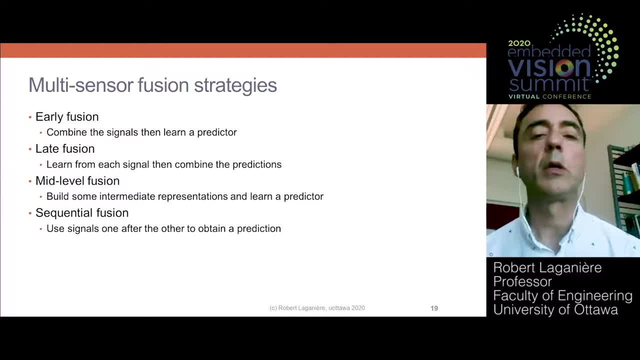 However, this is an expensive sensor and it does not provide any information about the appearance of object, which can make classification and recognition more difficult. However, this is an expensive sensor and it does not provide any information about the appearance of object, which can make classification and recognition more difficult. 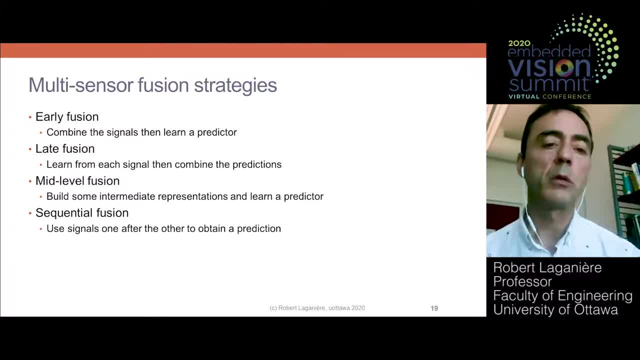 However, this is an expensive sensor and it does not provide any information about the appearance of object, which can make classification and recognition more difficult. However, this is an expensive sensor and it does not provide any information about the appearance of object, which can make classification and recognition more difficult. 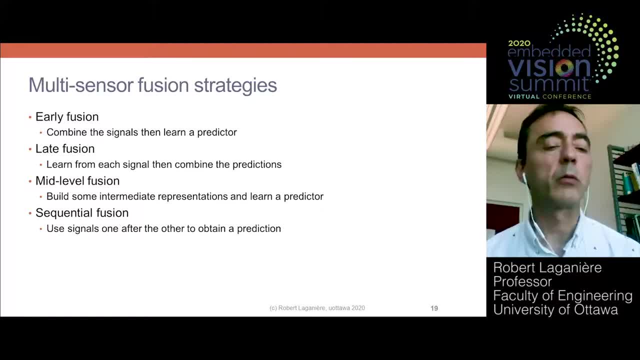 However, this is an expensive sensor and it does not provide any information about the appearance of object, which can make classification and recognition more difficult. However, this is an expensive sensor and it does not provide any information about the appearance of object, which can make classification and recognition more difficult. 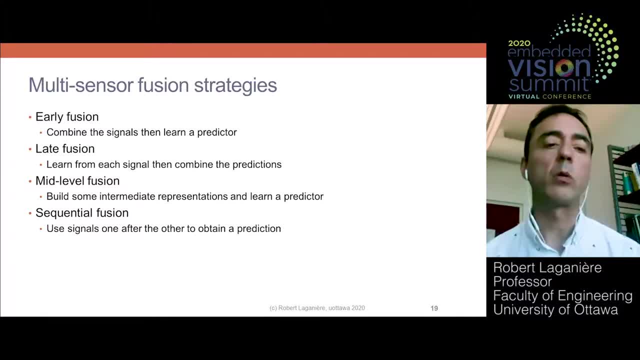 However, this is an expensive sensor and it does not provide any information about the appearance of object, which can make classification and recognition more difficult. However, this is an expensive sensor and it does not provide any information about the appearance of object, which can make classification and recognition more difficult. 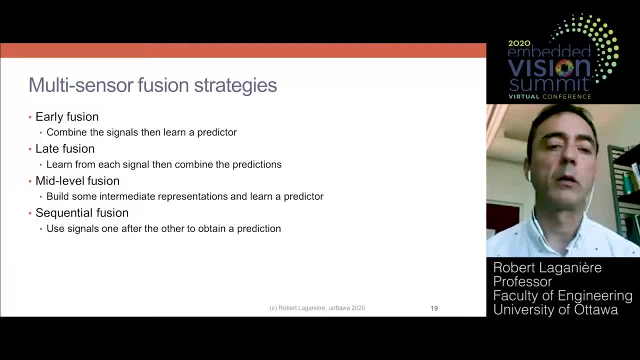 However, this is an expensive sensor and it does not provide any information about the appearance of object, which can make classification and recognition more difficult. However, this is an expensive sensor and it does not provide any information about the appearance of object, which can make classification and recognition more difficult. 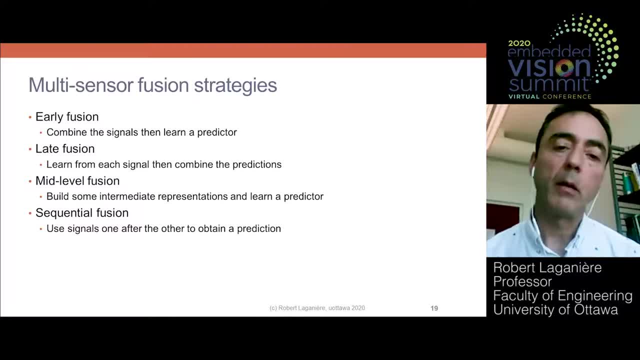 However, this is an expensive sensor and it does not provide any information about the appearance of object, which can make classification and recognition more difficult. However, this is an expensive sensor and it does not provide any information about the appearance of object, which can make classification and recognition more difficult. 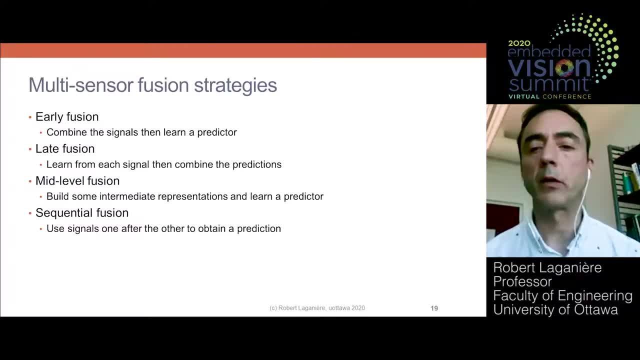 However, this is an expensive sensor and it does not provide any information about the appearance of object, which can make classification and recognition more difficult. However, this is an expensive sensor and it does not provide any information about the appearance of object, which can make classification and recognition more difficult. 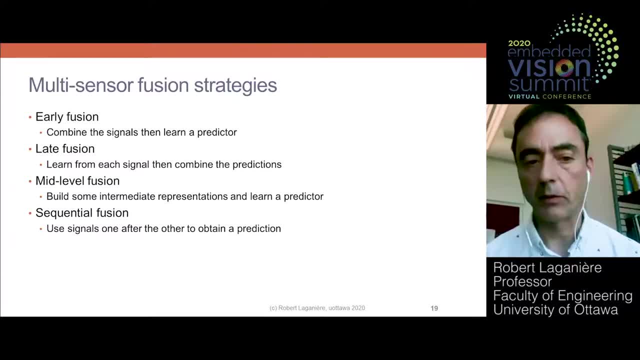 However, this is an expensive sensor and it does not provide any information about the appearance of object, which can make classification and recognition more difficult. However, this is an expensive sensor and it does not provide any information about the appearance of object, which can make classification and recognition more difficult. 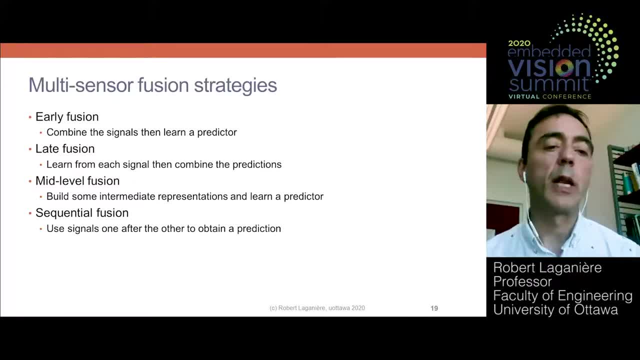 However, this is an expensive sensor and it does not provide any information about the appearance of object, which can make classification and recognition more difficult. However, this is an expensive sensor and it does not provide any information about the appearance of object, which can make classification and recognition more difficult. 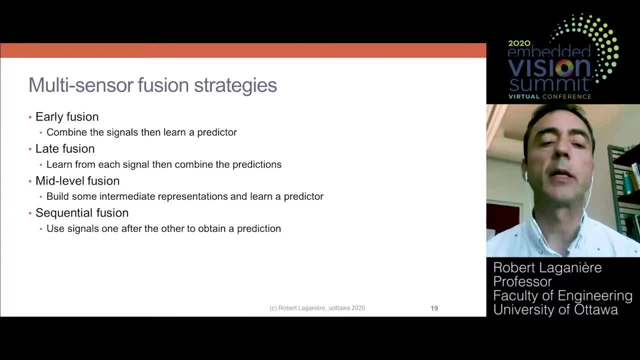 However, this is an expensive sensor and it does not provide any information about the appearance of object, which can make classification and recognition more difficult. However, this is an expensive sensor and it does not provide any information about the appearance of object, which can make classification and recognition more difficult. 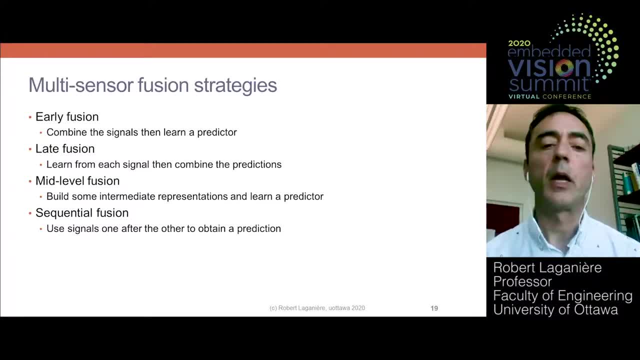 However, this is an expensive sensor and it does not provide any information about the appearance of object, which can make classification and recognition more difficult. However, this is an expensive sensor and it does not provide any information about the appearance of object, which can make classification and recognition more difficult. 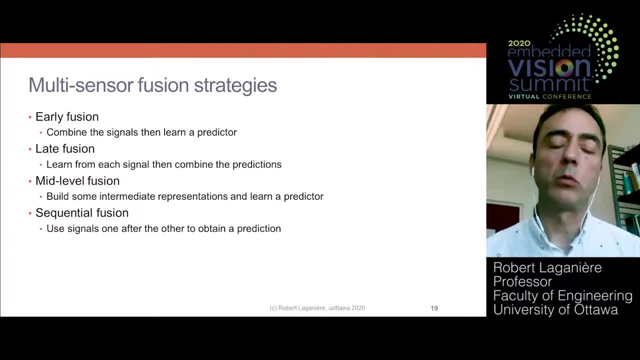 However, this is an expensive sensor and it does not provide any information about the appearance of object, which can make classification and recognition more difficult. However, this is an expensive sensor and it does not provide any information about the appearance of object, which can make classification and recognition more difficult. 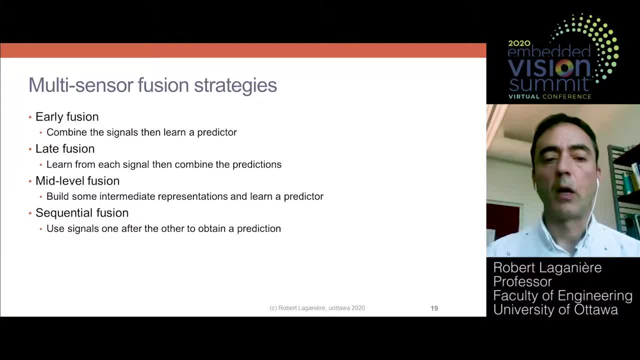 However, this is an expensive sensor and it does not provide any information about the appearance of object, which can make classification and recognition more difficult. However, this is an expensive sensor and it does not provide any information about the appearance of object, which can make classification and recognition more difficult. 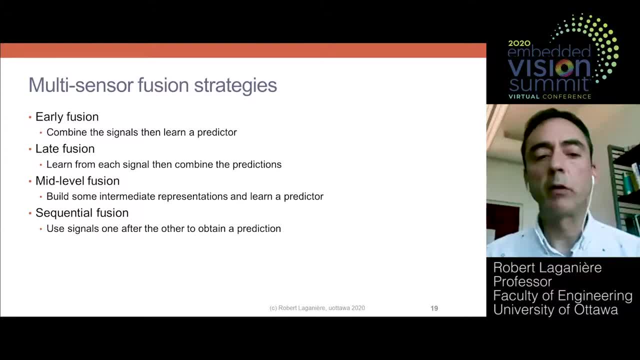 However, this is an expensive sensor and it does not provide any information about the appearance of object, which can make classification and recognition more difficult. However, this is an expensive sensor and it does not provide any information about the appearance of object, which can make classification and recognition more difficult. 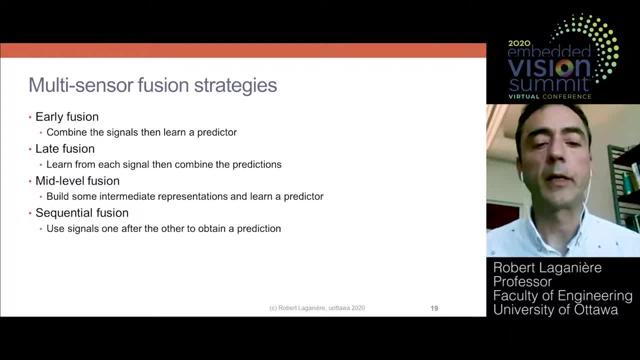 However, this is an expensive sensor and it does not provide any information about the appearance of object, which can make classification and recognition more difficult. However, this is an expensive sensor and it does not provide any information about the appearance of object, which can make classification and recognition more difficult. 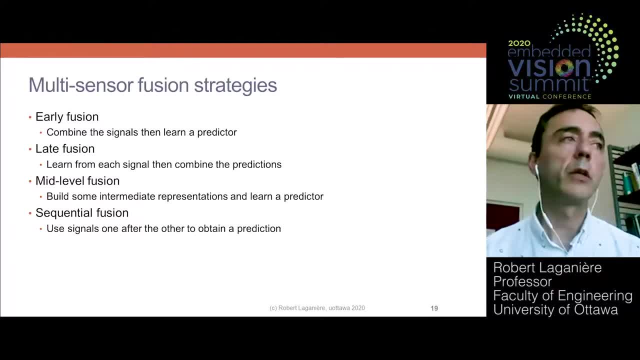 However, this is an expensive sensor and it does not provide any information about the appearance of object, which can make classification and recognition more difficult. However, this is an expensive sensor and it does not provide any information about the appearance of object, which can make classification and recognition more difficult. 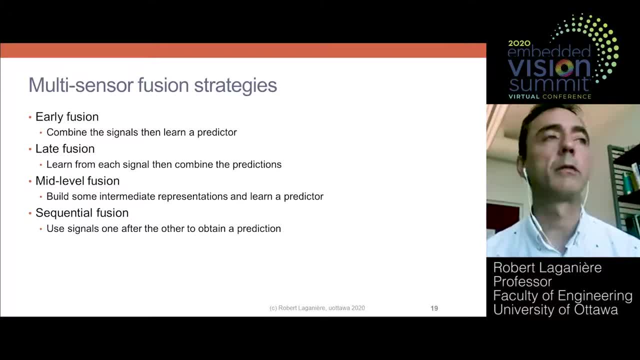 However, this is an expensive sensor and it does not provide any information about the appearance of object, which can make classification and recognition more difficult. However, this is an expensive sensor and it does not provide any information about the appearance of object, which can make classification and recognition more difficult. 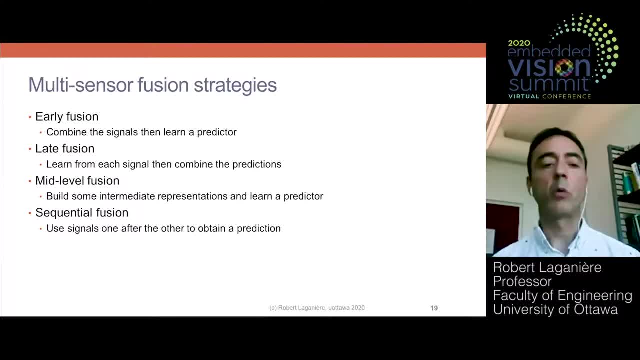 However, this is an expensive sensor and it does not provide any information about the appearance of object, which can make classification and recognition more difficult. However, this is an expensive sensor and it does not provide any information about the appearance of object, which can make classification and recognition more difficult. 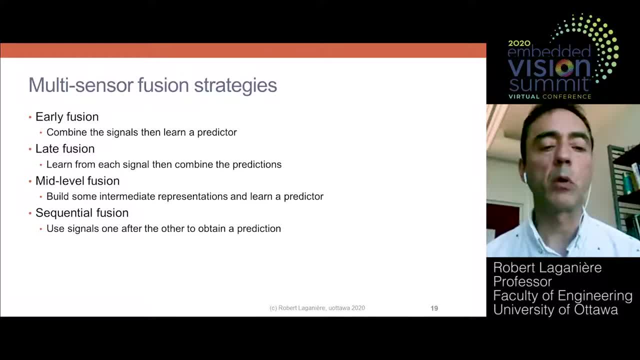 However, this is an expensive sensor and it does not provide any information about the appearance of object, which can make classification and recognition more difficult. However, this is an expensive sensor and it does not provide any information about the appearance of object, which can make classification and recognition more difficult. 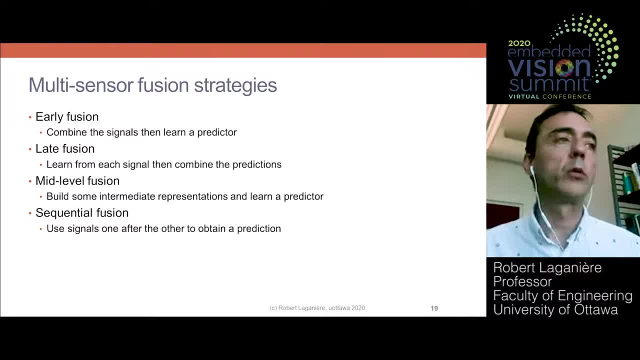 However, this is an expensive sensor and it does not provide any information about the appearance of object, which can make classification and recognition more difficult. However, this is an expensive sensor and it does not provide any information about the appearance of object, which can make classification and recognition more difficult. 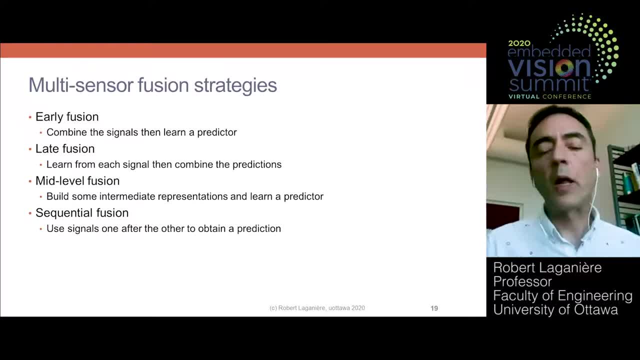 However, this is an expensive sensor and it does not provide any information about the appearance of object, which can make classification and recognition more difficult. However, this is an expensive sensor and it does not provide any information about the appearance of object, which can make classification and recognition more difficult. 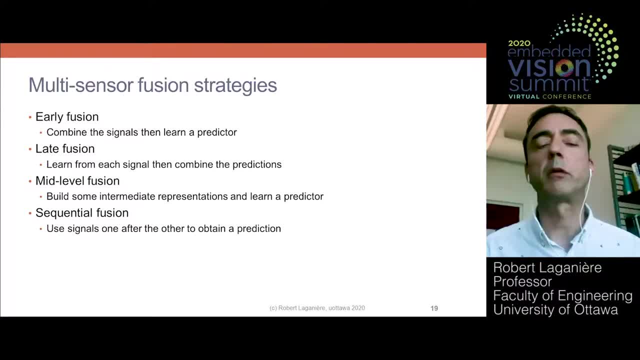 However, this is an expensive sensor and it does not provide any information about the appearance of object, which can make classification and recognition more difficult. However, this is an expensive sensor and it does not provide any information about the appearance of object, which can make classification and recognition more difficult. 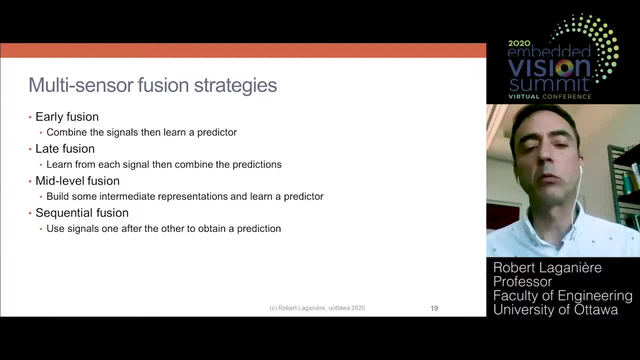 However, this is an expensive sensor and it does not provide any information about the appearance of object, which can make classification and recognition more difficult. However, this is an expensive sensor and it does not provide any information about the appearance of object, which can make classification and recognition more difficult. 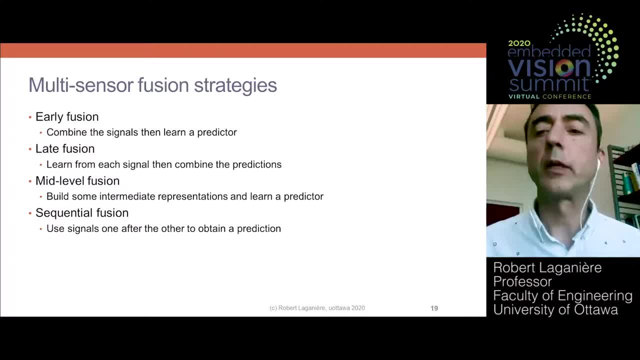 However, this is an expensive sensor and it does not provide any information about the appearance of object, which can make classification and recognition more difficult. However, this is an expensive sensor and it does not provide any information about the appearance of object, which can make classification and recognition more difficult. 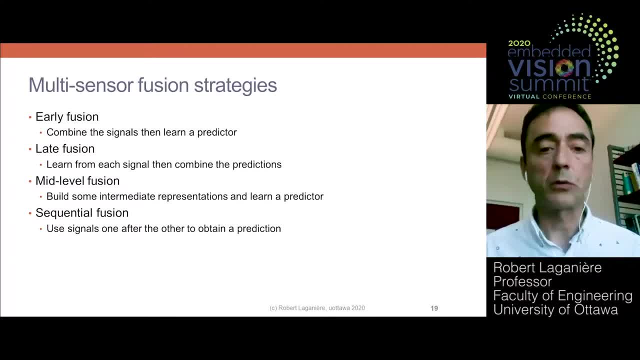 However, this is an expensive sensor and it does not provide any information about the appearance of object, which can make classification and recognition more difficult. However, this is an expensive sensor and it does not provide any information about the appearance of object, which can make classification and recognition more difficult. 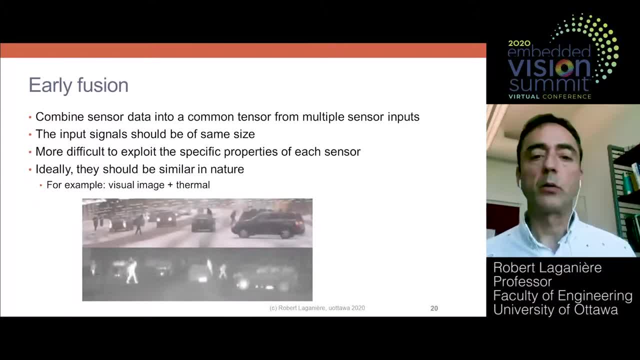 However, this is an expensive sensor and it does not provide any information about the appearance of object, which can make classification and recognition more difficult. However, this is an expensive sensor and it does not provide any information about the appearance of object, which can make classification and recognition more difficult. 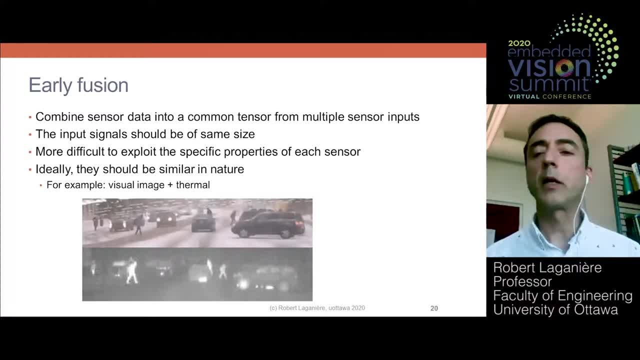 However, this is an expensive sensor and it does not provide any information about the appearance of object, which can make classification and recognition more difficult. However, this is an expensive sensor and it does not provide any information about the appearance of object, which can make classification and recognition more difficult. 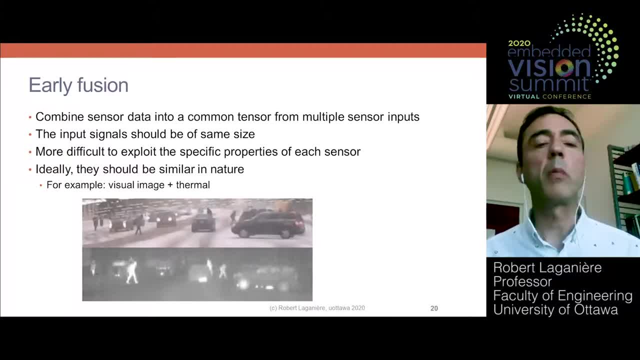 However, this is an expensive sensor and it does not provide any information about the appearance of object, which can make classification and recognition more difficult. However, this is an expensive sensor and it does not provide any information about the appearance of object, which can make classification and recognition more difficult. 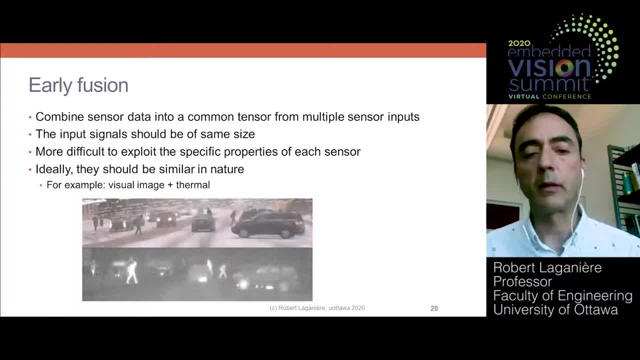 However, this is an expensive sensor and it does not provide any information about the appearance of object, which can make classification and recognition more difficult. However, this is an expensive sensor and it does not provide any information about the appearance of object, which can make classification and recognition more difficult. 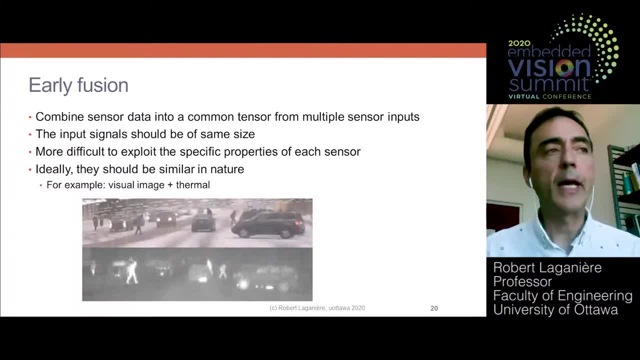 However, this is an expensive sensor and it does not provide any information about the appearance of object, which can make classification and recognition more difficult. However, this is an expensive sensor and it does not provide any information about the appearance of object, which can make classification and recognition more difficult. 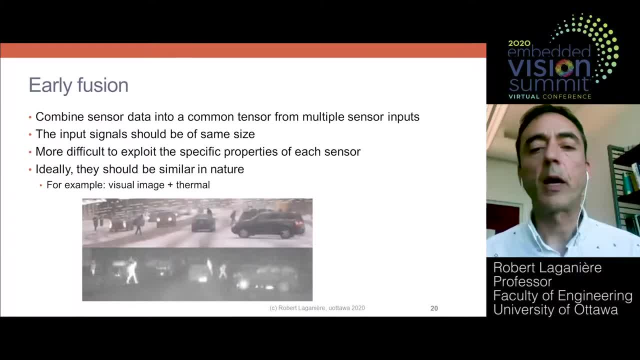 However, this is an expensive sensor and it does not provide any information about the appearance of object, which can make classification and recognition more difficult. However, this is an expensive sensor and it does not provide any information about the appearance of object, which can make classification and recognition more difficult. 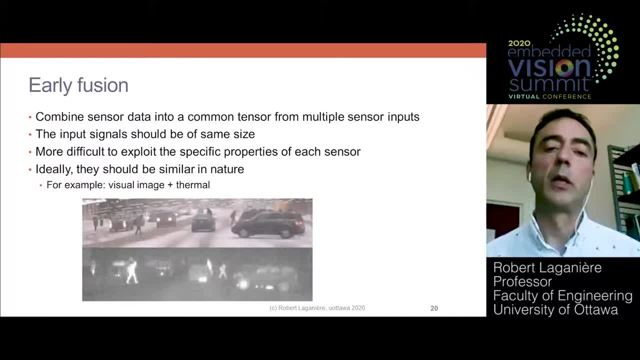 However, this is an expensive sensor and it does not provide any information about the appearance of object, which can make classification and recognition more difficult. However, this is an expensive sensor and it does not provide any information about the appearance of object, which can make classification and recognition more difficult. 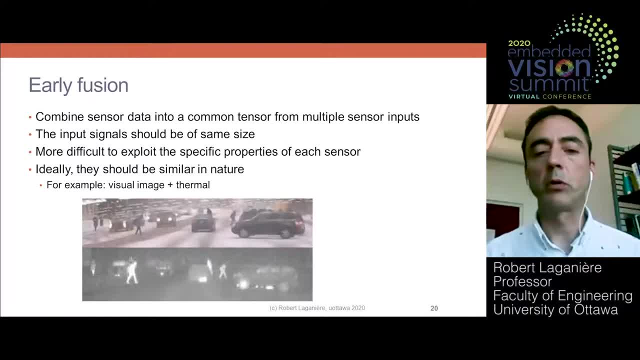 However, this is an expensive sensor and it does not provide any information about the appearance of object, which can make classification and recognition more difficult. However, this is an expensive sensor and it does not provide any information about the appearance of object, which can make classification and recognition more difficult. 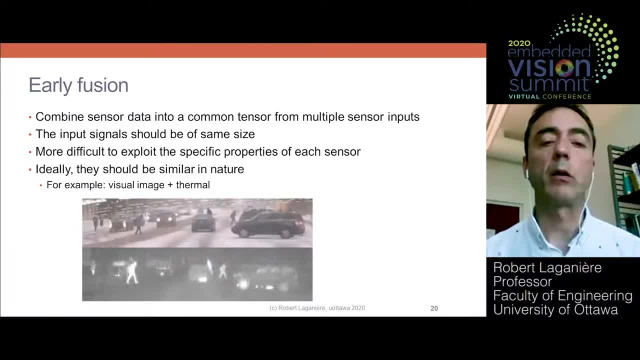 However, this is an expensive sensor and it does not provide any information about the appearance of object, which can make classification and recognition more difficult. However, this is an expensive sensor and it does not provide any information about the appearance of object, which can make classification and recognition more difficult. 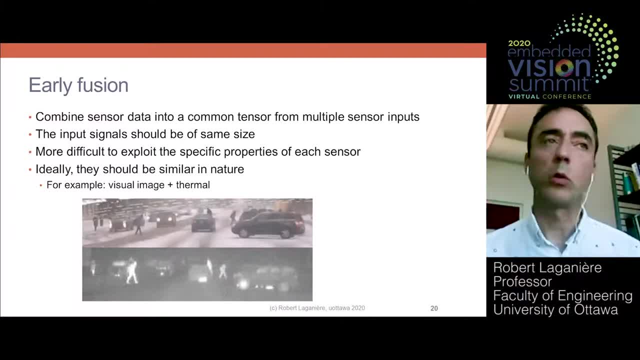 However, this is an expensive sensor and it does not provide any information about the appearance of object, which can make classification and recognition more difficult. However, this is an expensive sensor and it does not provide any information about the appearance of object, which can make classification and recognition more difficult. 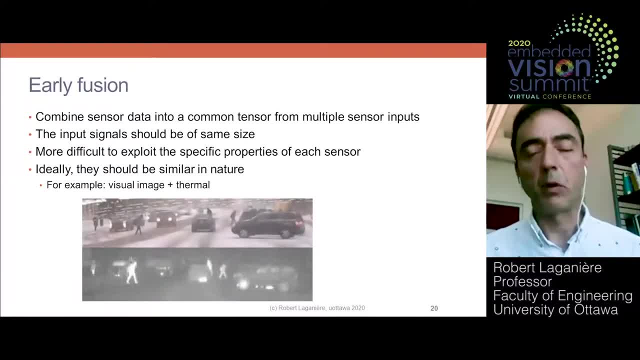 However, this is an expensive sensor and it does not provide any information about the appearance of object, which can make classification and recognition more difficult. However, this is an expensive sensor and it does not provide any information about the appearance of object, which can make classification and recognition more difficult. 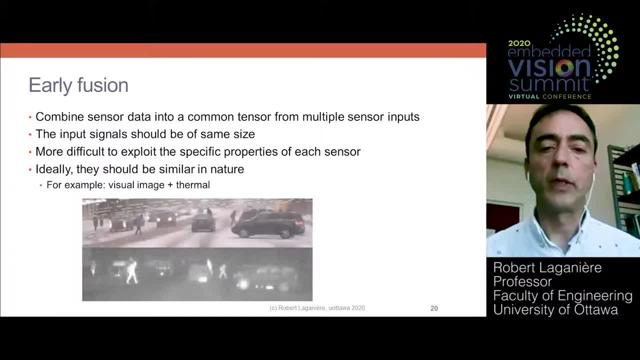 However, this is an expensive sensor and it does not provide any information about the appearance of object, which can make classification and recognition more difficult. However, this is an expensive sensor and it does not provide any information about the appearance of object, which can make classification and recognition more difficult. 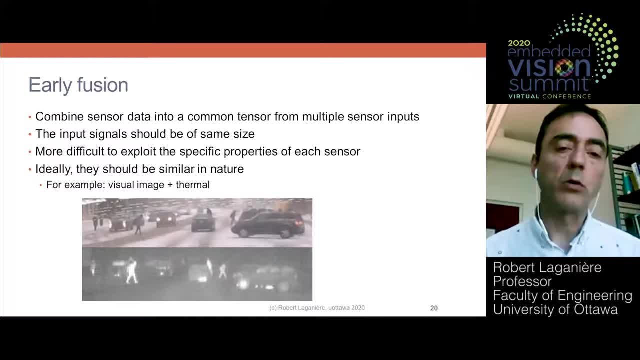 However, this is an expensive sensor and it does not provide any information about the appearance of object, which can make classification and recognition more difficult. However, this is an expensive sensor and it does not provide any information about the appearance of object, which can make classification and recognition more difficult. 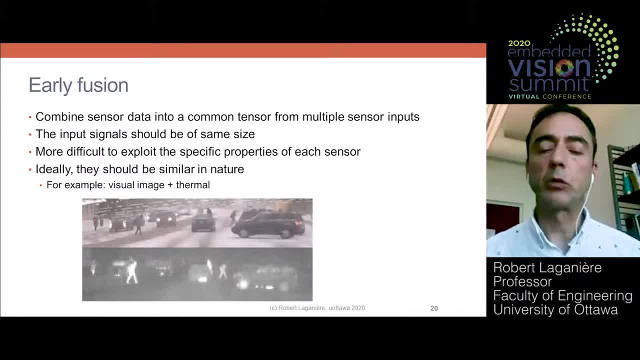 However, this is an expensive sensor and it does not provide any information about the appearance of object, which can make classification and recognition more difficult. However, this is an expensive sensor and it does not provide any information about the appearance of object, which can make classification and recognition more difficult. 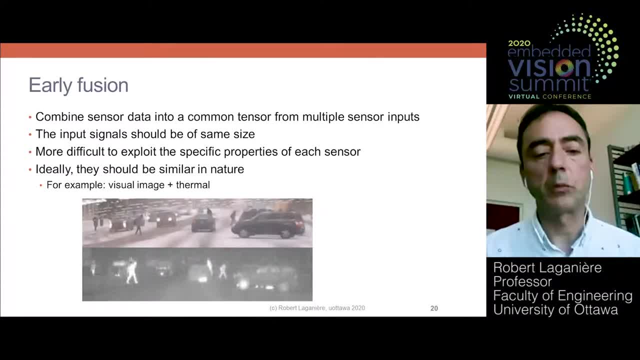 However, this is an expensive sensor and it does not provide any information about the appearance of object, which can make classification and recognition more difficult. However, this is an expensive sensor and it does not provide any information about the appearance of object, which can make classification and recognition more difficult. 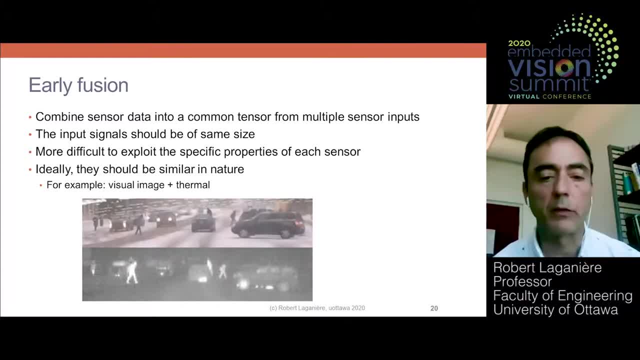 However, this is an expensive sensor and it does not provide any information about the appearance of object, which can make classification and recognition more difficult. However, this is an expensive sensor and it does not provide any information about the appearance of object, which can make classification and recognition more difficult. 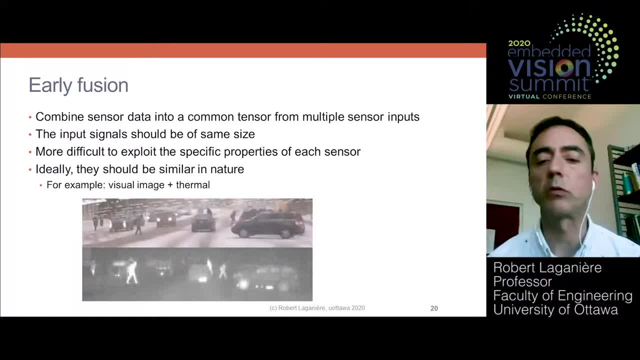 However, this is an expensive sensor and it does not provide any information about the appearance of object, which can make classification and recognition more difficult. However, this is an expensive sensor and it does not provide any information about the appearance of object, which can make classification and recognition more difficult. 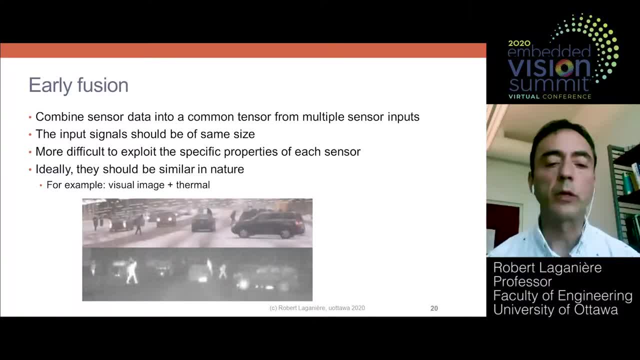 However, this is an expensive sensor and it does not provide any information about the appearance of object, which can make classification and recognition more difficult. However, this is an expensive sensor and it does not provide any information about the appearance of object, which can make classification and recognition more difficult. 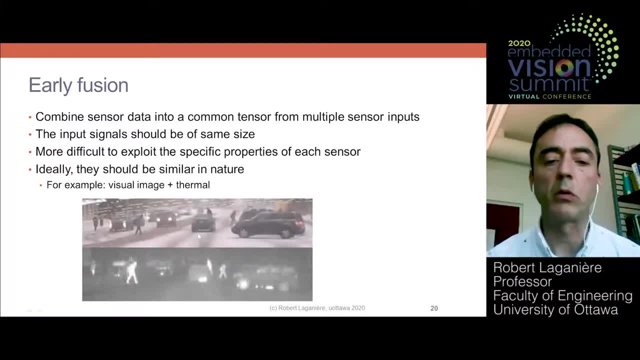 However, this is an expensive sensor and it does not provide any information about the appearance of object, which can make classification and recognition more difficult. However, this is an expensive sensor and it does not provide any information about the appearance of object, which can make classification and recognition more difficult. 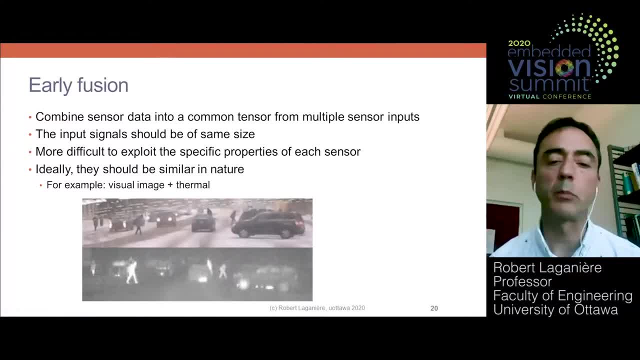 However, this is an expensive sensor and it does not provide any information about the appearance of object, which can make classification and recognition more difficult. However, this is an expensive sensor and it does not provide any information about the appearance of object, which can make classification and recognition more difficult. 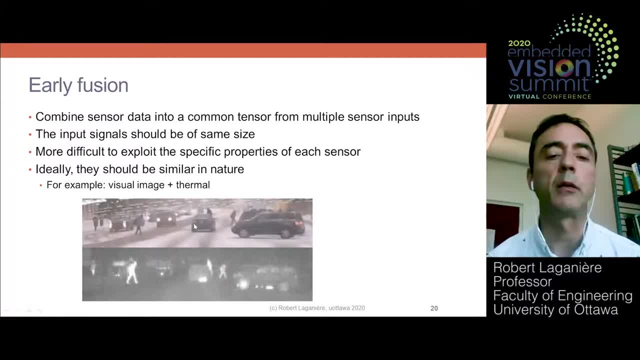 However, this is an expensive sensor and it does not provide any information about the appearance of object, which can make classification and recognition more difficult. However, this is an expensive sensor and it does not provide any information about the appearance of object, which can make classification and recognition more difficult. 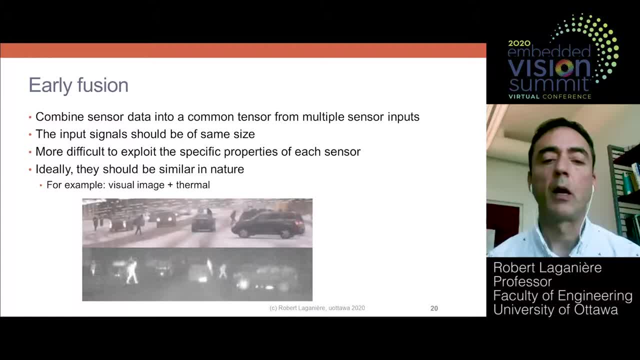 However, this is an expensive sensor and it does not provide any information about the appearance of object, which can make classification and recognition more difficult. However, this is an expensive sensor and it does not provide any information about the appearance of object, which can make classification and recognition more difficult. 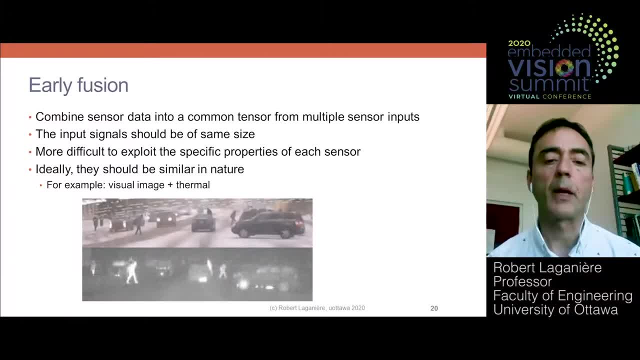 However, this is an expensive sensor and it does not provide any information about the appearance of object, which can make classification and recognition more difficult. However, this is an expensive sensor and it does not provide any information about the appearance of object, which can make classification and recognition more difficult. 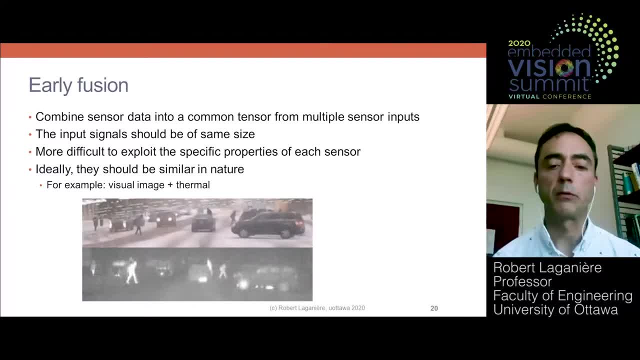 However, this is an expensive sensor and it does not provide any information about the appearance of object, which can make classification and recognition more difficult. However, this is an expensive sensor and it does not provide any information about the appearance of object, which can make classification and recognition more difficult. 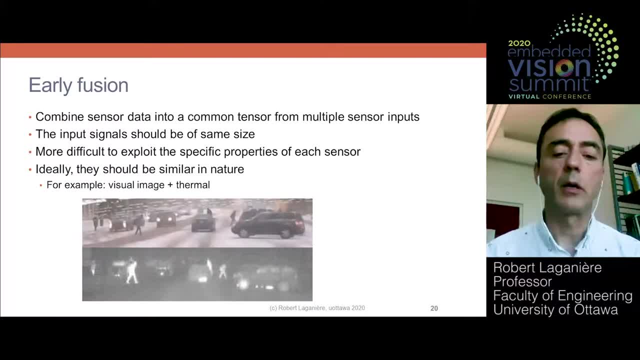 However, this is an expensive sensor and it does not provide any information about the appearance of object, which can make classification and recognition more difficult. However, this is an expensive sensor and it does not provide any information about the appearance of object, which can make classification and recognition more difficult. 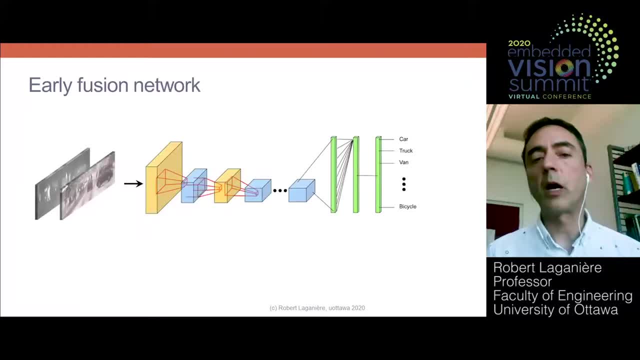 However, this is an expensive sensor and it does not provide any information about the appearance of object, which can make classification and recognition more difficult. However, this is an expensive sensor and it does not provide any information about the appearance of object, which can make classification and recognition more difficult. 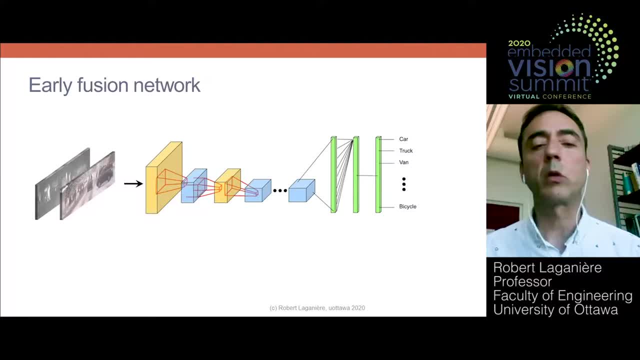 However, this is an expensive sensor and it does not provide any information about the appearance of object, which can make classification and recognition more difficult. However, this is an expensive sensor and it does not provide any information about the appearance of object, which can make classification and recognition more difficult. 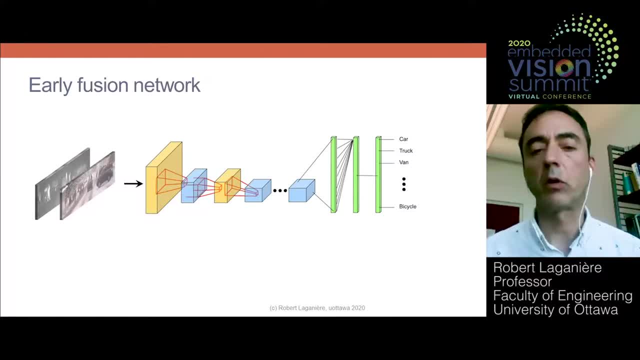 However, this is an expensive sensor and it does not provide any information about the appearance of object, which can make classification and recognition more difficult. However, this is an expensive sensor and it does not provide any information about the appearance of object, which can make classification and recognition more difficult. 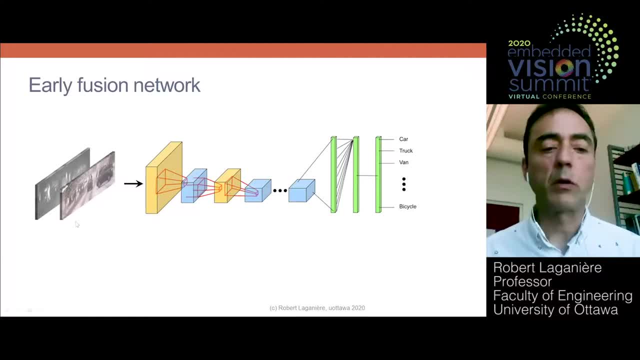 However, this is an expensive sensor and it does not provide any information about the appearance of object, which can make classification and recognition more difficult. However, this is an expensive sensor and it does not provide any information about the appearance of object, which can make classification and recognition more difficult. 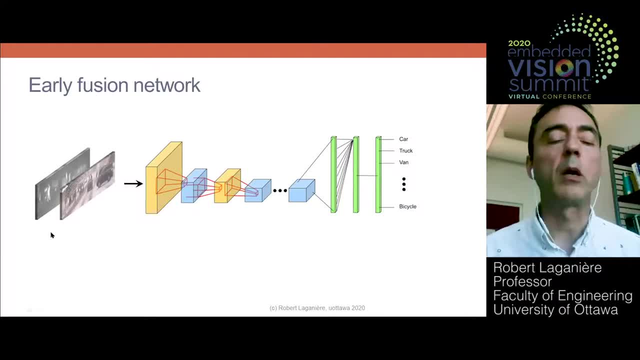 However, this is an expensive sensor and it does not provide any information about the appearance of object, which can make classification and recognition more difficult. However, this is an expensive sensor and it does not provide any information about the appearance of object, which can make classification and recognition more difficult. 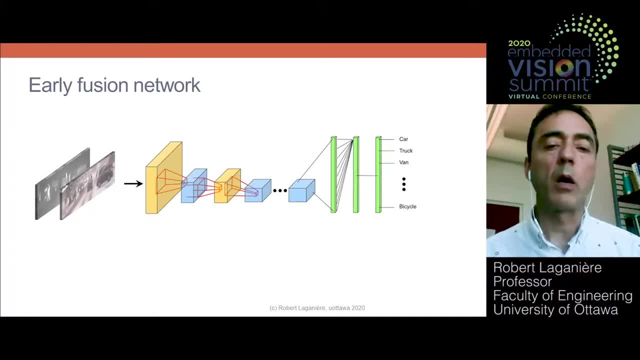 However, this is an expensive sensor and it does not provide any information about the appearance of object, which can make classification and recognition more difficult. However, this is an expensive sensor and it does not provide any information about the appearance of object, which can make classification and recognition more difficult. 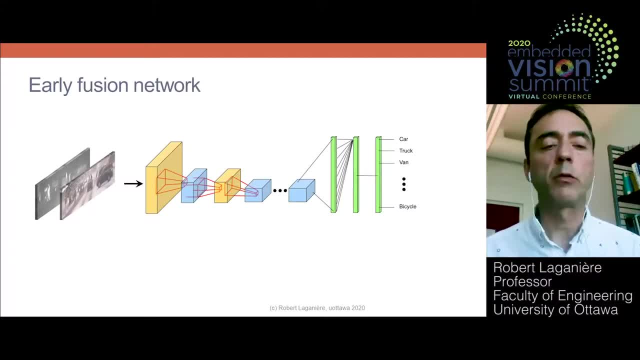 However, this is an expensive sensor and it does not provide any information about the appearance of object, which can make classification and recognition more difficult. However, this is an expensive sensor and it does not provide any information about the appearance of object, which can make classification and recognition more difficult. 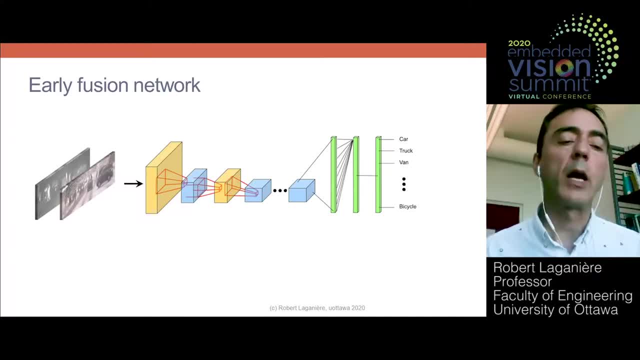 However, this is an expensive sensor and it does not provide any information about the appearance of object, which can make classification and recognition more difficult. However, this is an expensive sensor and it does not provide any information about the appearance of object, which can make classification and recognition more difficult. 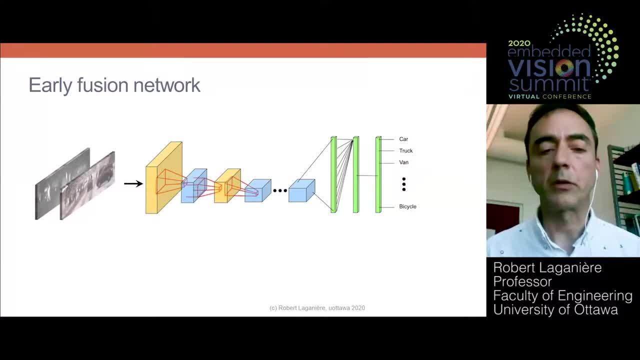 However, this is an expensive sensor and it does not provide any information about the appearance of object, which can make classification and recognition more difficult. However, this is an expensive sensor and it does not provide any information about the appearance of object, which can make classification and recognition more difficult. 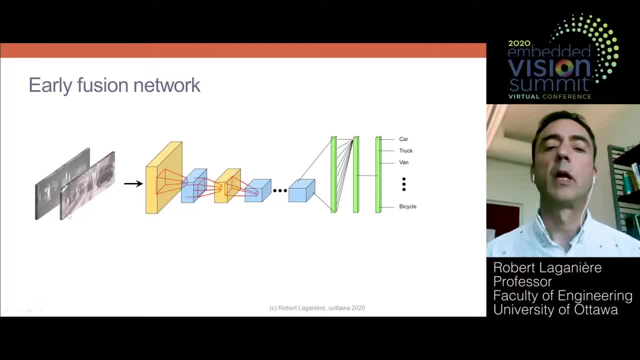 However, this is an expensive sensor and it does not provide any information about the appearance of object, which can make classification and recognition more difficult. However, this is an expensive sensor and it does not provide any information about the appearance of object, which can make classification and recognition more difficult. 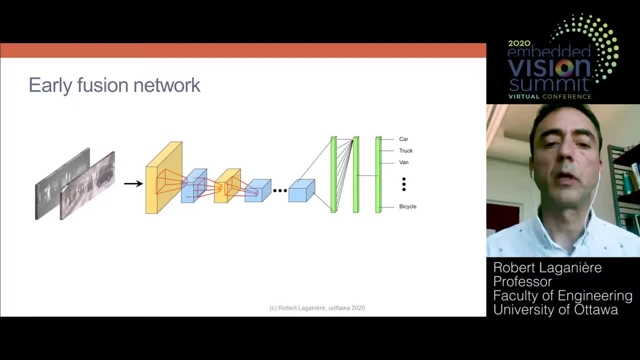 However, this is an expensive sensor and it does not provide any information about the appearance of object, which can make classification and recognition more difficult. However, this is an expensive sensor and it does not provide any information about the appearance of object, which can make classification and recognition more difficult. 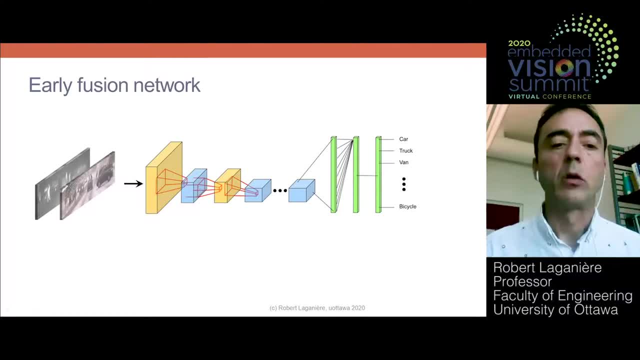 However, this is an expensive sensor and it does not provide any information about the appearance of object, which can make classification and recognition more difficult. However, this is an expensive sensor and it does not provide any information about the appearance of object, which can make classification and recognition more difficult. 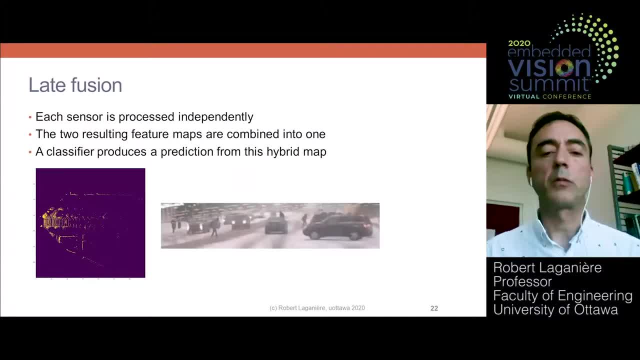 However, this is an expensive sensor and it does not provide any information about the appearance of object, which can make classification and recognition more difficult. However, this is an expensive sensor and it does not provide any information about the appearance of object, which can make classification and recognition more difficult. 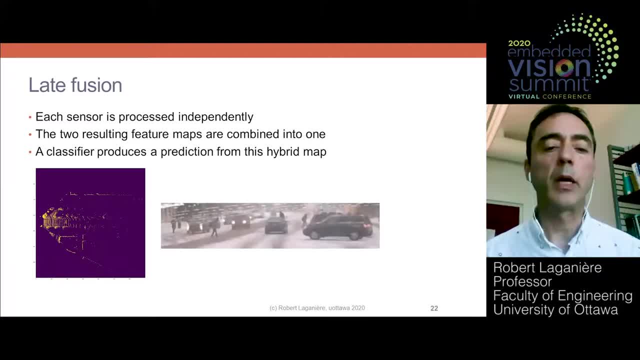 However, this is an expensive sensor and it does not provide any information about the appearance of object, which can make classification and recognition more difficult. However, this is an expensive sensor and it does not provide any information about the appearance of object, which can make classification and recognition more difficult. 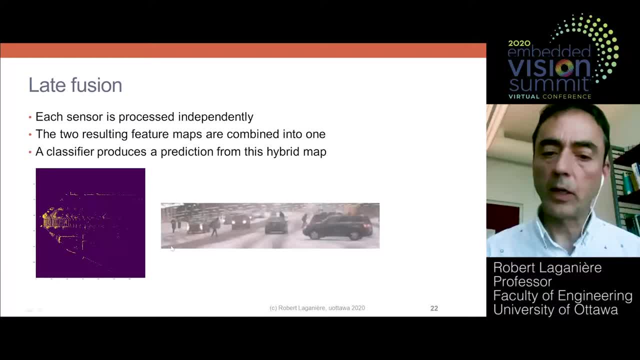 However, this is an expensive sensor and it does not provide any information about the appearance of object, which can make classification and recognition more difficult. However, this is an expensive sensor and it does not provide any information about the appearance of object, which can make classification and recognition more difficult. 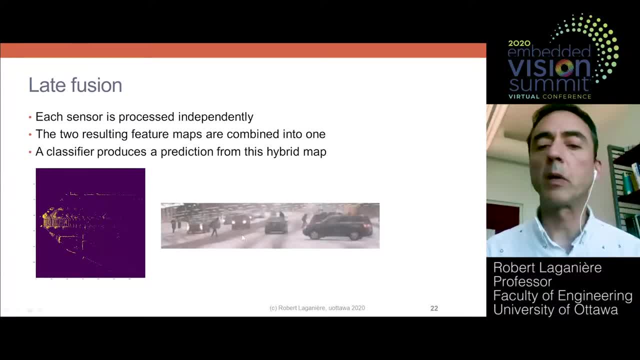 However, this is an expensive sensor and it does not provide any information about the appearance of object, which can make classification and recognition more difficult. However, this is an expensive sensor and it does not provide any information about the appearance of object, which can make classification and recognition more difficult. 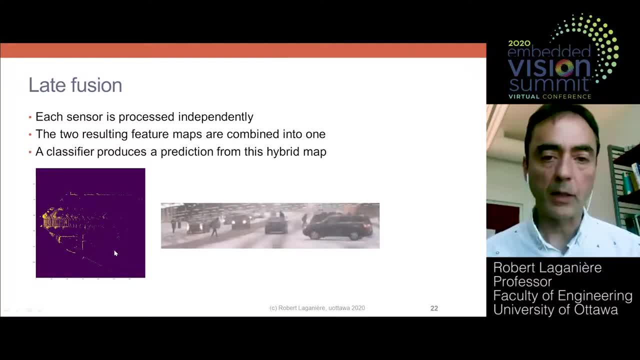 However, this is an expensive sensor and it does not provide any information about the appearance of object, which can make classification and recognition more difficult. However, this is an expensive sensor and it does not provide any information about the appearance of object, which can make classification and recognition more difficult. 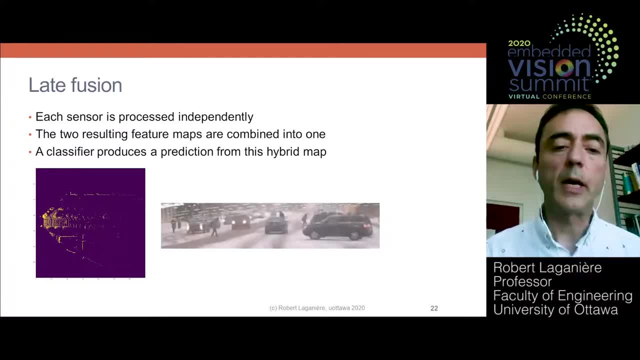 However, this is an expensive sensor and it does not provide any information about the appearance of object, which can make classification and recognition more difficult. However, this is an expensive sensor and it does not provide any information about the appearance of object, which can make classification and recognition more difficult. 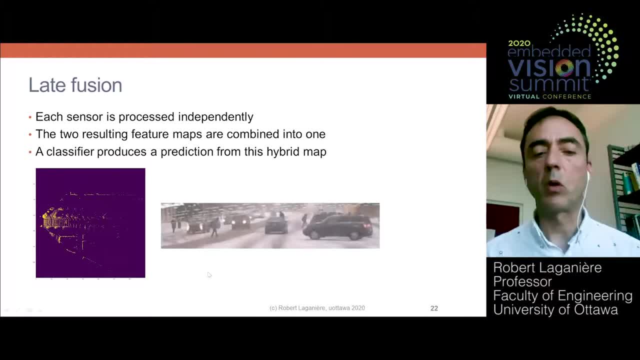 However, this is an expensive sensor and it does not provide any information about the appearance of object, which can make classification and recognition more difficult. However, this is an expensive sensor and it does not provide any information about the appearance of object, which can make classification and recognition more difficult. 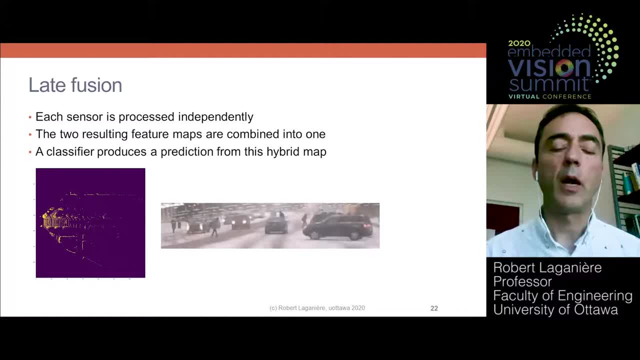 However, this is an expensive sensor and it does not provide any information about the appearance of object, which can make classification and recognition more difficult. However, this is an expensive sensor and it does not provide any information about the appearance of object, which can make classification and recognition more difficult. 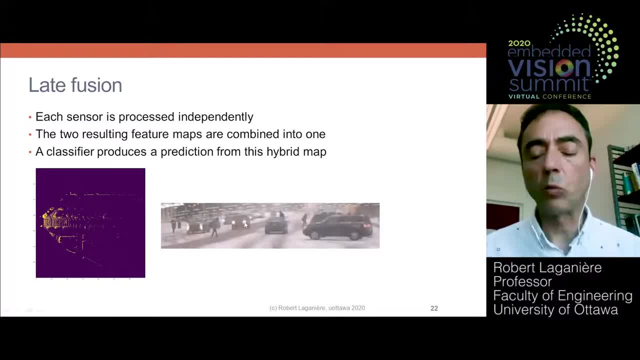 However, this is an expensive sensor and it does not provide any information about the appearance of object, which can make classification and recognition more difficult. However, this is an expensive sensor and it does not provide any information about the appearance of object, which can make classification and recognition more difficult. 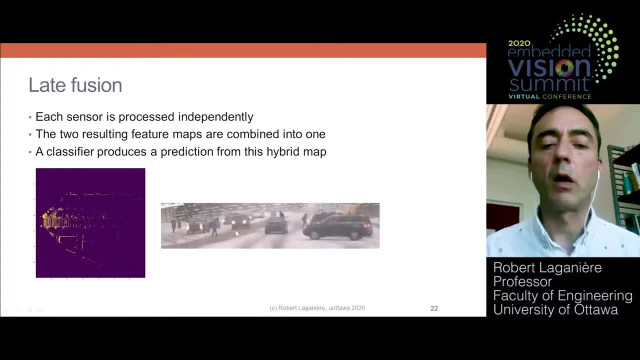 However, this is an expensive sensor and it does not provide any information about the appearance of object, which can make classification and recognition more difficult. However, this is an expensive sensor and it does not provide any information about the appearance of object, which can make classification and recognition more difficult. 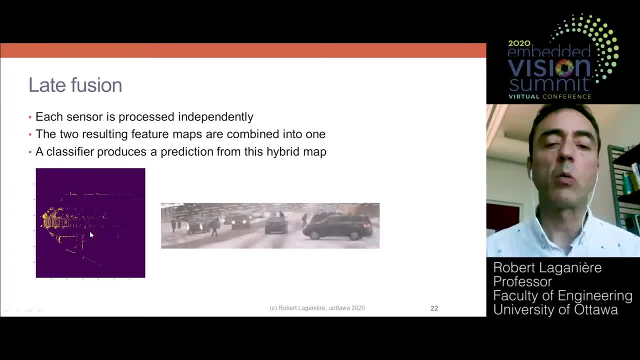 However, this is an expensive sensor and it does not provide any information about the appearance of object, which can make classification and recognition more difficult. However, this is an expensive sensor and it does not provide any information about the appearance of object, which can make classification and recognition more difficult. 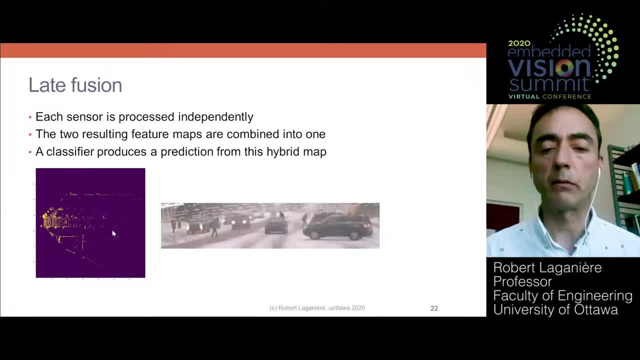 However, this is an expensive sensor and it does not provide any information about the appearance of object, which can make classification and recognition more difficult. However, this is an expensive sensor and it does not provide any information about the appearance of object, which can make classification and recognition more difficult. 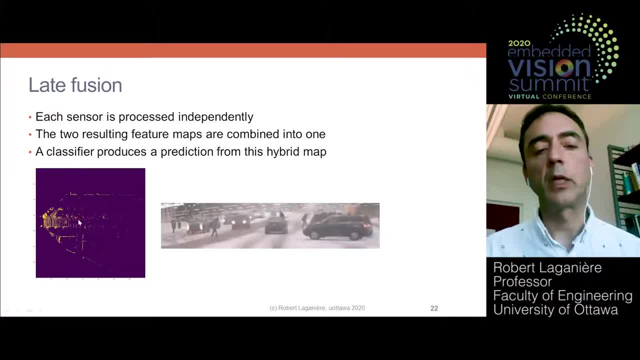 However, this is an expensive sensor and it does not provide any information about the appearance of object, which can make classification and recognition more difficult. However, this is an expensive sensor and it does not provide any information about the appearance of object, which can make classification and recognition more difficult. 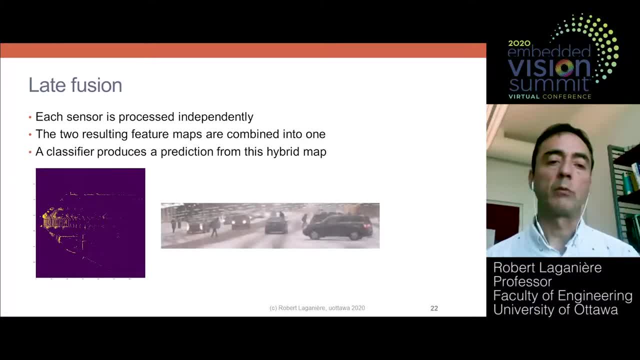 However, this is an expensive sensor and it does not provide any information about the appearance of object, which can make classification and recognition more difficult. However, this is an expensive sensor and it does not provide any information about the appearance of object, which can make classification and recognition more difficult. 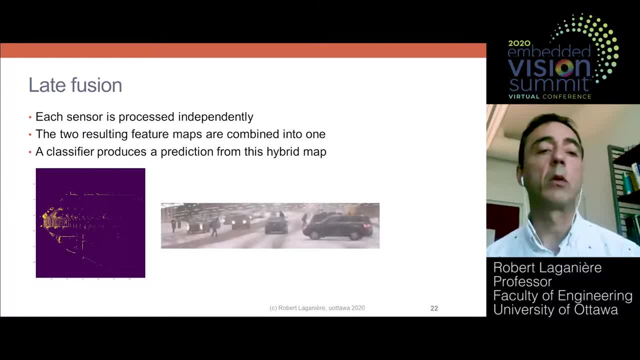 However, this is an expensive sensor and it does not provide any information about the appearance of object, which can make classification and recognition more difficult. However, this is an expensive sensor and it does not provide any information about the appearance of object, which can make classification and recognition more difficult. 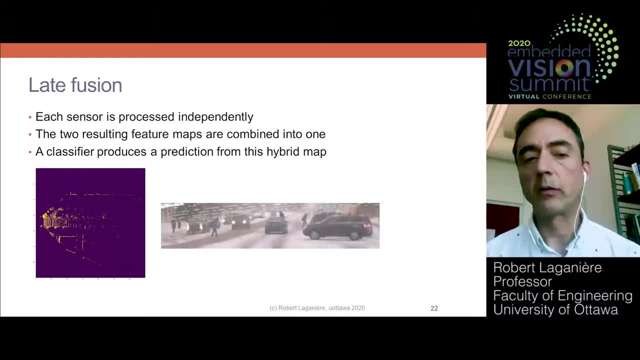 However, this is an expensive sensor and it does not provide any information about the appearance of object, which can make classification and recognition more difficult. However, this is an expensive sensor and it does not provide any information about the appearance of object, which can make classification and recognition more difficult. 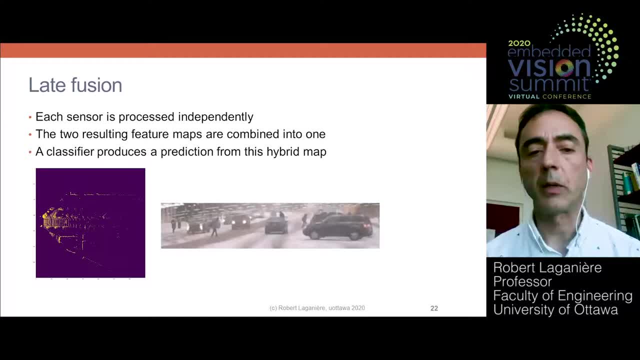 However, this is an expensive sensor and it does not provide any information about the appearance of object, which can make classification and recognition more difficult. However, this is an expensive sensor and it does not provide any information about the appearance of object, which can make classification and recognition more difficult. 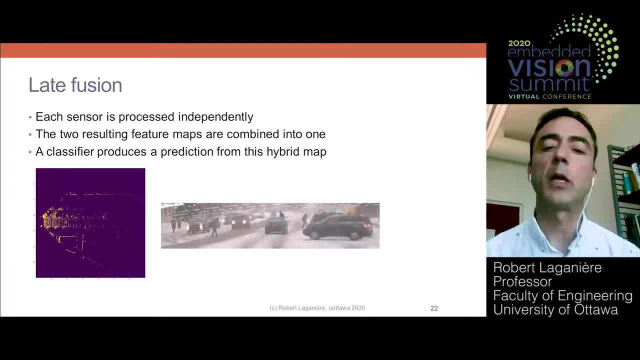 However, this is an expensive sensor and it does not provide any information about the appearance of object, which can make classification and recognition more difficult. However, this is an expensive sensor and it does not provide any information about the appearance of object, which can make classification and recognition more difficult. 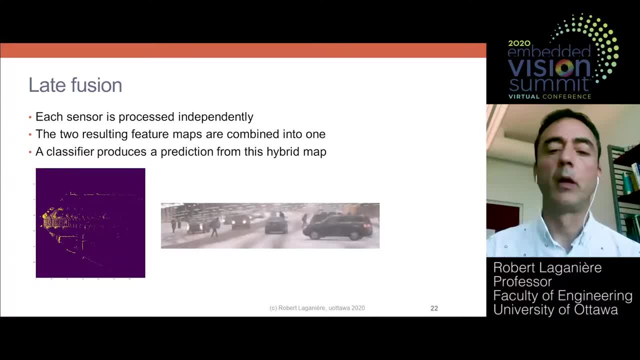 However, this is an expensive sensor and it does not provide any information about the appearance of object, which can make classification and recognition more difficult. However, this is an expensive sensor and it does not provide any information about the appearance of object, which can make classification and recognition more difficult. 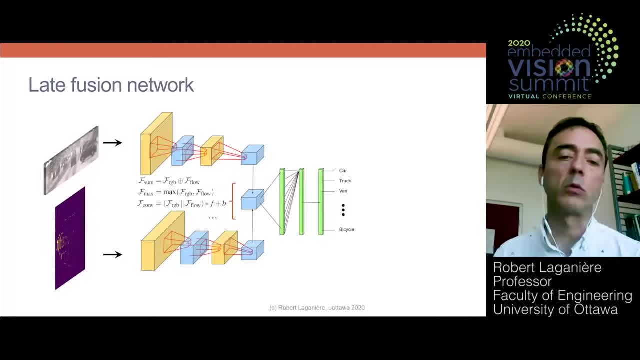 However, this is an expensive sensor and it does not provide any information about the appearance of object, which can make classification and recognition more difficult. However, this is an expensive sensor and it does not provide any information about the appearance of object, which can make classification and recognition more difficult. 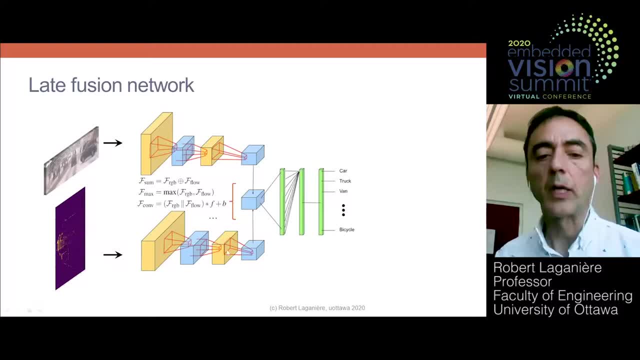 However, this is an expensive sensor and it does not provide any information about the appearance of object, which can make classification and recognition more difficult. However, this is an expensive sensor and it does not provide any information about the appearance of object, which can make classification and recognition more difficult. 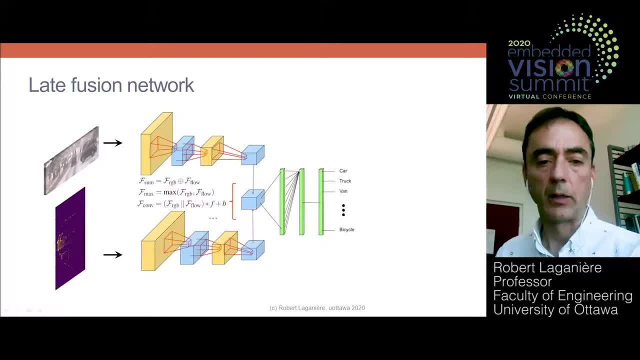 However, this is an expensive sensor and it does not provide any information about the appearance of object, which can make classification and recognition more difficult. However, this is an expensive sensor and it does not provide any information about the appearance of object, which can make classification and recognition more difficult. 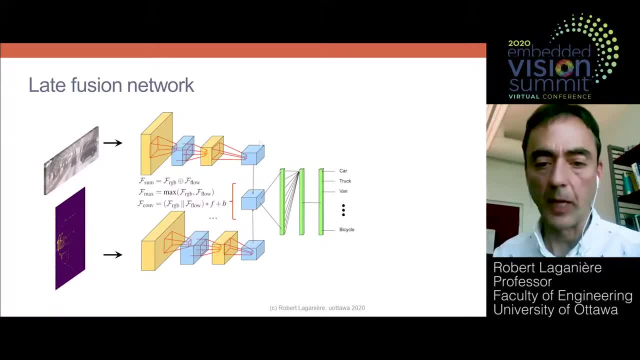 However, this is an expensive sensor and it does not provide any information about the appearance of object, which can make classification and recognition more difficult. However, this is an expensive sensor and it does not provide any information about the appearance of object, which can make classification and recognition more difficult. 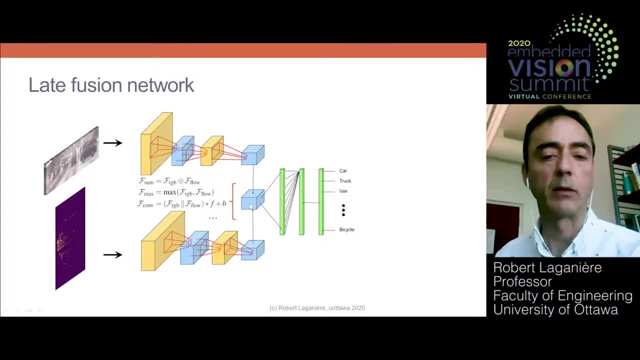 However, this is an expensive sensor and it does not provide any information about the appearance of object, which can make classification and recognition more difficult. However, this is an expensive sensor and it does not provide any information about the appearance of object, which can make classification and recognition more difficult. 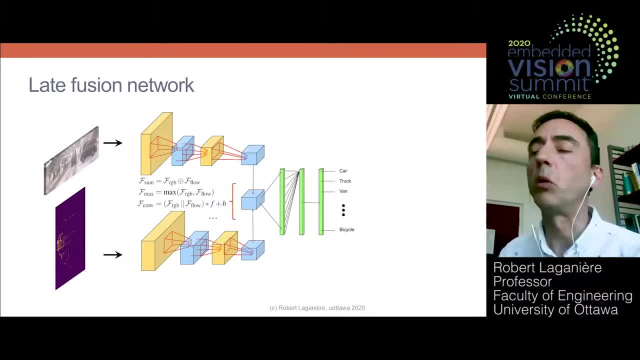 However, this is an expensive sensor and it does not provide any information about the appearance of object, which can make classification and recognition more difficult. However, this is an expensive sensor and it does not provide any information about the appearance of object, which can make classification and recognition more difficult. 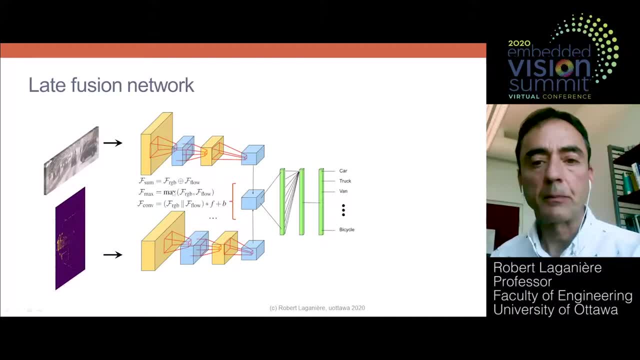 However, this is an expensive sensor and it does not provide any information about the appearance of object, which can make classification and recognition more difficult. However, this is an expensive sensor and it does not provide any information about the appearance of object, which can make classification and recognition more difficult. 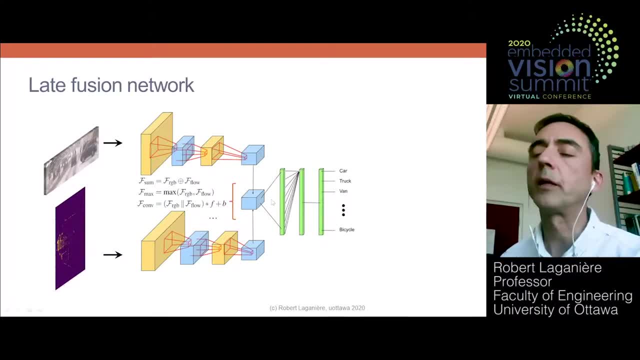 However, this is an expensive sensor and it does not provide any information about the appearance of object, which can make classification and recognition more difficult. However, this is an expensive sensor and it does not provide any information about the appearance of object, which can make classification and recognition more difficult. 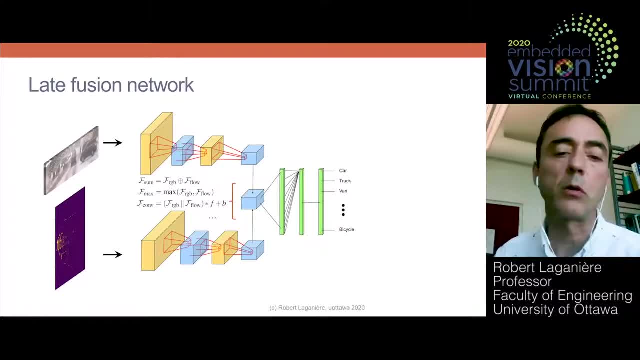 However, this is an expensive sensor and it does not provide any information about the appearance of object, which can make classification and recognition more difficult. However, this is an expensive sensor and it does not provide any information about the appearance of object, which can make classification and recognition more difficult. 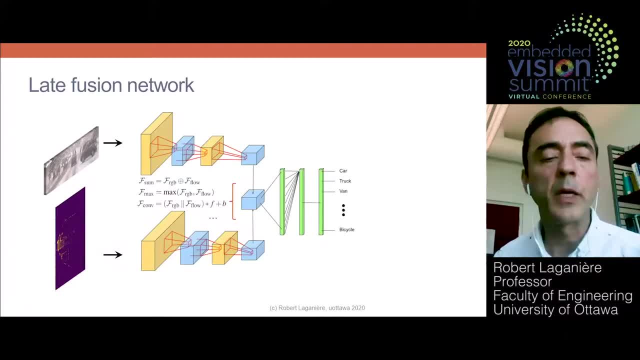 However, this is an expensive sensor and it does not provide any information about the appearance of object, which can make classification and recognition more difficult. However, this is an expensive sensor and it does not provide any information about the appearance of object, which can make classification and recognition more difficult. 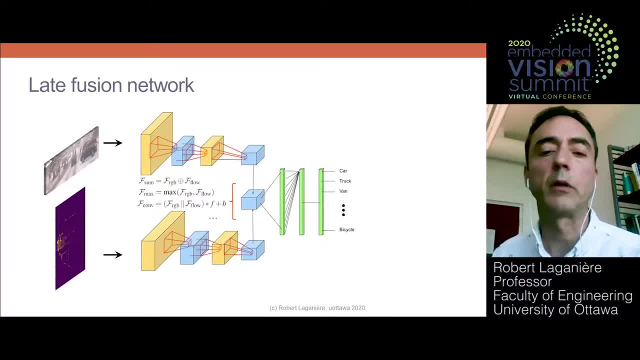 However, this is an expensive sensor and it does not provide any information about the appearance of object, which can make classification and recognition more difficult. However, this is an expensive sensor and it does not provide any information about the appearance of object, which can make classification and recognition more difficult. 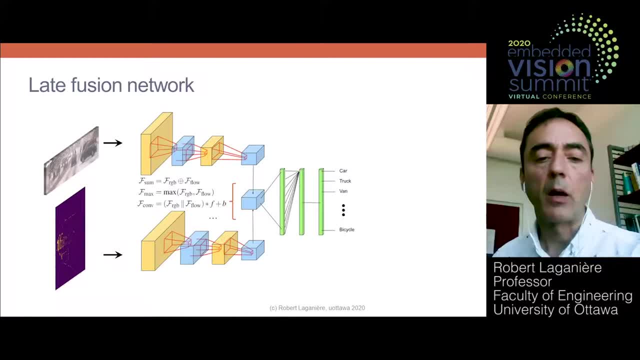 However, this is an expensive sensor and it does not provide any information about the appearance of object, which can make classification and recognition more difficult. However, this is an expensive sensor and it does not provide any information about the appearance of object, which can make classification and recognition more difficult. 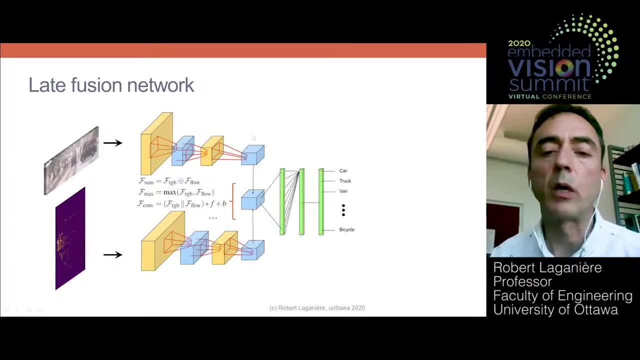 However, this is an expensive sensor and it does not provide any information about the appearance of object, which can make classification and recognition more difficult. However, this is an expensive sensor and it does not provide any information about the appearance of object, which can make classification and recognition more difficult. 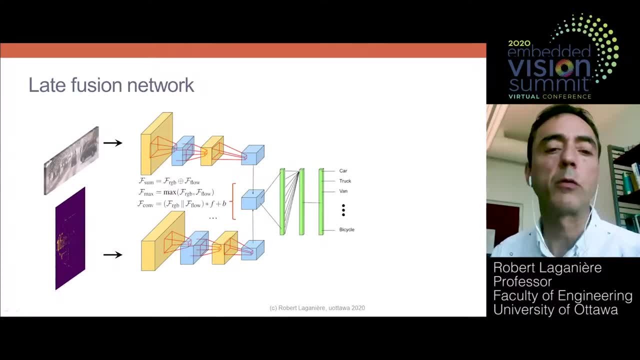 However, this is an expensive sensor and it does not provide any information about the appearance of object, which can make classification and recognition more difficult. However, this is an expensive sensor and it does not provide any information about the appearance of object, which can make classification and recognition more difficult. 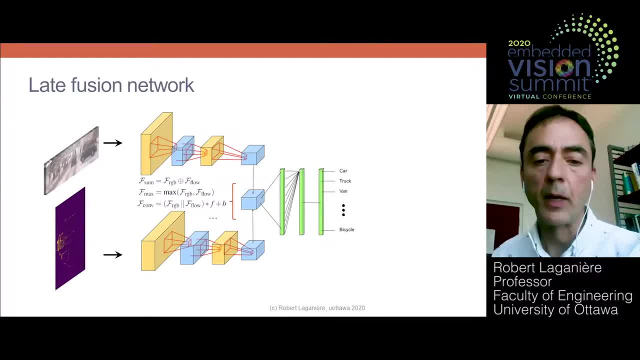 However, this is an expensive sensor and it does not provide any information about the appearance of object, which can make classification and recognition more difficult. However, this is an expensive sensor and it does not provide any information about the appearance of object, which can make classification and recognition more difficult. 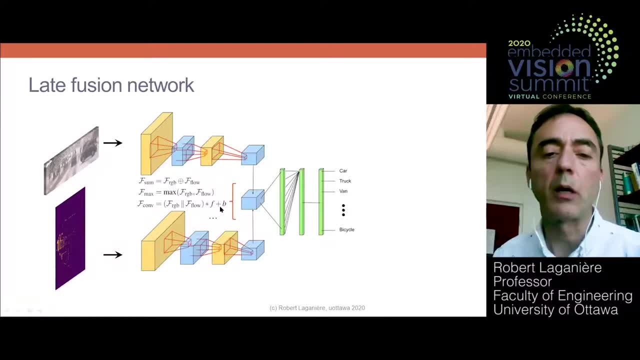 However, this is an expensive sensor and it does not provide any information about the appearance of object, which can make classification and recognition more difficult. However, this is an expensive sensor and it does not provide any information about the appearance of object, which can make classification and recognition more difficult. 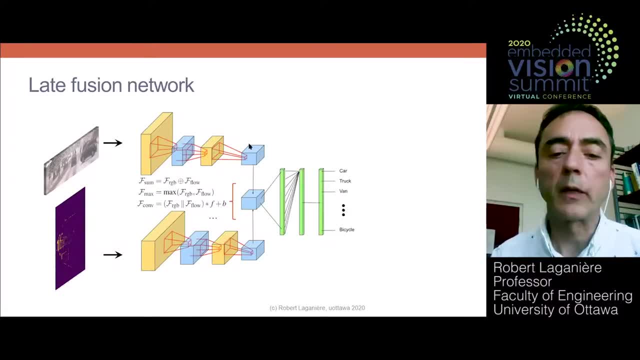 However, this is an expensive sensor and it does not provide any information about the appearance of object, which can make classification and recognition more difficult. However, this is an expensive sensor and it does not provide any information about the appearance of object, which can make classification and recognition more difficult. 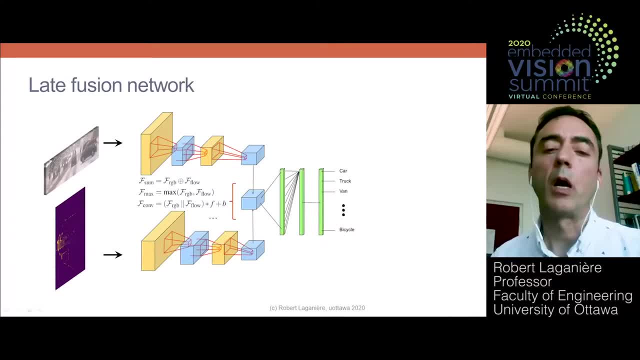 However, this is an expensive sensor and it does not provide any information about the appearance of object, which can make classification and recognition more difficult. However, this is an expensive sensor and it does not provide any information about the appearance of object, which can make classification and recognition more difficult. 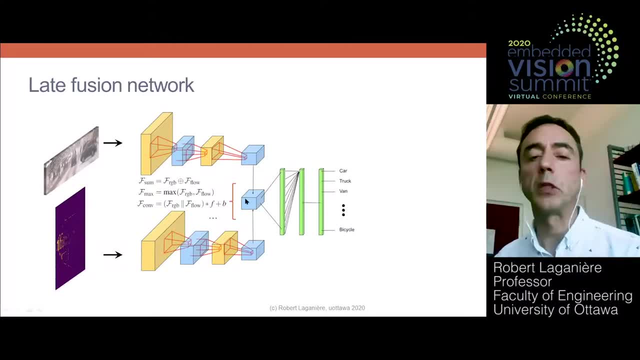 However, this is an expensive sensor and it does not provide any information about the appearance of object, which can make classification and recognition more difficult. However, this is an expensive sensor and it does not provide any information about the appearance of object, which can make classification and recognition more difficult. 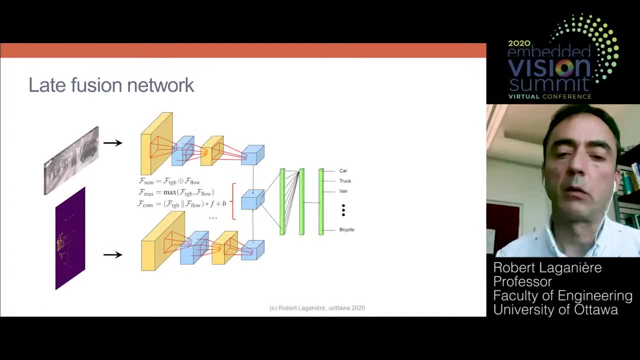 However, this is an expensive sensor and it does not provide any information about the appearance of object, which can make classification and recognition more difficult. However, this is an expensive sensor and it does not provide any information about the appearance of object, which can make classification and recognition more difficult. 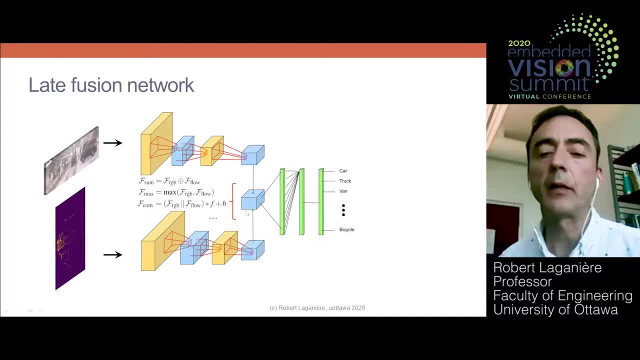 However, this is an expensive sensor and it does not provide any information about the appearance of object, which can make classification and recognition more difficult. However, this is an expensive sensor and it does not provide any information about the appearance of object, which can make classification and recognition more difficult. 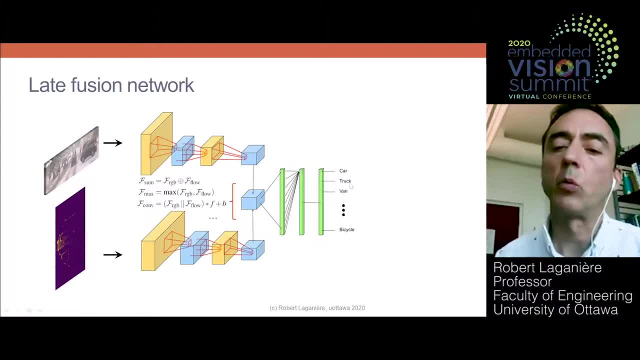 However, this is an expensive sensor and it does not provide any information about the appearance of object, which can make classification and recognition more difficult. However, this is an expensive sensor and it does not provide any information about the appearance of object, which can make classification and recognition more difficult. 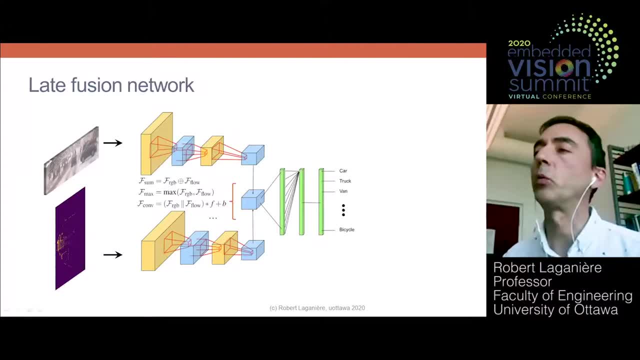 However, this is an expensive sensor and it does not provide any information about the appearance of object, which can make classification and recognition more difficult. However, this is an expensive sensor and it does not provide any information about the appearance of object, which can make classification and recognition more difficult. 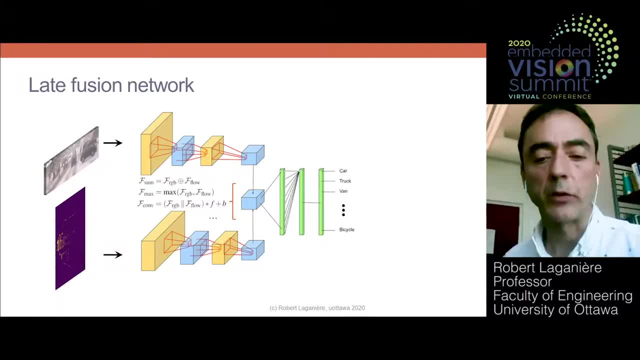 However, this is an expensive sensor and it does not provide any information about the appearance of object, which can make classification and recognition more difficult. However, this is an expensive sensor and it does not provide any information about the appearance of object, which can make classification and recognition more difficult. 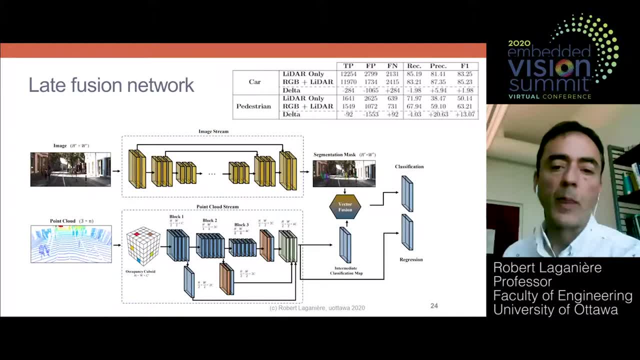 However, this is an expensive sensor and it does not provide any information about the appearance of object, which can make classification and recognition more difficult. However, this is an expensive sensor and it does not provide any information about the appearance of object, which can make classification and recognition more difficult. 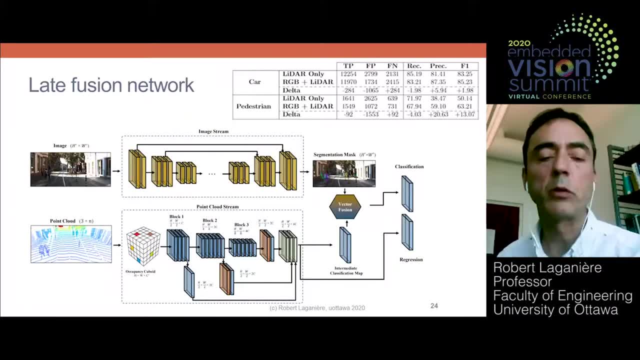 However, this is an expensive sensor and it does not provide any information about the appearance of object, which can make classification and recognition more difficult. However, this is an expensive sensor and it does not provide any information about the appearance of object, which can make classification and recognition more difficult. 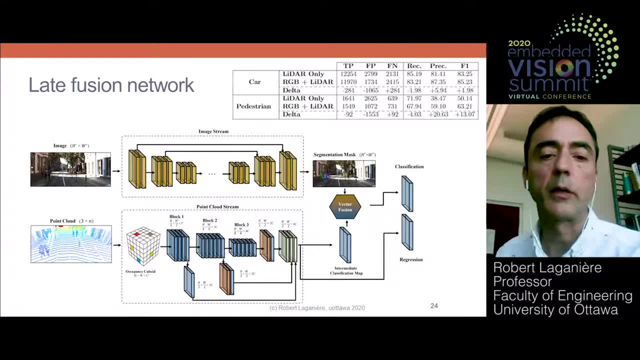 However, this is an expensive sensor and it does not provide any information about the appearance of object, which can make classification and recognition more difficult. However, this is an expensive sensor and it does not provide any information about the appearance of object, which can make classification and recognition more difficult. 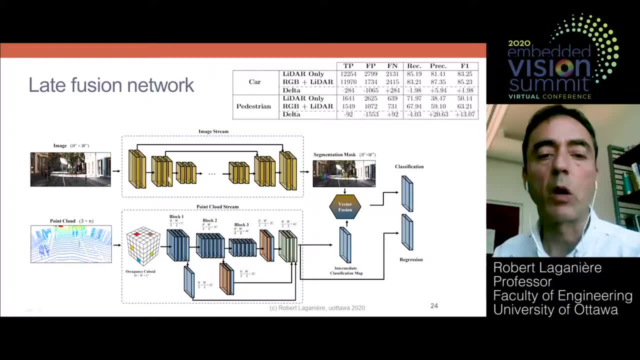 However, this is an expensive sensor and it does not provide any information about the appearance of object, which can make classification and recognition more difficult. However, this is an expensive sensor and it does not provide any information about the appearance of object, which can make classification and recognition more difficult. 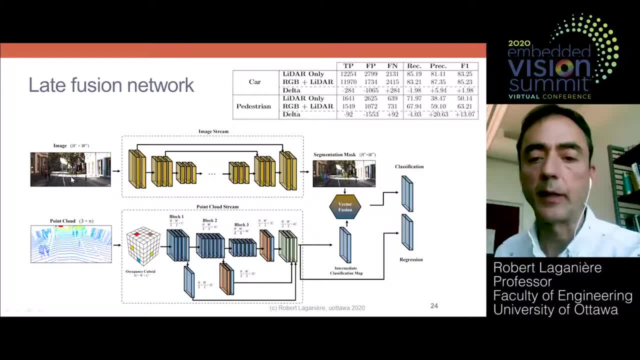 However, this is an expensive sensor and it does not provide any information about the appearance of object, which can make classification and recognition more difficult. However, this is an expensive sensor and it does not provide any information about the appearance of object, which can make classification and recognition more difficult. 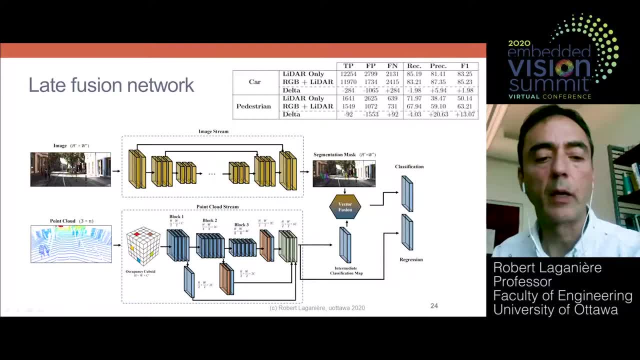 However, this is an expensive sensor and it does not provide any information about the appearance of object, which can make classification and recognition more difficult. However, this is an expensive sensor and it does not provide any information about the appearance of object, which can make classification and recognition more difficult. 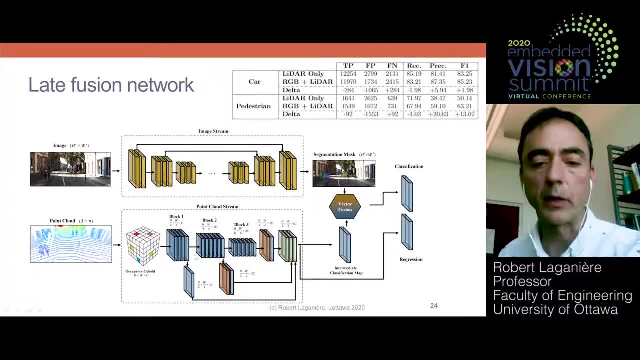 However, this is an expensive sensor and it does not provide any information about the appearance of object, which can make classification and recognition more difficult. However, this is an expensive sensor and it does not provide any information about the appearance of object, which can make classification and recognition more difficult. 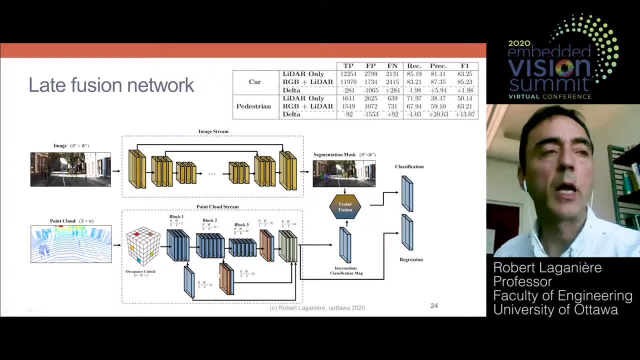 However, this is an expensive sensor and it does not provide any information about the appearance of object, which can make classification and recognition more difficult. However, this is an expensive sensor and it does not provide any information about the appearance of object, which can make classification and recognition more difficult. 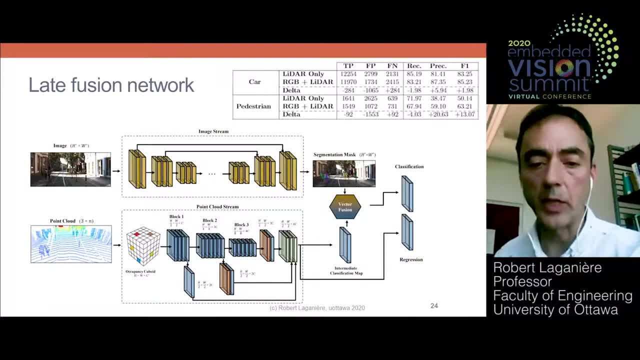 However, this is an expensive sensor and it does not provide any information about the appearance of object, which can make classification and recognition more difficult. However, this is an expensive sensor and it does not provide any information about the appearance of object, which can make classification and recognition more difficult. 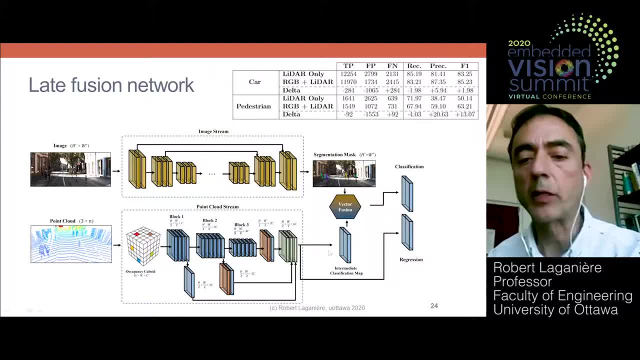 However, this is an expensive sensor and it does not provide any information about the appearance of object, which can make classification and recognition more difficult. However, this is an expensive sensor and it does not provide any information about the appearance of object, which can make classification and recognition more difficult. 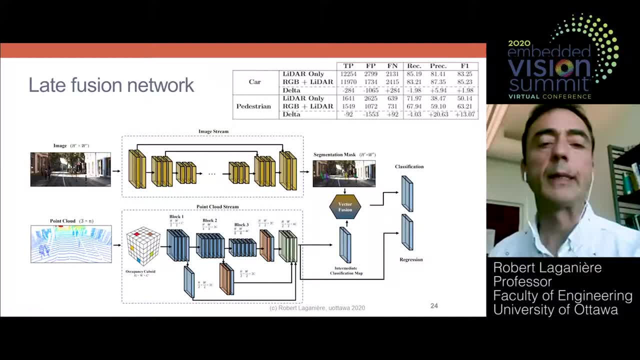 However, this is an expensive sensor and it does not provide any information about the appearance of object, which can make classification and recognition more difficult. However, this is an expensive sensor and it does not provide any information about the appearance of object, which can make classification and recognition more difficult. 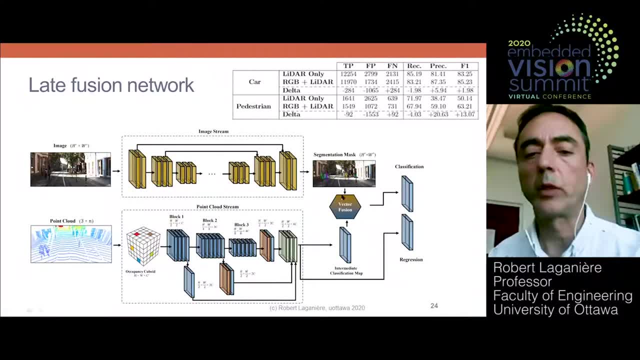 However, this is an expensive sensor and it does not provide any information about the appearance of object, which can make classification and recognition more difficult. However, this is an expensive sensor and it does not provide any information about the appearance of object, which can make classification and recognition more difficult. 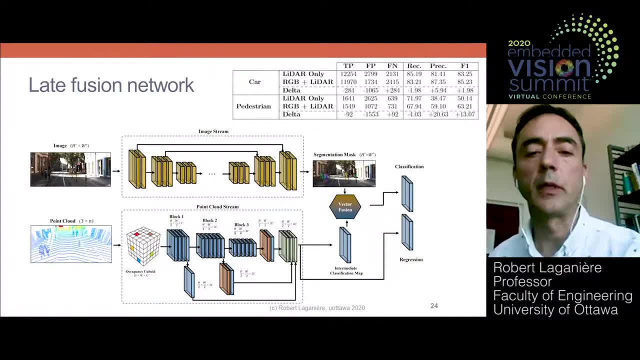 However, this is an expensive sensor and it does not provide any information about the appearance of object, which can make classification and recognition more difficult. However, this is an expensive sensor and it does not provide any information about the appearance of object, which can make classification and recognition more difficult. 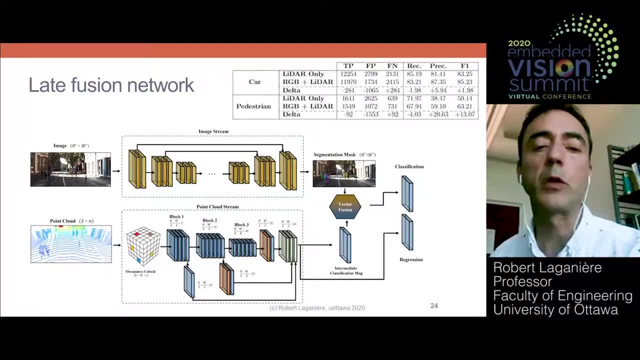 However, this is an expensive sensor and it does not provide any information about the appearance of object, which can make classification and recognition more difficult. However, this is an expensive sensor and it does not provide any information about the appearance of object, which can make classification and recognition more difficult. 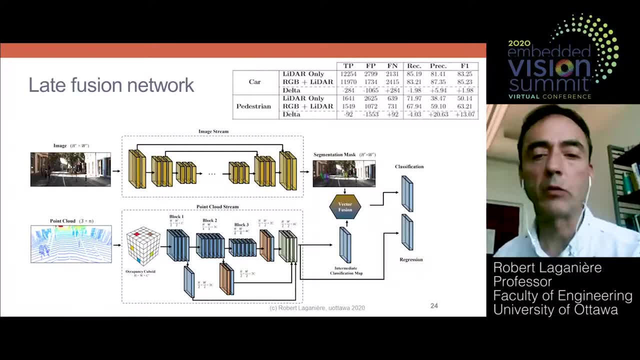 However, this is an expensive sensor and it does not provide any information about the appearance of object, which can make classification and recognition more difficult. However, this is an expensive sensor and it does not provide any information about the appearance of object, which can make classification and recognition more difficult. 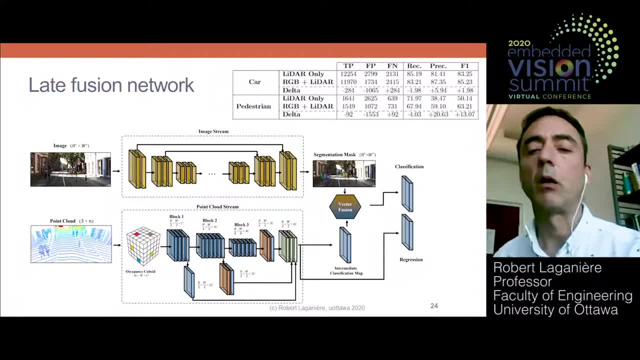 However, this is an expensive sensor and it does not provide any information about the appearance of object, which can make classification and recognition more difficult. However, this is an expensive sensor and it does not provide any information about the appearance of object, which can make classification and recognition more difficult. 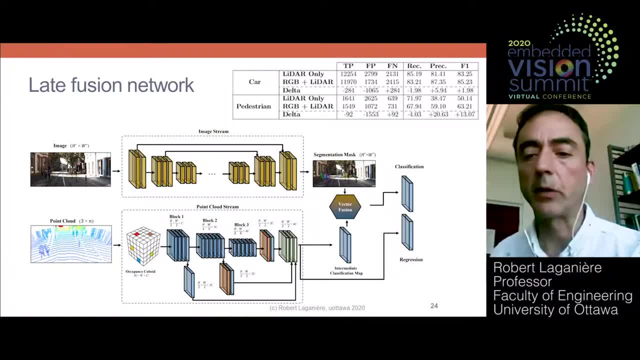 However, this is an expensive sensor and it does not provide any information about the appearance of object, which can make classification and recognition more difficult. However, this is an expensive sensor and it does not provide any information about the appearance of object, which can make classification and recognition more difficult. 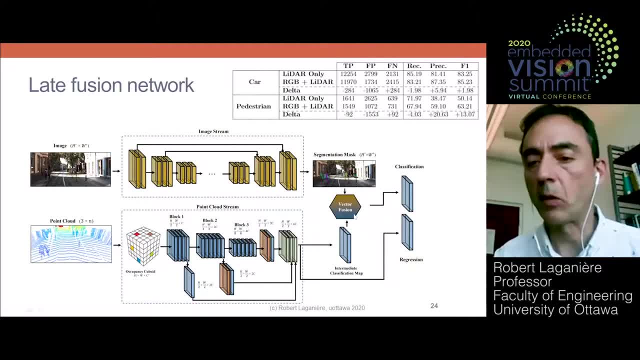 However, this is an expensive sensor and it does not provide any information about the appearance of object, which can make classification and recognition more difficult. However, this is an expensive sensor and it does not provide any information about the appearance of object, which can make classification and recognition more difficult. 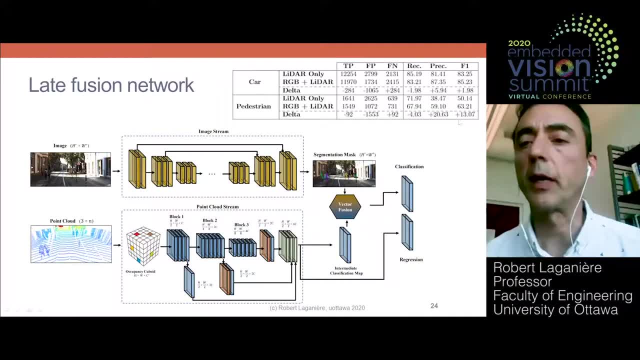 However, this is an expensive sensor and it does not provide any information about the appearance of object, which can make classification and recognition more difficult. However, this is an expensive sensor and it does not provide any information about the appearance of object, which can make classification and recognition more difficult. 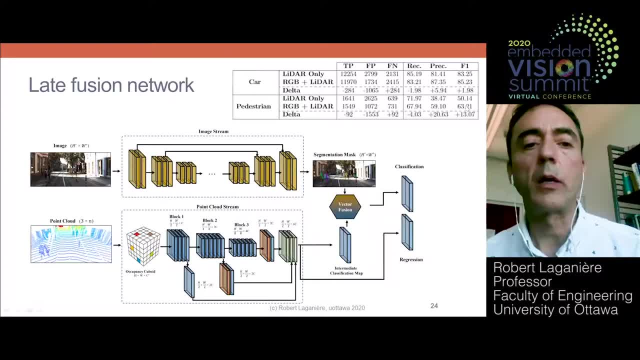 However, this is an expensive sensor and it does not provide any information about the appearance of object, which can make classification and recognition more difficult. However, this is an expensive sensor and it does not provide any information about the appearance of object, which can make classification and recognition more difficult. 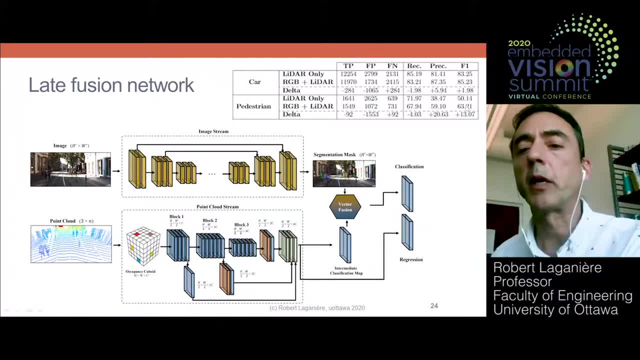 However, this is an expensive sensor and it does not provide any information about the appearance of object, which can make classification and recognition more difficult. However, this is an expensive sensor and it does not provide any information about the appearance of object, which can make classification and recognition more difficult. 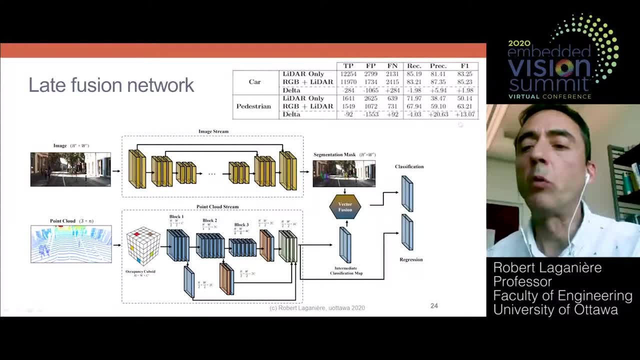 However, this is an expensive sensor and it does not provide any information about the appearance of object, which can make classification and recognition more difficult. However, this is an expensive sensor and it does not provide any information about the appearance of object, which can make classification and recognition more difficult. 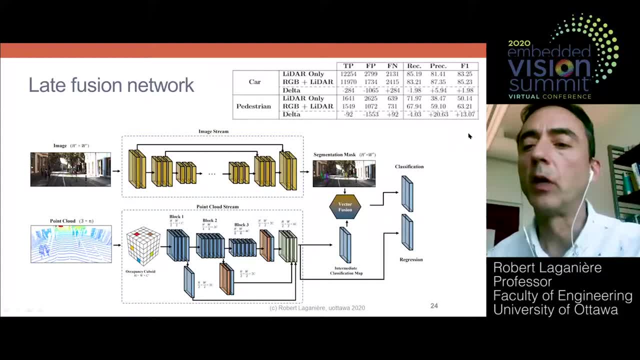 However, this is an expensive sensor and it does not provide any information about the appearance of object, which can make classification and recognition more difficult. However, this is an expensive sensor and it does not provide any information about the appearance of object, which can make classification and recognition more difficult. 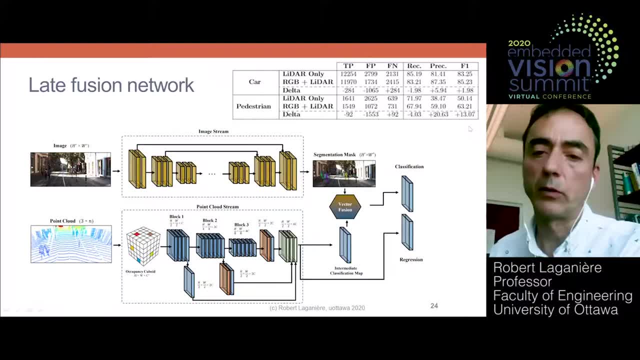 However, this is an expensive sensor and it does not provide any information about the appearance of object, which can make classification and recognition more difficult. However, this is an expensive sensor and it does not provide any information about the appearance of object, which can make classification and recognition more difficult. 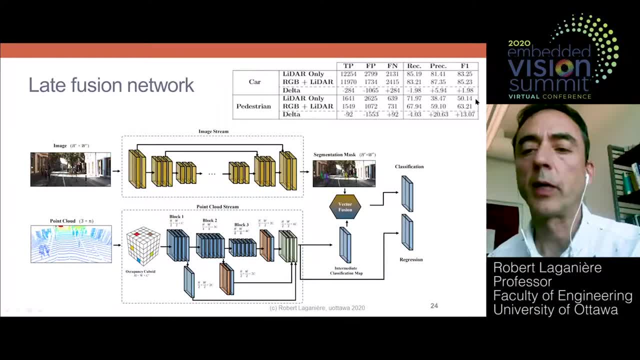 However, this is an expensive sensor and it does not provide any information about the appearance of object, which can make classification and recognition more difficult. However, this is an expensive sensor and it does not provide any information about the appearance of object, which can make classification and recognition more difficult. 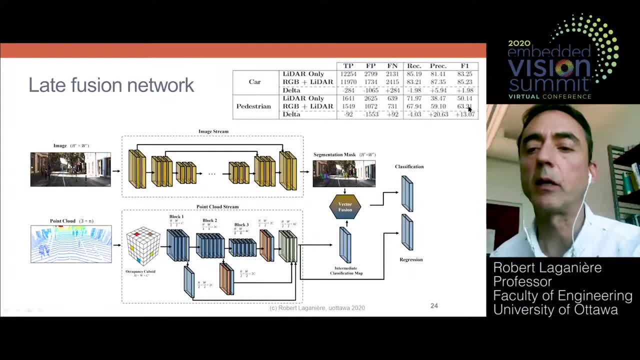 However, this is an expensive sensor and it does not provide any information about the appearance of object, which can make classification and recognition more difficult. However, this is an expensive sensor and it does not provide any information about the appearance of object, which can make classification and recognition more difficult. 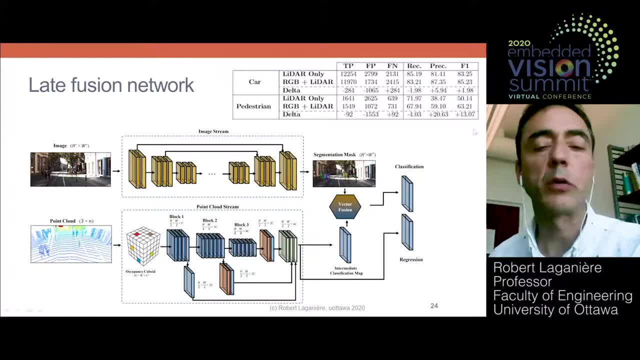 However, this is an expensive sensor and it does not provide any information about the appearance of object, which can make classification and recognition more difficult. However, this is an expensive sensor and it does not provide any information about the appearance of object, which can make classification and recognition more difficult. 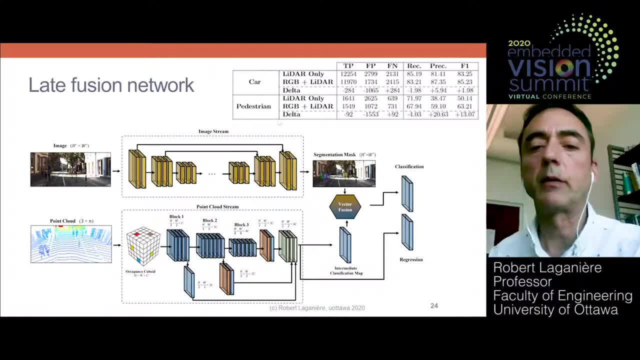 However, this is an expensive sensor and it does not provide any information about the appearance of object, which can make classification and recognition more difficult. However, this is an expensive sensor and it does not provide any information about the appearance of object, which can make classification and recognition more difficult. 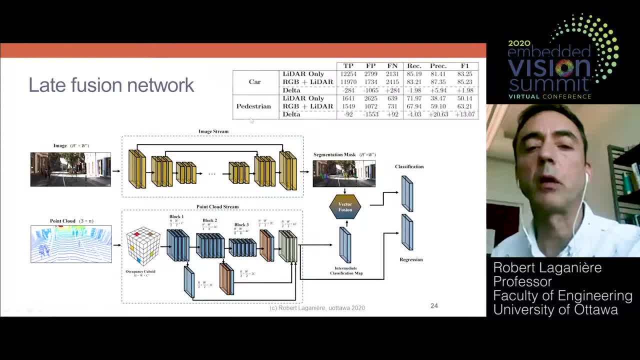 However, this is an expensive sensor and it does not provide any information about the appearance of object, which can make classification and recognition more difficult. However, this is an expensive sensor and it does not provide any information about the appearance of object, which can make classification and recognition more difficult. 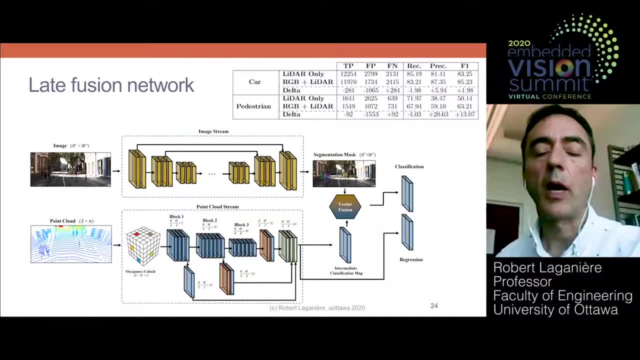 However, this is an expensive sensor and it does not provide any information about the appearance of object, which can make classification and recognition more difficult. However, this is an expensive sensor and it does not provide any information about the appearance of object, which can make classification and recognition more difficult. 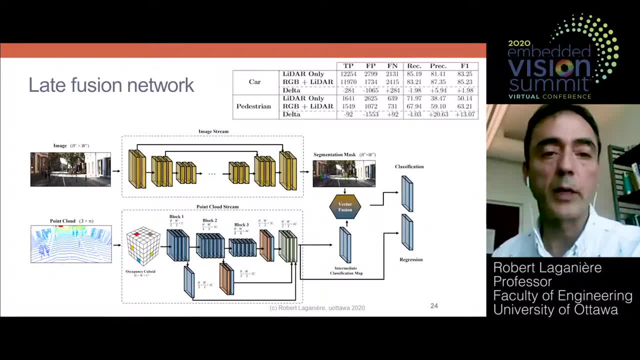 However, this is an expensive sensor and it does not provide any information about the appearance of object, which can make classification and recognition more difficult. However, this is an expensive sensor and it does not provide any information about the appearance of object, which can make classification and recognition more difficult. 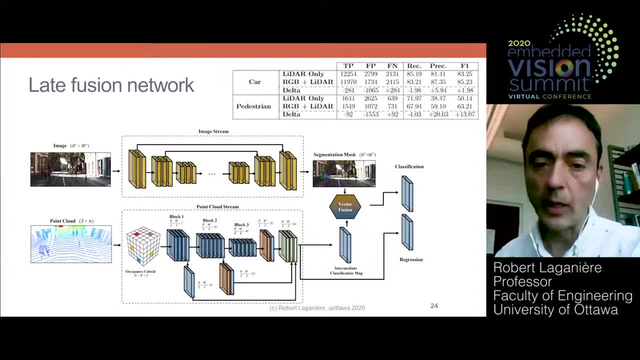 However, this is an expensive sensor and it does not provide any information about the appearance of object, which can make classification and recognition more difficult. However, this is an expensive sensor and it does not provide any information about the appearance of object, which can make classification and recognition more difficult. 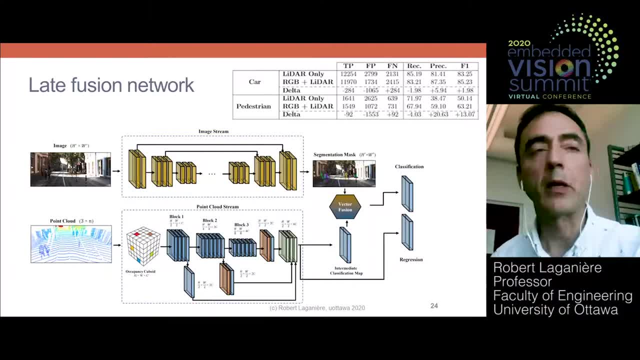 However, this is an expensive sensor and it does not provide any information about the appearance of object, which can make classification and recognition more difficult. However, this is an expensive sensor and it does not provide any information about the appearance of object, which can make classification and recognition more difficult. 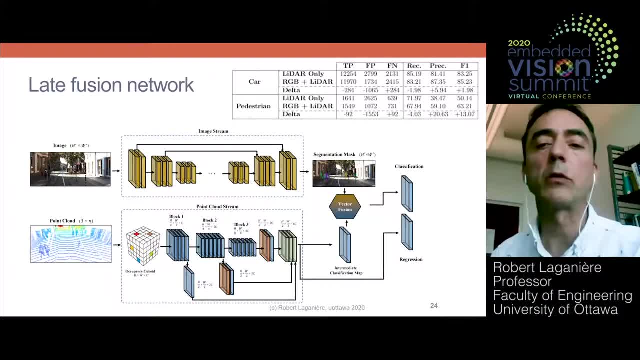 However, this is an expensive sensor and it does not provide any information about the appearance of object, which can make classification and recognition more difficult. However, this is an expensive sensor and it does not provide any information about the appearance of object, which can make classification and recognition more difficult. 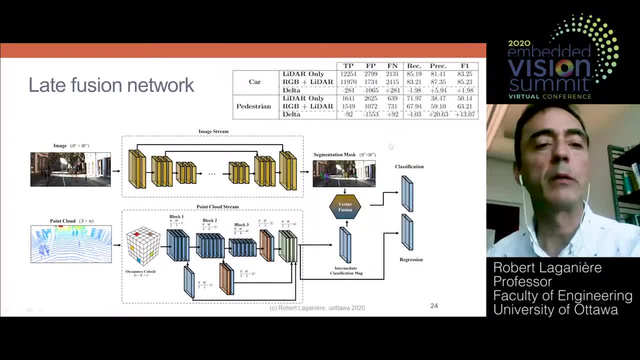 However, this is an expensive sensor and it does not provide any information about the appearance of object, which can make classification and recognition more difficult. However, this is an expensive sensor and it does not provide any information about the appearance of object, which can make classification and recognition more difficult. 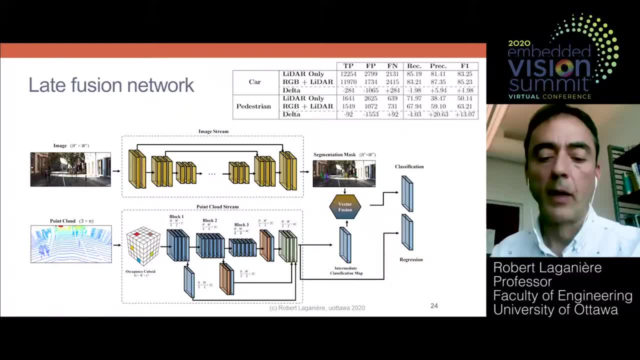 However, this is an expensive sensor and it does not provide any information about the appearance of object, which can make classification and recognition more difficult. However, this is an expensive sensor and it does not provide any information about the appearance of object, which can make classification and recognition more difficult. 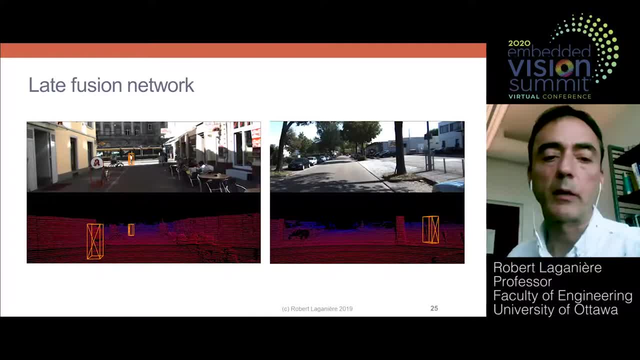 However, this is an expensive sensor and it does not provide any information about the appearance of object, which can make classification and recognition more difficult. However, this is an expensive sensor and it does not provide any information about the appearance of object, which can make classification and recognition more difficult. 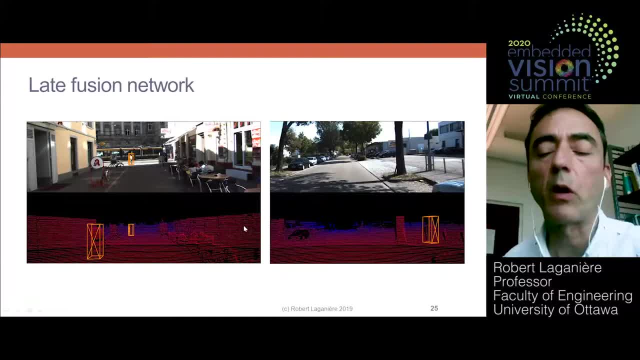 However, this is an expensive sensor and it does not provide any information about the appearance of object, which can make classification and recognition more difficult. However, this is an expensive sensor and it does not provide any information about the appearance of object, which can make classification and recognition more difficult. 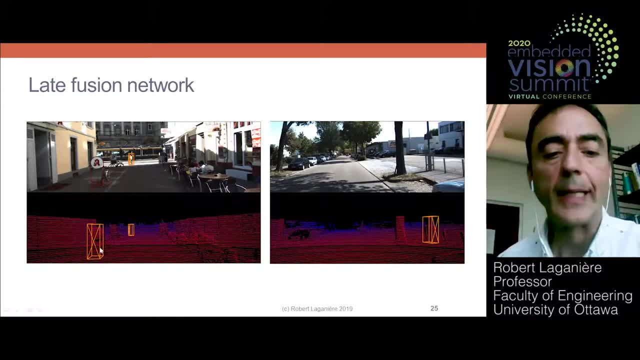 However, this is an expensive sensor and it does not provide any information about the appearance of object, which can make classification and recognition more difficult. However, this is an expensive sensor and it does not provide any information about the appearance of object, which can make classification and recognition more difficult. 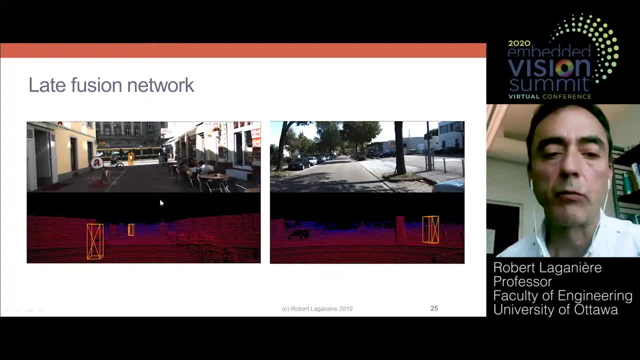 However, this is an expensive sensor and it does not provide any information about the appearance of object, which can make classification and recognition more difficult. However, this is an expensive sensor and it does not provide any information about the appearance of object, which can make classification and recognition more difficult. 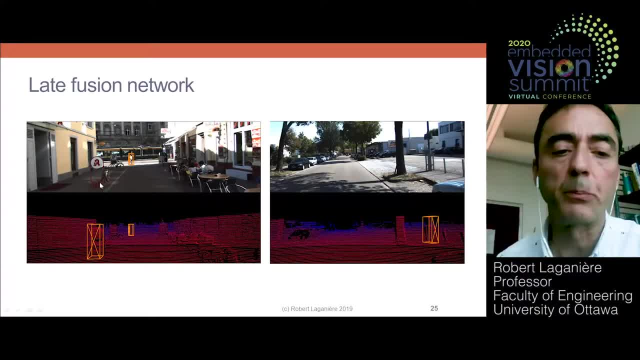 However, this is an expensive sensor and it does not provide any information about the appearance of object, which can make classification and recognition more difficult. However, this is an expensive sensor and it does not provide any information about the appearance of object, which can make classification and recognition more difficult. 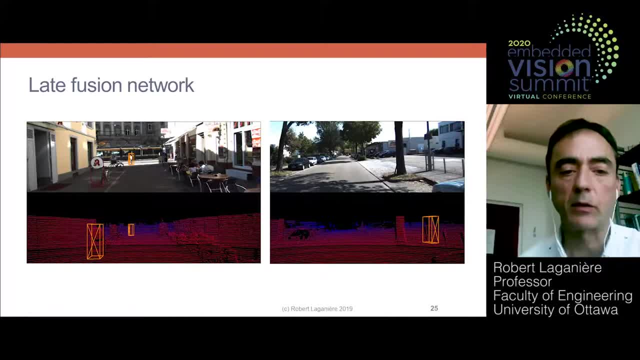 However, this is an expensive sensor and it does not provide any information about the appearance of object, which can make classification and recognition more difficult. However, this is an expensive sensor and it does not provide any information about the appearance of object, which can make classification and recognition more difficult. 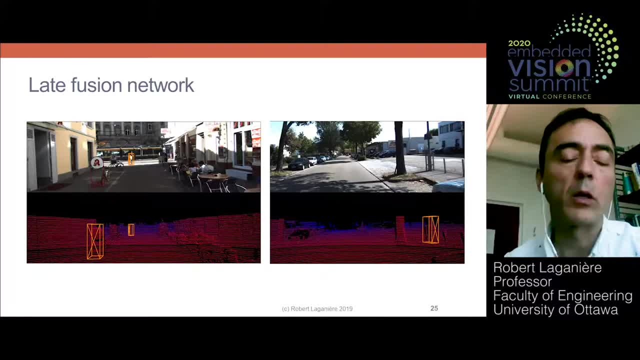 However, this is an expensive sensor and it does not provide any information about the appearance of object, which can make classification and recognition more difficult. However, this is an expensive sensor and it does not provide any information about the appearance of object, which can make classification and recognition more difficult. 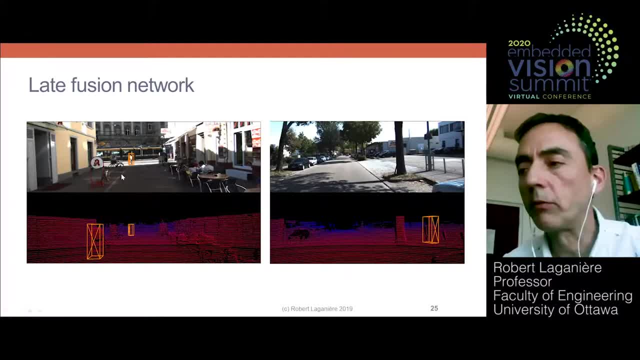 However, this is an expensive sensor and it does not provide any information about the appearance of object, which can make classification and recognition more difficult. However, this is an expensive sensor and it does not provide any information about the appearance of object, which can make classification and recognition more difficult. 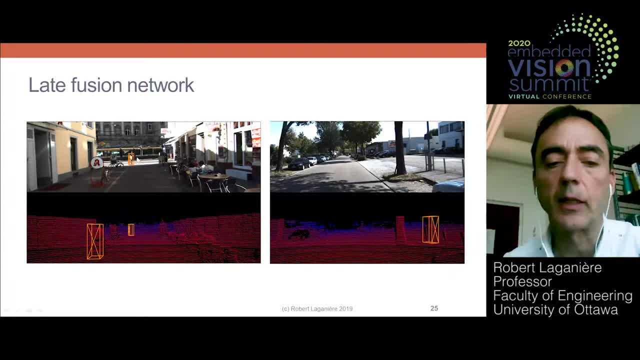 However, this is an expensive sensor and it does not provide any information about the appearance of object, which can make classification and recognition more difficult. However, this is an expensive sensor and it does not provide any information about the appearance of object, which can make classification and recognition more difficult. 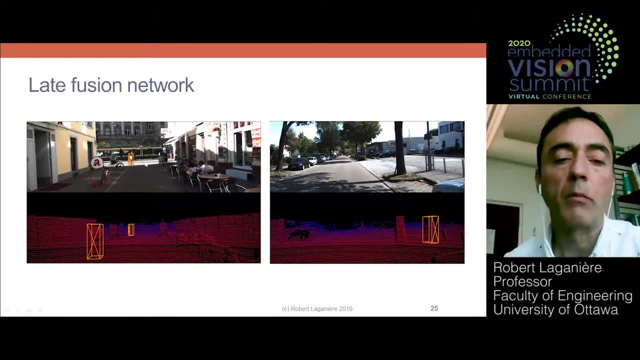 However, this is an expensive sensor and it does not provide any information about the appearance of object, which can make classification and recognition more difficult. However, this is an expensive sensor and it does not provide any information about the appearance of object, which can make classification and recognition more difficult. 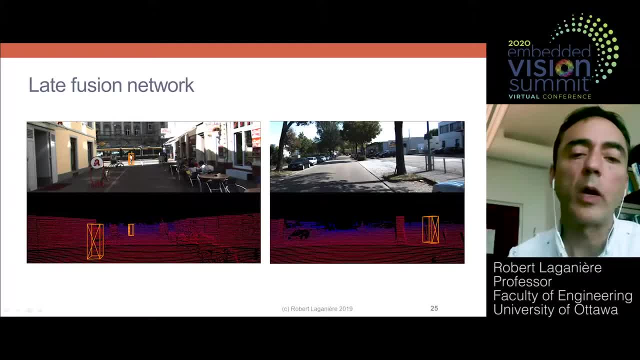 However, this is an expensive sensor and it does not provide any information about the appearance of object, which can make classification and recognition more difficult. However, this is an expensive sensor and it does not provide any information about the appearance of object, which can make classification and recognition more difficult. 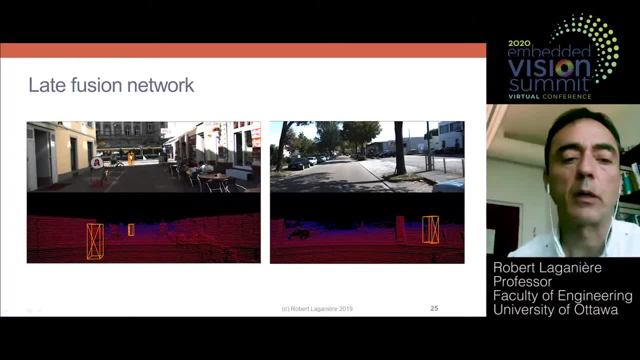 However, this is an expensive sensor and it does not provide any information about the appearance of object, which can make classification and recognition more difficult. However, this is an expensive sensor and it does not provide any information about the appearance of object, which can make classification and recognition more difficult. 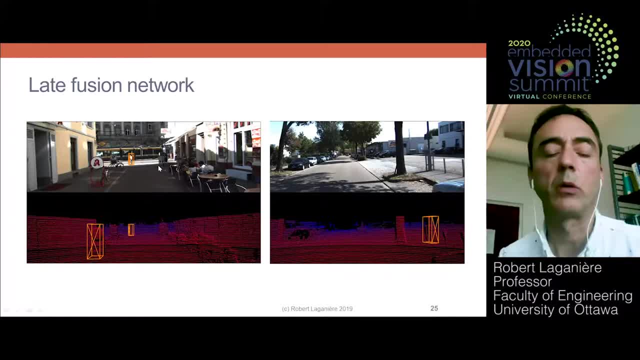 However, this is an expensive sensor and it does not provide any information about the appearance of object, which can make classification and recognition more difficult. However, this is an expensive sensor and it does not provide any information about the appearance of object, which can make classification and recognition more difficult. 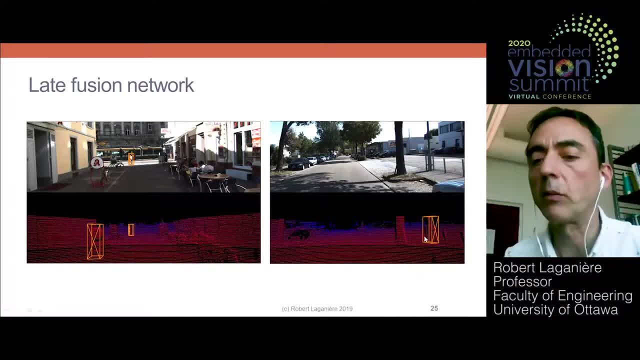 However, this is an expensive sensor and it does not provide any information about the appearance of object, which can make classification and recognition more difficult. However, this is an expensive sensor and it does not provide any information about the appearance of object, which can make classification and recognition more difficult. 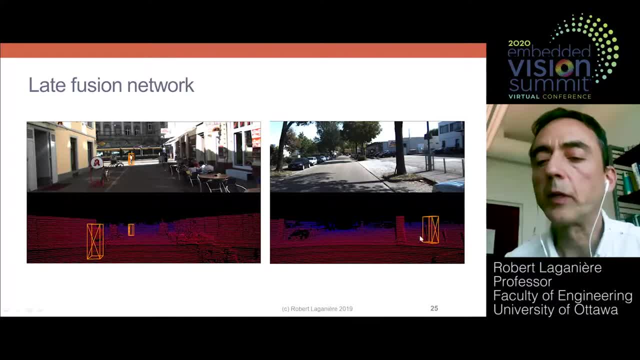 However, this is an expensive sensor and it does not provide any information about the appearance of object, which can make classification and recognition more difficult. However, this is an expensive sensor and it does not provide any information about the appearance of object, which can make classification and recognition more difficult. 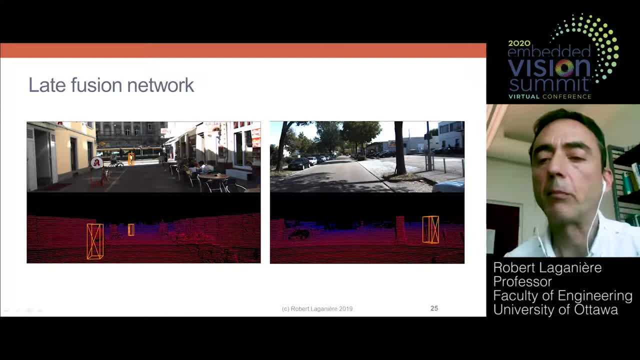 However, this is an expensive sensor and it does not provide any information about the appearance of object, which can make classification and recognition more difficult. However, this is an expensive sensor and it does not provide any information about the appearance of object, which can make classification and recognition more difficult. 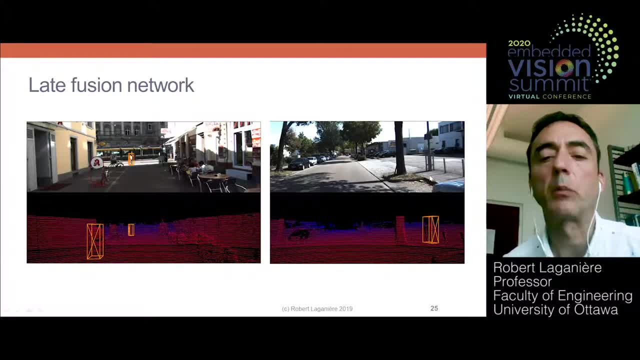 However, this is an expensive sensor and it does not provide any information about the appearance of object, which can make classification and recognition more difficult. However, this is an expensive sensor and it does not provide any information about the appearance of object, which can make classification and recognition more difficult. 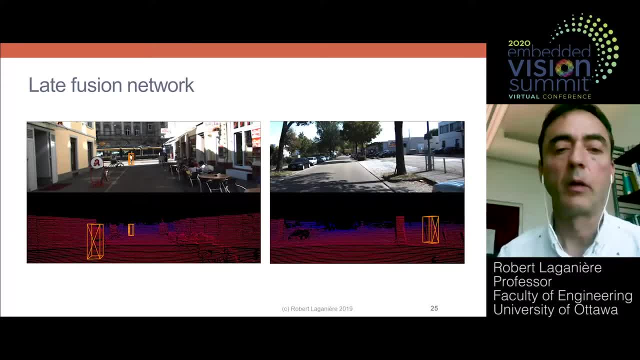 However, this is an expensive sensor and it does not provide any information about the appearance of object, which can make classification and recognition more difficult. However, this is an expensive sensor and it does not provide any information about the appearance of object, which can make classification and recognition more difficult. 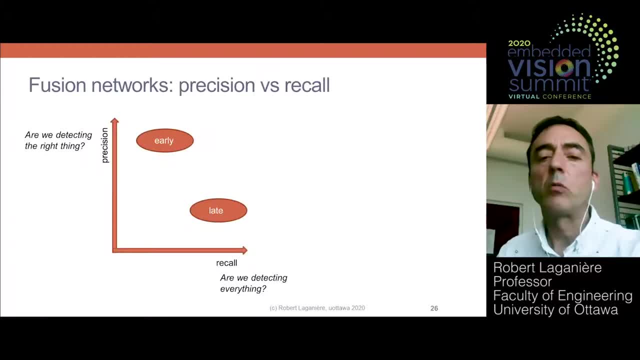 Goodbye, Goodbye, Goodbye, Goodbye, Bye, Goodbye, Goodbye, Goodbye, Bye, Goodbye, Goodbye, Goodbye, Goodbye, Goodbye. really a pedestrian. And the recall metric is: are we detecting everything? 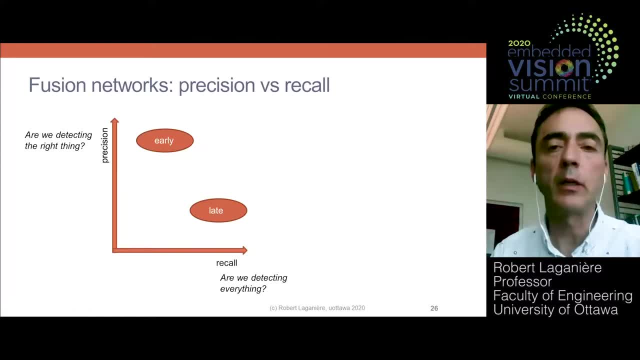 So whenever there is a pedestrian in the scene, are we sure that we will be able to detect it? So whenever you design a detection system, you will get either very high precision, but maybe a lower recall, or the opposite, a very high recall. 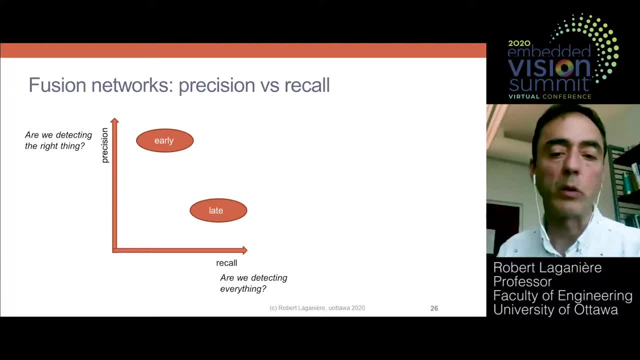 and a lower precision, And it's very difficult to get both. And if you look at the fusion strategy, usually the early fusion strategy will get high precision because you're processing a very rich sensor that is made of the concatenation of the information from many different sensors. 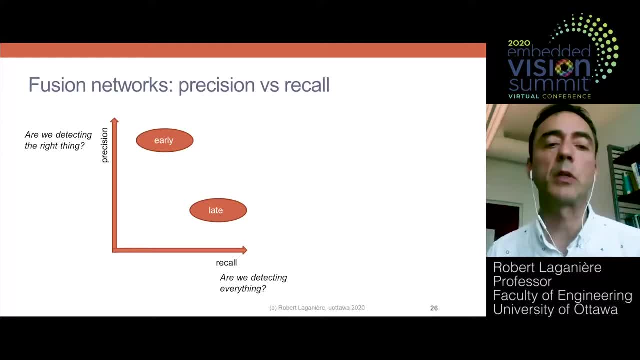 So from that information, whenever you detect something, you're pretty sure that you detect the right thing, While if you're using a late fusion approach, very often you will get a high recall because you independently detect object from the different sensors. So whenever there is something you 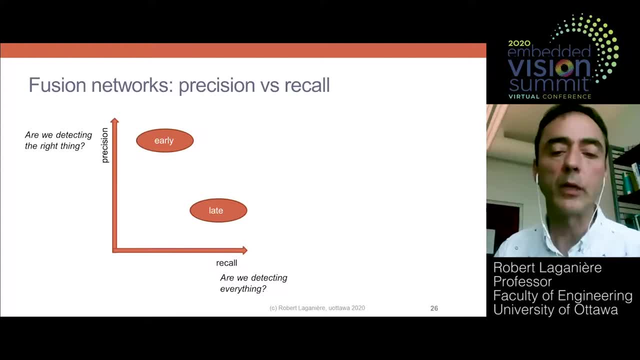 have a good chance that one of the sensor will be able to see it. So that way you will get a very high recall. But because you process each sensor independently, you might not- You might not always be as accurate as you wish. 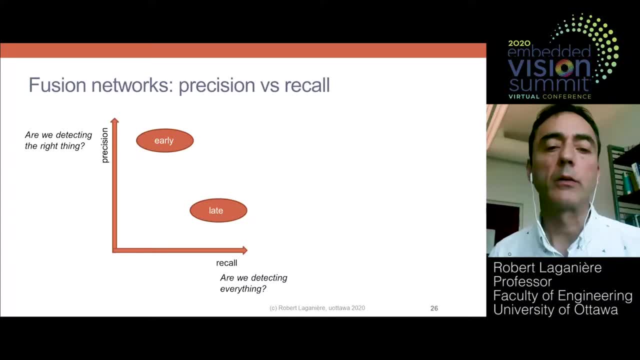 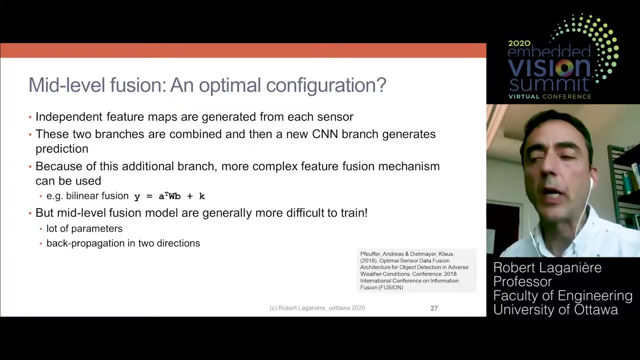 But this is just a very general statement. But that's more or less what you could expect from these two different sensor fusion strategies. Now let's have a look at the third approach, which is the mid-level fusion, which could be, in a sense, considered. 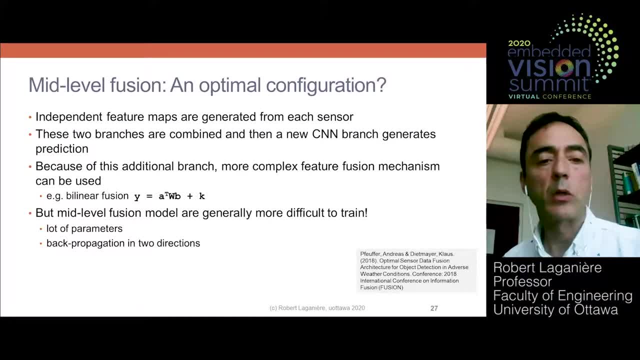 as the most optimal configuration. Indeed, what you will do in that case. you will first build feature map from each of the sensors, So you will have two branches, or the number of branches corresponding to the number of sensor you use, And so these branches will create. 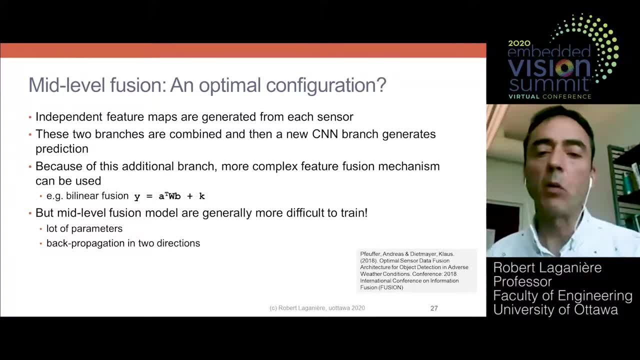 intermediate representation that will then be combined at the mid-level of the network And a new branch will then process that combined system signal in order to generate, at the end, a prediction about the detected object. So, because you have now to combine a more complex representation, very often you will, you will. 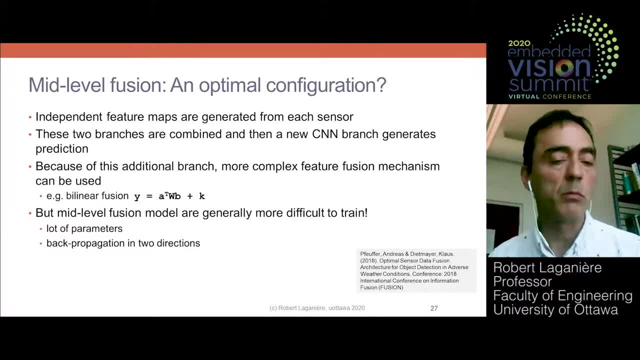 you will want to use a more complex fusion mechanism. Mid-level fusion is such a representation that is more complex, a strategy that is more complex in order to combine your system, But you can also use more basic one. I invite you to look at the reference there in order. 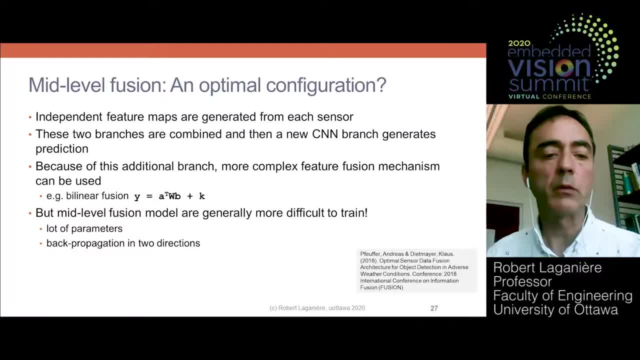 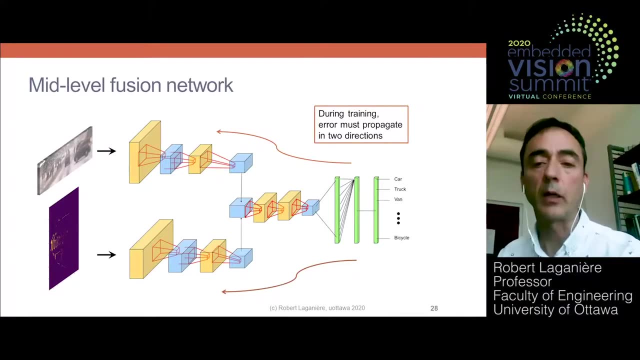 to learn more about these, Thank you. So this is the most optimal approach, But it turns out that mid-level representation, mid-level fusion network are much more difficult to train, And this can be explained by the following illustration. Basically, as I told you when you, 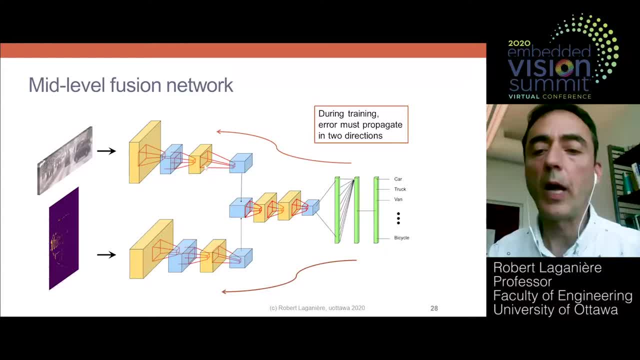 will have to train this system you will have, whenever the end results, the result detection, is wrong, you will have to propagate the error from the top of the network to the lower layers in order to adjust the weight for the network to converge to a network of higher accuracy. 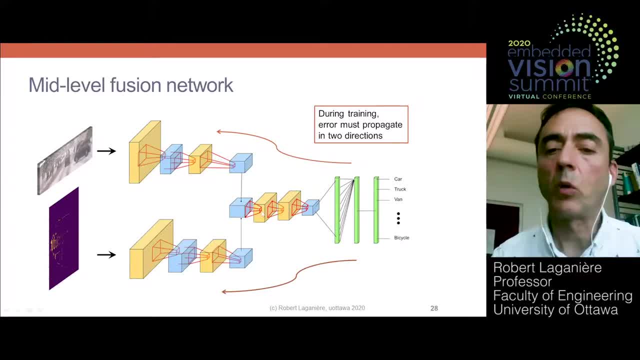 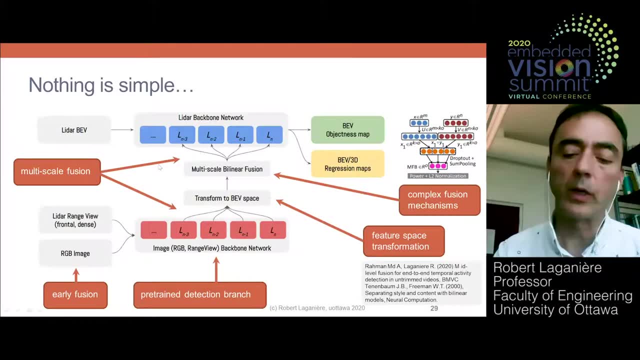 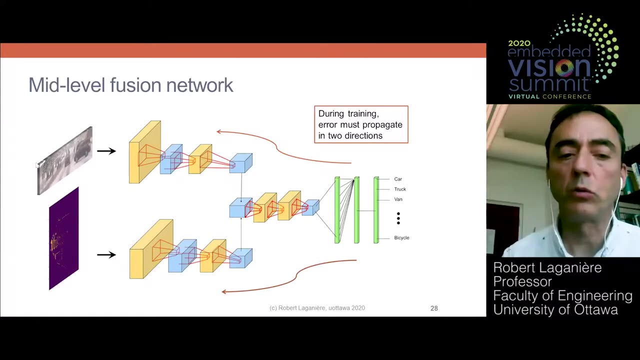 However, when you have two branches like that and you have to propagate the error at the point of intersection, when you perform your propagation, you won't know exactly where you should go. And is the error due to the camera branch Or is it, in that case, due to the LiDAR branch? 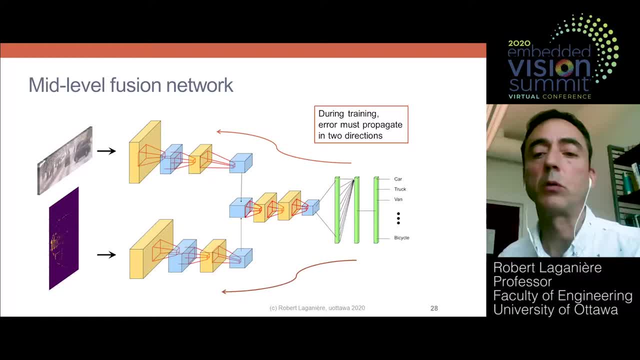 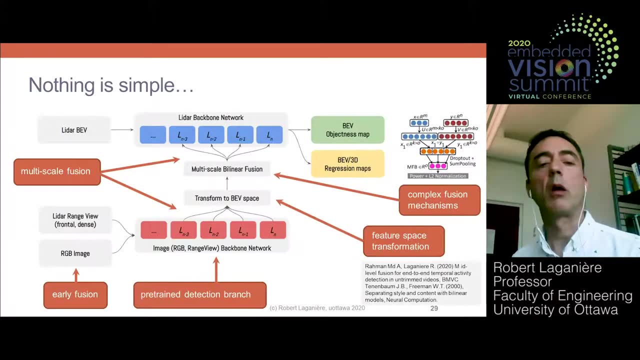 So for this reason it is much more difficult to correctly train your network. So in practice you can use Many different strategies in order to obtain a strong mid-level fusion network. But this is in practice quite complex And I just illustrate here one of the networks. 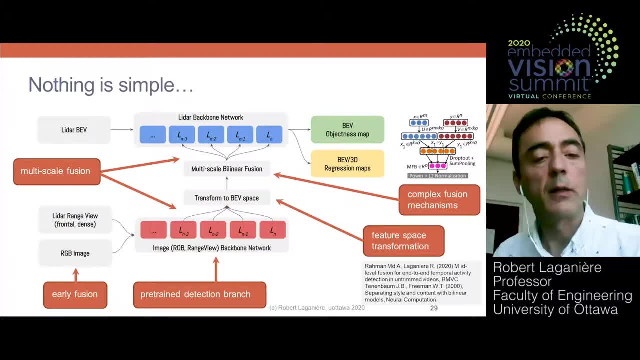 that we have designed And this shows you the different elements that we had to add In order to have our network being able to learn and to process efficiently, in that case, LiDAR and image data. So we incorporate different strategies, One of them. I just will talk about just one of them. 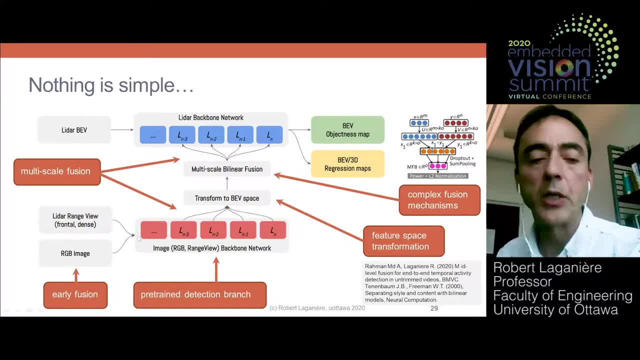 is the fact that we use an independent branch in order to process the LiDAR And And And the LiDAR data and the camera data into using an early fusion strategy, And this allows us to basically pre-train that branch before training the fusion network. 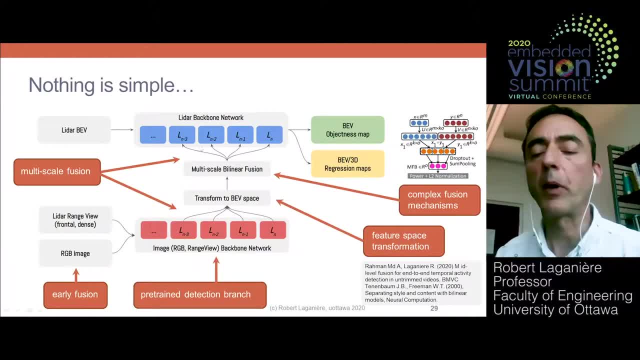 And this way, whenever after that we propagate the error, it's mainly the other network that gets corrected in order to obtain a more performing, more efficient fusion network. So again, I invite you to look at the different references to learn more about that strategy. 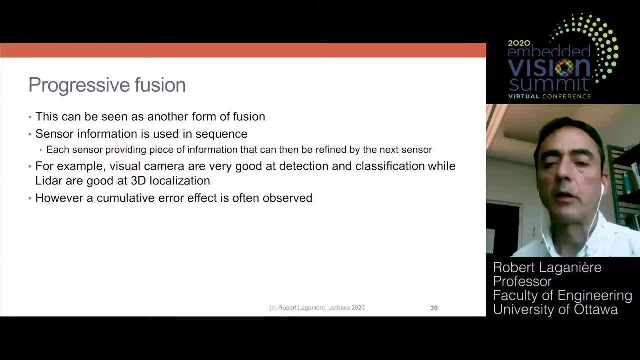 The last type of fusion approach is the sequential fusion. So this is a fusion, but in the sense that you will. you will use multiple sensors in order to get your detection result, But in this case, each sensor will be used one after the other. 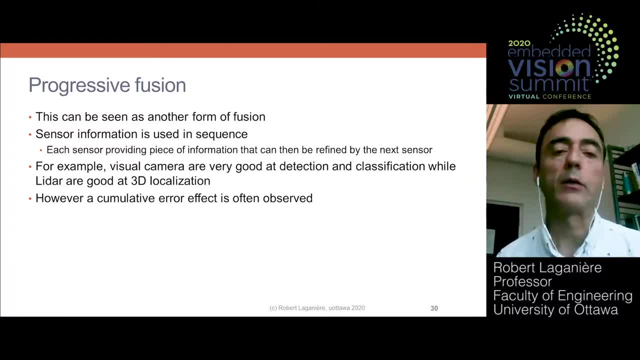 And you will. the idea is really to exploit the strength of each network to guide the decision of the next one. For example, we know that a visual camera is very good at detection. What LiDAR? why LiDAR is good? 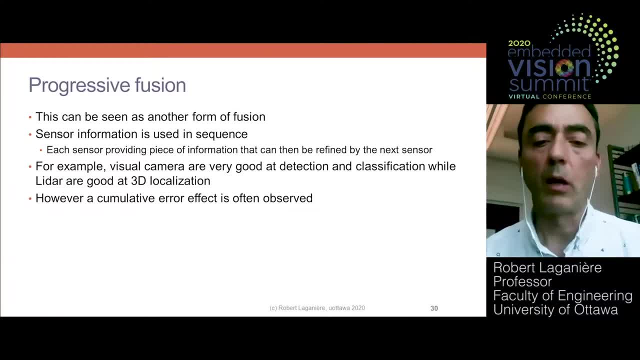 It's good at 3D localization, So there's a way to benefit from these different properties. But one of the risks is that, since we are using each network, each sensor, one after the other, well, we might get an accumulation of error. 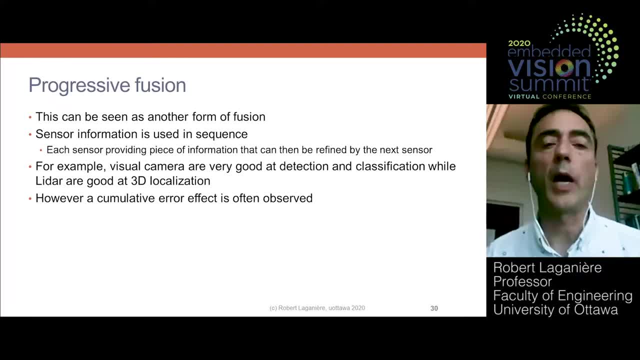 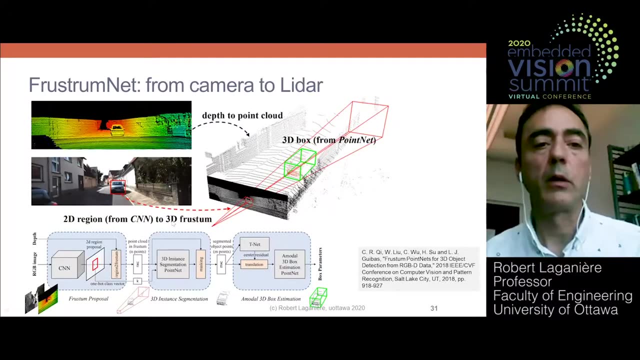 So whenever one sensor output a wrong result, that result might propagate to the other sensor Right. So that's the processing of the other network. Just to give you an example, this is the Froston network. the Froston net, which is a recent approach that really 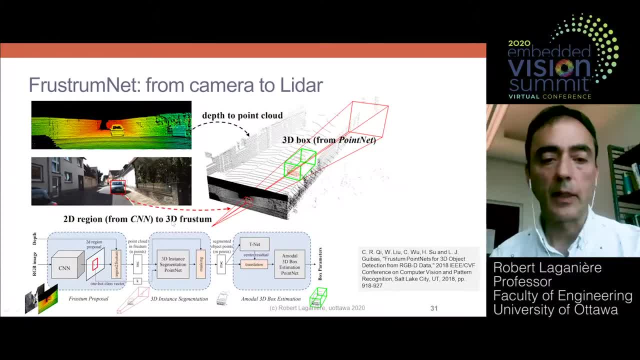 use sequential fusion. In that case, the idea is to use the camera information in order to locate. So if you have any potential object in the scene, when you have the detection in 2D you can you then construct a, build a representation. 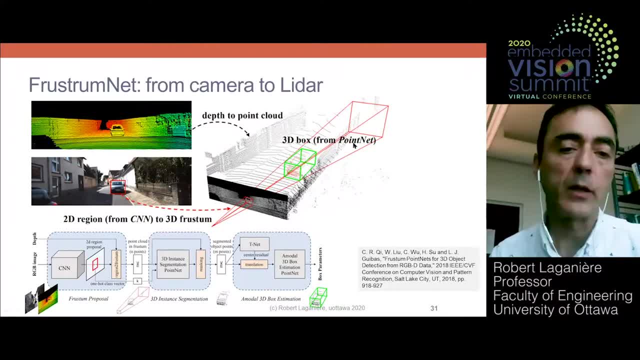 of that 2D detection into the point cloud generated by your LiDAR, for example. So you know that this 2D object is somewhere within that Froston of the point cloud. You train another network in order to detect 3D object within that 3D Froston. 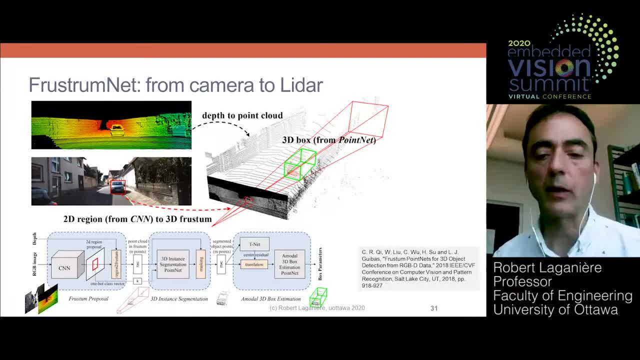 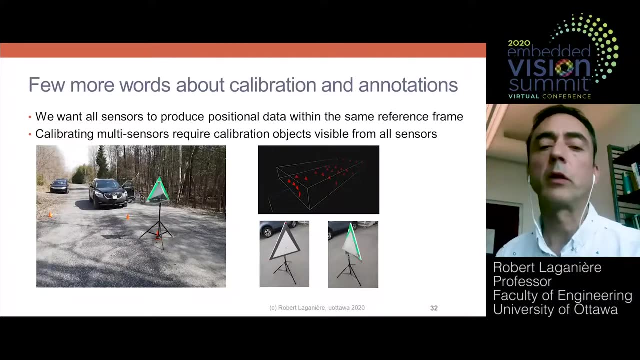 So very good results were obtained by using that sequential approach And, again, you can refer to this paper if you want to learn more about this approach. So before we finish our discussion on sensor fusion, I just want to add a few words about the calibration. 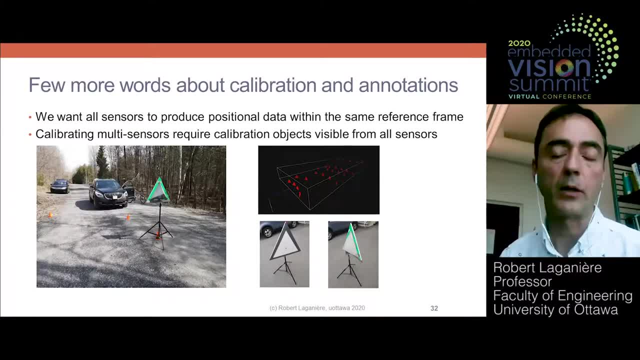 and annotation issue. So this is very important to train a neural network. But in the context of multi-sensor fusion this become more challenging. So the idea is that if you want to calibrate your multi-sensor system, you must have or you must use object. 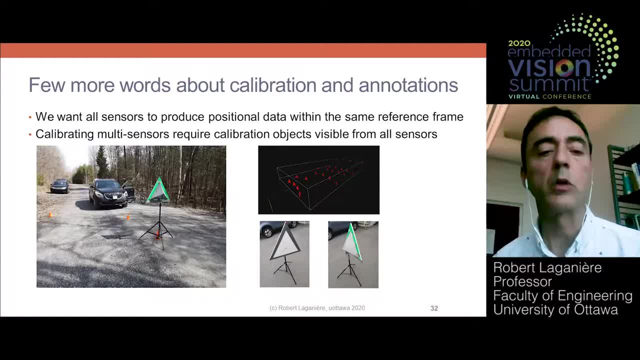 That are visible from these multiple sensor at the same time. So, for example, if you have a camera, LiDAR and radar system, you could use a calibration object like this one, which is made of what we call a reflector cone, which. 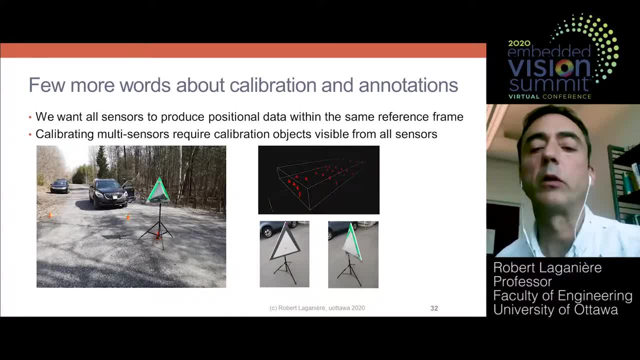 is able to strongly reflect the radar signal. LiDAR will also be able to see that object because there is a planar form that has been fixed in front of the corner reflector And obviously the camera also will be able to see that object. 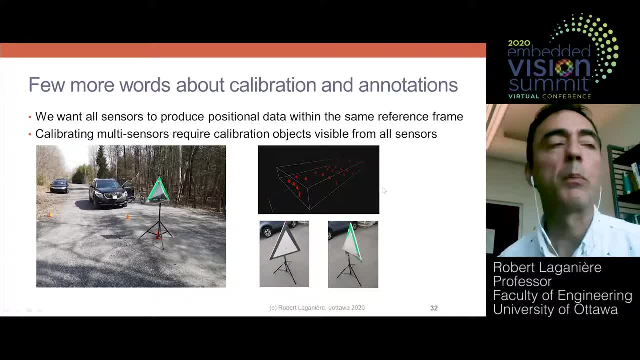 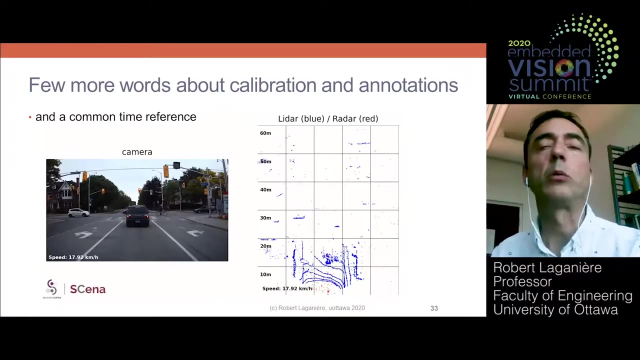 So this way you are able to generate a representation of this calibration object that you move over the scene And you have That object capture simultaneously by all the sensor. So this way, if, in addition, you were able to get these sensors synchronized- 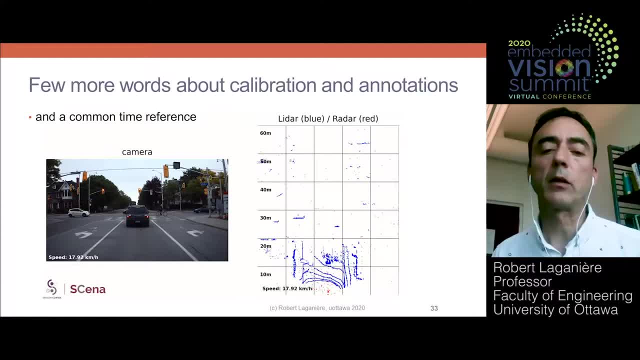 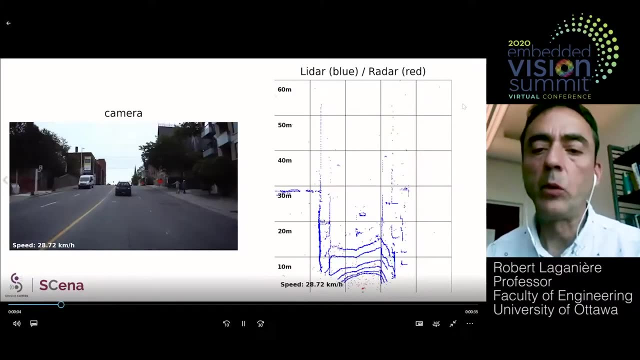 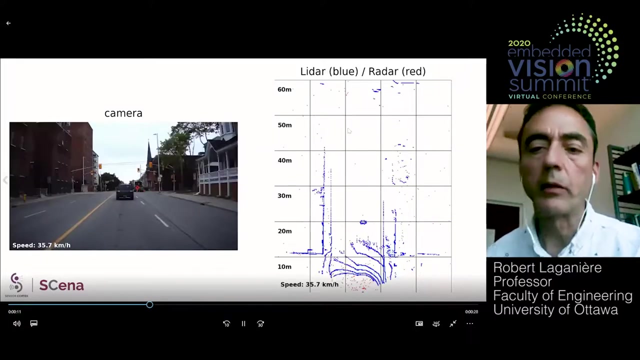 you will be able to generate a data set where that will contain synchronized information from LiDAR camera and radar. So here is a video where you have in blue the result from the LiDAR In red. so the few red points that you see. 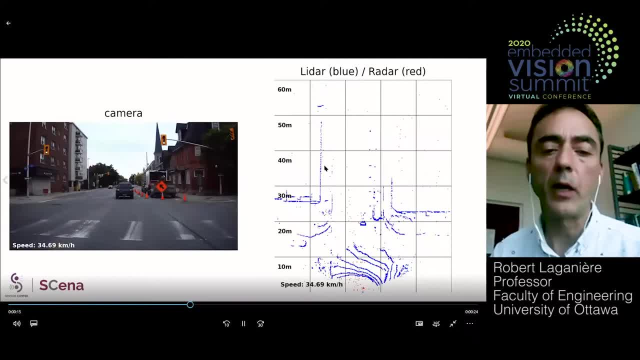 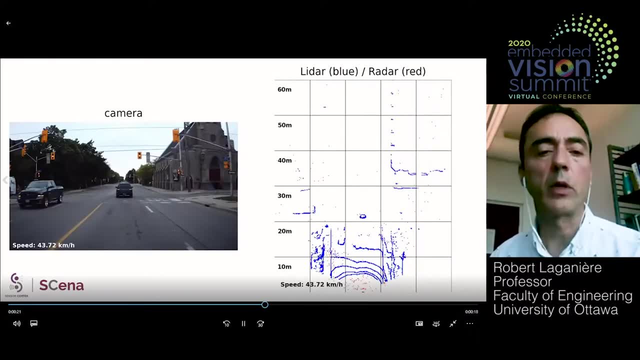 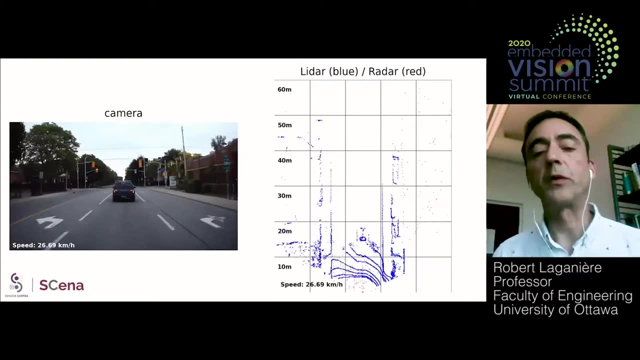 correspond to the point cloud obtained from the radar, And you have the image information as well. So everything is synchronized and overlaid onto the same presentation. So this way you can use that signal, that multisignal, So you can use that multisignal signal. 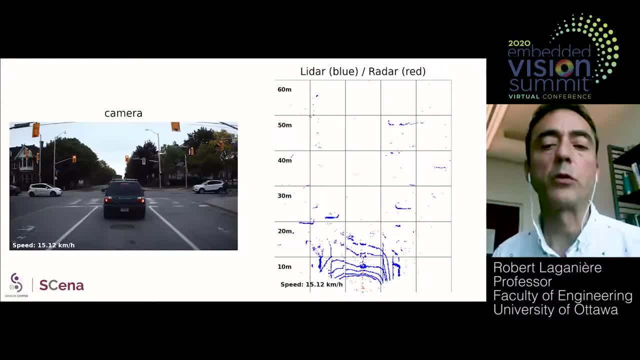 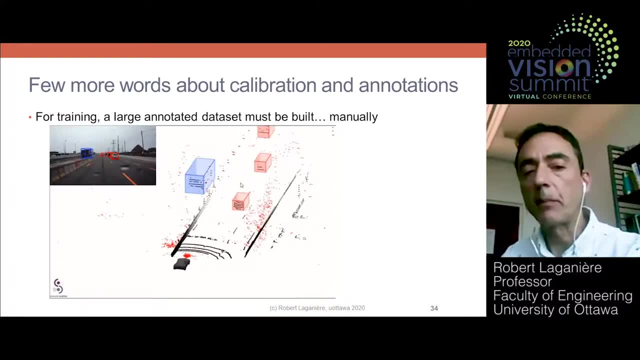 and input it to your multisensor fusion system. So once you have your multisensor data, so the next step is to be able to build an annotated data set from this multisensor data. So you certainly need to have an annotation tool at your disposal. 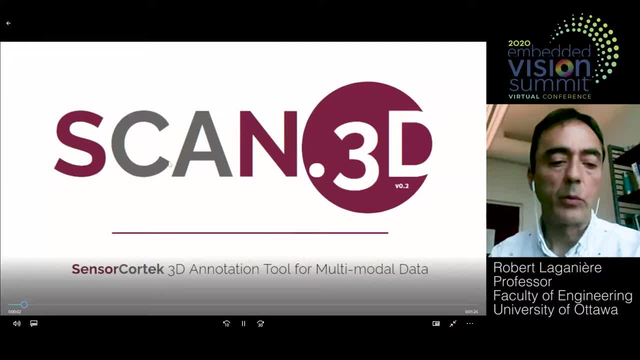 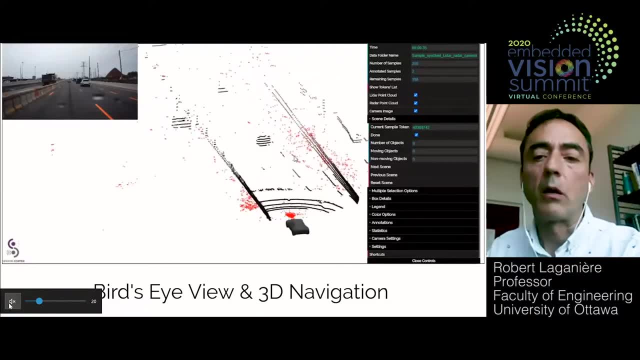 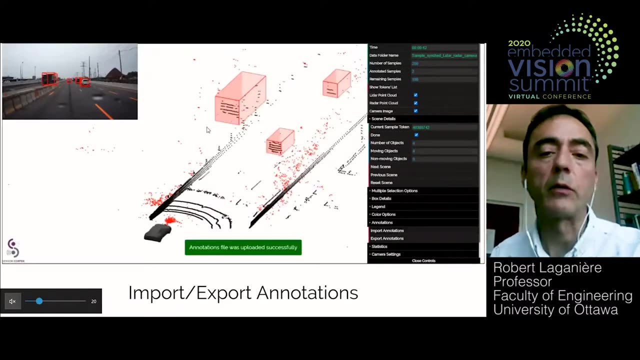 So here is an example. This is a tool that we developed at SensorCortex. It consists of a 3D web application that is able to display the multisensor data into one frame And, as you can see, whenever you have a 3D box. 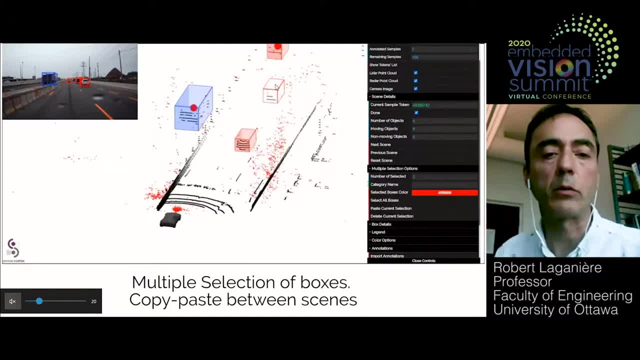 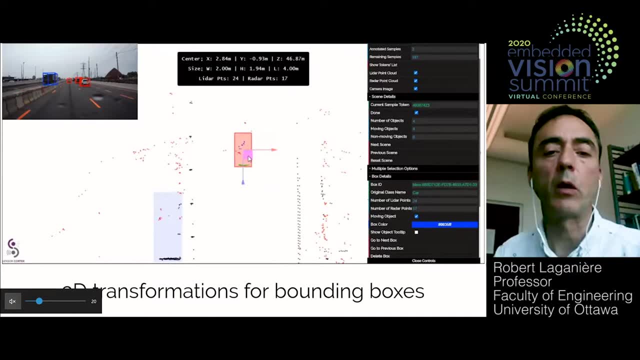 and you select that box, you can move it, And when you move it, you can move it, And when you move it, you can move it. I mean, the information will be projected as well onto the camera image, So you really have annotation in that case. 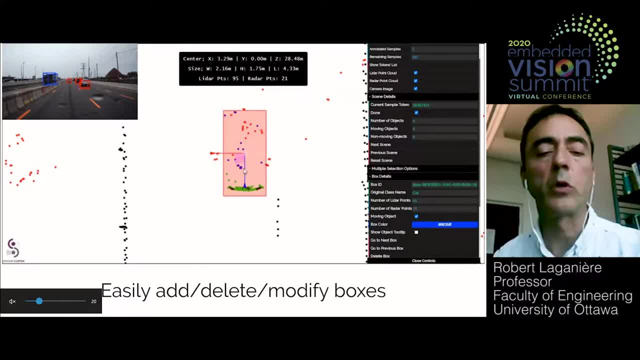 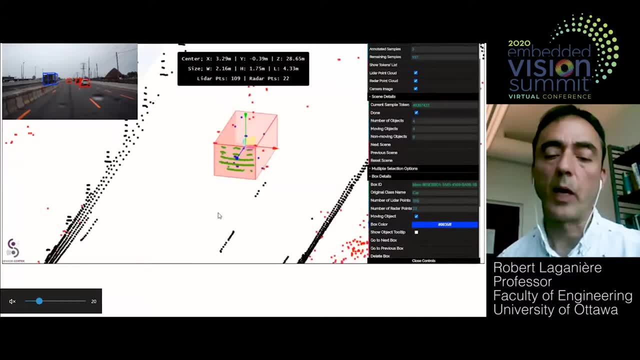 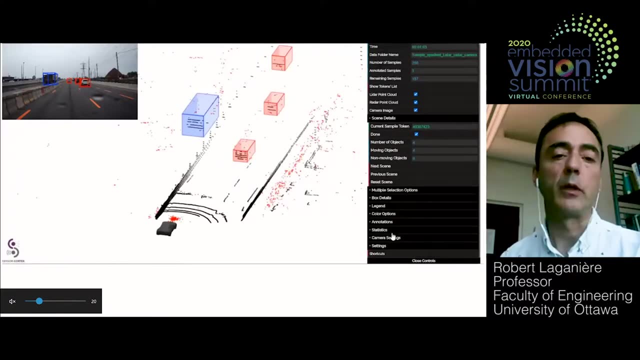 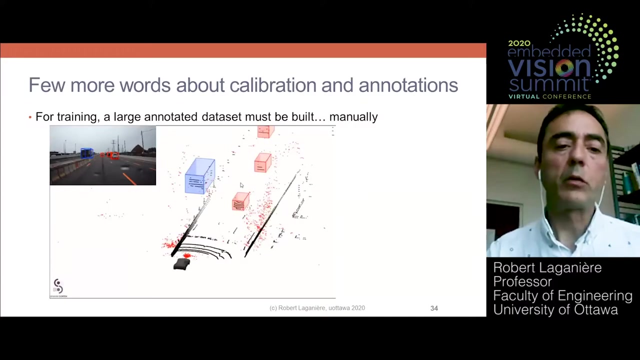 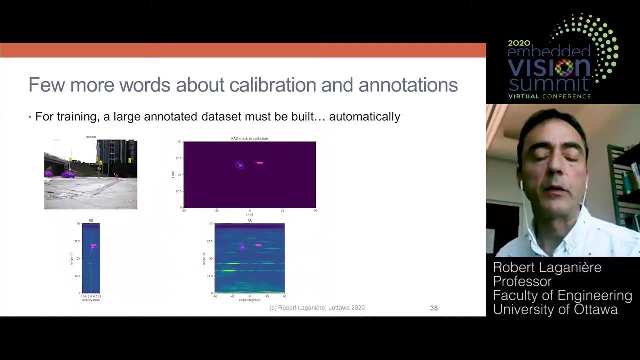 that are simultaneously reprojected onto each sensor. So this is quite an extensive task, but that way this is the only way you can get a very reliable annotated data set. But there is also another way of obtaining annotated data, and this can be done using some neural network that you train. 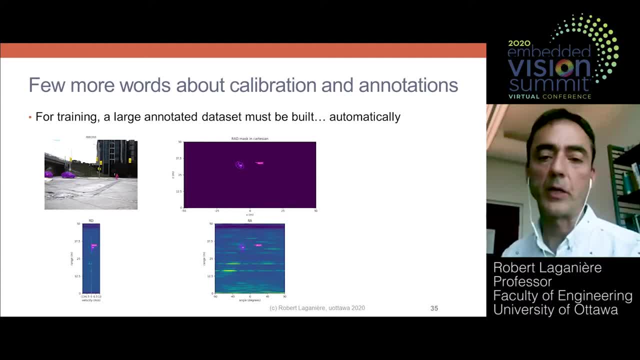 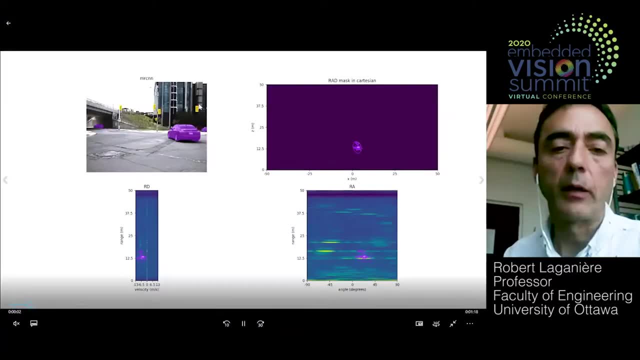 in order to build, to pre-annotate the information. Let me show you an example of that. So, in that case, what we did? we used, you know, we used- a 3D model of the multisensor data. We used a 3D model of the multisensor data. 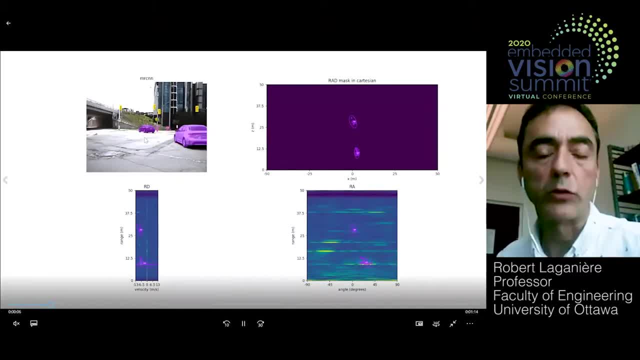 a stereo system of camera. here you just see one image of that stereo system and we use a network that process that image in order to detect the object of the scene. so, in that case, the object of the scene being the pedestrian and and the cars. so the segmentation we obtain once we obtain 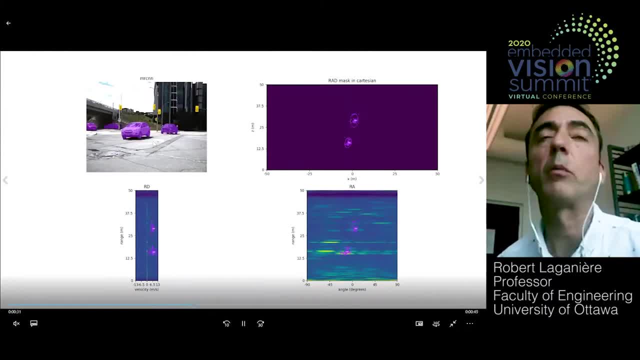 the segmentation from the stereo we are able to get the range information, the distance to the camera. so, uh, that way we are able to reproject that uh 2d and 3d information, 2d plus range information, onto each representation of, in that case, the radar data. so i showed you earlier the 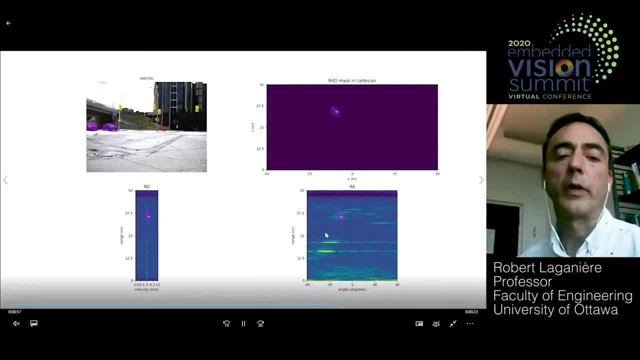 different possible representation for for radar and, as you can see, the label so pedestrian car are reprojected automatically onto each of these representations. so this is a way to completely automate the process of annotation from multi-sensor. but in order to do that you need to have a accurate uh calibration of your of your sensor. 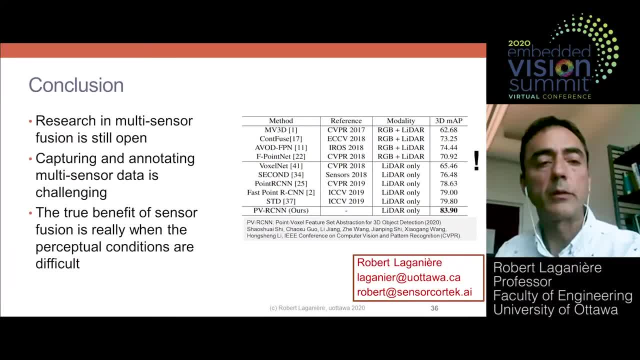 okay, so, uh, just to uh summarize, so the research on in multi-sensor fusion is is still an open subject. uh, it's still very difficult to obtain a good multi-sensor uh fusion system. uh, one of the challenges is obviously to be able to capture and annotate data from multi-sensor uh. and remember what we said: why do we want to perform? 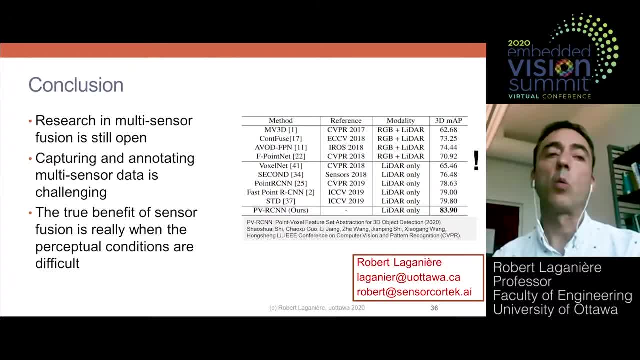 multi-sensor fusion because when the perception environment is become more challenging, when to perceive accurately the environment become more challenging, then you need to rely on the information from multiple sensors. the fact is that the current research done uh often use data set that are of good quality. 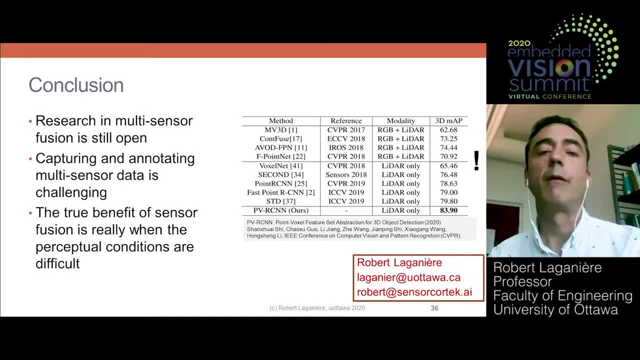 by that i mean that i said capture on the fair weather condition during the day. so for that reason you will often see single sensor solution that perform better than a state-of-the-art multi-sensor solution. this is just an example that i have extracted from the this year conference on computer vision and 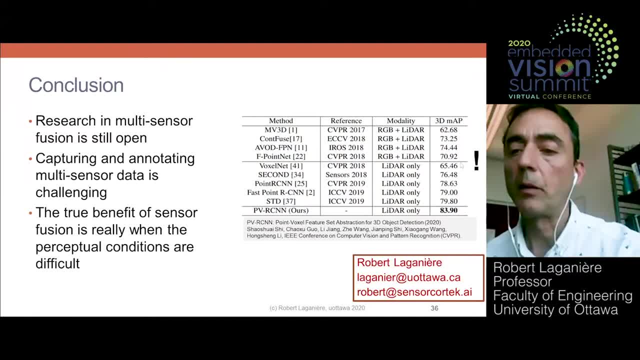 and pattern recognition. it shows that one method here was able to surpass- and this is a method that use lidar only- was able to surpass the result from rgb, from camera plus lidar data. and again, this is because basically the data set that is used to measure these performance. 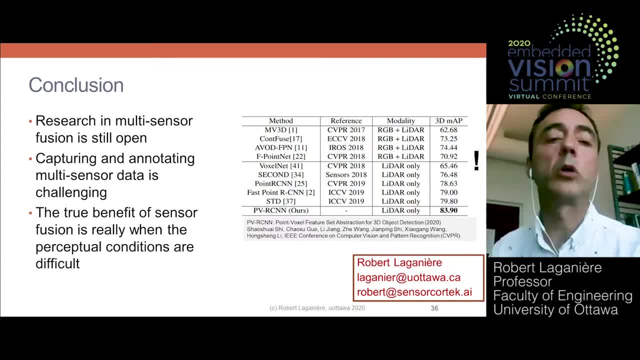 is of too good quality for multi-sensor to really to really surpass the single sensor, so we still need to progress on multi-sensor fusion. but multi-sensor fusion is key when the environmental conditions are challenging and we need to build data set that contain this more difficult driving condition. 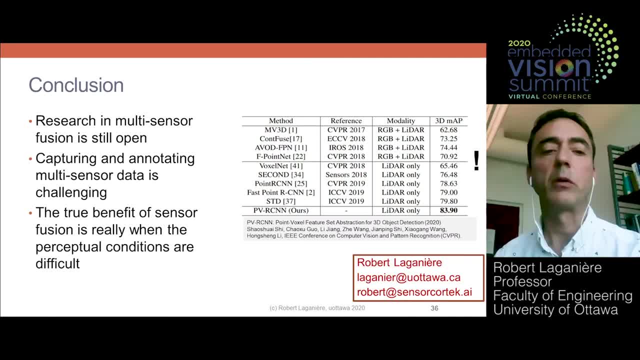 on that. thank you for your attention.